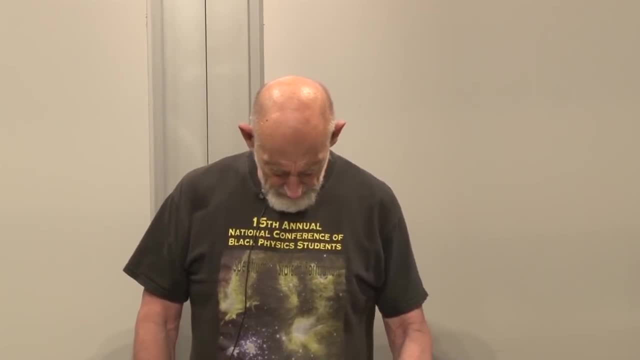 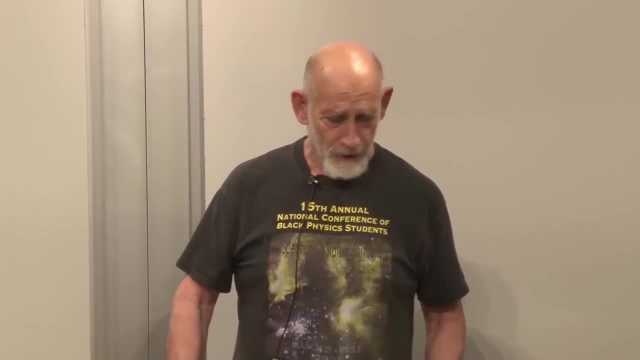 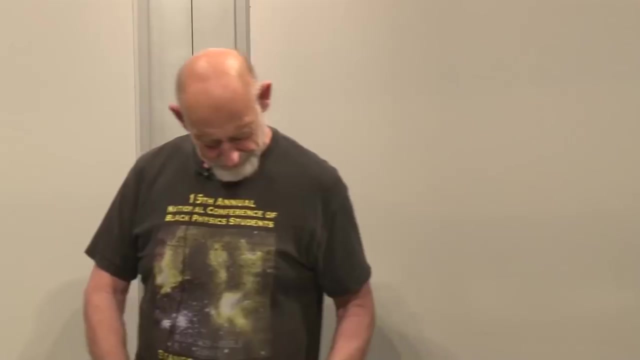 the world as we know it, And in fact without statistical mechanics we probably would not know about the Higgs boson. So with that little starting point, Combat mechanical throwing makes a lot of sense. What is statistical mechanics about? 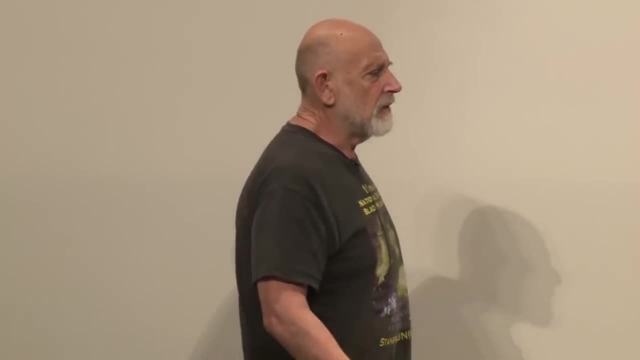 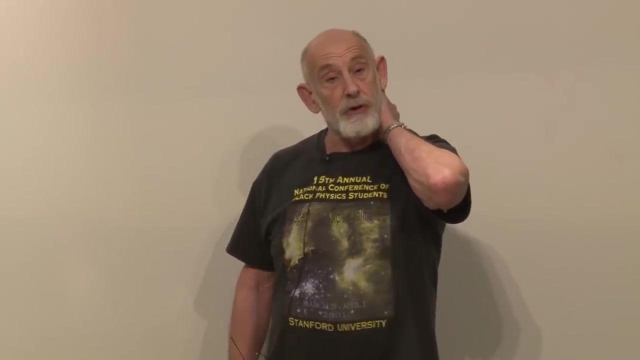 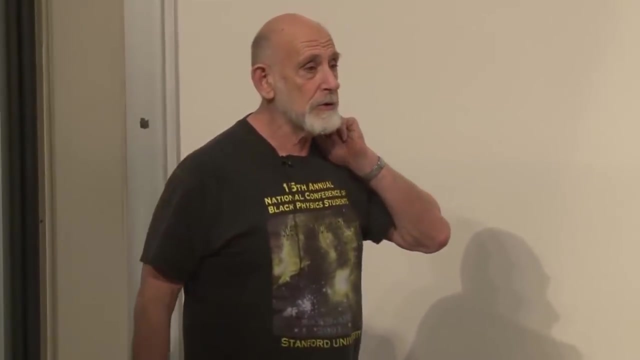 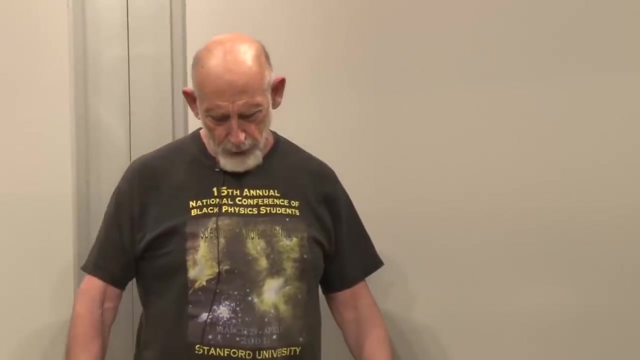 Well, let's go back a step. The laws of physics, the basic laws of physics, Newton's laws, principles of classical physics, classical mechanics, the things that were in classical mechanics' course, quantum mechanics and so forth, those things are all about predictability, perfect predictability, пол. 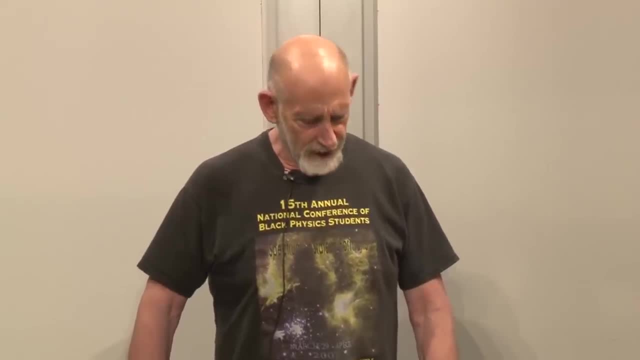 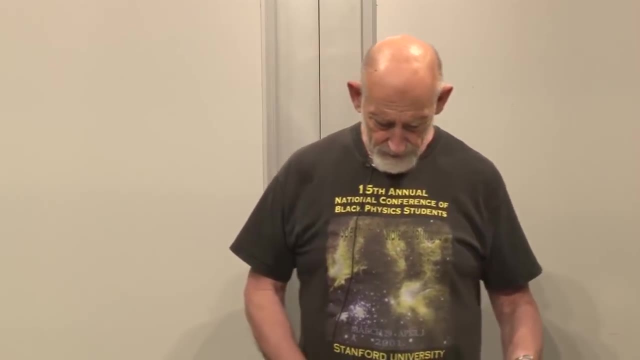 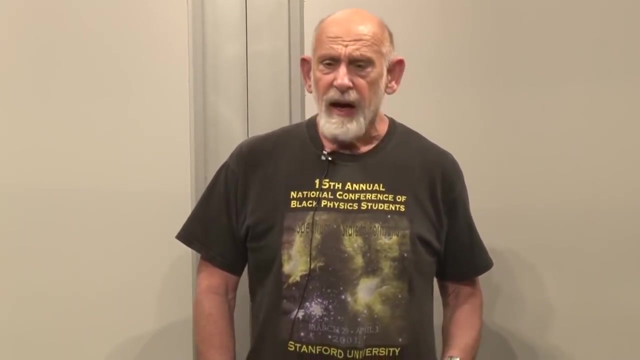 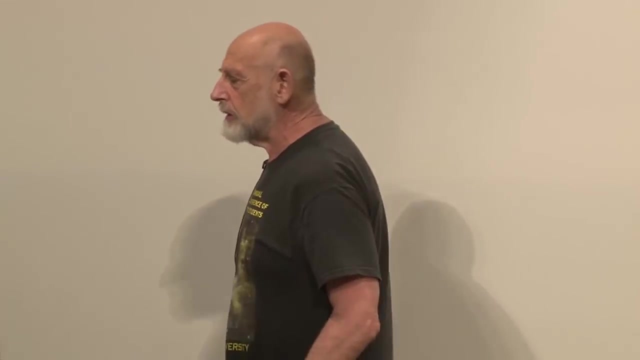 well, in quantum mechanics you can't predict perfectly, And that's true. but there are some things you can predict perfectly, And those things are the predictables of quantum mechanics. Again, as in classical mechanics, you can make your predictions with maximal. 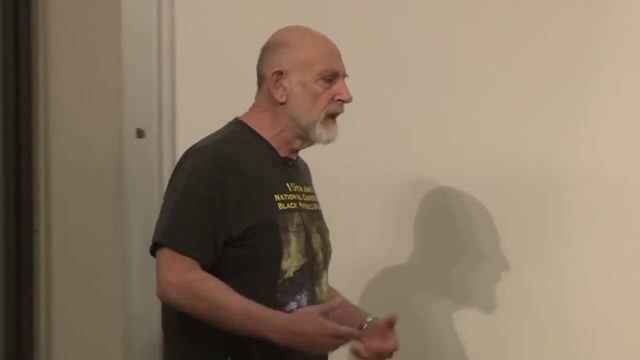 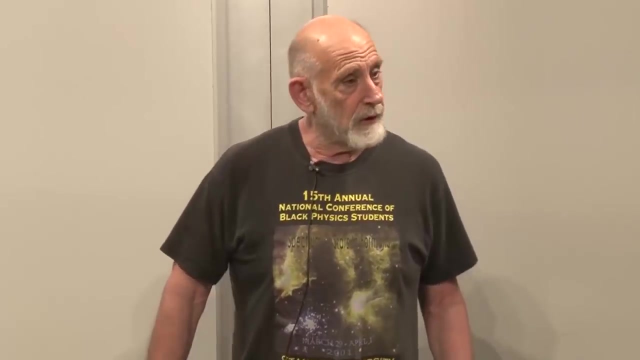 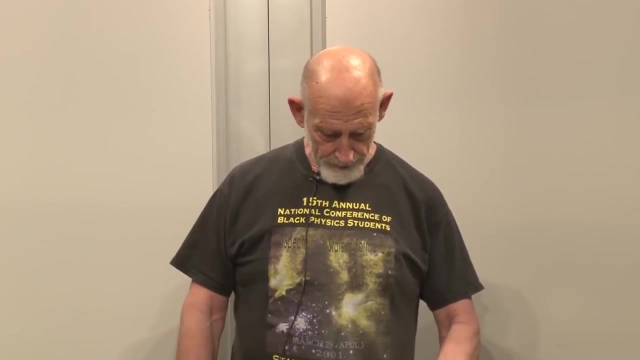 let's call it maximal precision or maximal, whatever it is- predictability. if you know two things: If you know the starting point, which is what we call initial conditions, and if you know the laws of evolution of a system, If you can measure the, or if you know, for whatever reason, 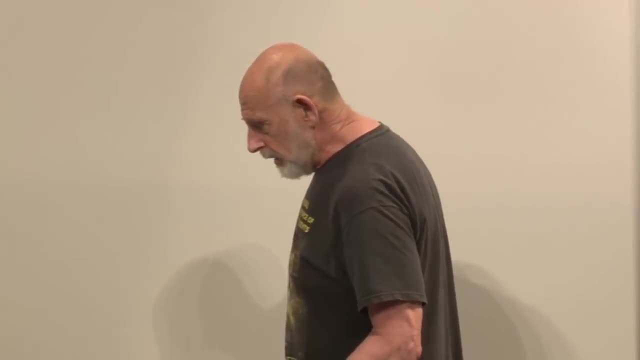 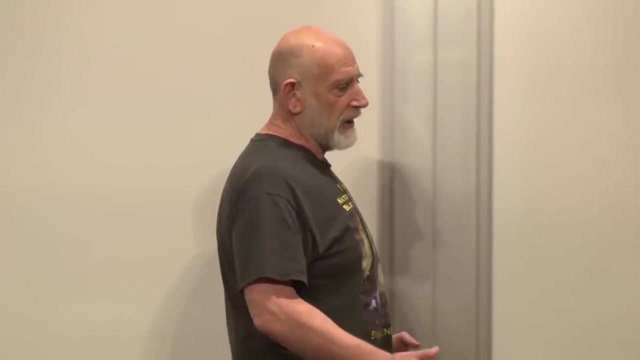 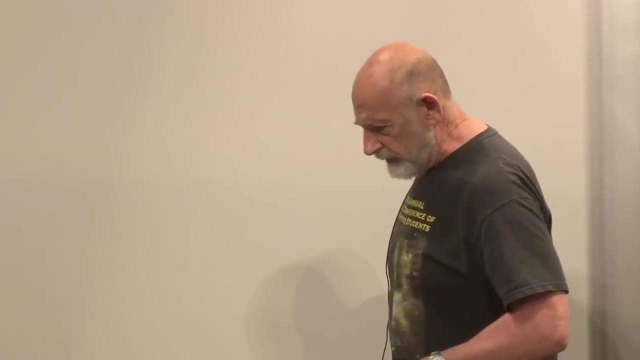 the initial starting point of a closed system. a closed system means one which is either everything or it is sufficiently isolated from everything else that the other things in the system don't influence it. If you have a closed system, if you know the initial conditions exactly, 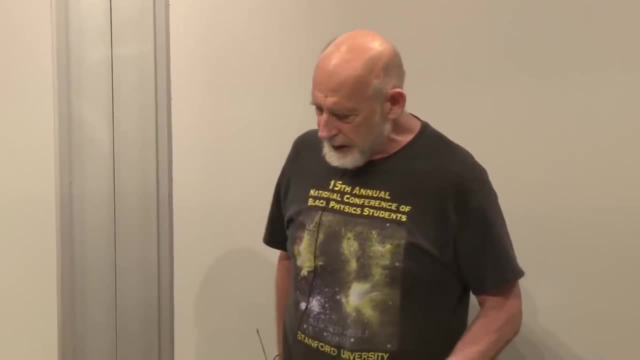 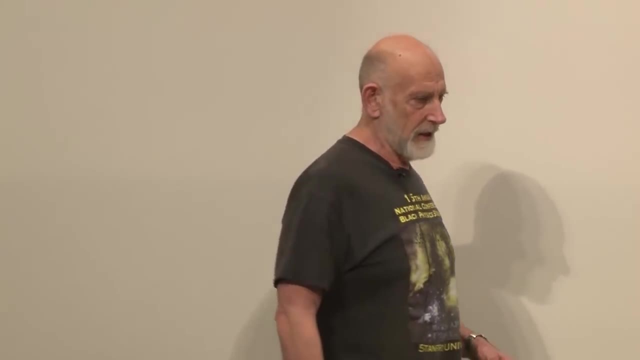 or at least with whatever precision is necessary, and you know the laws of evolution of the system. you have complete predictability, And that's all there is to say Now. of course, in many cases that complete predictability would be totally useless. 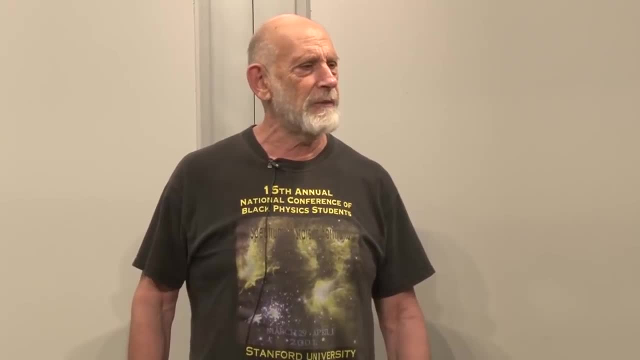 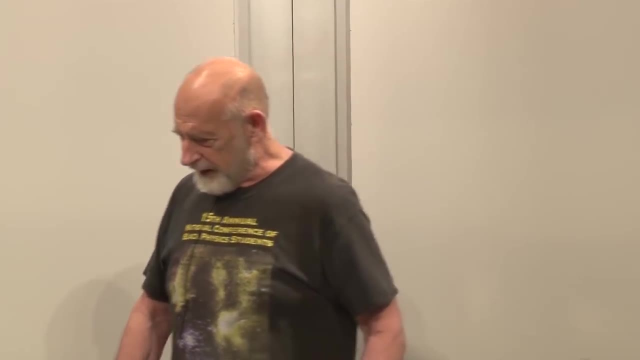 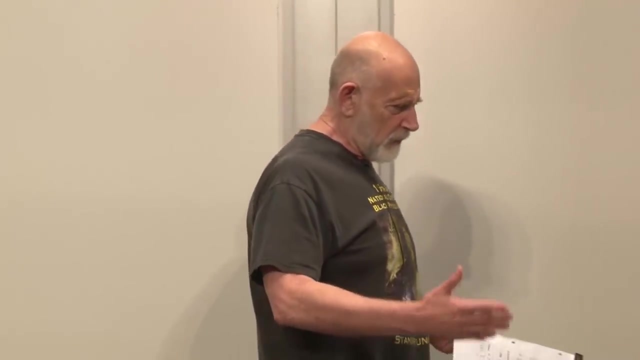 Having a list of the position and velocities of every particle in this room would not be very useful to us. The list would be too long and subject to rather quick change, as a matter of fact. So you can see, while the basic laws of physics 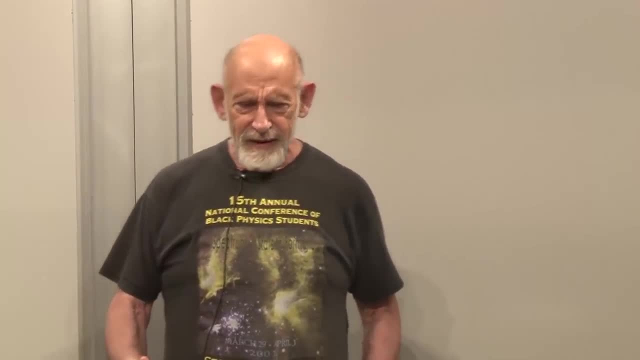 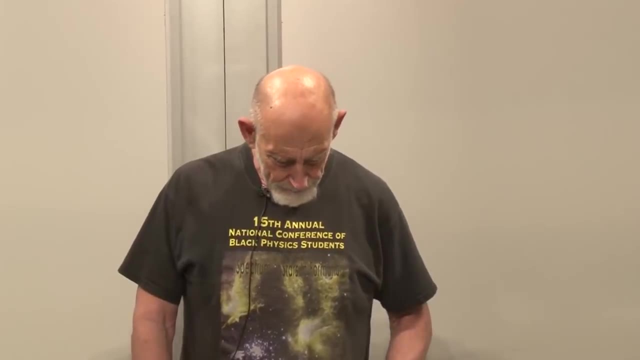 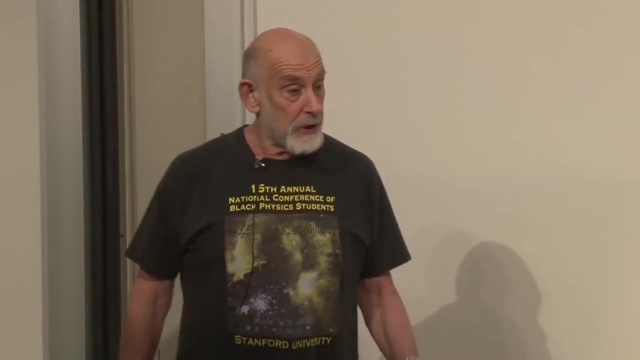 are very, very powerful in their predictability, they also in many cases can be totally useless for actually analyzing what's really going on. Statistical mechanics is what you use Basically: probability theory, Statistical mechanics. let me say first of all: 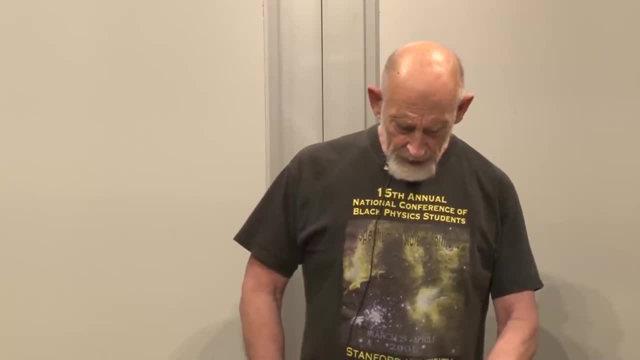 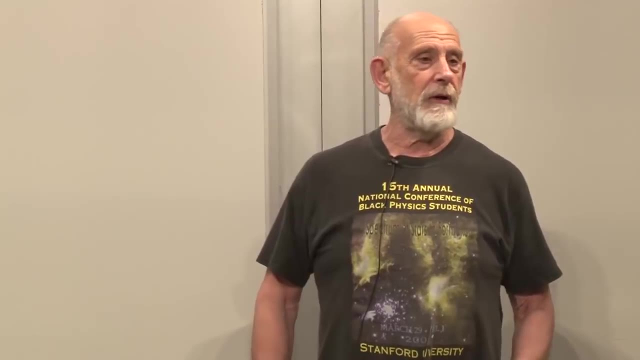 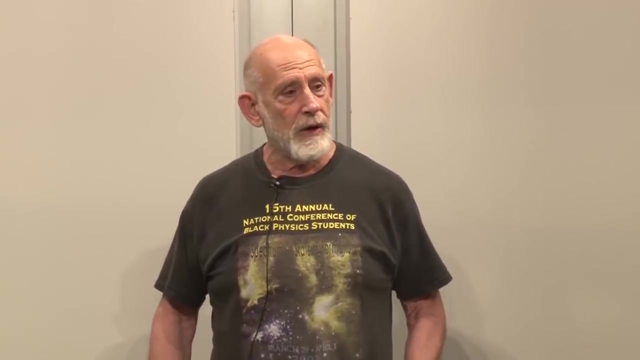 it is just basic probability theory, Statistical as applied to physical systems. But when is it applicable? It's applicable when you don't know the initial conditions with complete perfection. It's applicable when you it may even be applicable when you don't know the initial conditions. 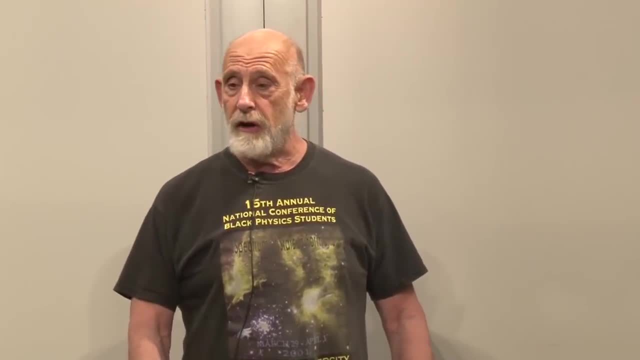 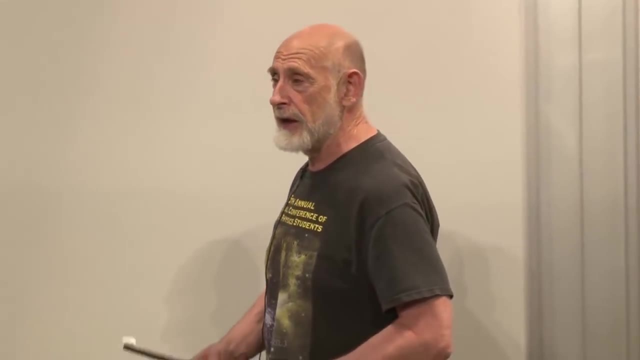 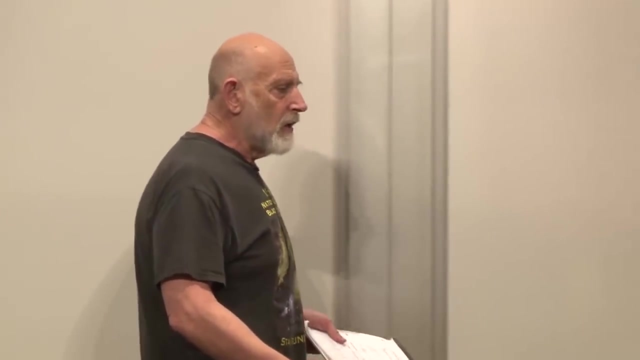 It's applicable if you don't know the laws of motion with infinite precision, And it's applicable when the system you're investigating is not a closed system, whether it's interacting with other things on the outside, In other words, in just those situations where ideal predictability is impossible. 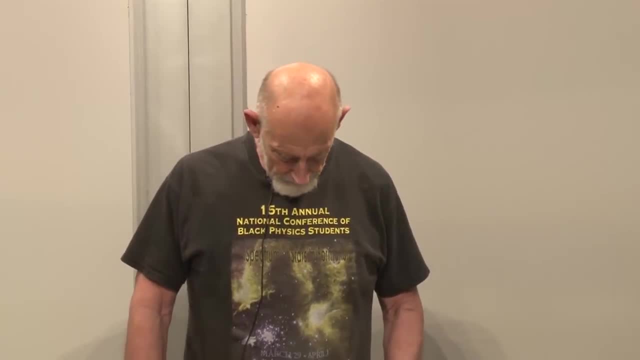 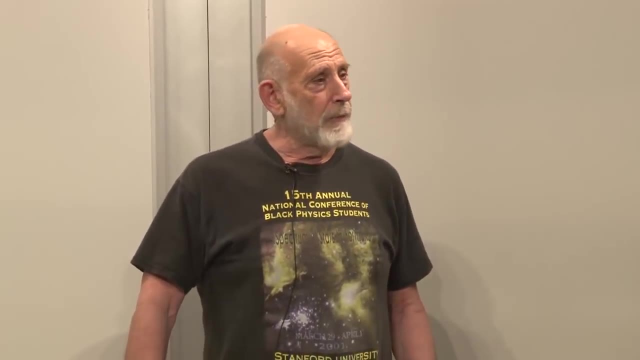 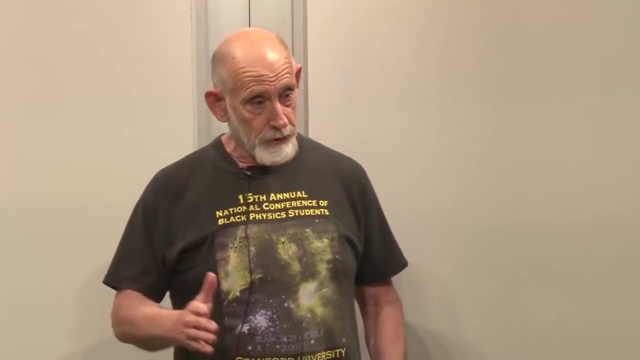 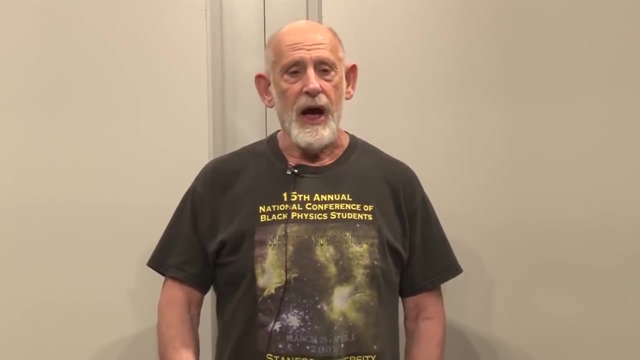 Then what do you resort to? You resort to probabilities, But because the number of molecules in this room is so large and probabilities tend to become very, very precise predictors when the laws of large numbers are applicable, statistical mechanics itself can be highly predictable, but not for everything. 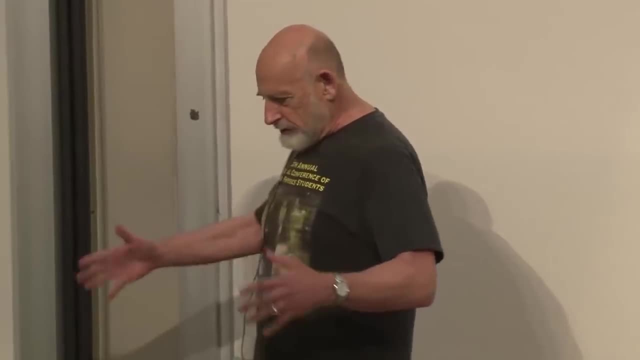 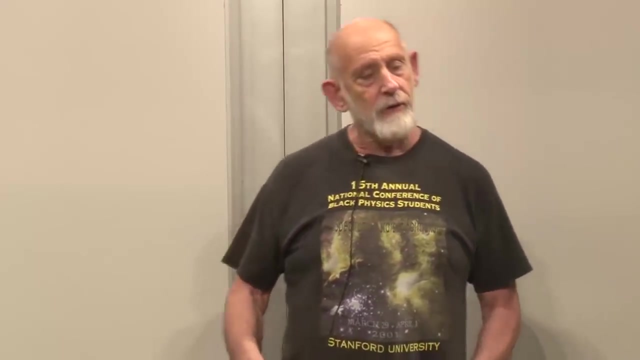 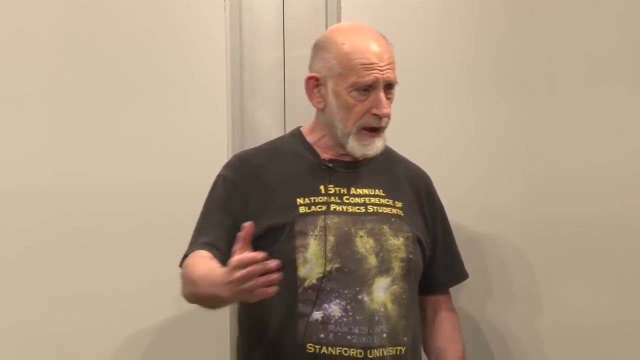 As an illustration, you have a box of gas. The box of gas might even be an isolated, closed box of gas. It has some energy in it. The particles rattle around. If you know some things about that box of gas, you can predict other things with great precision. 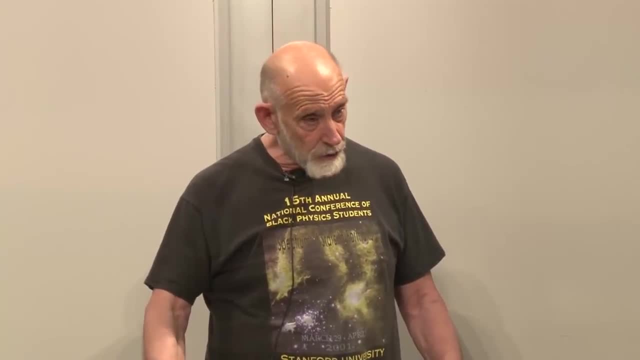 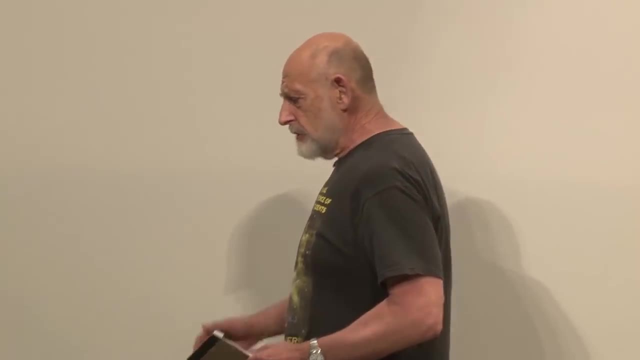 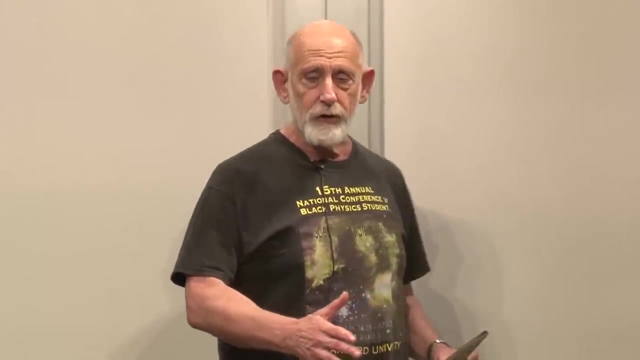 If you know the temperature, you can predict the energy in the box of gas, You can predict the pressure. These things are highly predictable. but there are some things you can't predict. You can't predict the position of every molecule. You can't predict when there might be a fluctuation. 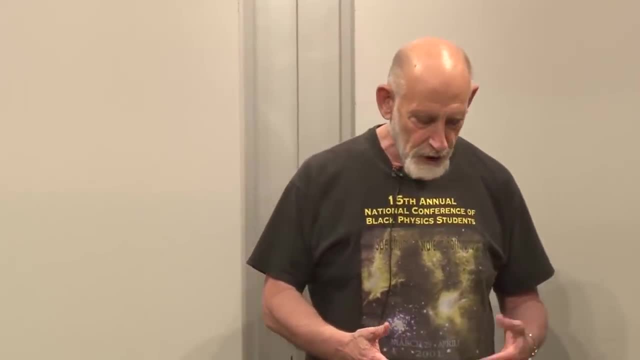 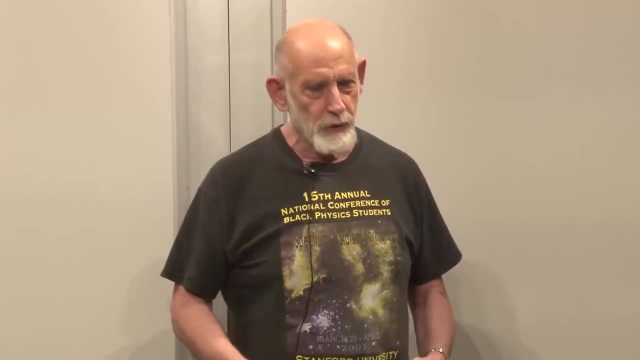 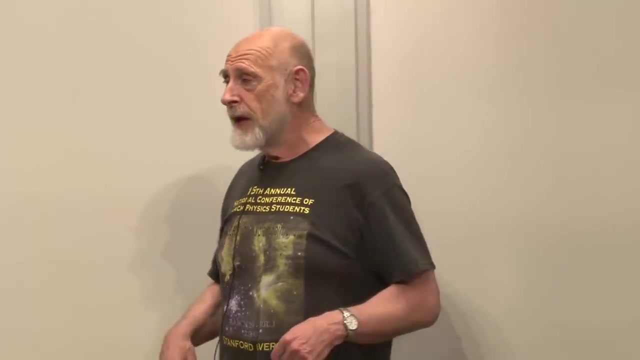 Fluctuations are things which happen which don't really violate probability theory. They're the sort of tails of the probability distribution, things which are unlikely but not impossible. Fluctuations happen from time to time in a sealed room, every so often An extra large group. 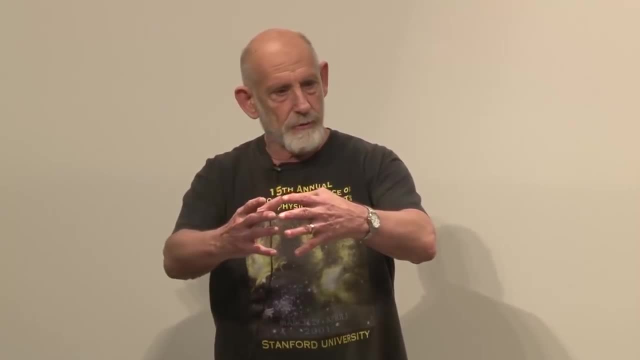 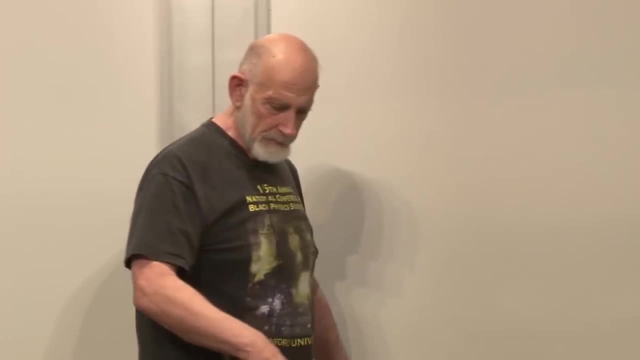 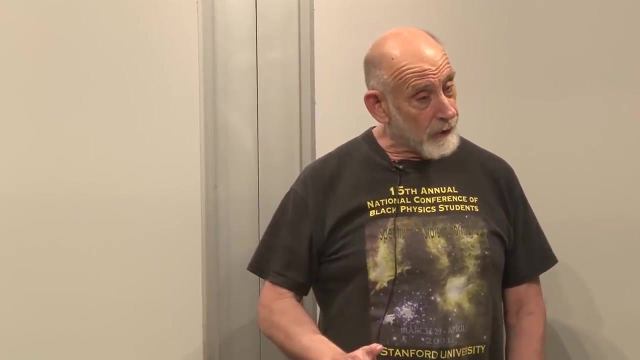 an extra large density of molecules will appear in some small region bigger than the average. someplace else, Molecules will be less dense And fluctuations like that are hard to predict. You can predict the probability for a fluctuation, but you can't predict when a fluctuation is going to happen. 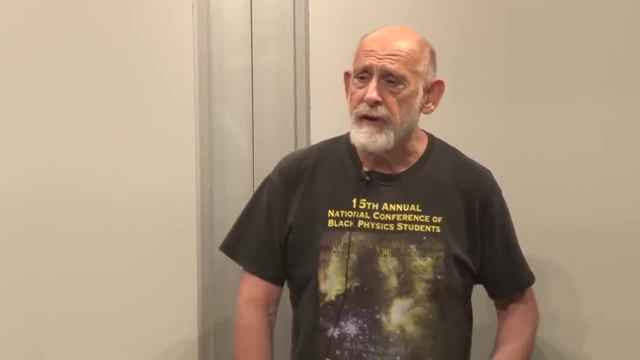 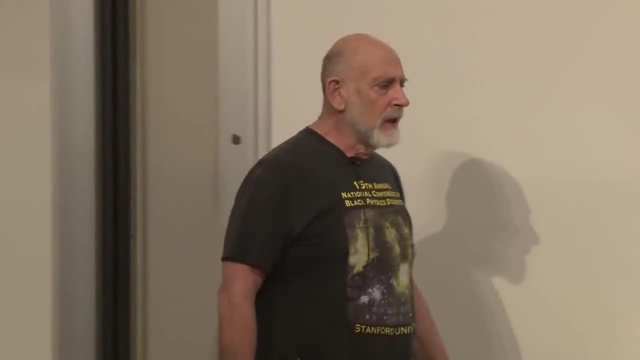 It's exactly the same sort of thing as flipping coins. Flipping coins is a good example. It's probably our favorite example. It's a good example for thinking about probabilities. If I flip a coin a billion times, you can bet that approximately half of them will come up heads. 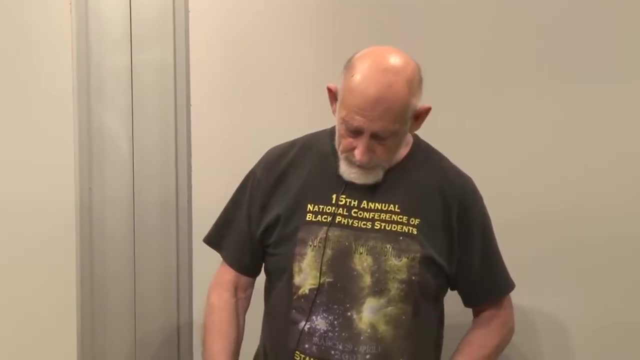 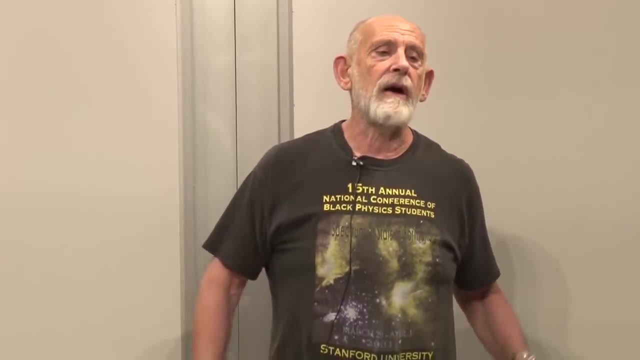 and half will come up. tails within some margin of error, But there will also be fluctuations Every now and then. if you do it enough times, a thousand heads in a row will come up. Can you predict when a thousand heads will come up? 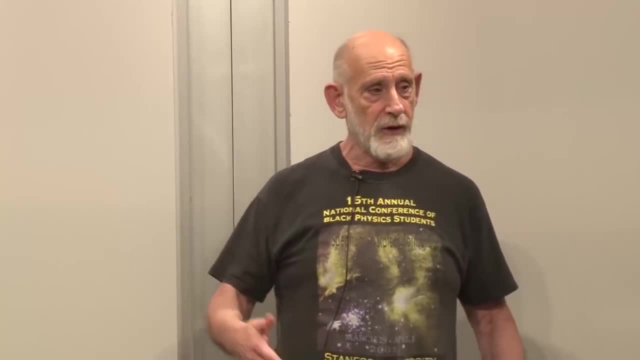 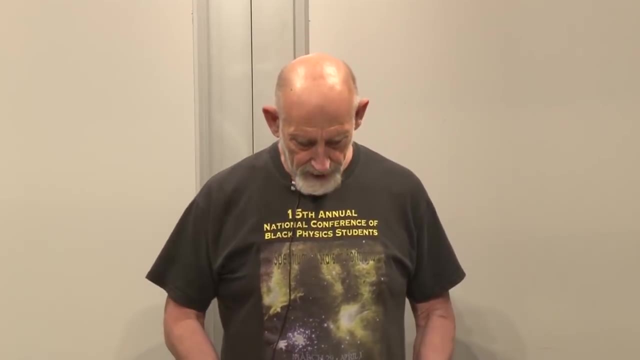 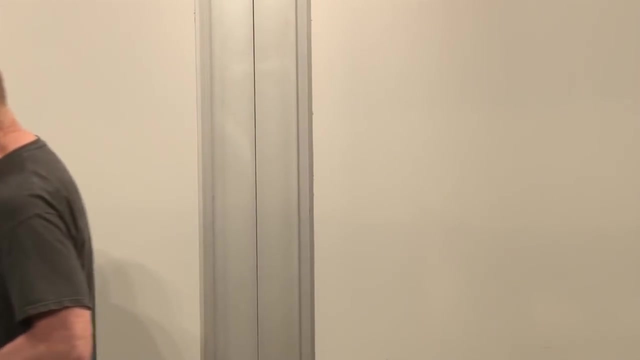 No, But can you predict how often a thousand heads will come up? Yes, Not very often. So that's what statistical mechanics is for. It's for making statistical, probabilistic predictions about systems which are either too small, contain elements which are too small to see. 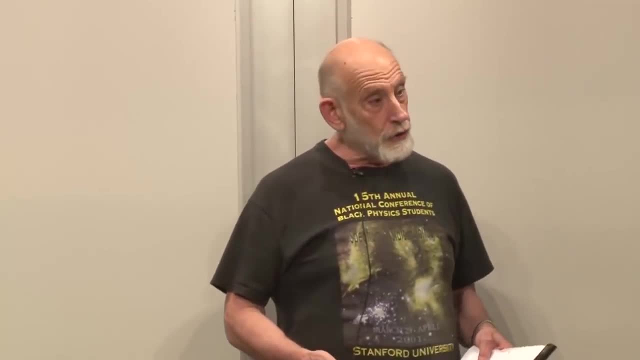 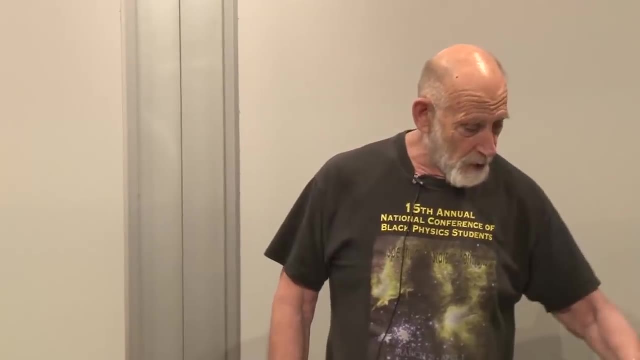 too numerous to keep track of, usually both too small to see. by see, I mean, you know, it's true, You can see some pretty small things, molecules, but so they may not be too small to see, But there are too many of them. 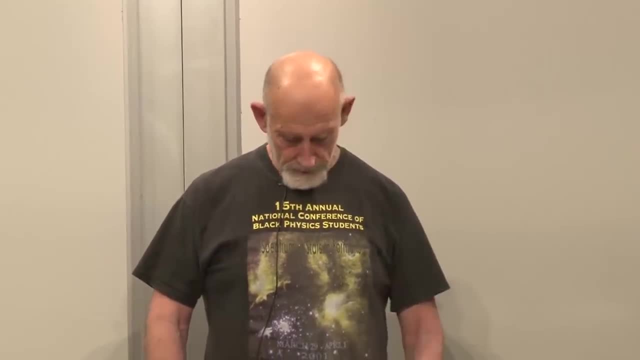 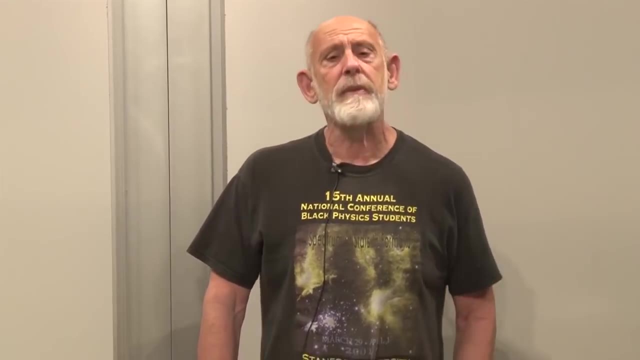 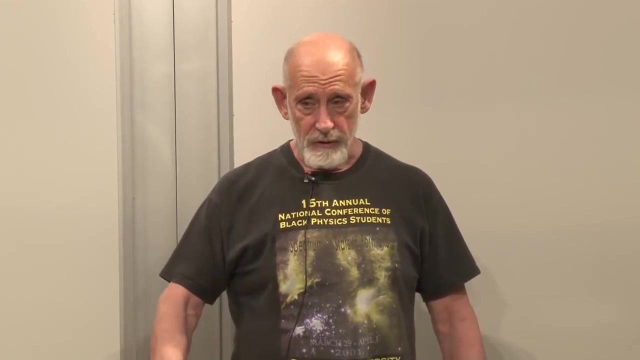 There are too many of them to keep track of, And that's when we use probability theory or statistical mechanics. We're going to go through some of the basic statistical mechanics applications- not just applications- the theory, the laws of thermodynamics, the laws of statistical mechanics. 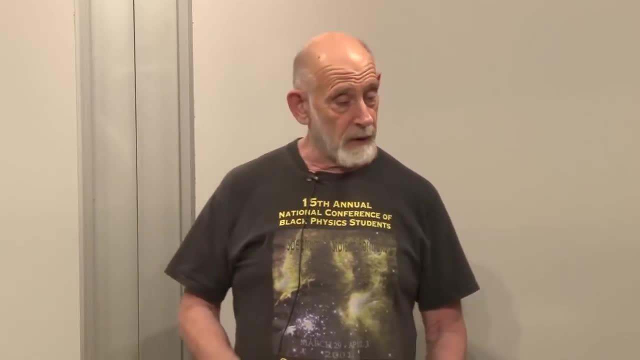 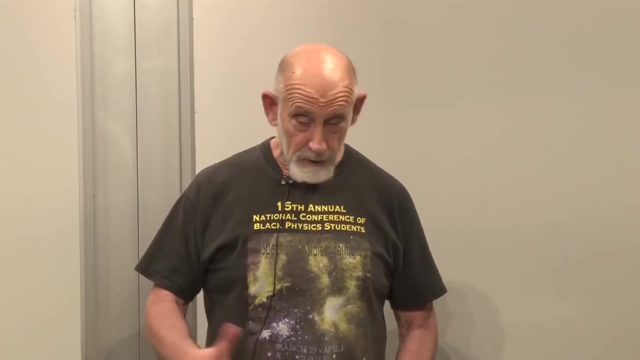 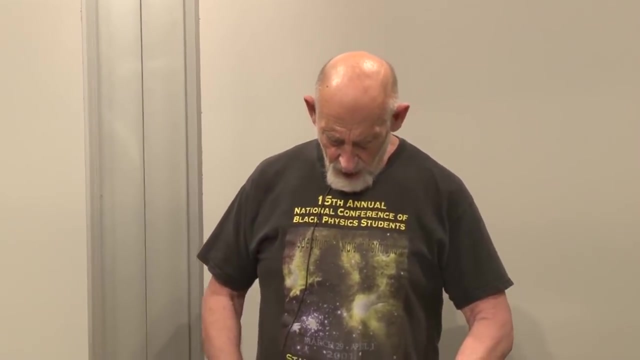 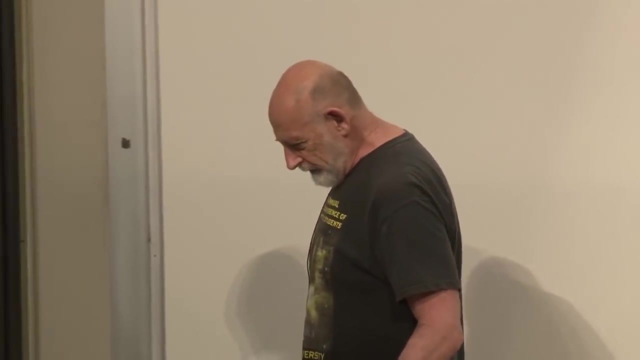 and then how they apply to gases, liquids, solids. whether we will get to quantum mechanical systems or not, I don't know, but just the basic ideas, Okay. Incidentally, another thing which is very striking is that, generally speaking, over the history of 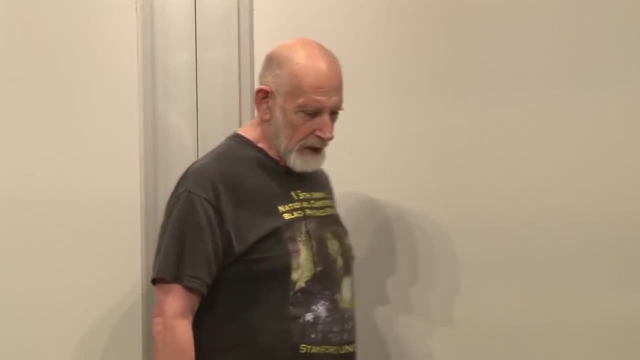 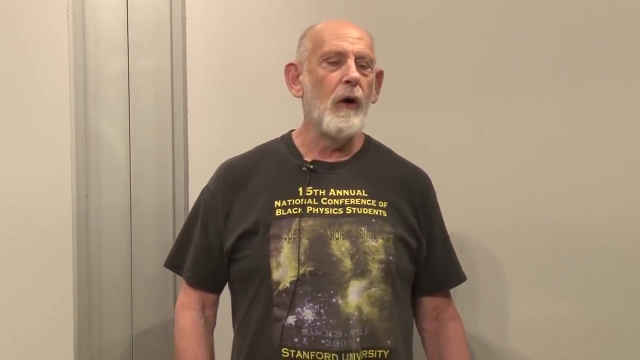 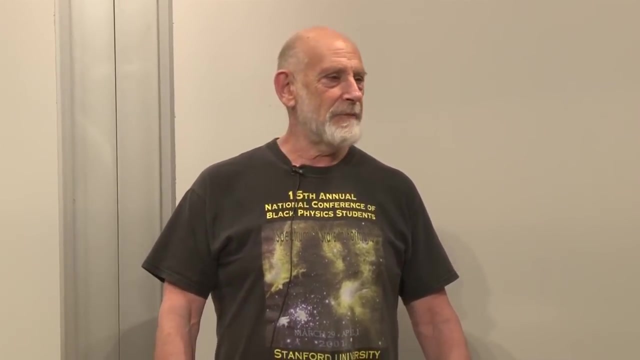 certainly over my history in physics, and I'm sure this goes back to the middle of the 19th century sometime- all great physicists- all of them were masters of statistical mechanics. It may not have been the sexiest thing in the world. 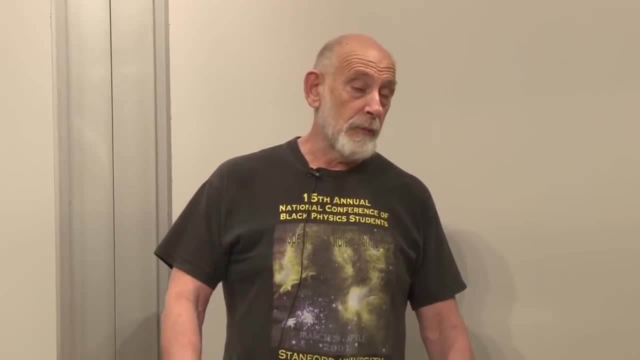 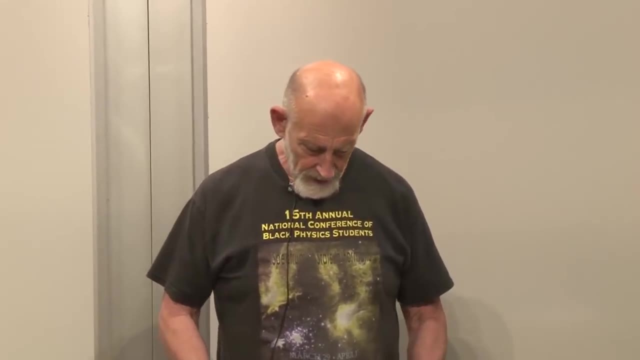 but they were all masters of it. Why? First of all, because it was useful, but second of all, because it is truly beautiful. It is a truly beautiful subject of physics and mathematics And it's hard to say it's hard not to get caught up in it. 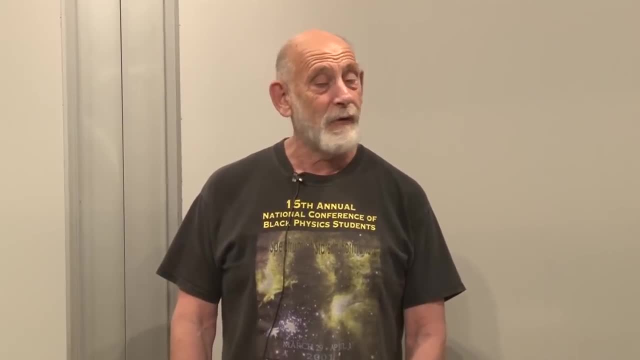 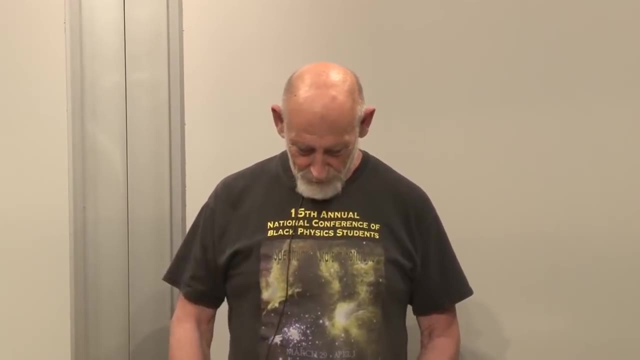 hard not to get, not to fall in love with it. The reason I teach it is not for you, it's for me. I love teaching it, I love teaching it. I teach it over and, over and over again and in a sense, my life has consisted of learning. 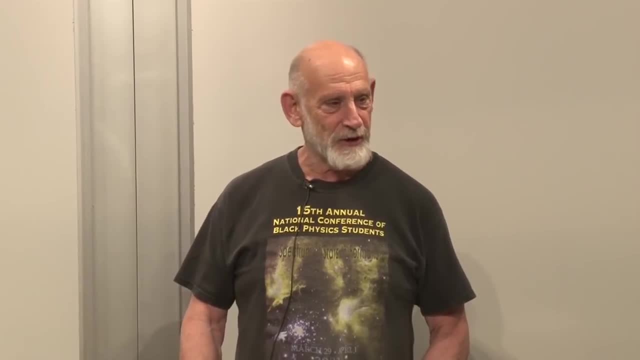 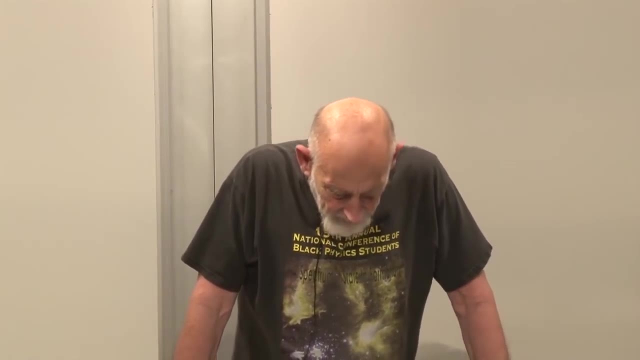 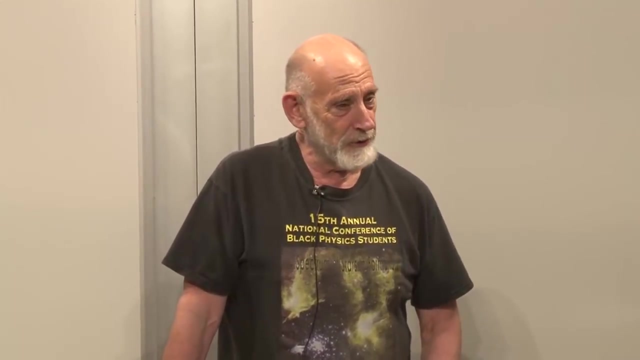 and forgetting, and learning and forgetting, and learning and forgetting statistical mechanics. So here's my opportunity to learn it again. Okay, Let's begin with what I usually call a mathematical interlude. In this case, it's not an interlude, it's a starting point. 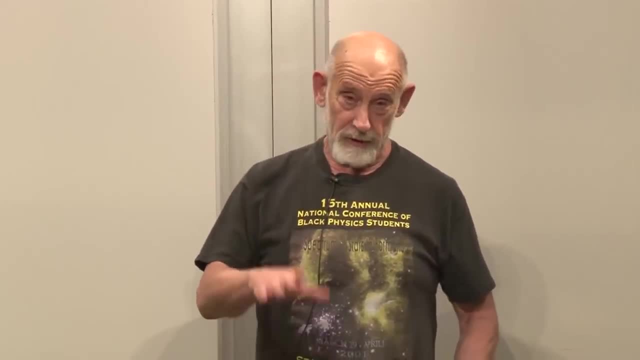 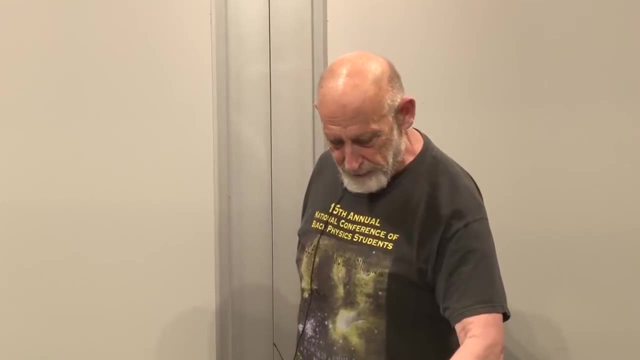 And I'm just going to make some extremely brief remarks, which you all know- at least I think you all know them- about probability, Just to have you know, just to level the ground, What are we talking about And what I am not going to explain. 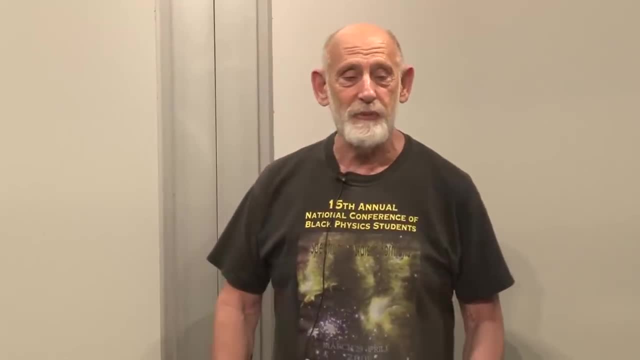 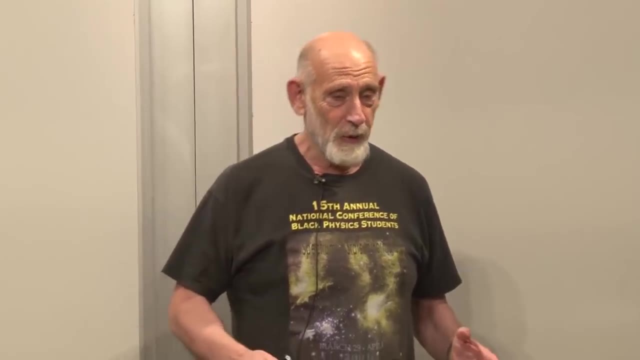 because I don't think anybody can explain it is why probability works. Why does it work? If you ask why it works, the first answer will be: it doesn't always work. You may have a probability for something and you test it out. 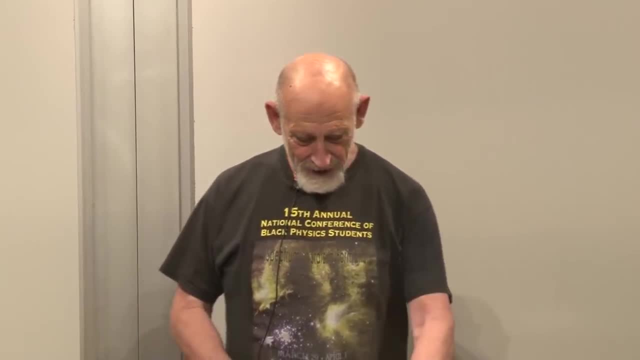 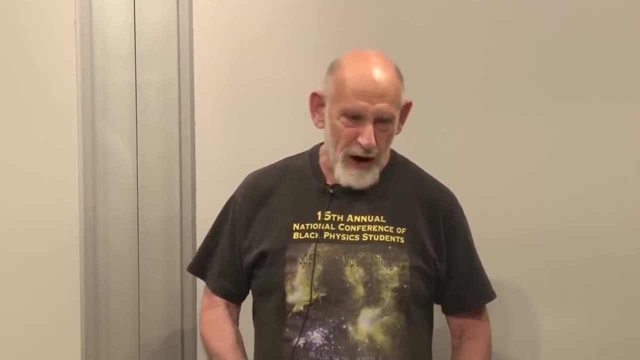 and sometimes it doesn't work. Those are called the exceptions. So the answer to the question is: why does it work? Well, it doesn't always work. It mostly works, except when it doesn't. When doesn't it Rarely? 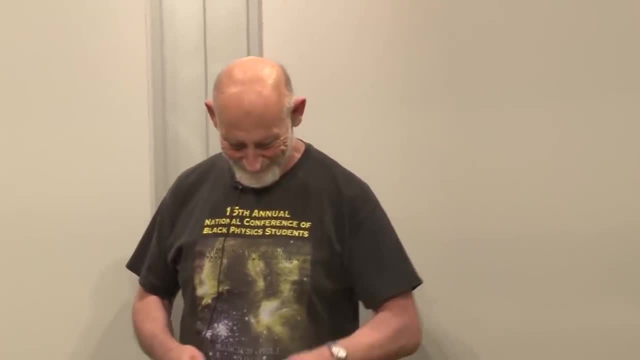 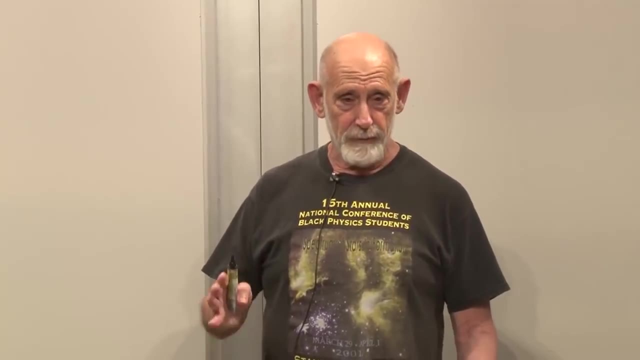 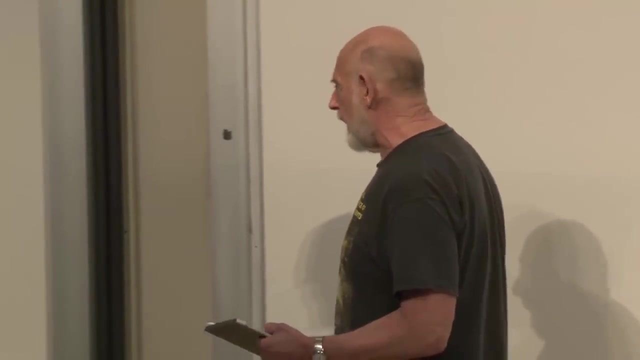 How rarely? Every so often. But there is a calculus of probability, a mathematical theory of probabilities, and we'll talk about it a little bit. Okay, so we'll take probability to be a primitive concept, basically a primitive concept, and we'll suppose that there is a space of some sort. 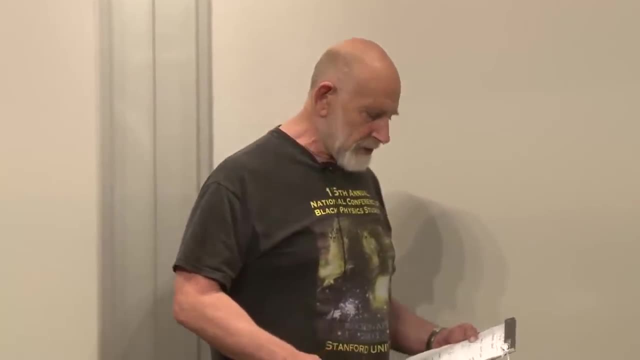 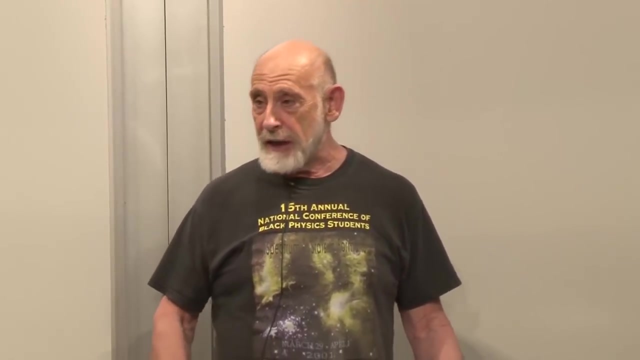 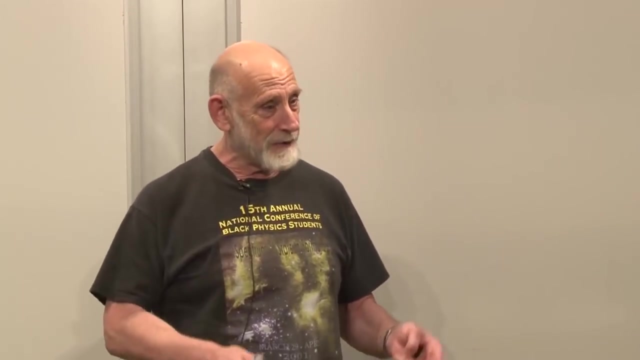 a space of possibilities. The space of possibilities could be the space of outcomes of experiments, or it could actually be the space of states of a system. The state of a system could be this, or it could be the outcome of an experiment, If the experiment consists of determining the state of the system. 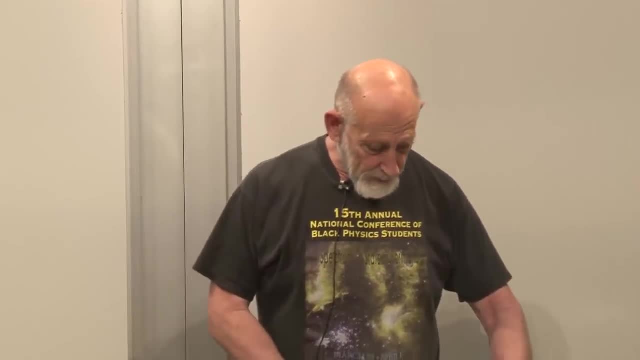 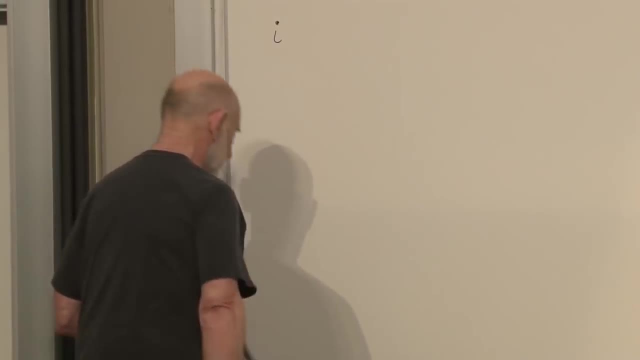 then the state of the system is the outcome. So we have a space and let's call that space, let's label the elements of that space with a little i. For example, if we were flipping coins, i would be either heads or tails. 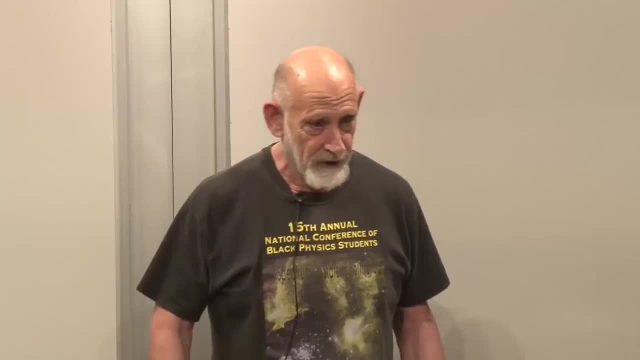 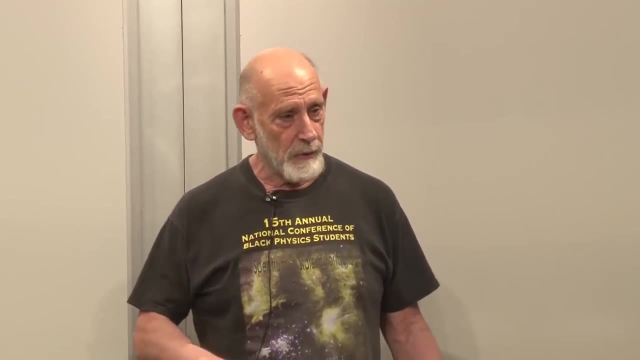 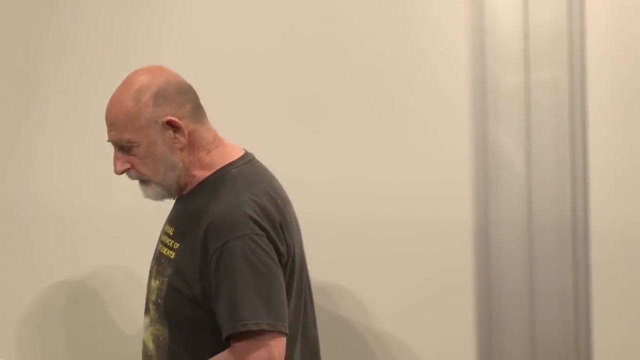 If we were flipping die, you know, like dice, dies of dice i would run from one to six. If there were two dies, then we would have enough indices to keep track of two dice and so forth. So i is the space of possibilities, of outcomes. 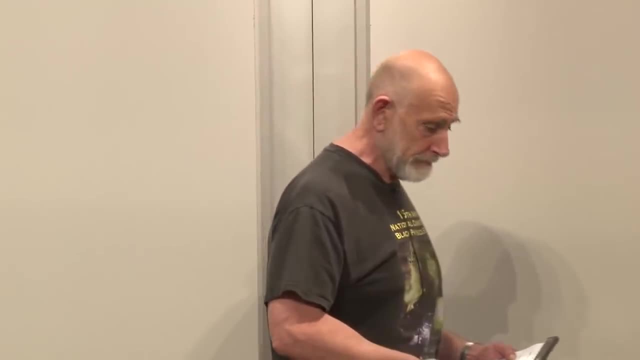 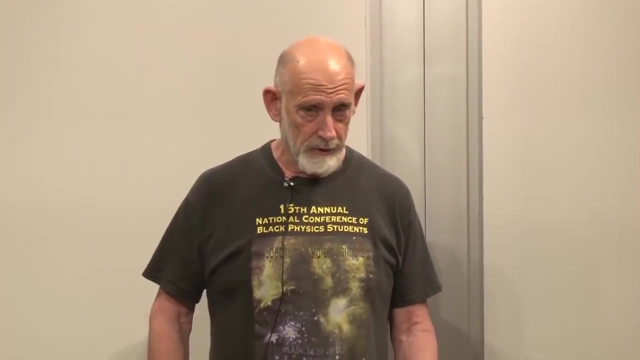 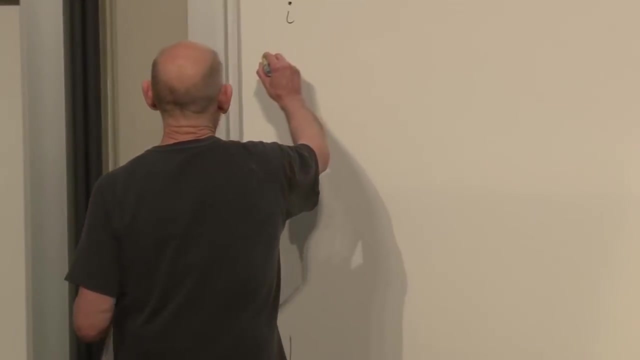 or the space of possible states of a system. And if we are ignorant, statistics always has to do with ignorance. You don't know everything, and so you assign probabilities to outcomes, and so we assign a probability p of i to the ith outcome. 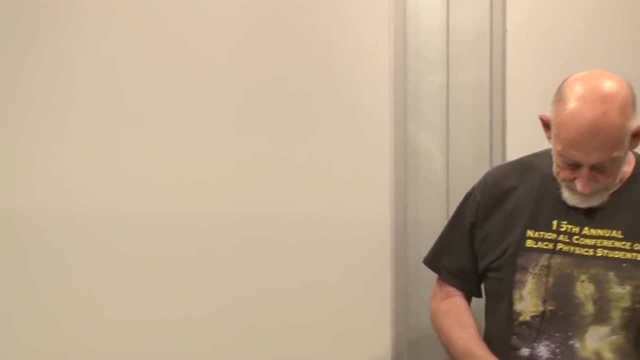 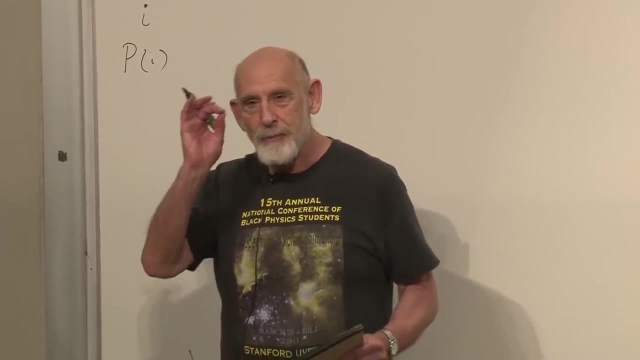 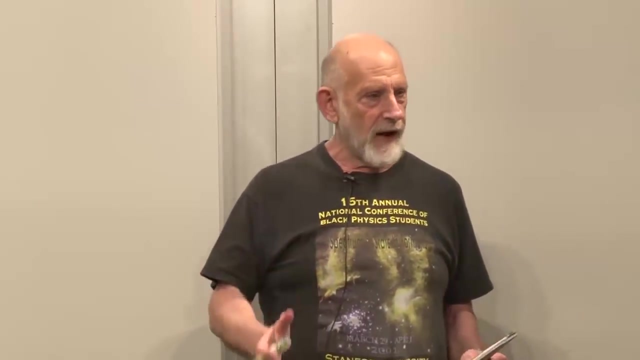 to the answer to our question: What are the rules for p of i? What does p of i have to satisfy? And let's, for the beginning, at least in the beginning, let's imagine that i enumerates some discrete, finite collection of possibilities. 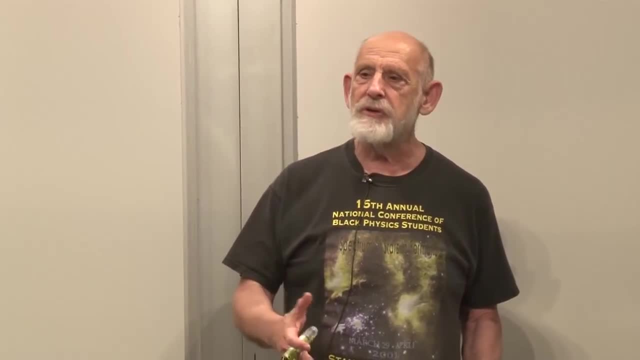 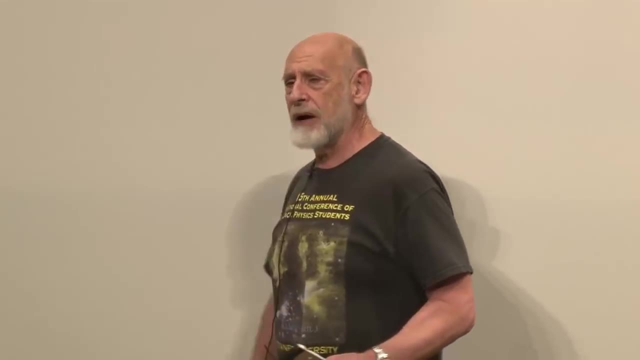 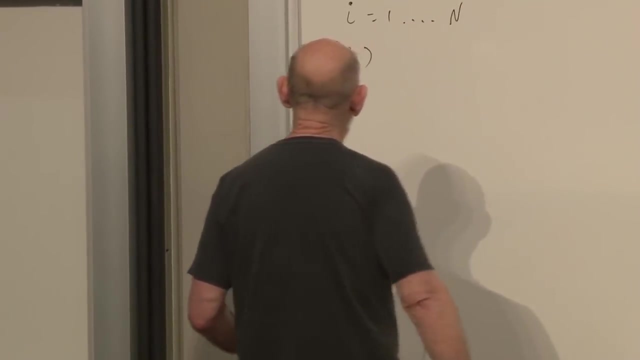 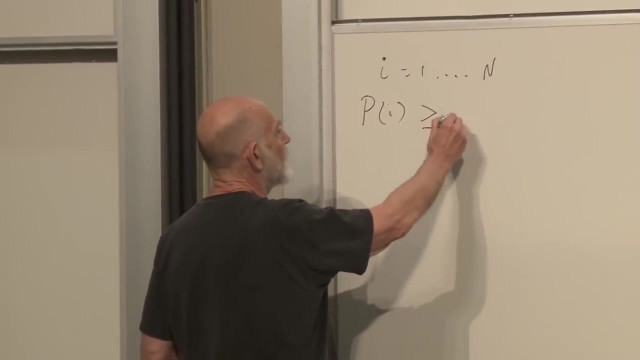 Later on we can have an infinite number of possibilities, or even a continuously infinite number of possibilities, But for the time being i might run from one to n n possibilities, and the rules are, first of all, p of i has to be greater than or equal to zero. 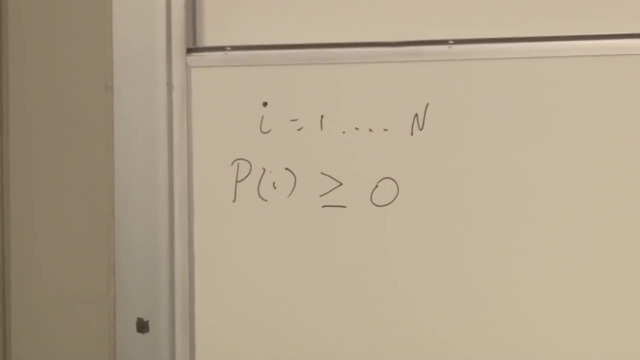 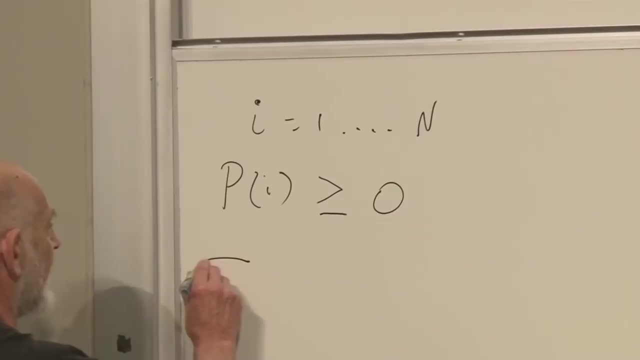 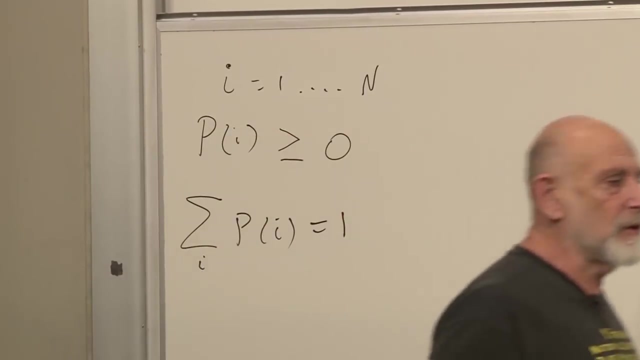 Negative probabilities. we don't like them, We don't know what they mean. Okay, Next, the summation over i of p, sub i, p of i should be one. That means that the total probability when you add everything up, 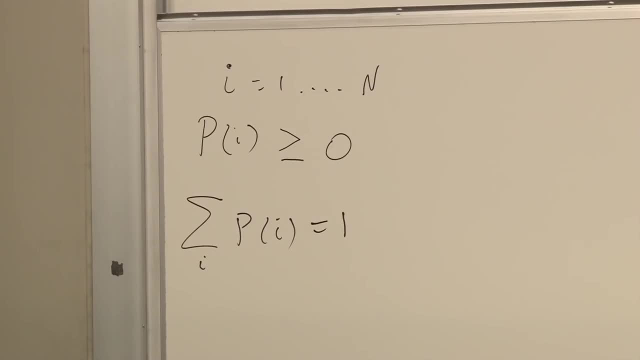 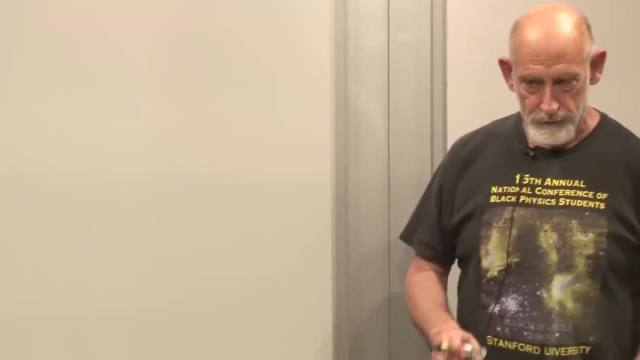 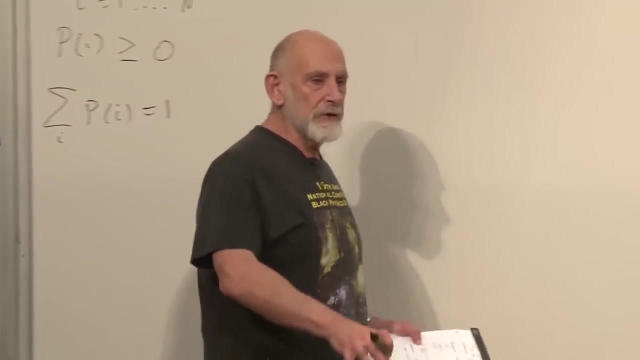 all possibilities should be one. You certainly should get some result. Okay, Next now this is a kind of hypothesis. This is the law of large numbers, that if you either make many replicas of the same system or do the same experiment over and over, 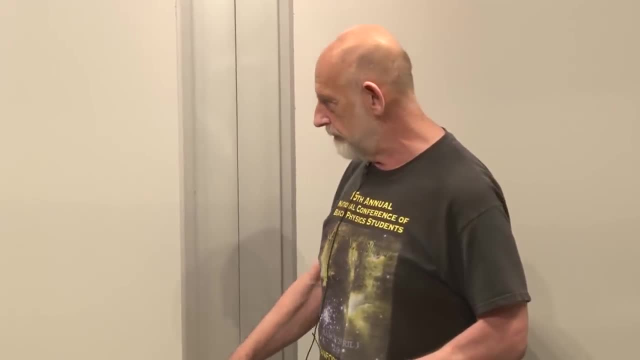 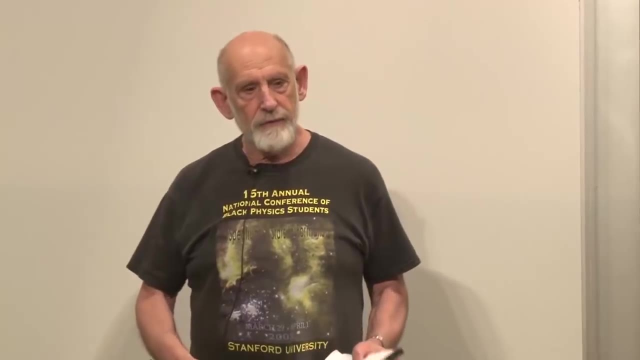 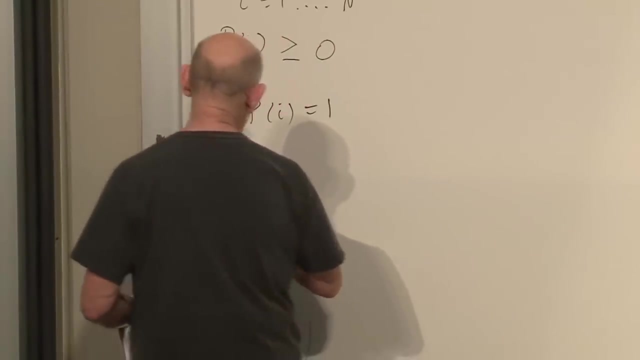 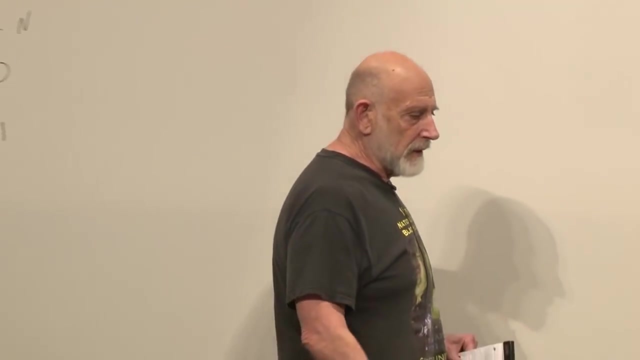 a very, very large number of times and take all of the outcomes which gave you, all of the experiments which gave you the i-th outcome. that's some number, let's call it n of i. that's the number of times that the experiment turned up. 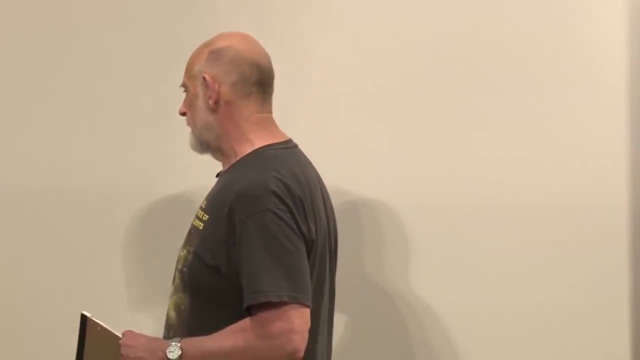 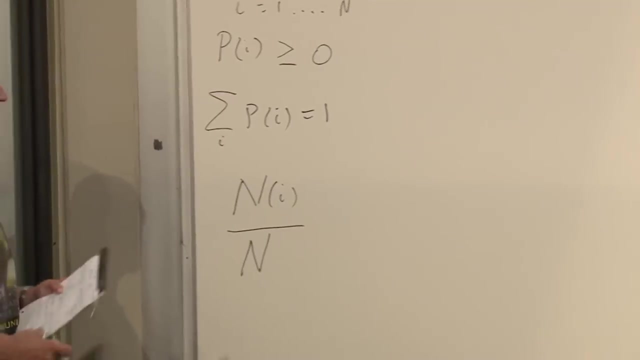 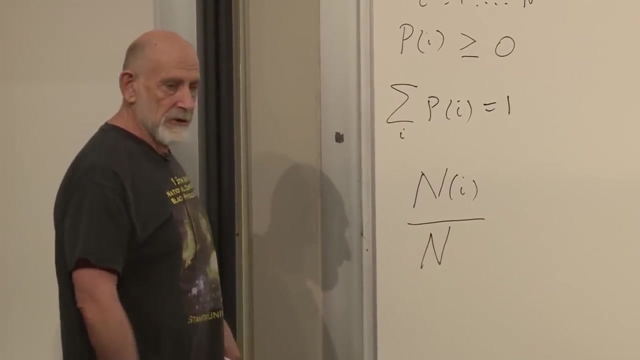 the i-th possibility and you divide it by the total number of trials. total number of trials means the sum over all i or just the total number of trials. that the limit of this. this is a physical hypothesis. it's a physical hypothesis. 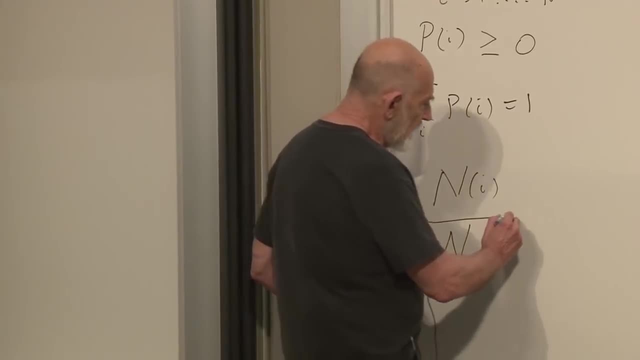 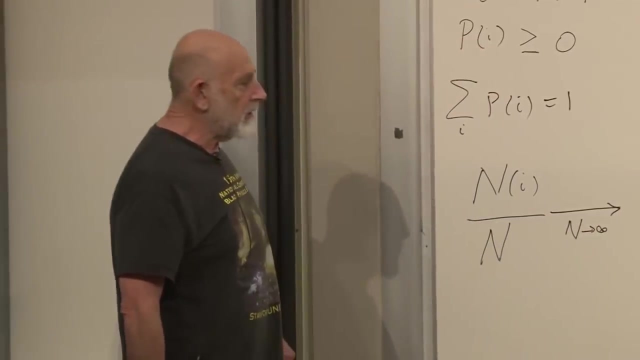 it can go wrong if n is not large enough. but in the limit of large n n goes to infinity. in the limit of very, very, of course n never goes to infinity. you never get to do an infinite number of experiments. 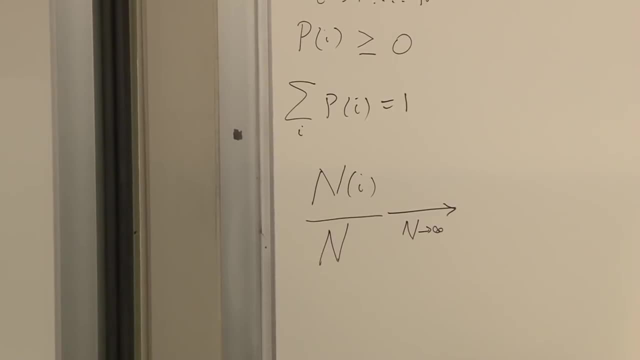 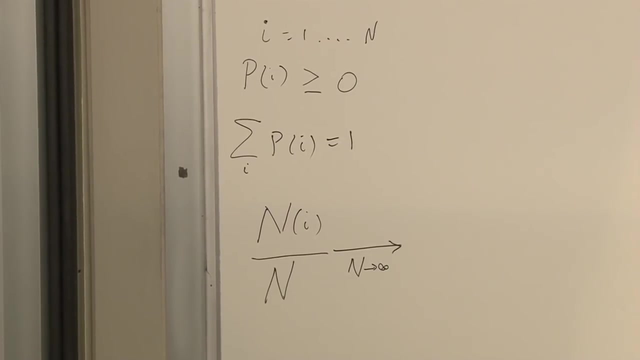 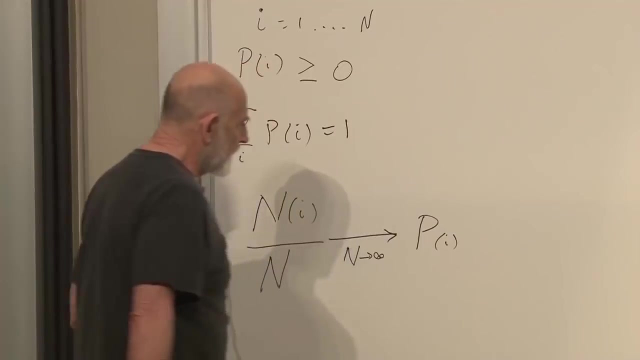 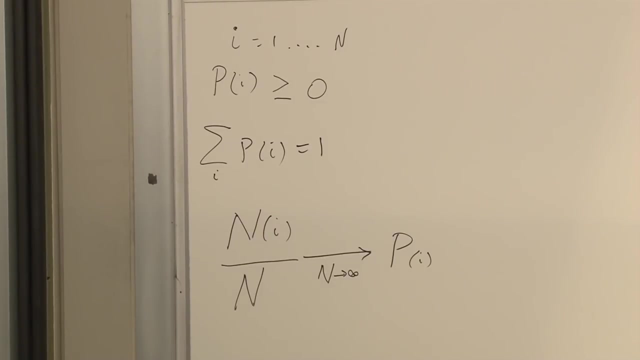 but nevertheless we're kind of idealizing, we're assuming we can do so many experiments that the limit- n goes to infinity- is effectively been reached, then that is p of i. So p of i controls by assumption the ratio of the n of i's. 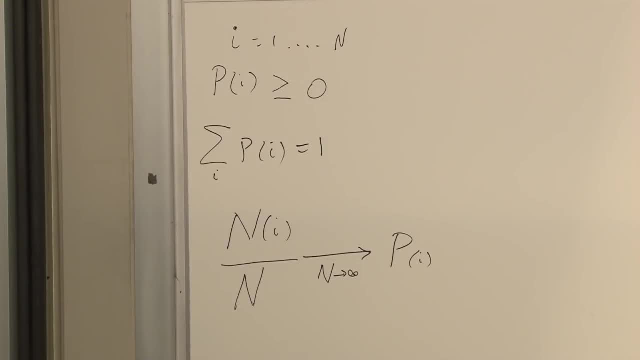 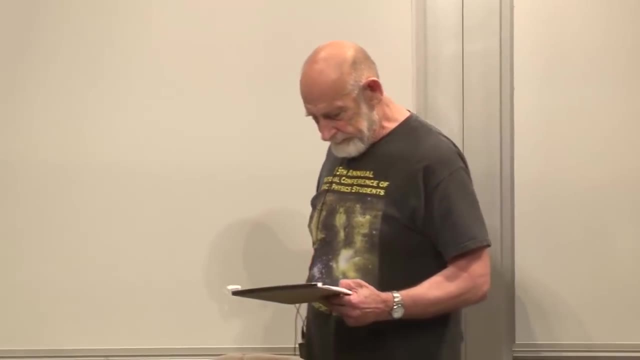 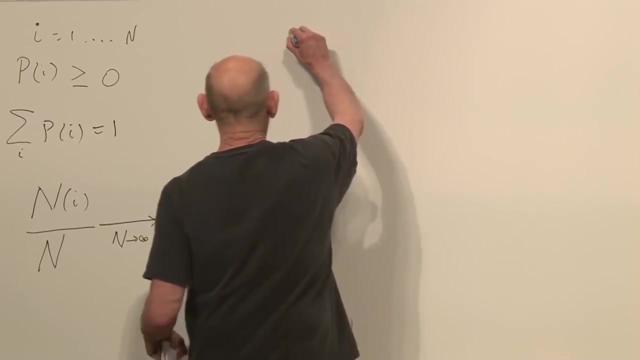 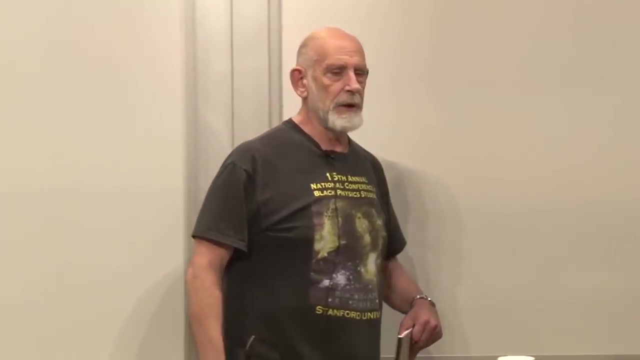 Okay, everybody happy with that. You use this all the time. I think. Well, sometimes we use it. Now let's suppose that there is a quantity, let's call it f of i. it's some quantity that's associated with the i-th state. 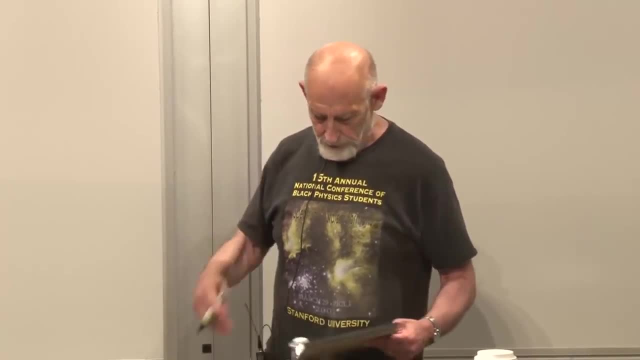 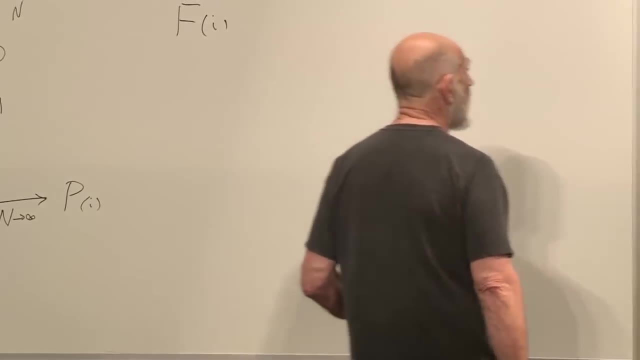 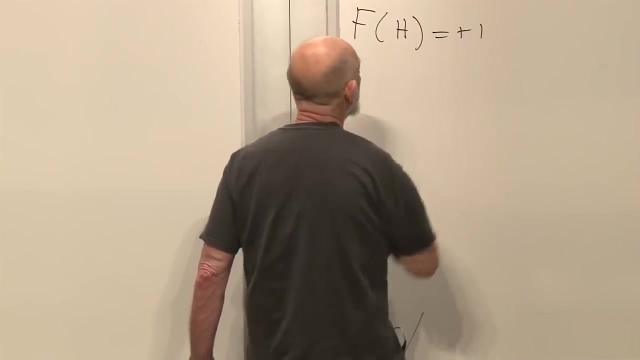 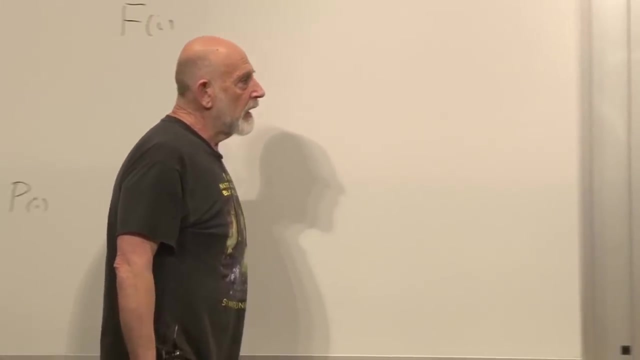 We can assign it, we can make it up. For example, if our system is heads and tails and nothing but heads and tails, we could assign f of heads and call it plus one, and f of tails and call it minus one If our system has many, many more states. 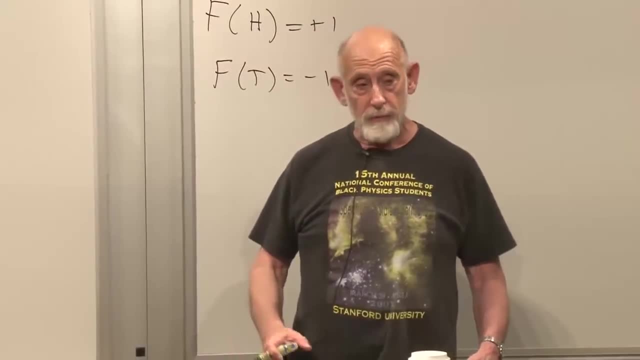 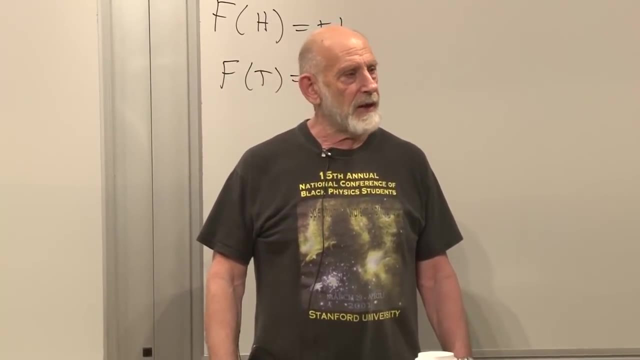 we may want to assign a much larger number of possible f's, but f is some function of the state. It's also a thing that we imagine measuring. It could be the energy of a state or it could be the momentum of a state. 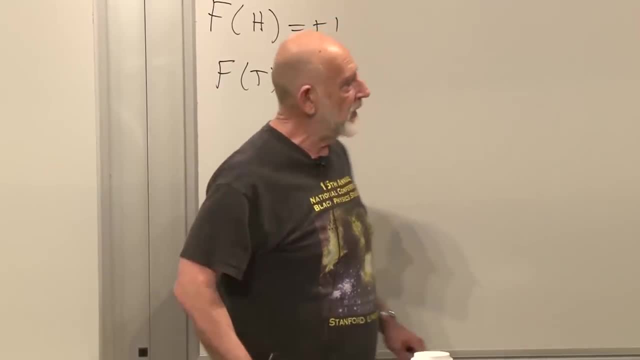 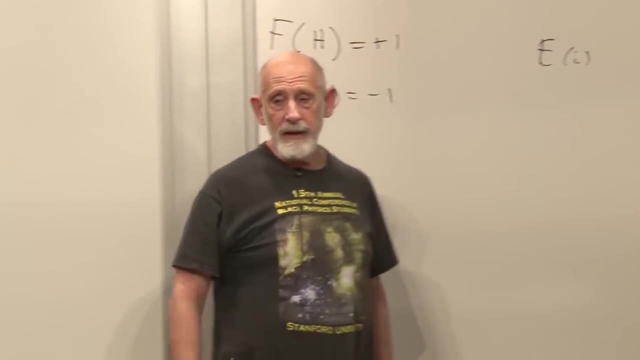 Given a state of some system, it has an energy. It would be called a natural state in that case, perhaps e of i, Or it could be the momentum, Or it could be something else. It could be whatever you happen to like. 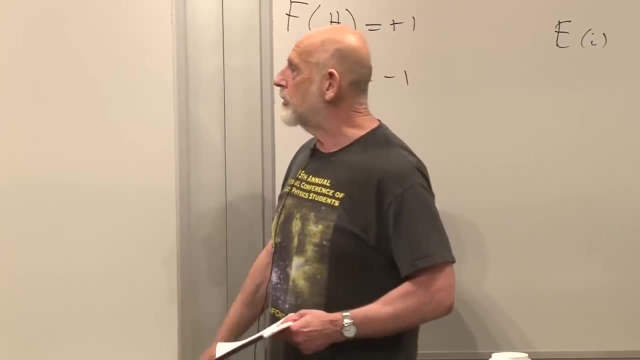 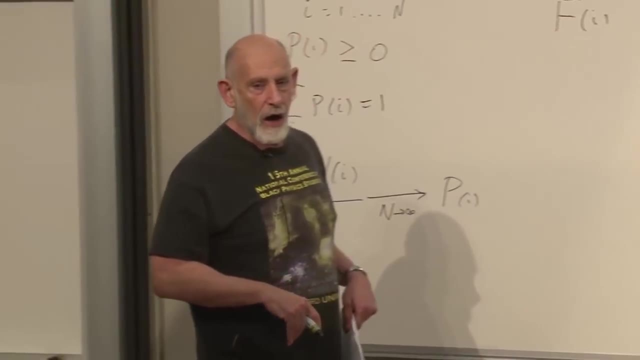 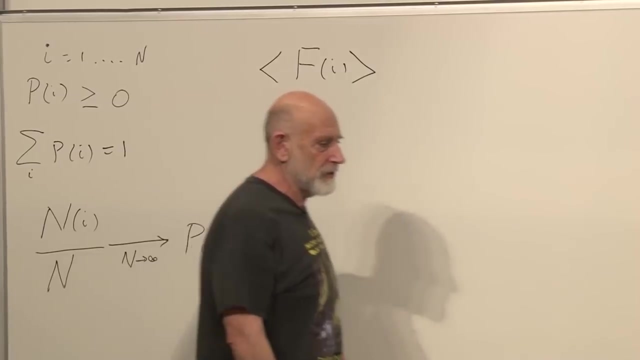 to think about. Then, an important quantity is the average of f of i And the average of f of i. I will use the quantum mechanical notation for it, even though we're not doing quantum mechanics. It's a nice notation. Physicists tend to use it all over the place. 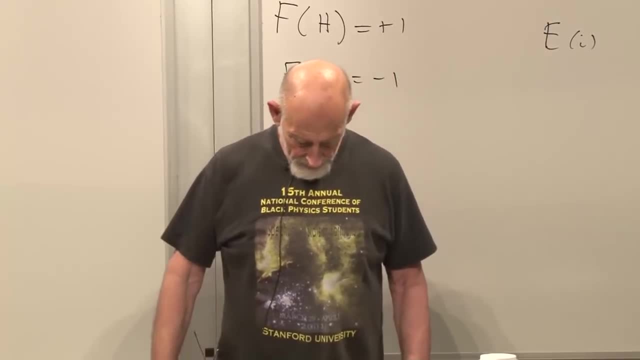 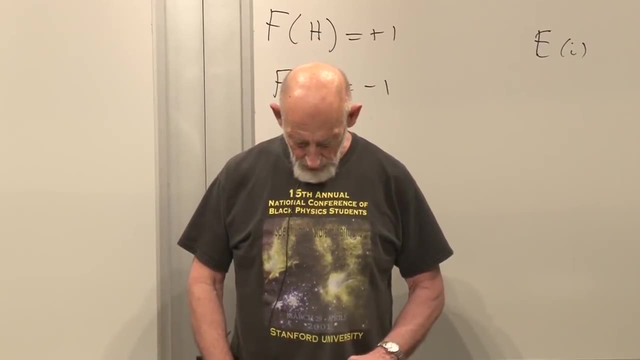 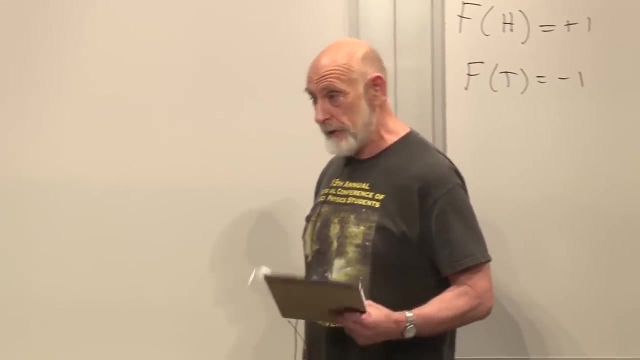 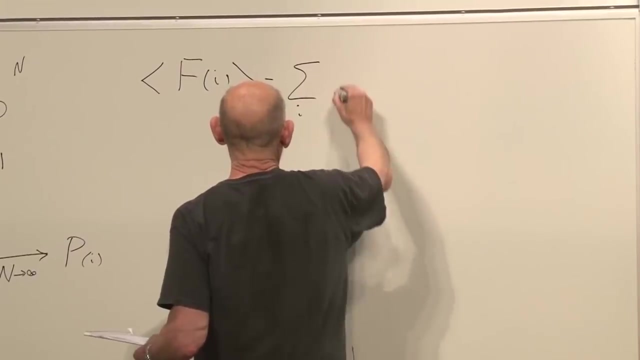 Mathematicians hate it. Just put a pair of brackets around it. It means the average, The average value of the quantity averaged over the probability distribution. It has a definition. Its definition is that it's the sum over i, of f, of i weighted. 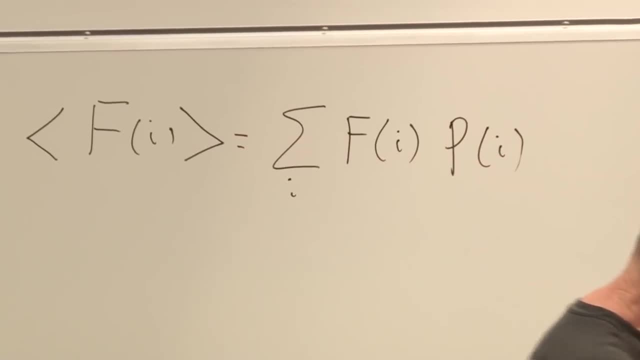 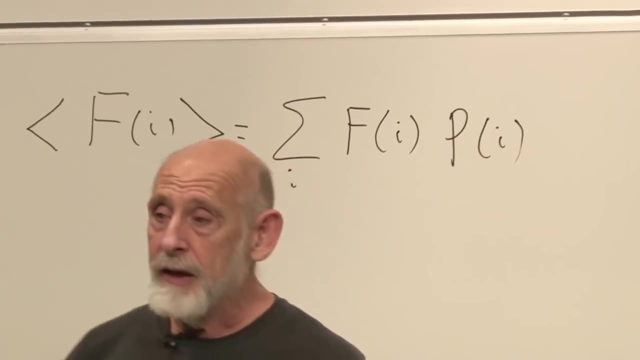 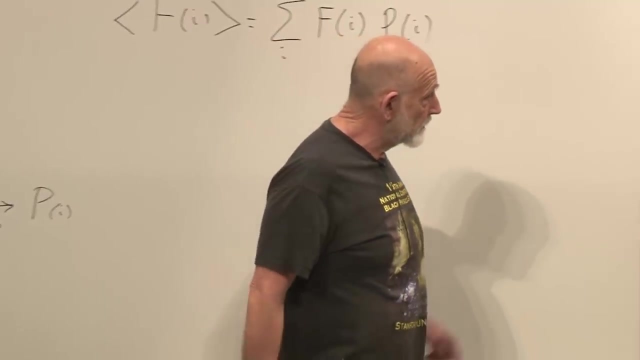 with the probability, For example, if- and incidentally- the average of f of i does not have to be any of the possible values that f can take on, For example, in this case where f of heads is plus one and f of tails is minus one. 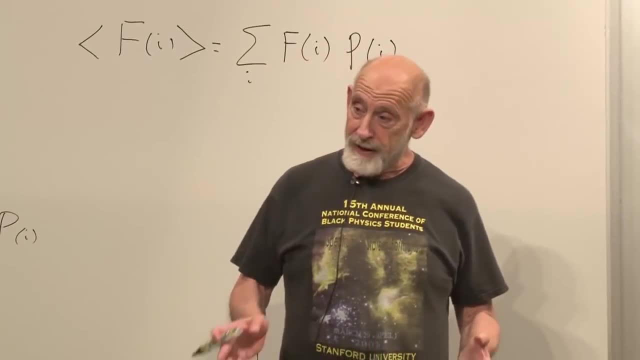 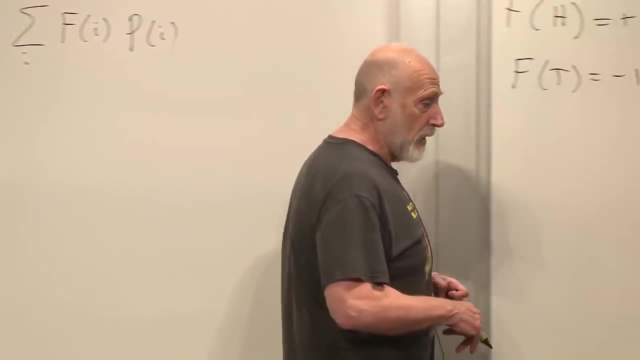 and you flip a million times and the probability is a half of heads and a half of tails. the average of f, of i, the average of f will be zero. Zero is not a possible outcome to the experiment. There's no rule. why the 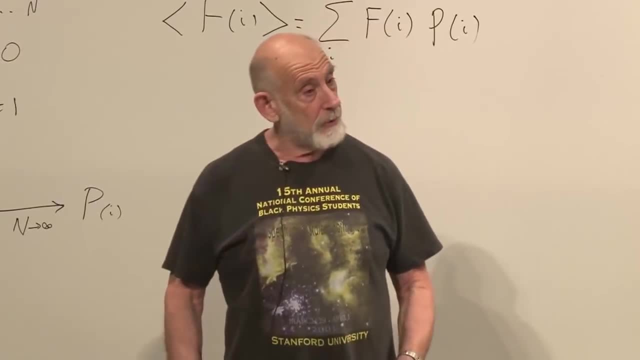 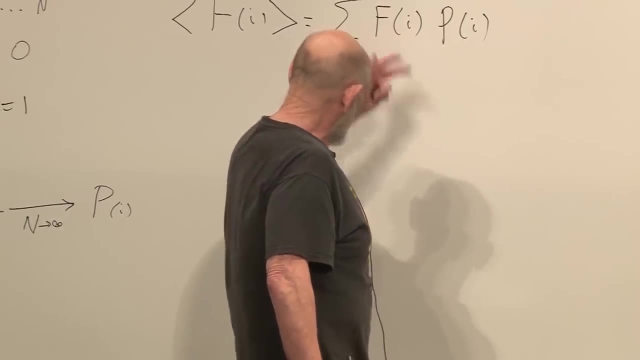 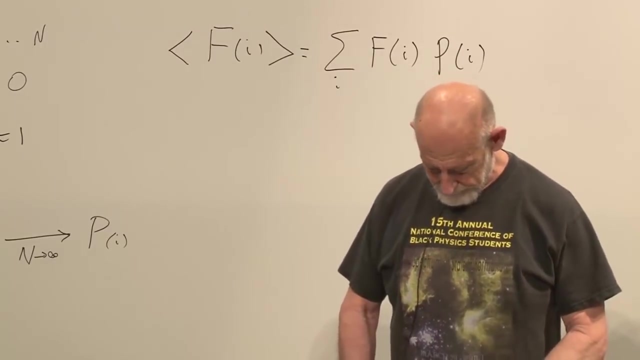 why the average should be one of the possible experimental outputs. But it is the average And this is its definition. It's: each value of f is weighted with the probability for that value of f. You can write it another way. You can write it as a sum over i. 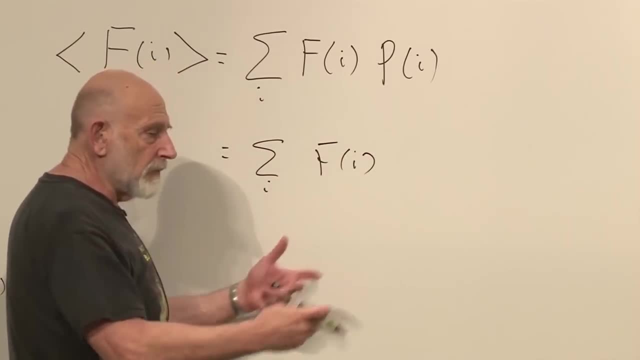 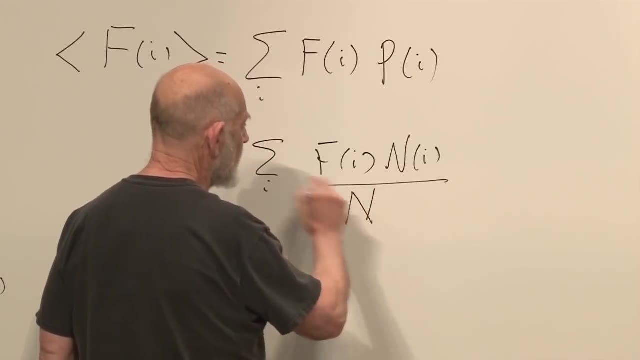 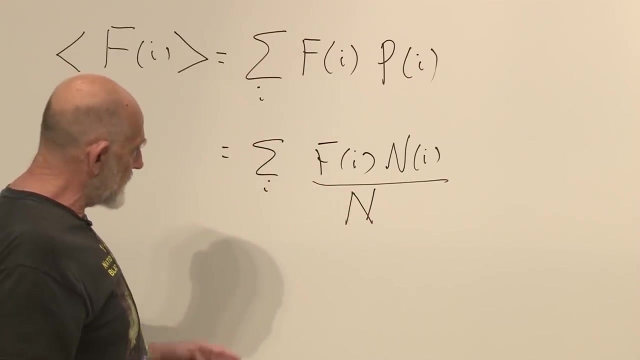 of f of i times the number of times that you measure i divided by the total number of measurements. that's what p of i is in the limit that there are a large number of measurements. So that's defined to be the average. That's our mathematical. 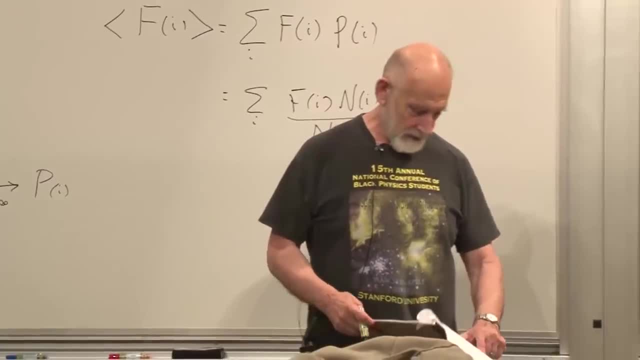 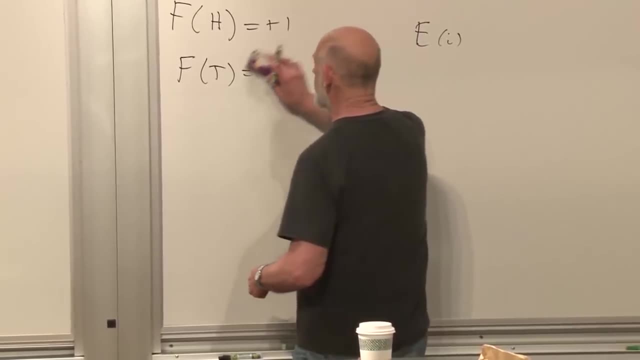 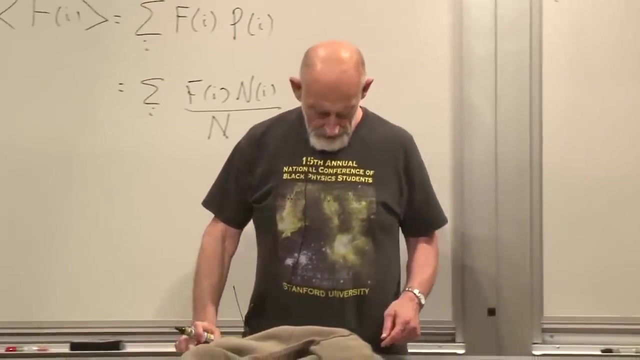 preliminary for today. That's all we, that's all I wanted to to level the playing field by making sure everybody knows what a probability is and what an average is, Because we'll use it over and over. Okay, let's start with. 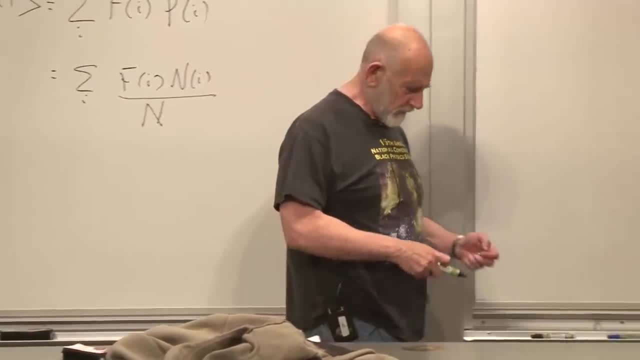 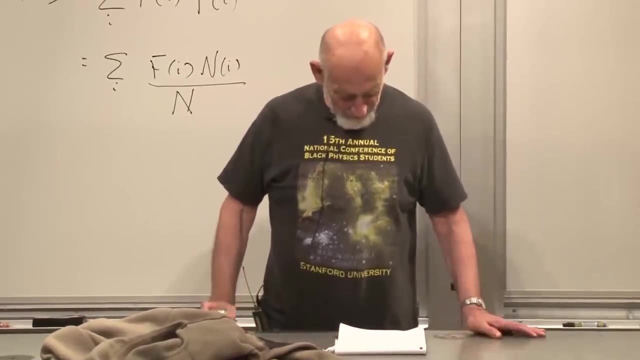 let's start with coin flips. I always start with coin. I start every single class with coin flips, Even when I'm teaching about the Higgs boson. Okay, If I flip a coin a lot of times, or whether I flip a coin. 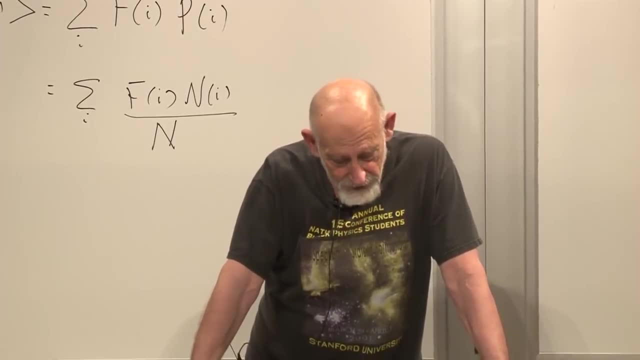 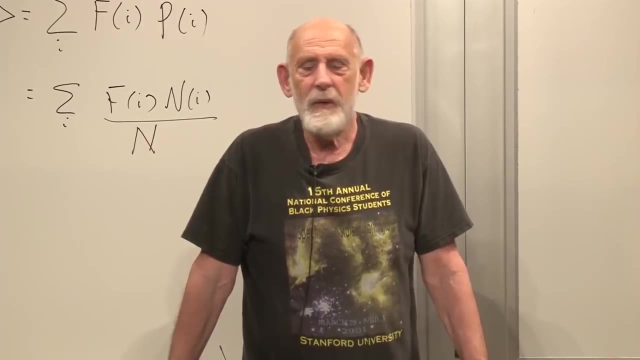 a lot of times or not. the probability for heads is usually deemed to be one half, and the probability for tails is usually also deemed to be one half. Why do we do that? Why is it a half and a half? What's the logic there? 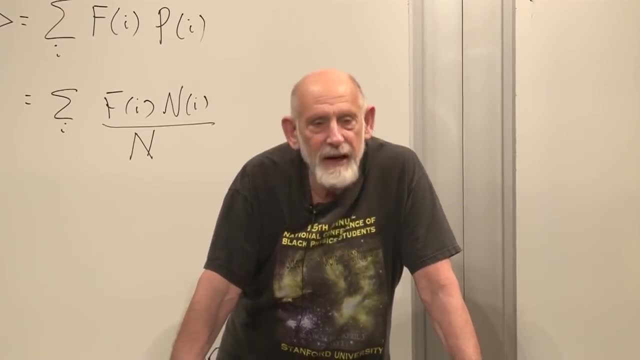 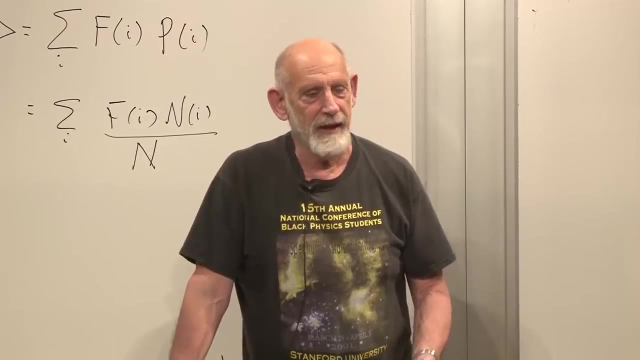 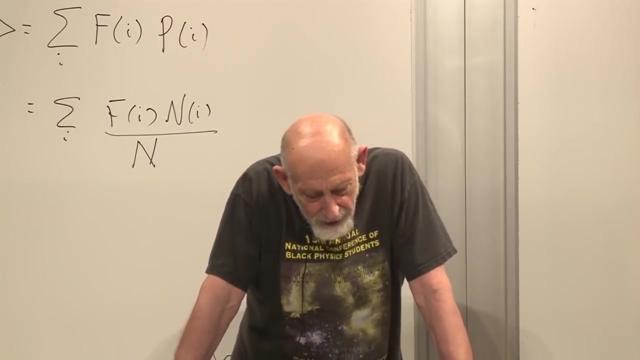 What logic tells us that? And in this case it's symmetry, The symmetry of the coin. Of course, no coin is perfectly symmetric and even making a little mark on it to distinguish a heads and tails biases it a little bit. But apart from that, tiny, tiny bias, 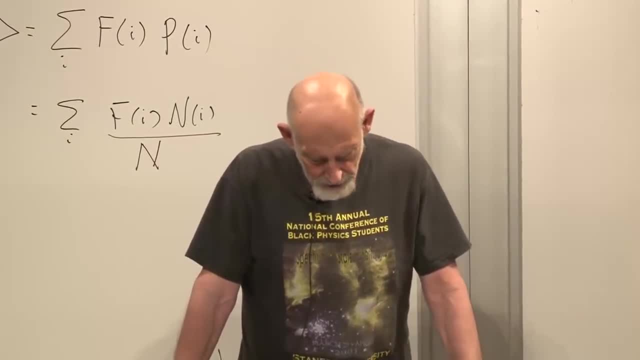 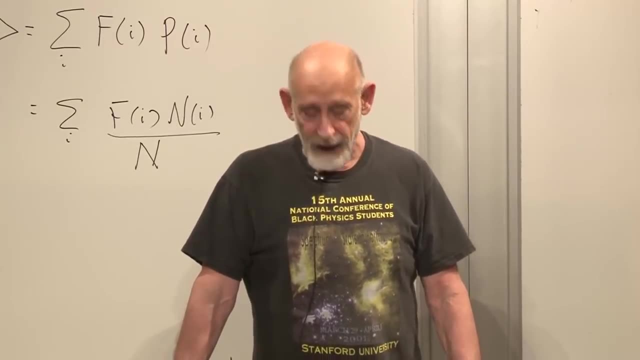 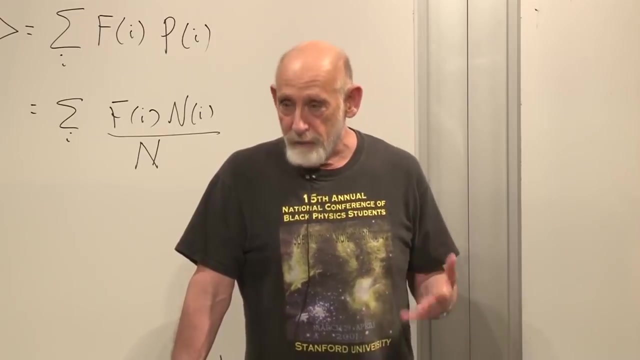 of marking the coin with maybe just a tiny little scratch. the coin is symmetric, Heads and tails are symmetric with respect to each other and therefore there is no, no reason, no rationale for, when you flip a coin, for it to turn up heads. 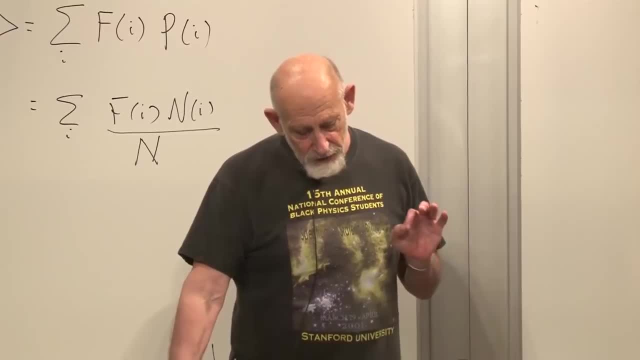 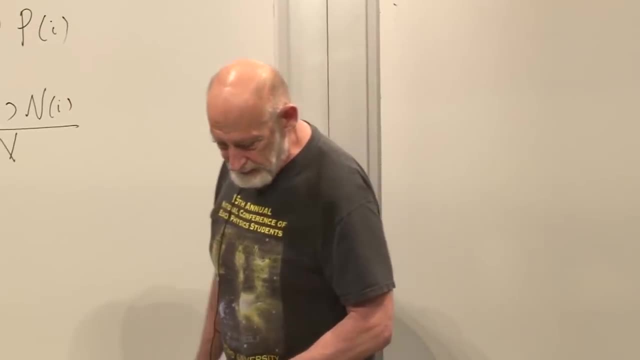 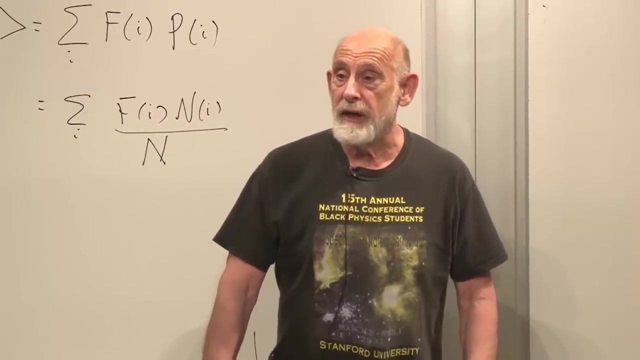 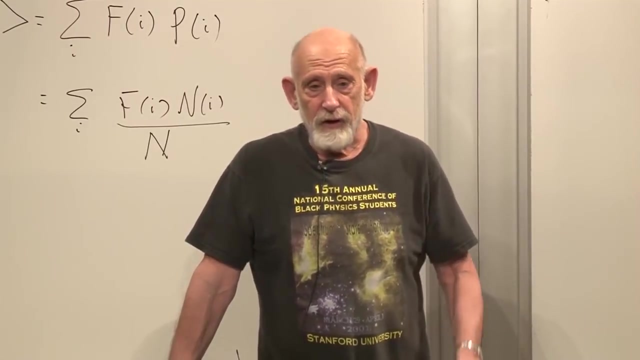 more often than tails, And so it's symmetry quite often- I might even say always- in some deeper sense, but at least in many cases, symmetry is the thing which dictates probabilities. Probabilities are usually taken to be equal for configurations which are related to each other. 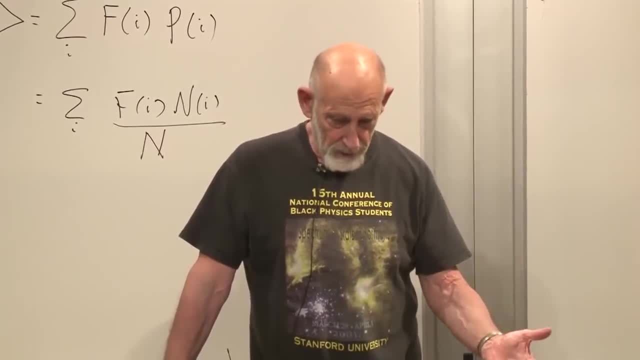 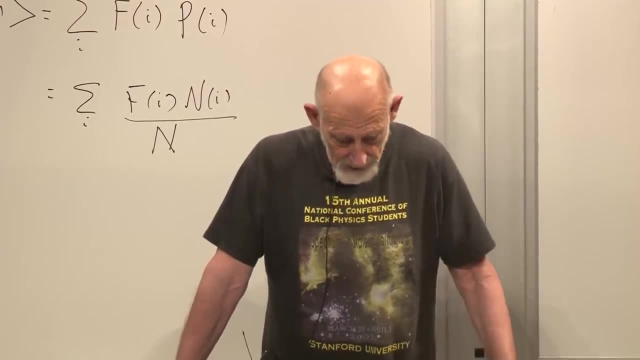 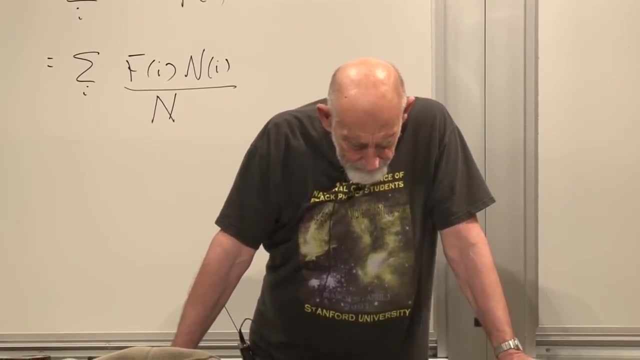 by some symmetry. Symmetry means: if you, you know you act with the symmetry, you reflect everything, you turn everything over that the system behaves the same way. Okay, another example besides coin flipping would be dice flipping. Dice flipping, instead of having 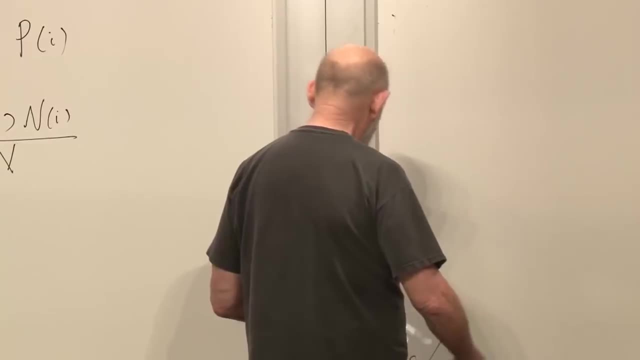 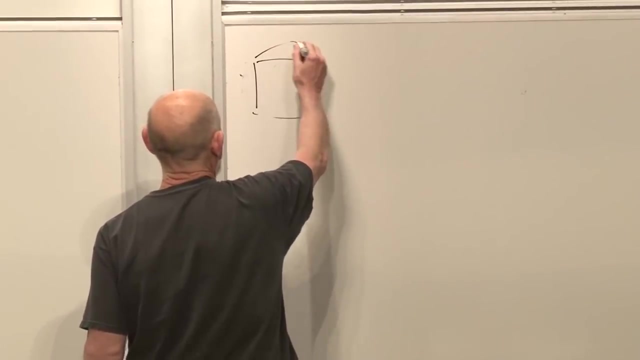 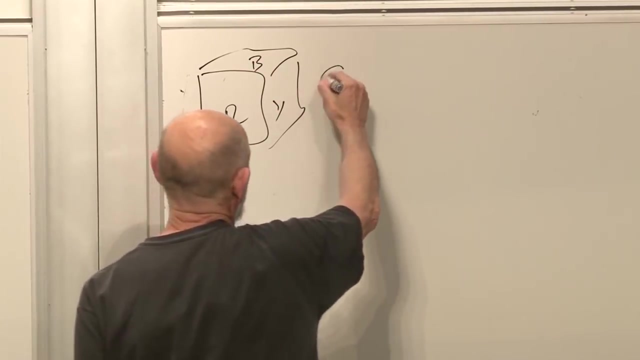 two states has six states, one die and we can imagine coloring them. Let's do that. We color the faces red, yellow, blue, and then on the back green, purple and orange. Okay, that's our. 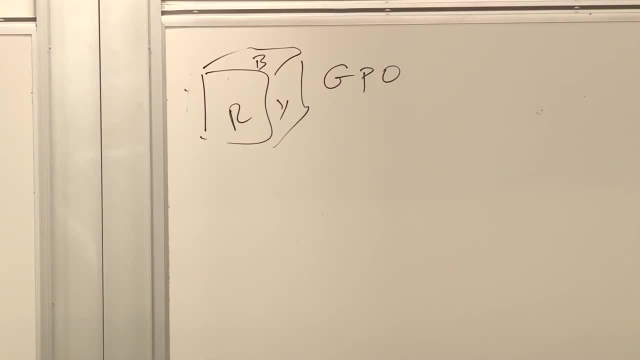 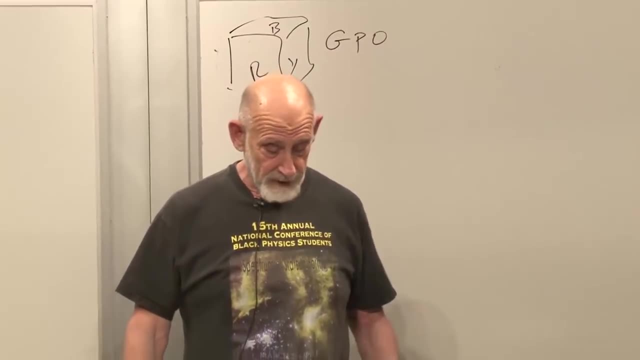 die and it's been colored. We don't have to keep track of numbers, we can keep track of colors. And what is the probability that when we flip the die? flip it into the air, hits the ground. what's the probability that it turns up? 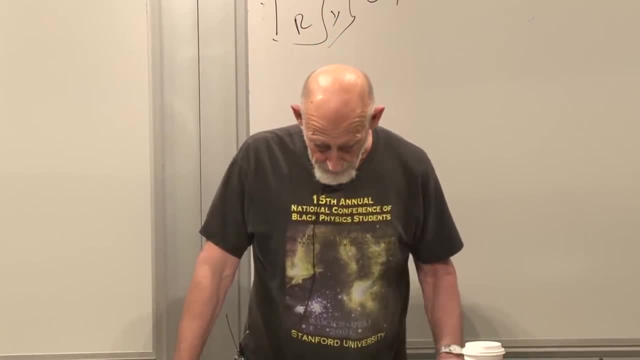 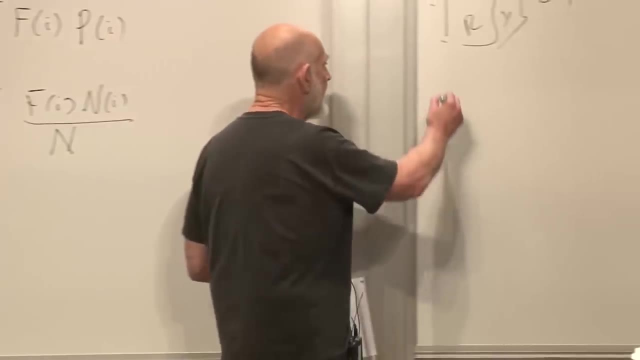 red: One-sixth. right, There are six possibilities. they're all symmetric with respect to each other. We use the principle of symmetry to tell us that the p of each i, they're all equal and they're all equal to one-sixth. 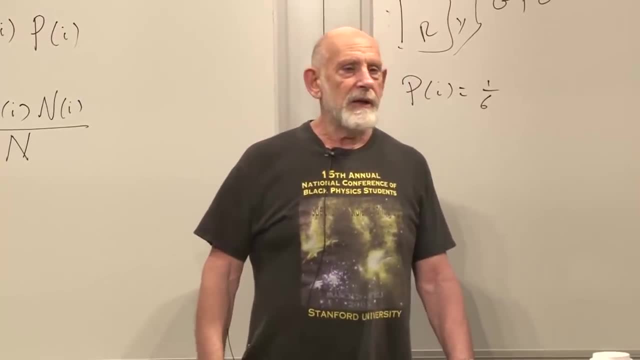 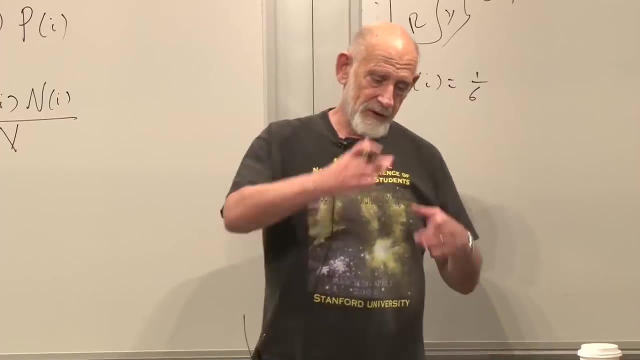 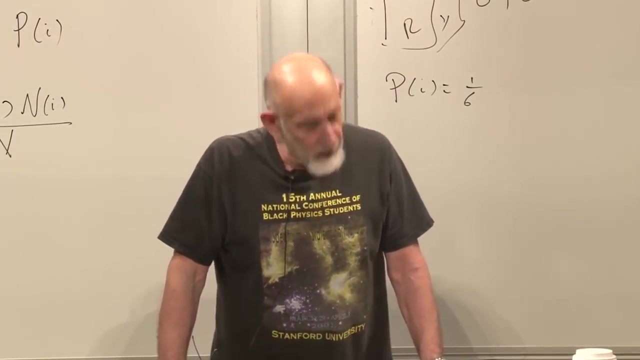 But what if there is no symmetry? What if really the die is not symmetric? For example, what if it's weighted in some unfair way? Or what if it's been cut with faces that are not nice and parallel cubes? Then what's the? 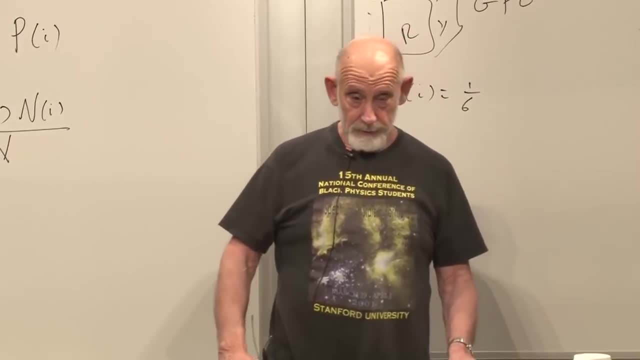 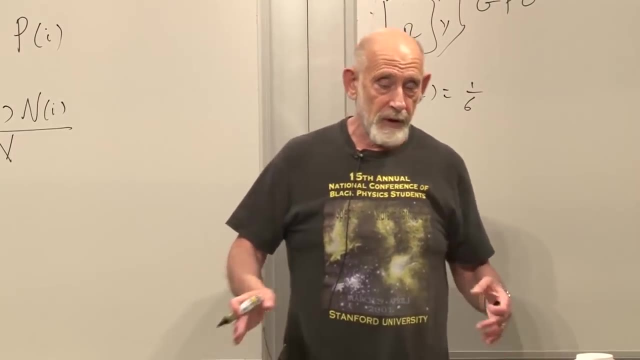 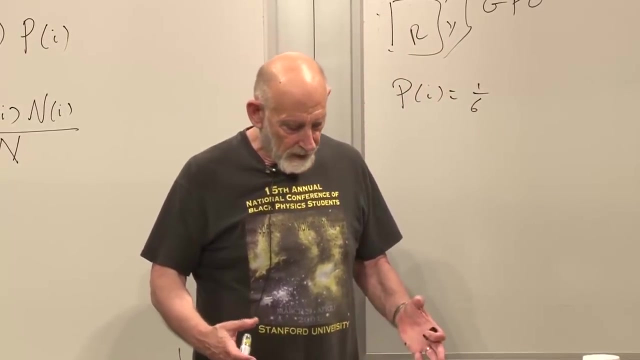 answer, And the answer is symmetry, won't tell you. You may be able to use some deeper underlying theory and to use some concept of symmetry from the deeper underlying theory, but in the absence of some something else, there is no answer. The answer is: experiment, Do this. 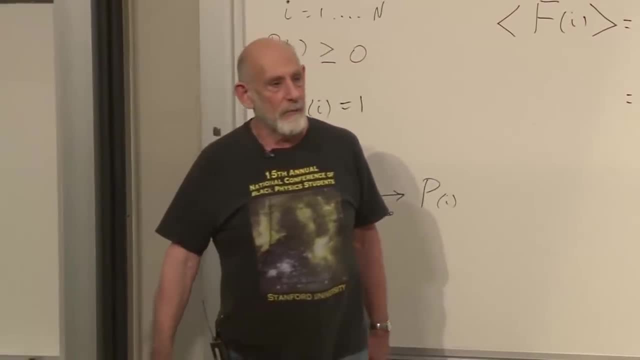 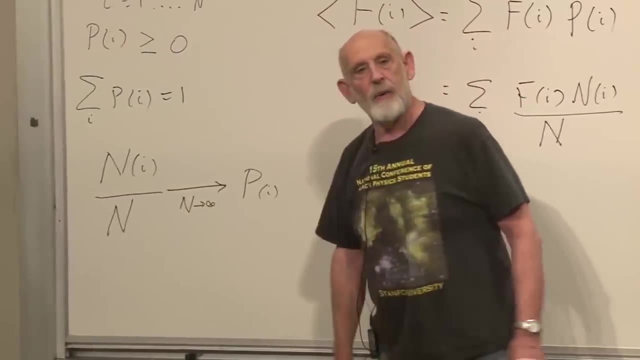 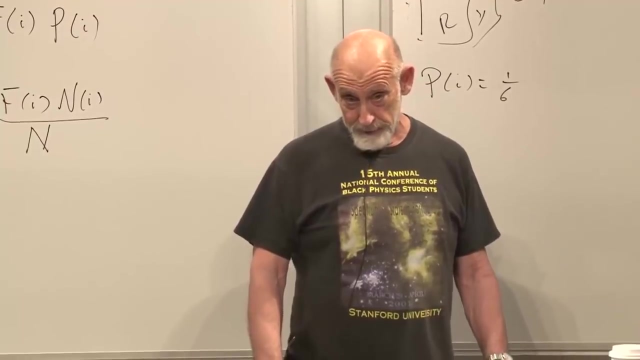 experiment a billion times, keep track of the numbers or assume that things have converged, and that way you measure the probabilities. You measure the probabilities and thereafter you can use them. You can use them if you keep a table of them and then you can use them in the 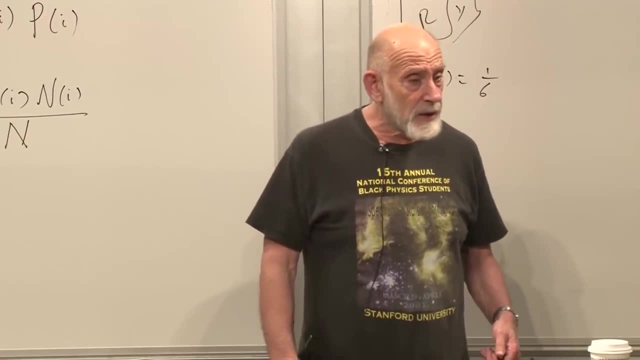 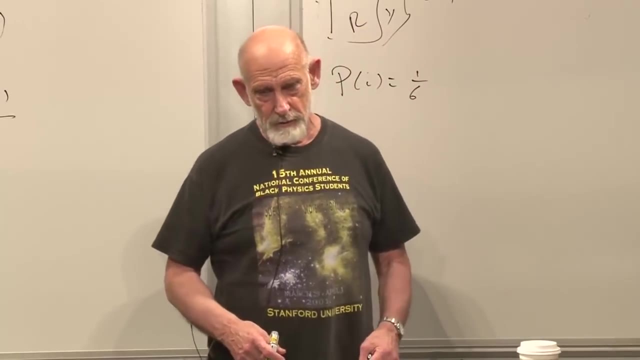 next round of experiments. Or you may have some theory, some deep underlying theory which tells you where, like quantum mechanics or statistical mechanics, Statistical mechanics tends to rely mostly on symmetry, As we'll see. So if there's no symmetry to guide you, 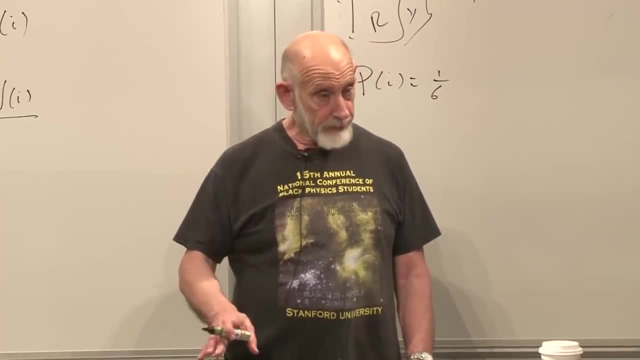 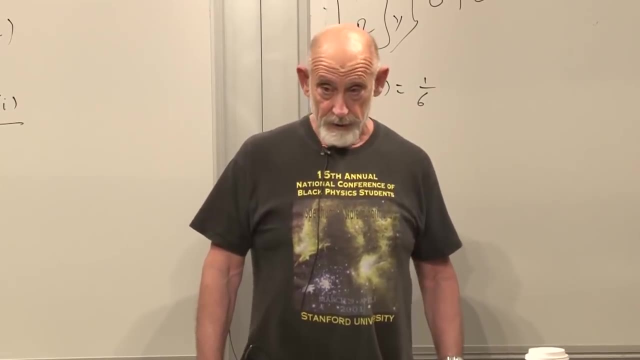 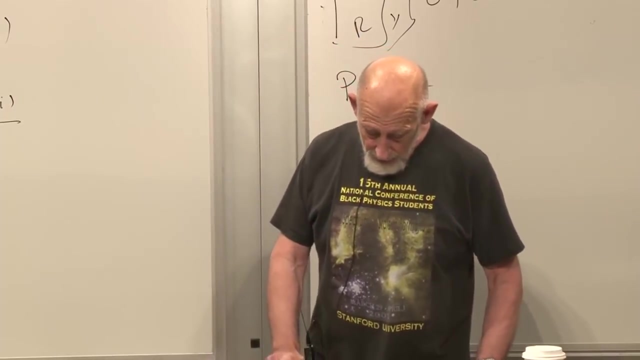 or to guide your implementation of probabilities, then it's experiment. Now there's another answer, There's another possible answer. This answer is often frequently invoked and it's a correct answer. under other circumstances It can have to do with the evolution of a 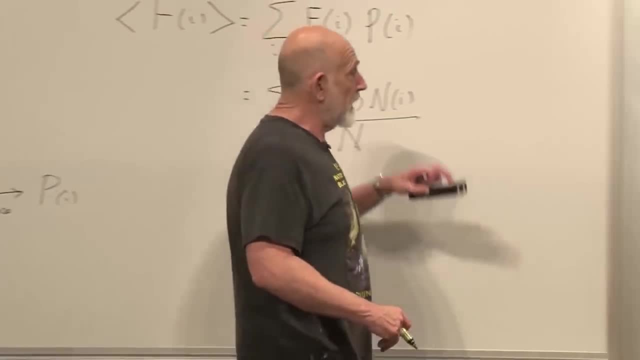 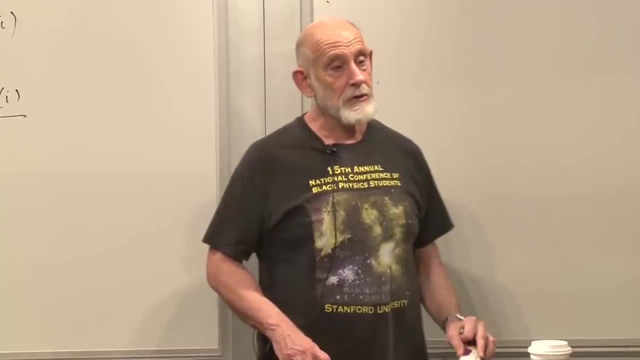 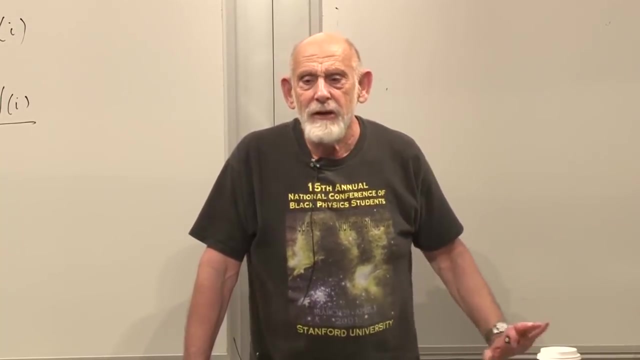 system, the way a system changes with time. So let me give you some examples Of what it might have to do. Let's take our six-sided cube and assume that our six-sided cube is not symmetric. It's not symmetric, but we know a rule. 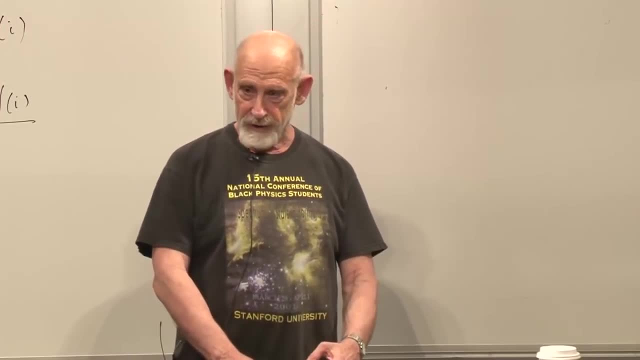 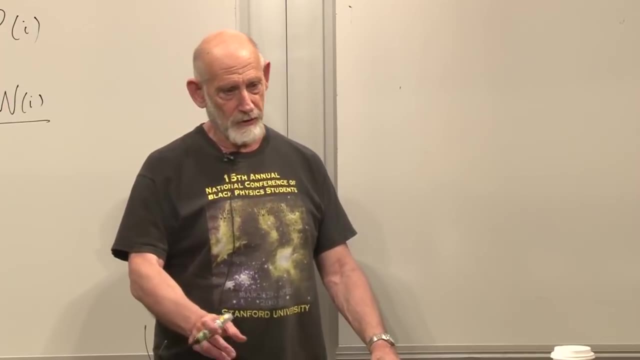 We know that if we put that cube down on the table, it's not a cube. When we put that die down on the table and we stand back, this thing has this habit of jumping to another state and jumping to another state and jumping to another state, It's called. 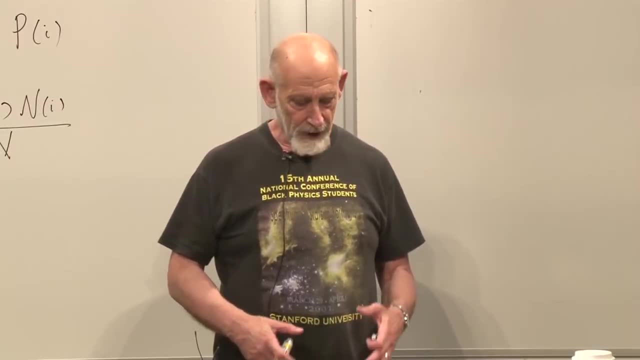 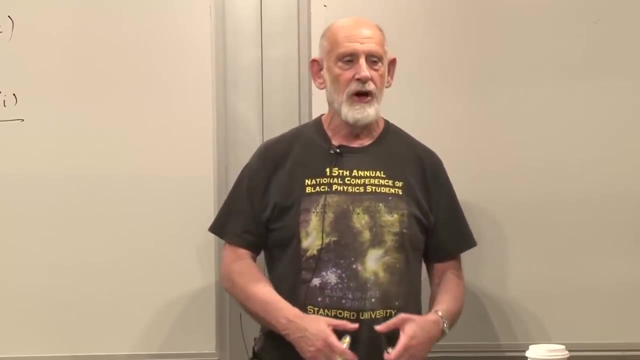 the law of motion of the system. The law of motion of the system is that whatever it is at one instant, at some next instant it will be something else according to a definite rule. The instance could be seconds, it could be microseconds or whatever. 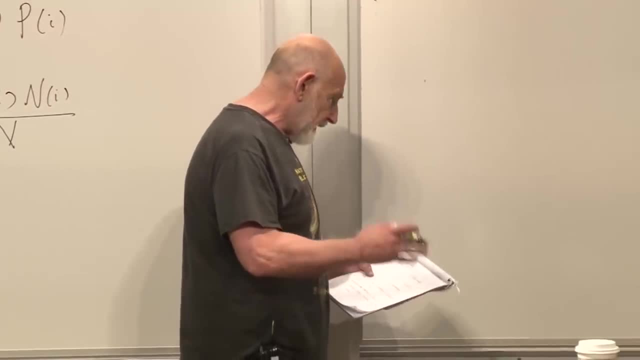 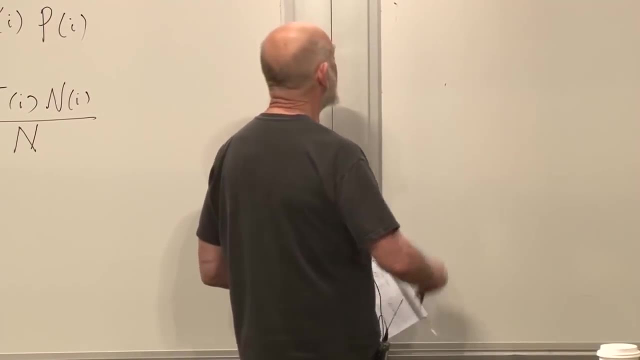 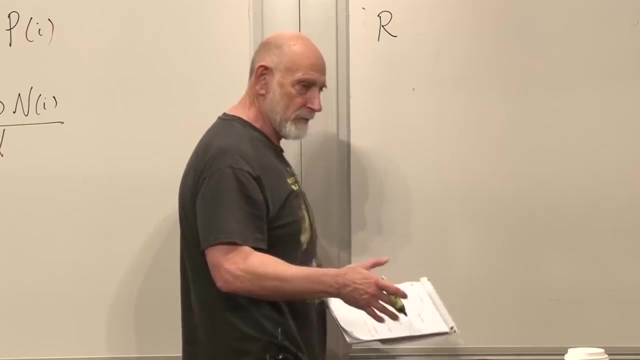 but imagine a discrete sequence, and let's suppose there's a law, a genuine law, that tells us how this cube moves around, For example, if it's red. now, we've done this over and over many times in different contexts, but it is so important. 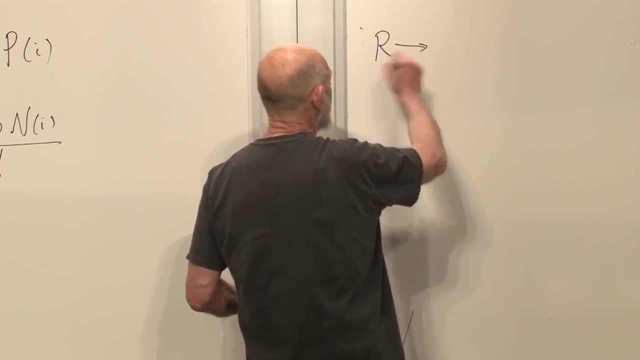 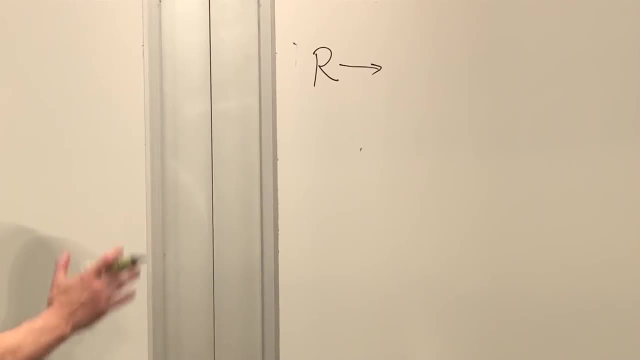 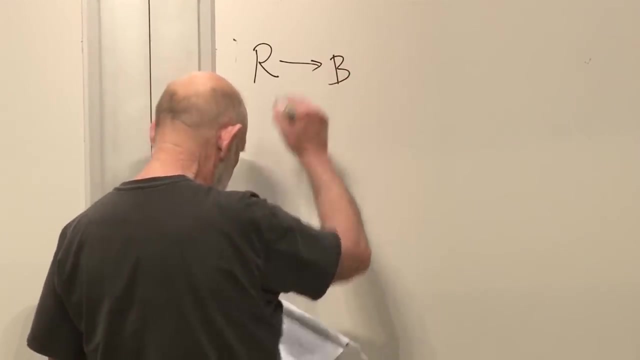 that I feel a need to emphasize it again. This is what a law of motion is. It's a rule telling you what the next configuration will be given. It's a rule of updating, of updating configurations: Red goes to blue, blue goes to yellow. 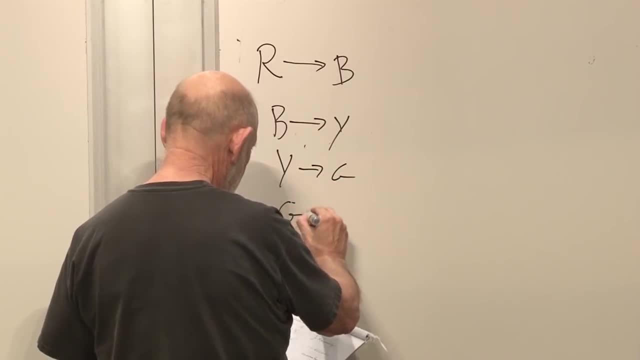 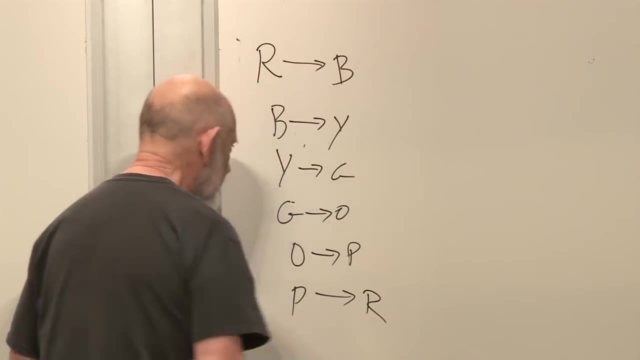 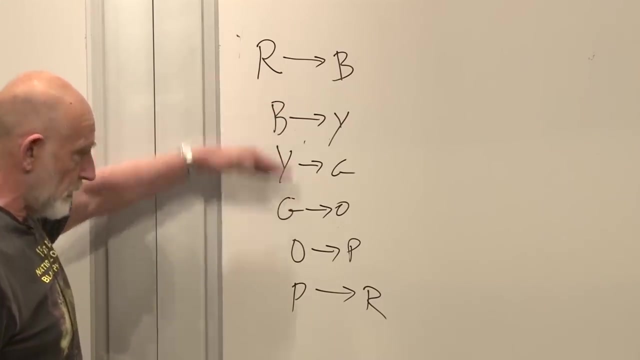 yellow goes to green, green goes to orange, orange goes to purple and purple goes back to red. Okay, Given the configuration, at any time, you know what it will be next and you know what it will continue to do, Of course. 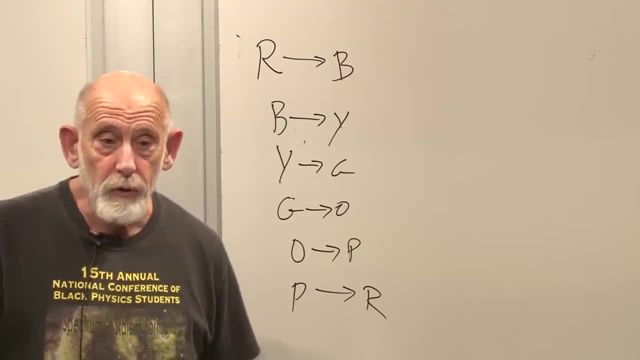 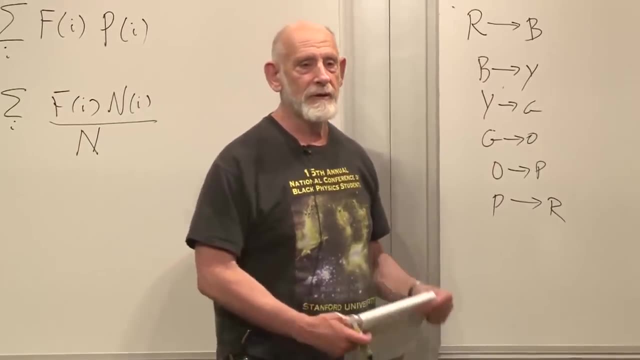 you may not know the law. Maybe all you know is that there is a law of this type. Alright, so you know what I'm going to do next. What am I going to do next? I'm going to draw this law as a diagram. 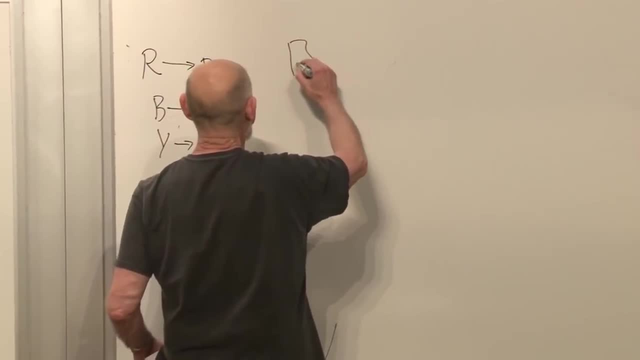 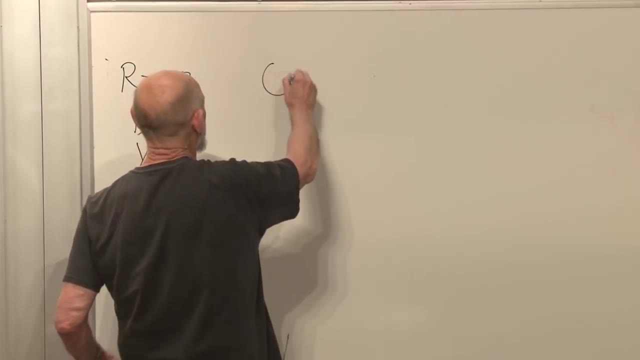 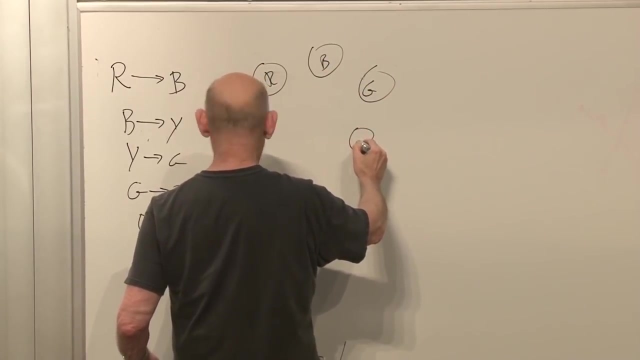 and you've all seen me do this in other contexts, so let's do it. We have red- too hard to draw squares. red, blue, green, orange. what happened? Oh, yellow, Yellow, orange, purple, Alright, so. 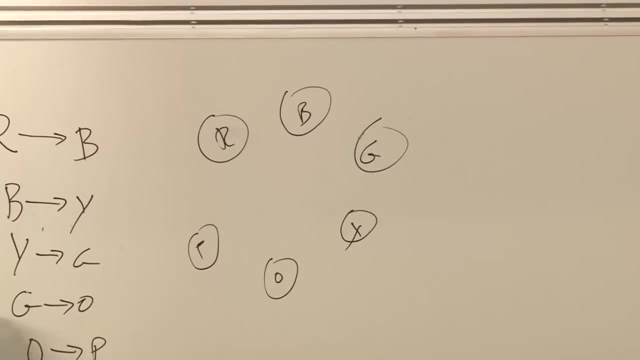 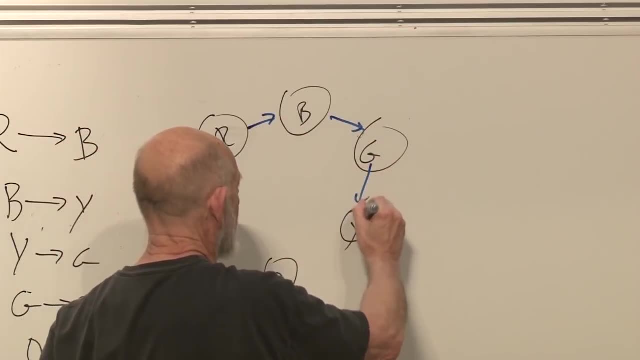 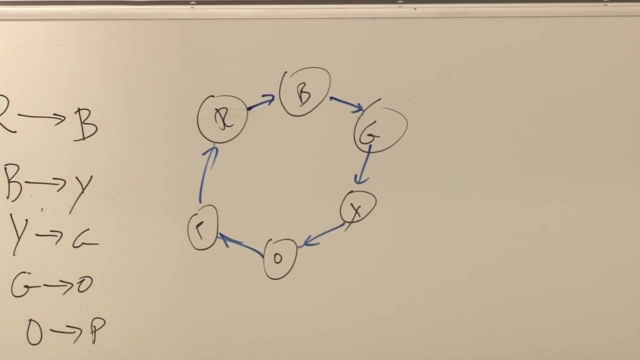 a law like this can be just represented by a set of lines connecting a set of arrows: red goes to blue, blue goes to green, green goes to yellow, yellow goes to orange, orange goes to purple, purple goes back to red. Making the assumption, 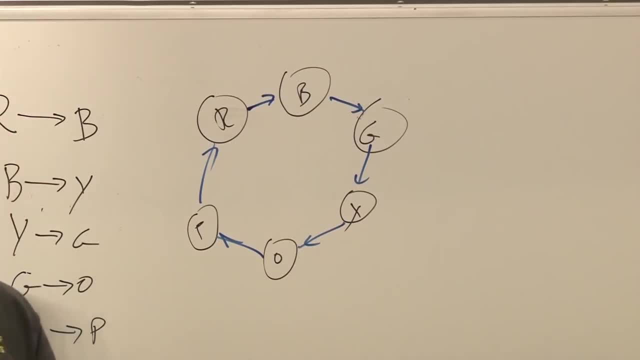 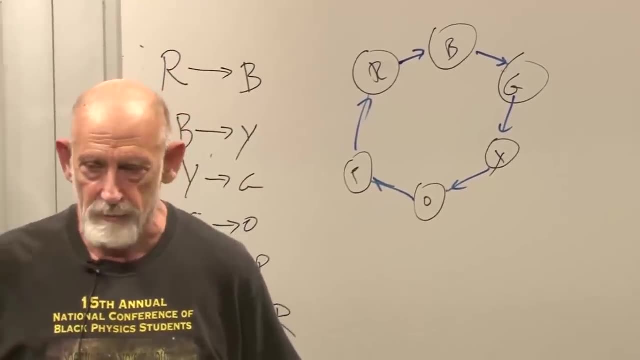 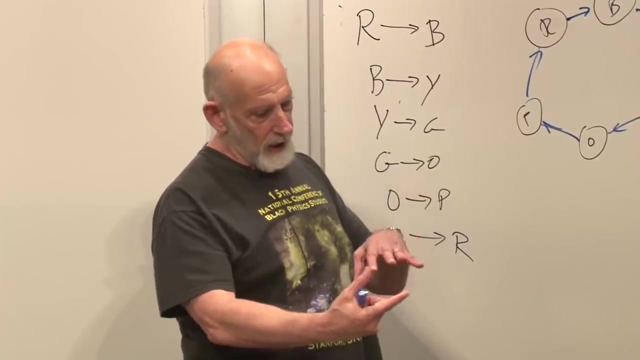 now that there's a discrete time interval between such events, I am not assuming that the cube has any symmetry to it anymore. The cube may not be symmetric at all. It may have points, you know. one edge, one face, maybe tiny, another face. 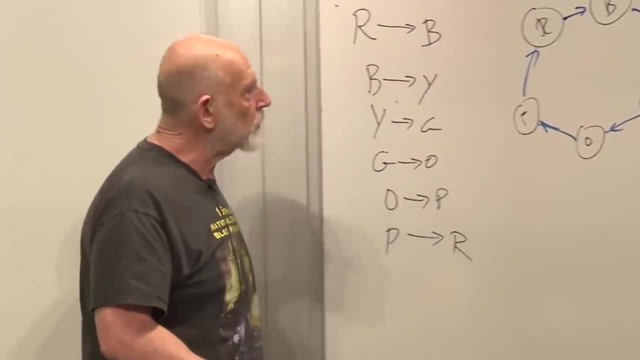 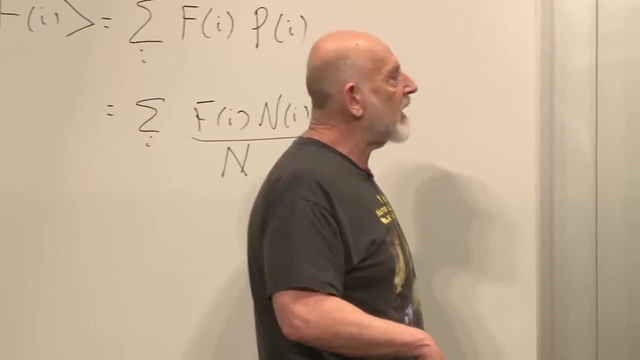 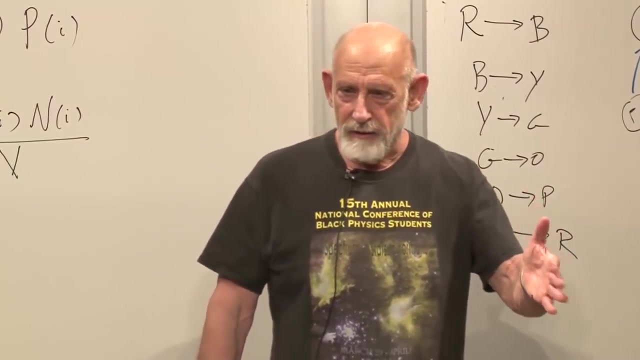 but if this is the rule- to go from one configuration to another and each step takes, let's say, a microsecond- I might have no idea where I begin, but I can still tell you if I let's say it's a microsecond. 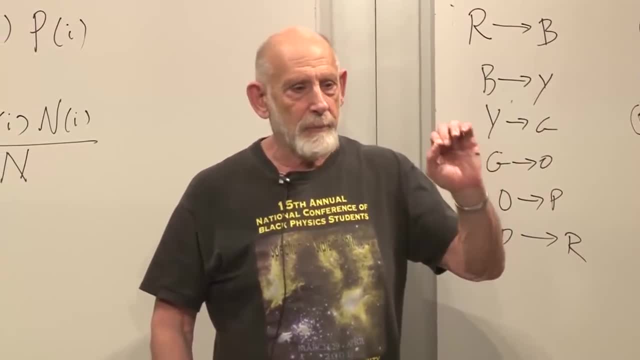 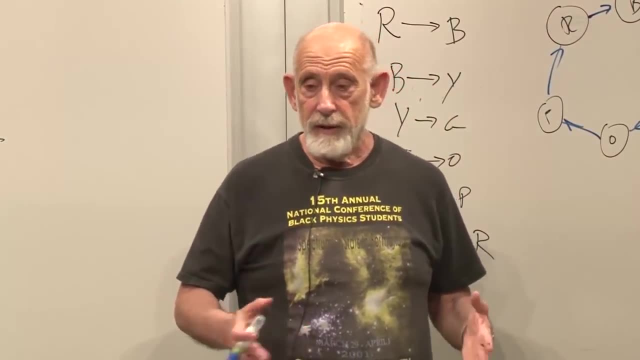 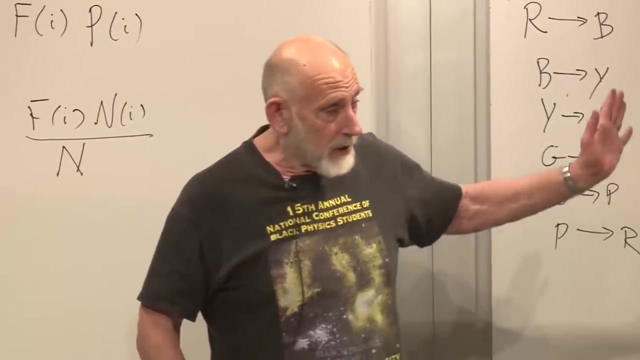 a microsecond and my job is to catch it at a particular instant and ask what the color is. I don't know where it started, but I can still tell you the probability for each one of these is one-sixth. It doesn't have to do with symmetry. 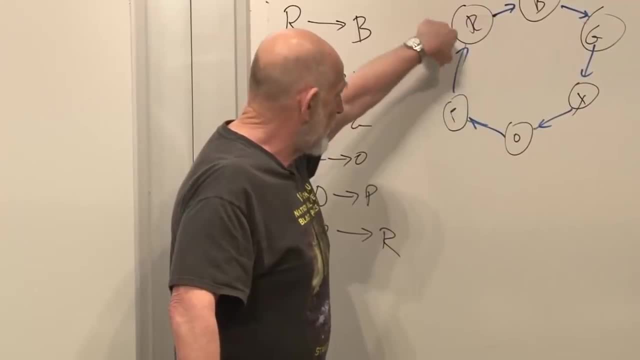 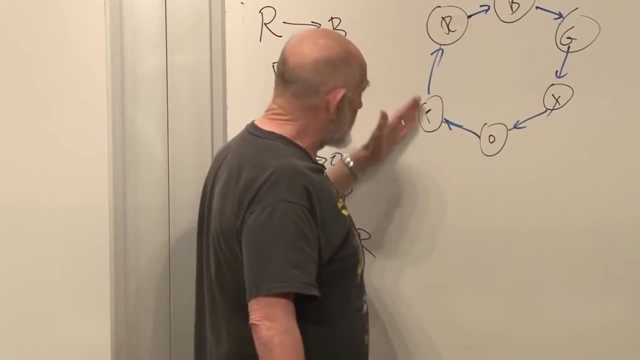 well, maybe it does have to do with some symmetry, but in this case it wouldn't be the symmetry of the structure of a die, it would just be the fact that, as it passes through these sequence of states, it spends one-sixth of its time red. 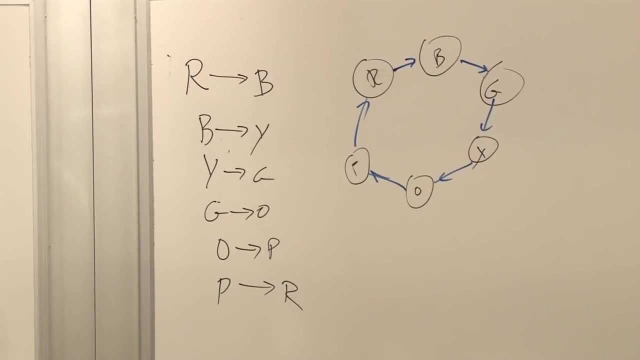 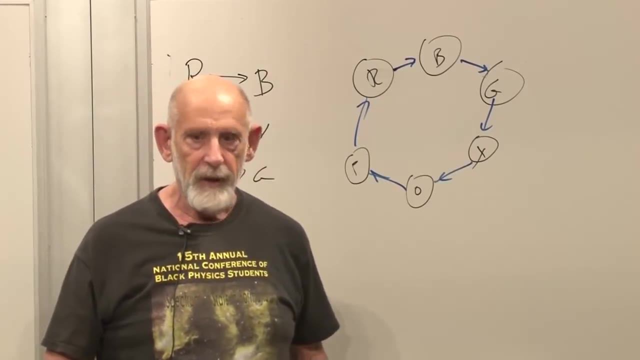 one-sixth of its time blue, one-sixth of its time green, and if I don't know where it starts and I just take a flash, you know a flash shot of it, my probability will be one-sixth, Now that 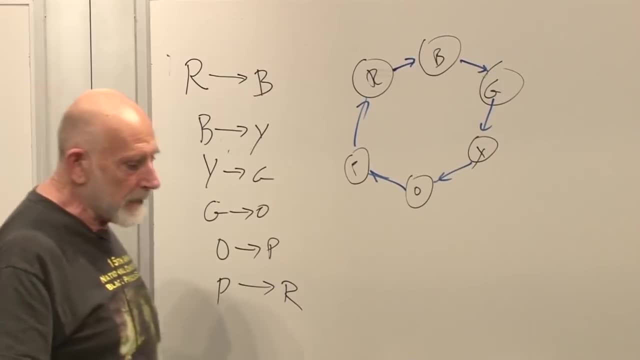 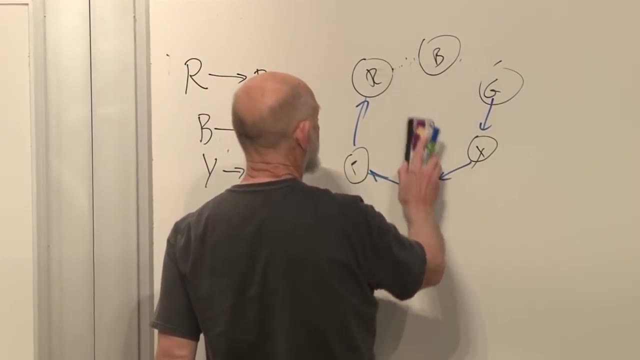 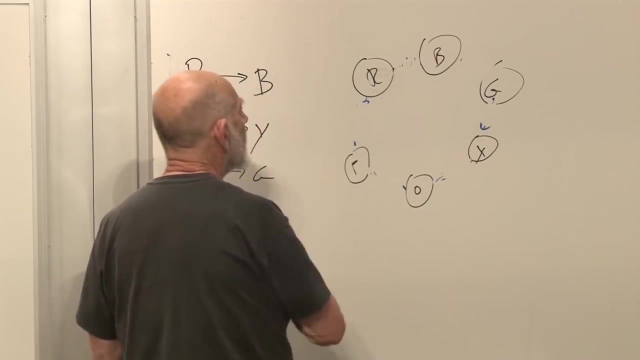 one-sixth did not really depend on knowing the detailed law. For example, the law could have been different. Let's make up a new law: Red goes to green, green goes to orange, orange goes to yellow, yellow goes to purple. 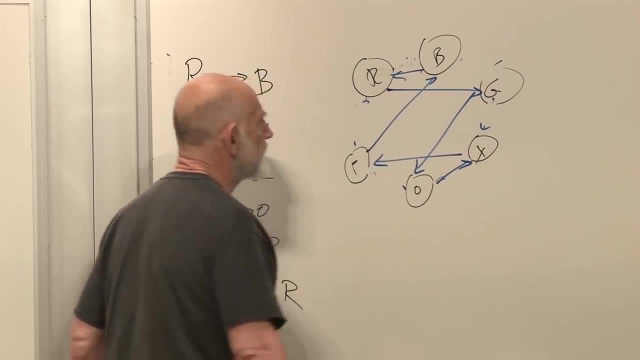 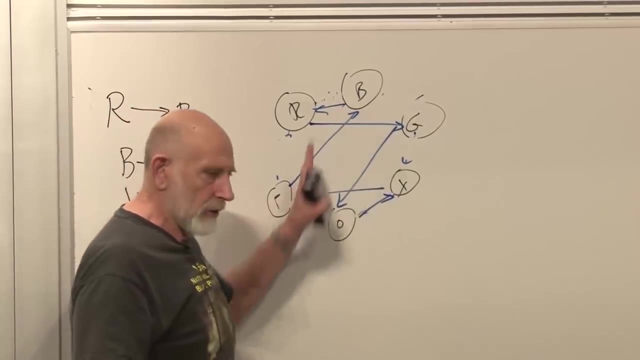 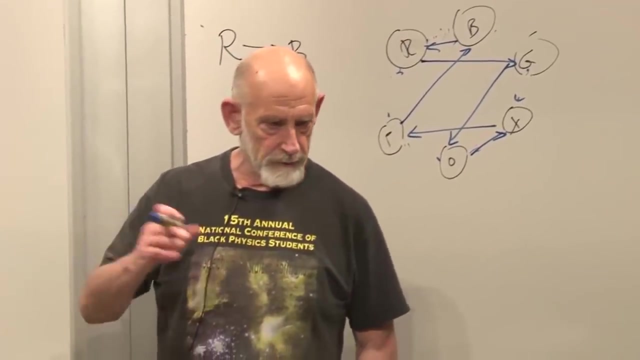 purple goes to blue and blue goes back to red. This shares with the previous law that there's a closed cycle of events in which you pass through each color once before you cycle around. You may not know which law of nature is for this system, but you can tell me. 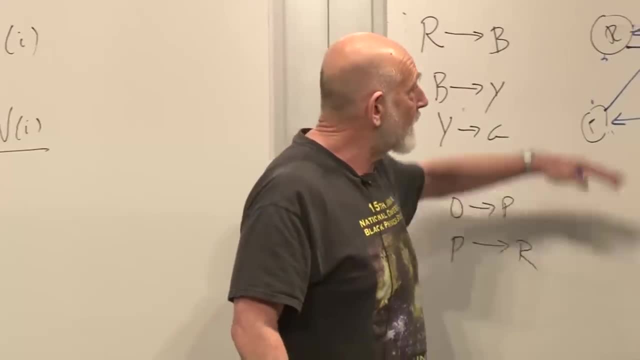 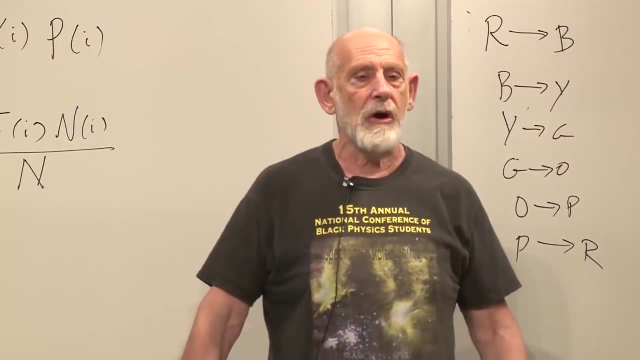 again that the probability will be one-sixth for each one of them. So this prediction of one-sixth doesn't depend on knowing the starting point and doesn't depend on knowing the law of physics. It's just important to know that there is a 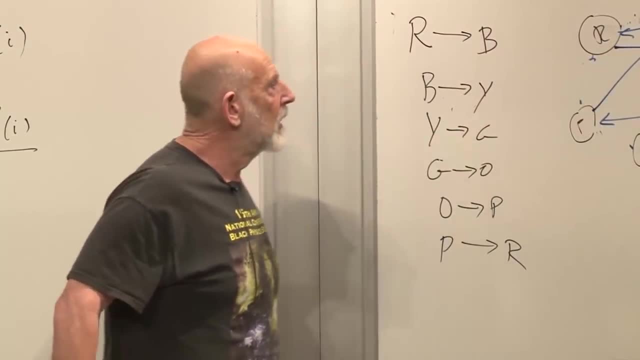 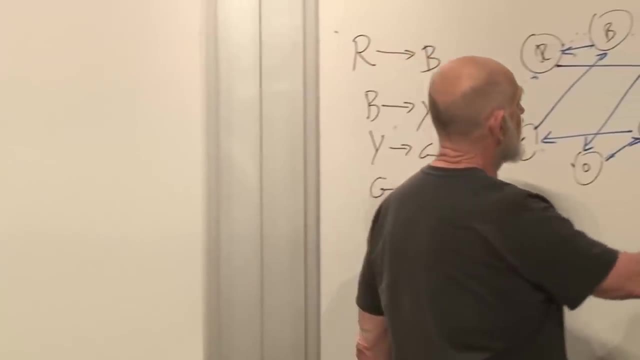 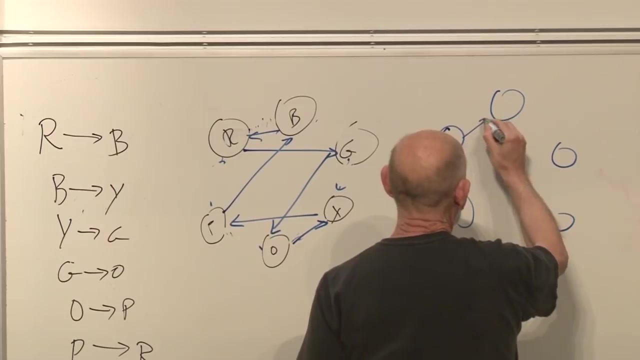 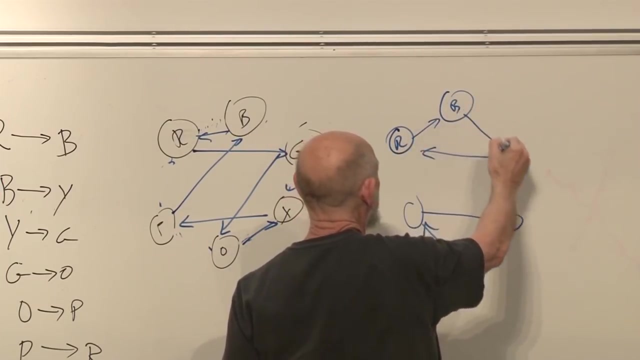 particular kind of law. Are there possible laws for this system which will not give you one-sixth? Yes, Let's write another law: Red, blue, green, yellow, orange, purple. This rule says that if you start with red, 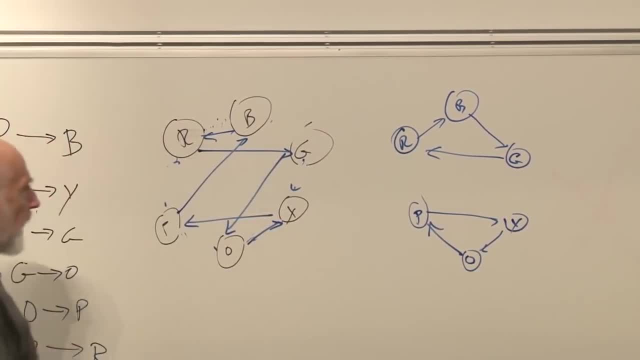 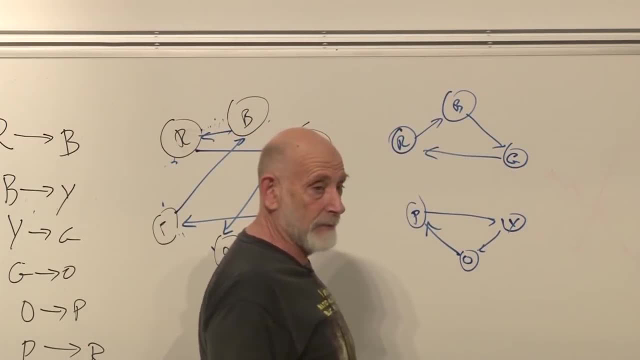 you go to blue. if you start with blue, you go to green, and if you get to green, you go back to red. Or if you start with purple, you go to yellow, yellow to orange orange, back to purple. Notice in this case. 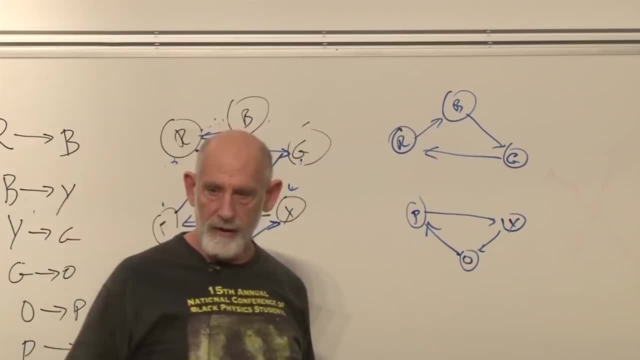 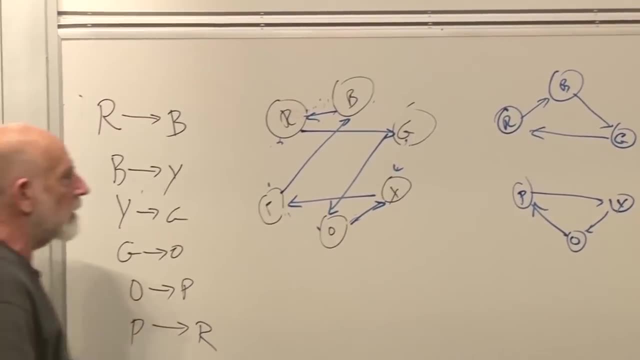 if you're on one of these two cycles, you stay there forever. If you knew you were on the upper cycle, if you knew you had started, it doesn't matter where you start, but if you knew that, you started on the upper cycle. 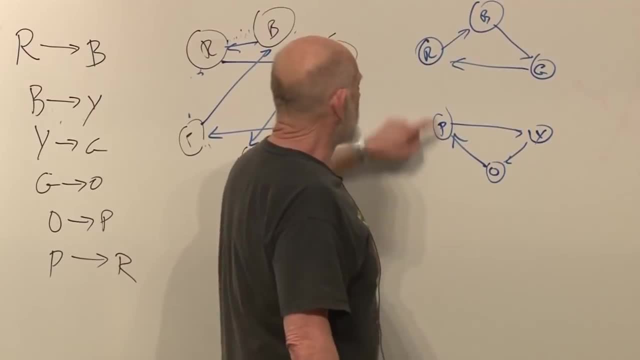 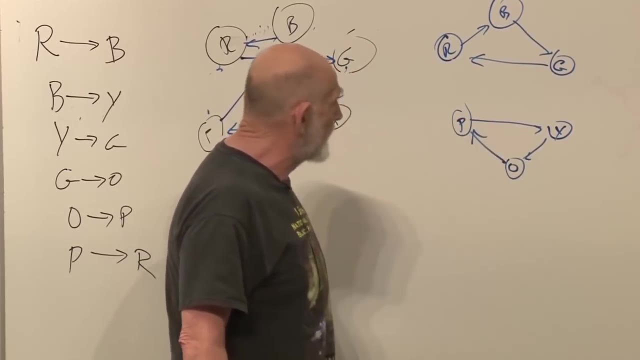 somewheres, then you would know that there was a one-third probability to be red, one-third probability to be blue and one-third probability to be green and zero probability to be red, yellow or orange. On the other hand, 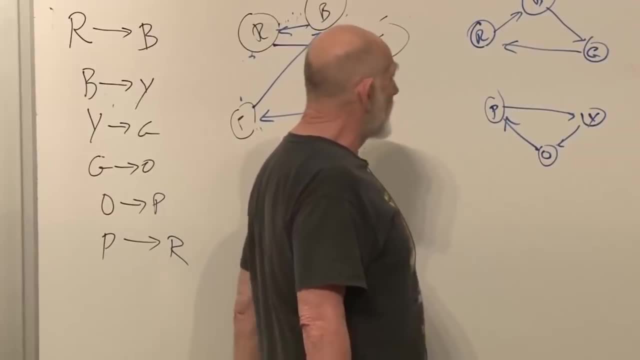 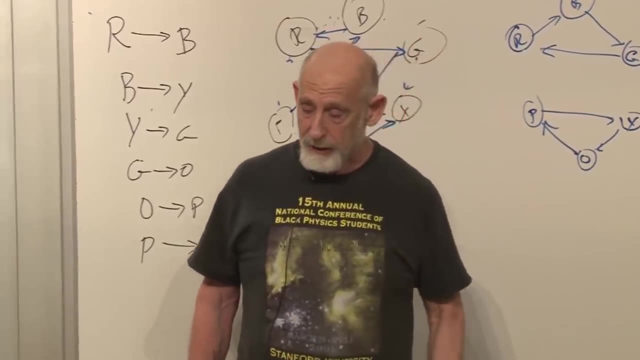 you could have started with the second cycle. you could have started with purple, might not have known where you started, but you knew that you started in the lower triangle, in the lower cycle. here. then you would know the probabilities of one-third for each of these. 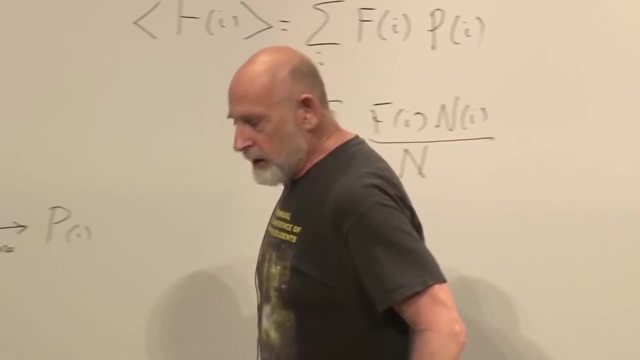 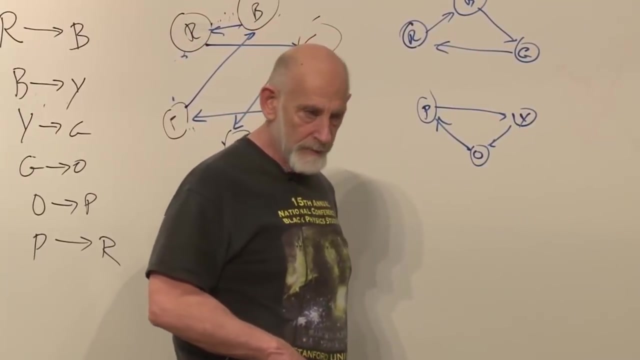 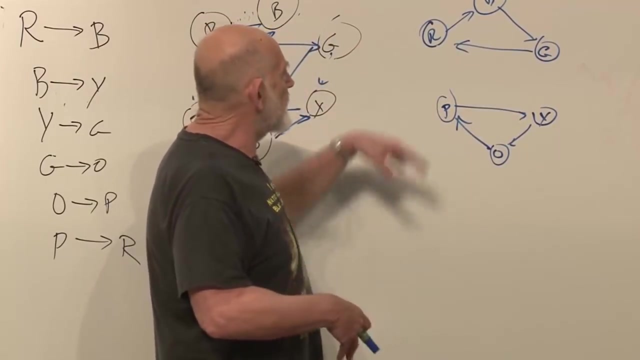 and zero for each of these. Now, what about a more general case? The more general case is to know, with some probability, that you start on the upper triangle here and with some other probability, on the lower triangle. In fact, let's give these triangles names. 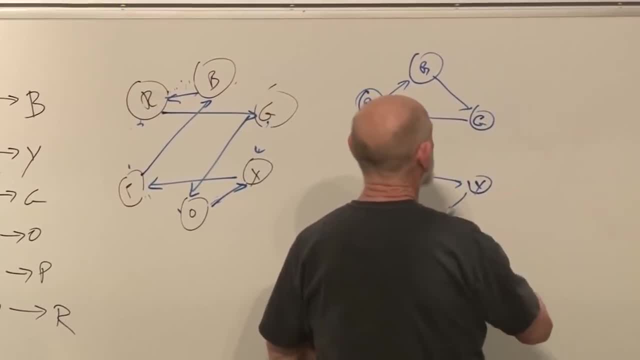 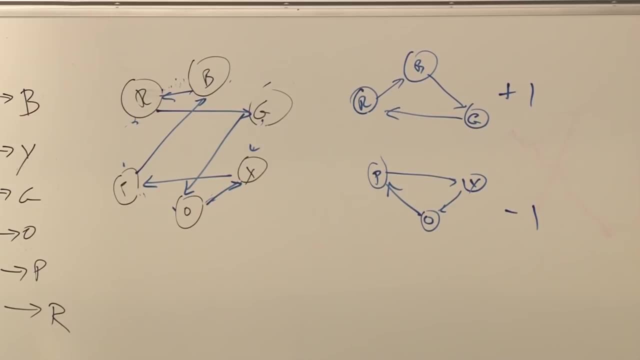 Let's call this triangle the plus-one triangle and this one the minus-one triangle, Just giving them names, Attaching to them a number, a numerical value. If you hear something or other is called plus-one, something or other is called minus-one. 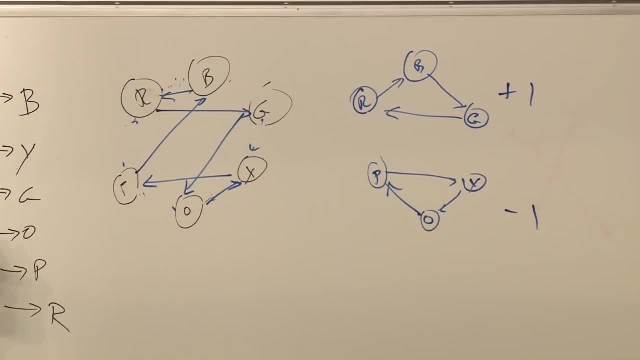 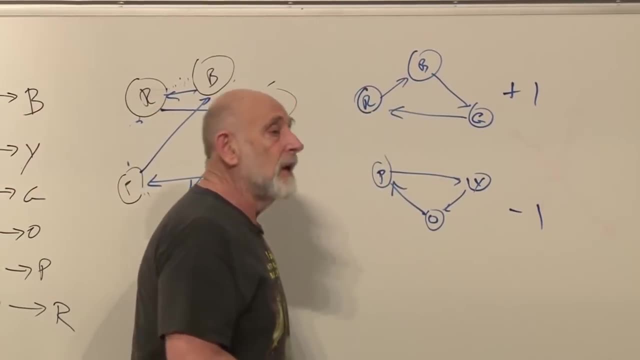 Alright, now you have to append. you have to start with something you've got to get from someplace else. It doesn't follow from symmetry and it doesn't follow from cycling through the system: some probability that you're either on cycle plus-one. 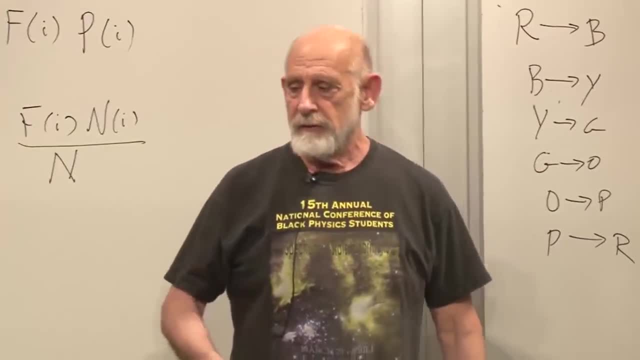 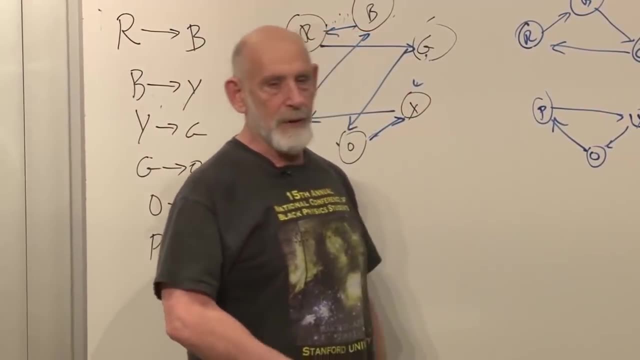 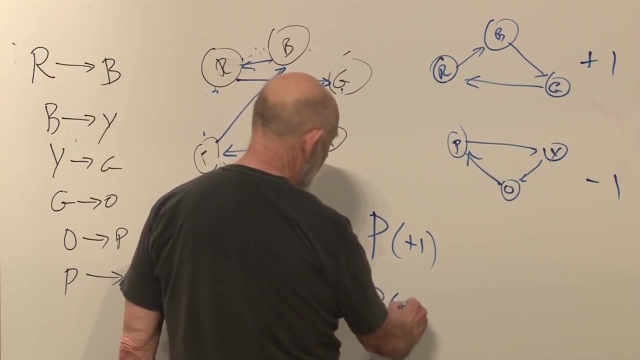 or cycle minus-one. Where might that come from? Well, flipping somebody else's coin over here, flipping a coin over here, might decide which of these two It might be a biased coin. so you will have a probability to be plus-one and a probability to be minus-one. 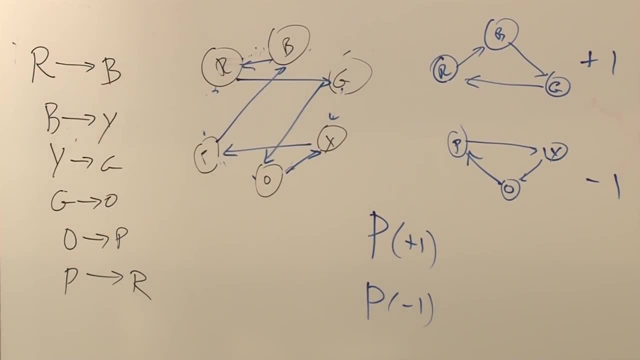 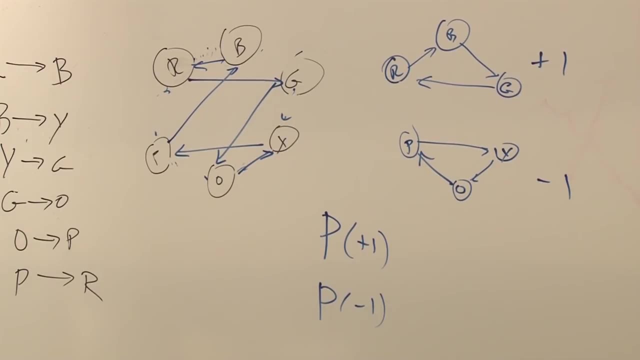 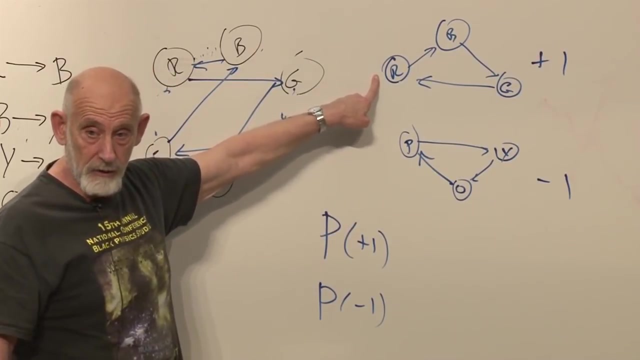 These two probabilities are not probabilities for individual colors. they're probabilities for individual cycles. Okay, now what's the probability for blue? The probability for blue begins with the probability that you're on the first cycle, times the probability that, if you're on the first cycle, 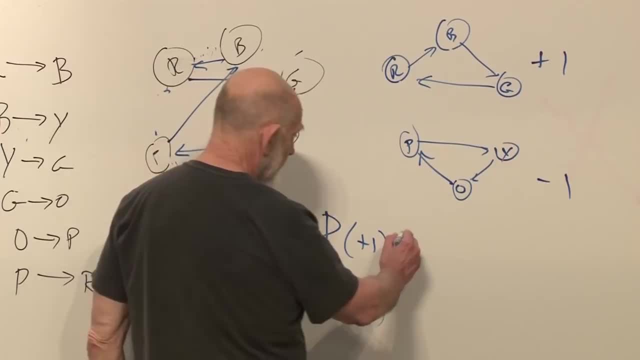 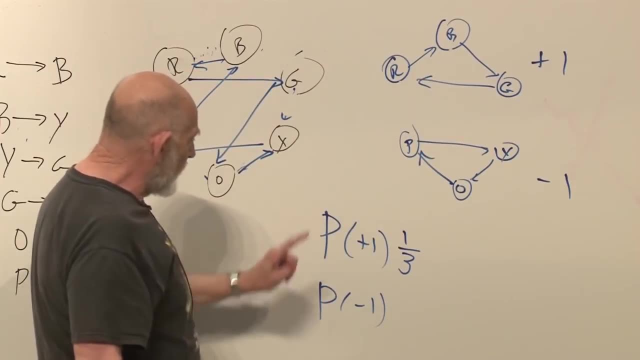 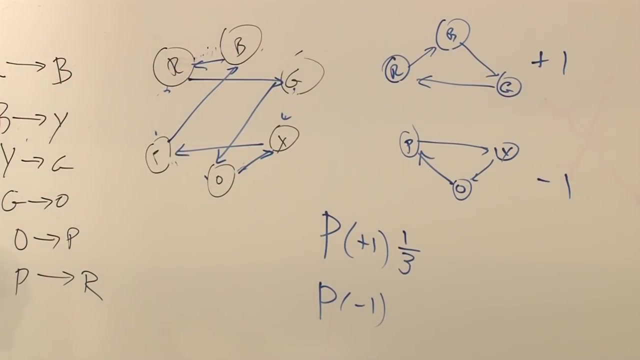 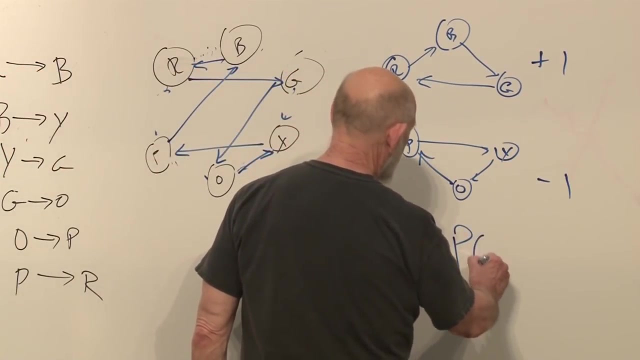 you get blue. That's one-third. So the probability for blue, red or green is one-third. the probability that you're on the first cycle, and likewise the probability that you're at yellow, will be. this is the probability for red, blue. 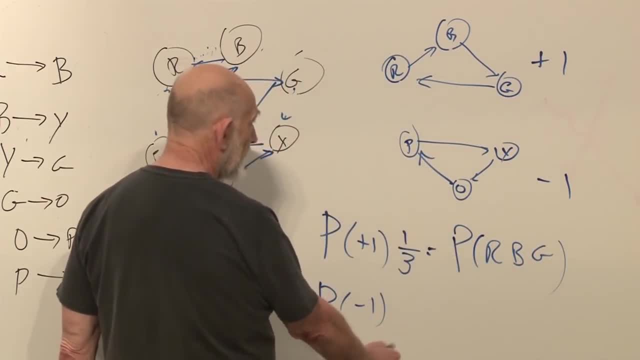 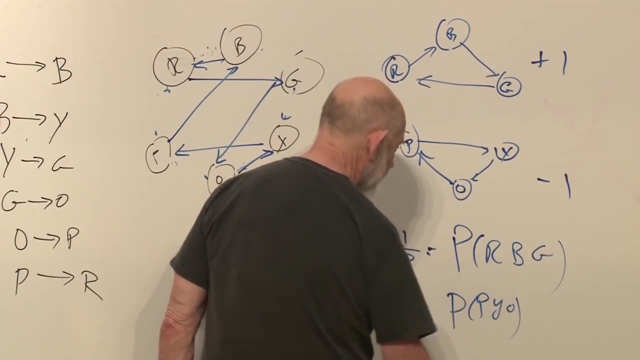 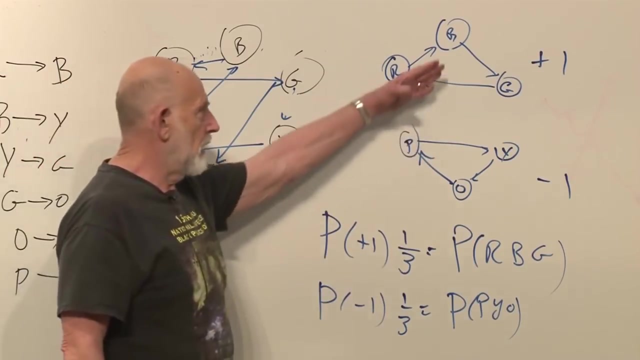 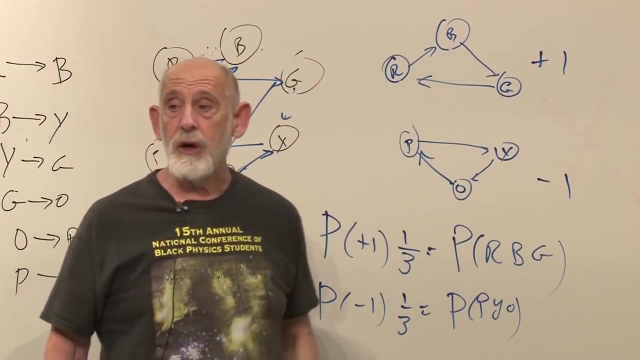 or green in this case, and this times, one-third will be the probability for purple, yellow or orange. Okay, so in this case you need to supply another probability that you've got to get from somewhere else. This case here is what we call having a. 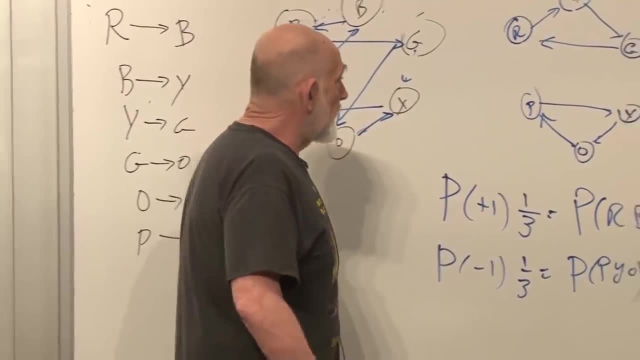 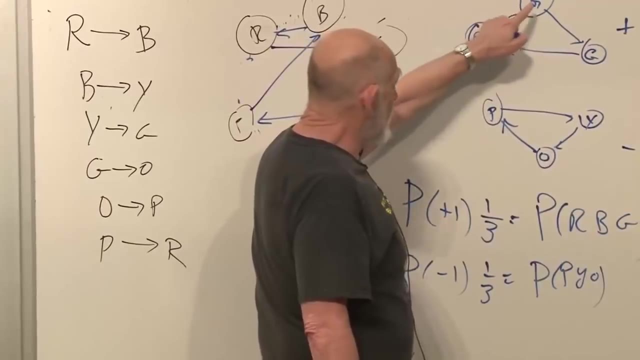 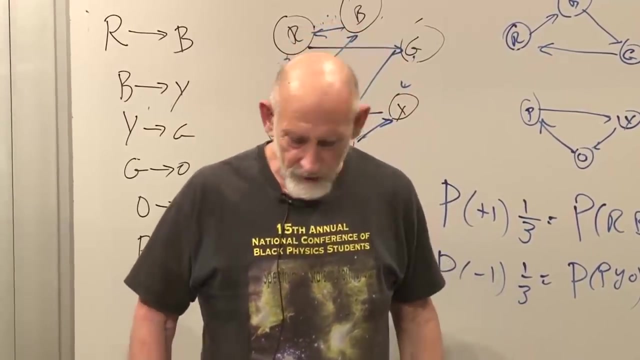 conservation law. In this case, the conservation law would be just the conservation of this number- red, blue and green. we've assigned the value plus one. That plus one could be the energy, or it could be something else. I tend to call it the zilch, for some reason. 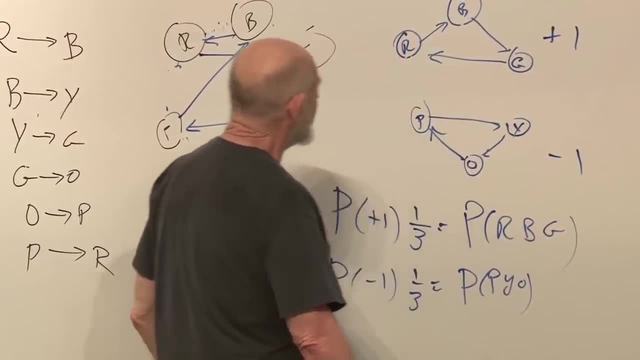 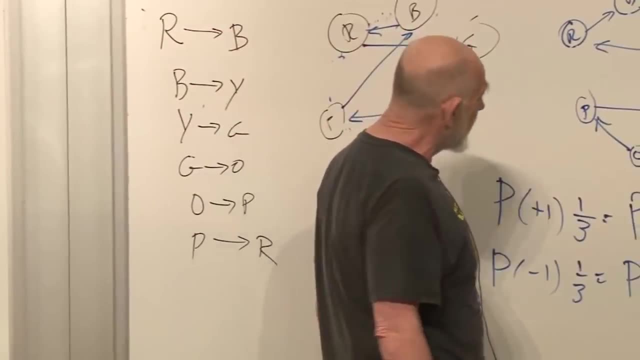 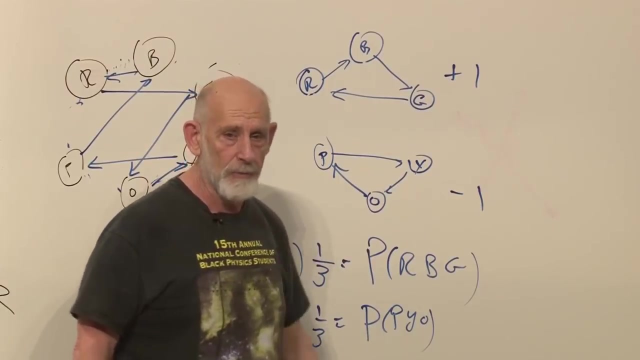 I call everything a zilch if there is no name for it. Yeah, so anyway, let's think of it as the energy. to keep things familiar, The energy of these three configurations might all be plus one, and the energy of these three configurations might all be minus one. 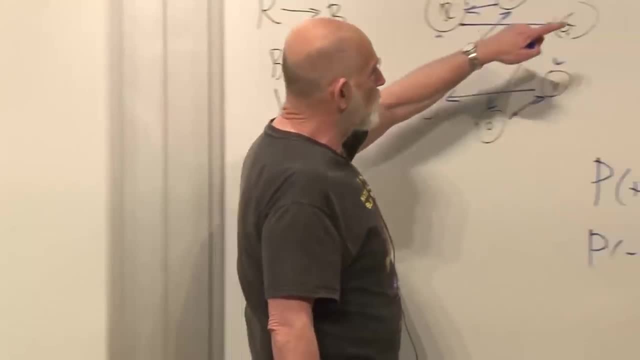 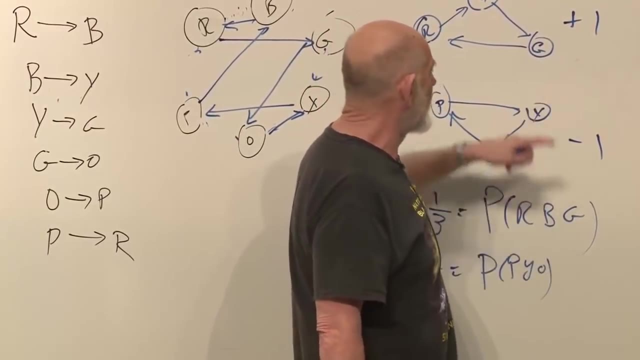 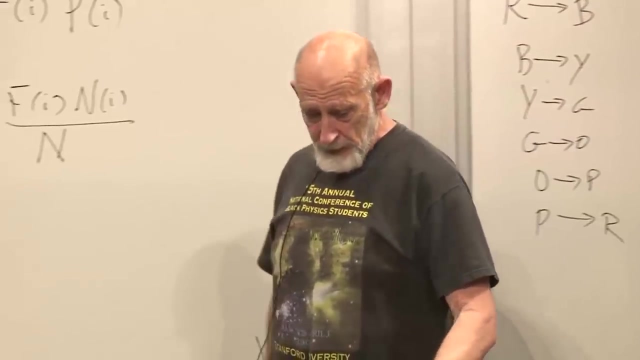 And the point is that because the rule keeps you always on the same cycle, that quantity, energy, zilch, whatever we call it, is conserved. It doesn't change. That's what a conservation law is. A conservation law is that the configuration space. 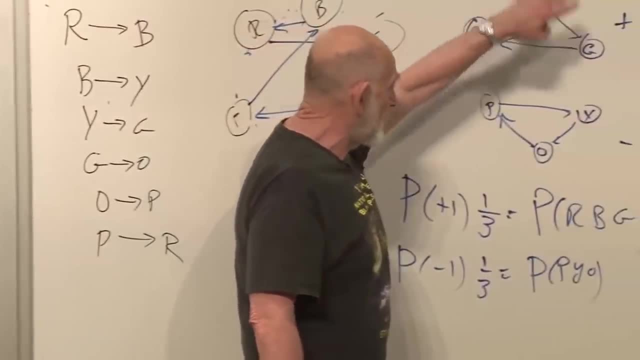 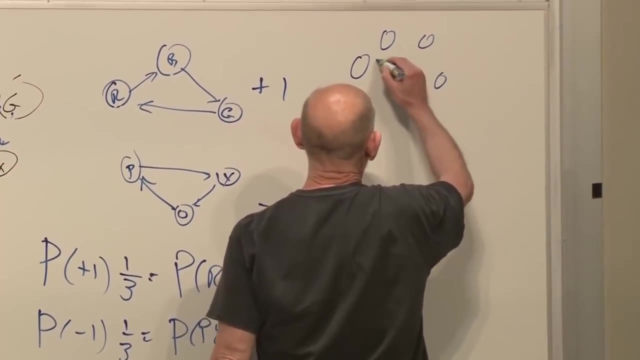 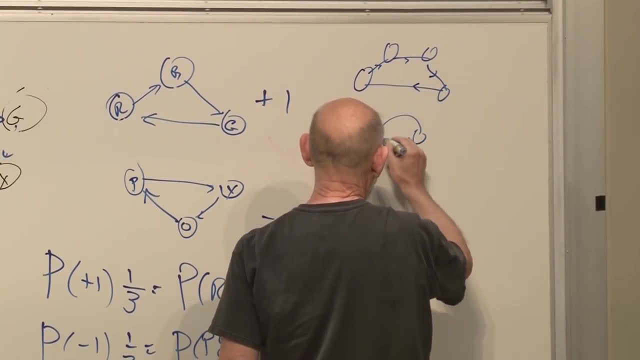 the space of possibilities divides up into cycles like this. Now, the cycles don't have to have equal size. Here's another case: One, two, three, four. you go around this way and then the two guys over here go into each other. 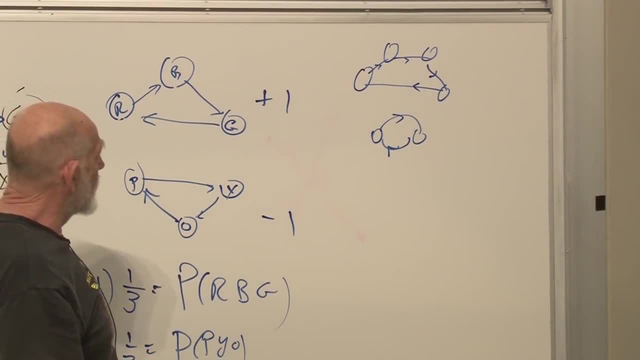 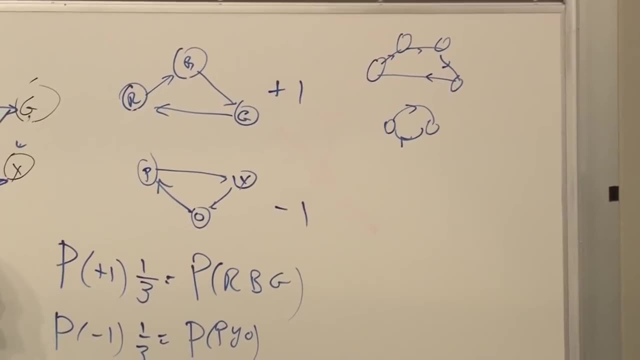 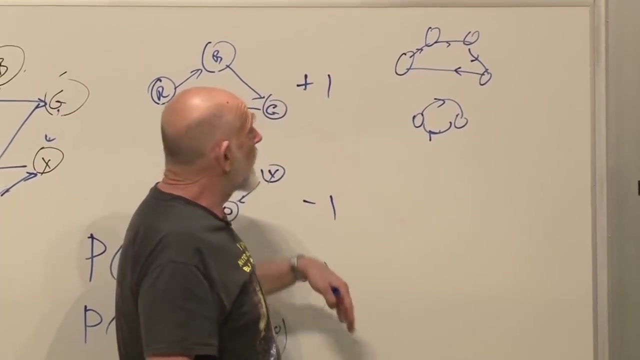 So red goes to blue, goes to green, goes to purple. that's the upper cycle here, and the lower cycle is yellow goes to orange, goes to yellow, goes to orange. Still, we have a conservation law here. it's just the number of states with one value. 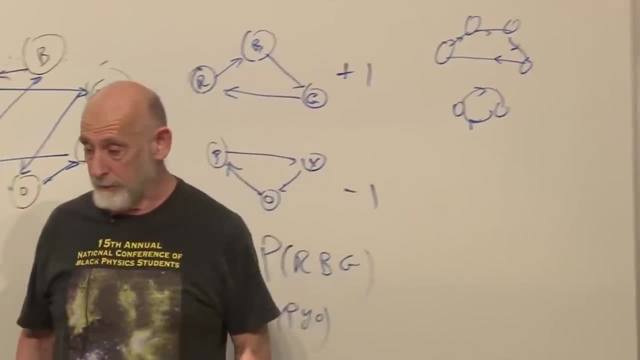 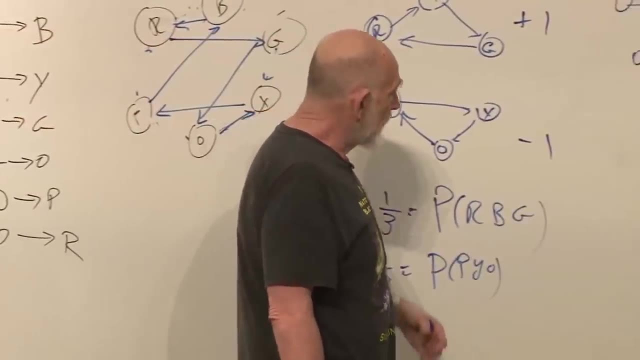 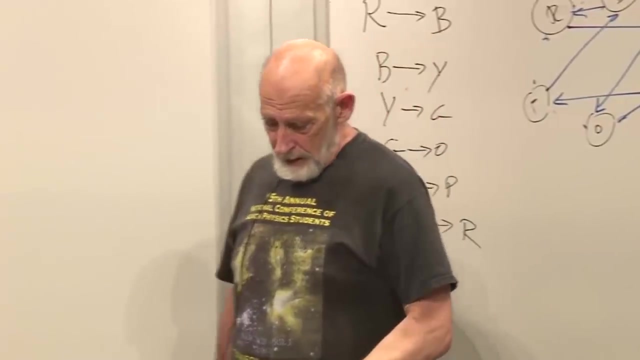 of the conserved quantity is not the same as the number of states with the other value, but still it's a conservation law and again, somebody would have to supply for you some idea of the relative probabilities of these two. Where that comes from is part of the study of statistical mechanics. 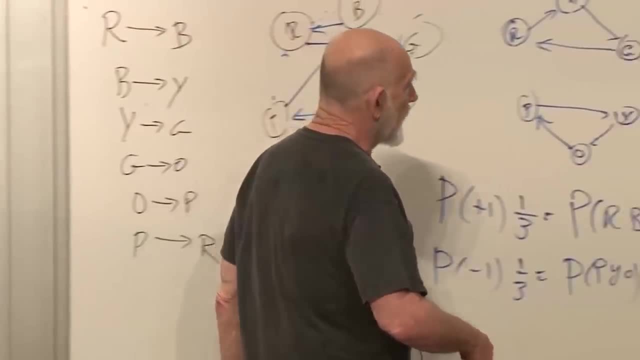 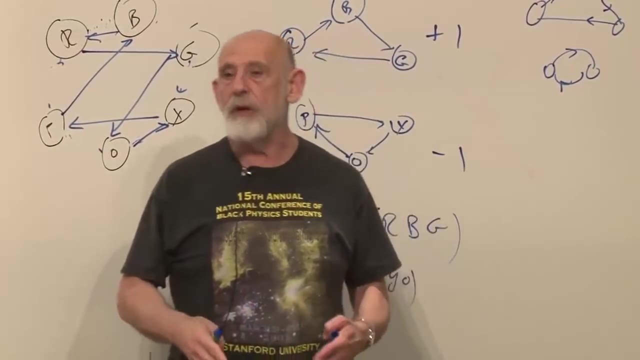 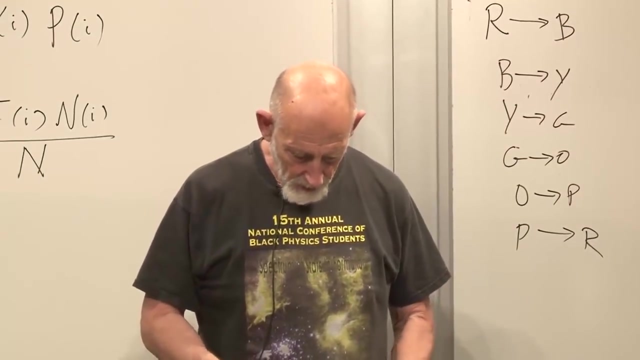 and the other part of the study has to do with saying: if I know I'm on one of these tracks, how much time do I spend with each particular configuration? That's what determines probabilities of statistical mechanics, Some a priori probability from somewheres. 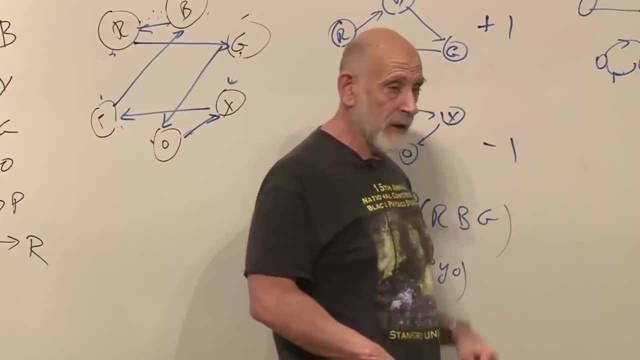 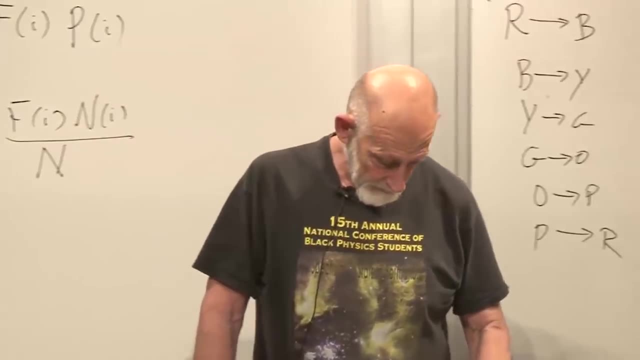 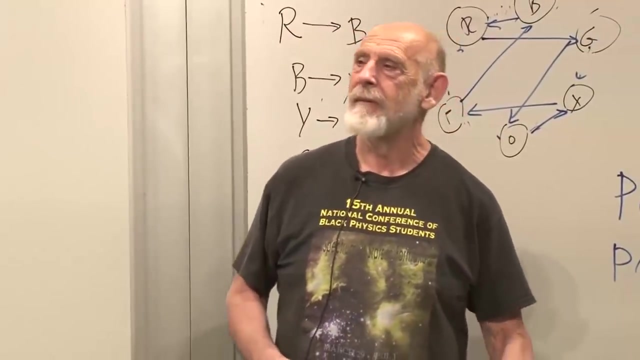 that tells you the probabilities for different conserved quantities and cycling through the system. Yeah, question No, No. okay, So so far you're assuming that within any conservation arena, if you will, the probabilities of all states are the same. 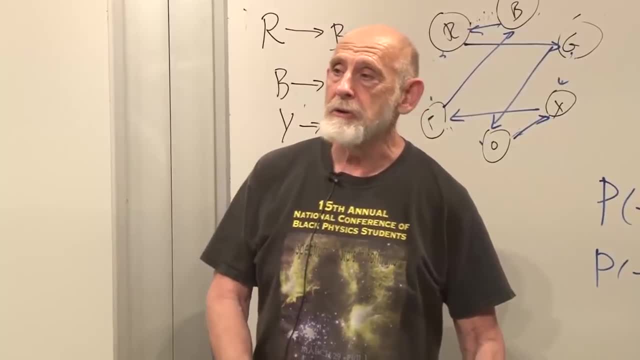 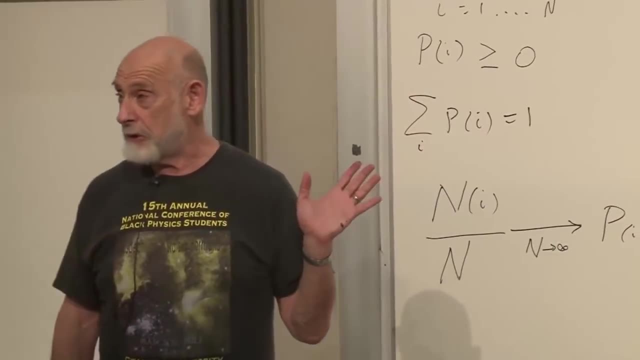 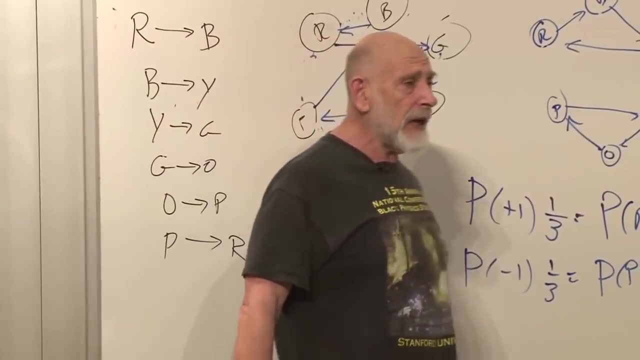 The time spent in each state is the same Right, so it's completely deterministic. laws are completely deterministic. this would be classical physics laws, completely deterministic. no real ambiguity of what the state is. except you're kind of lazy- you didn't determine the initial condition. 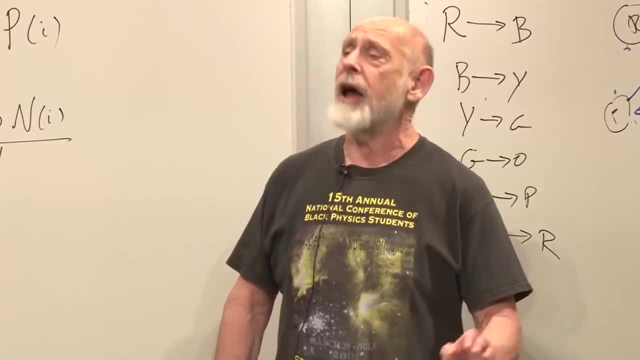 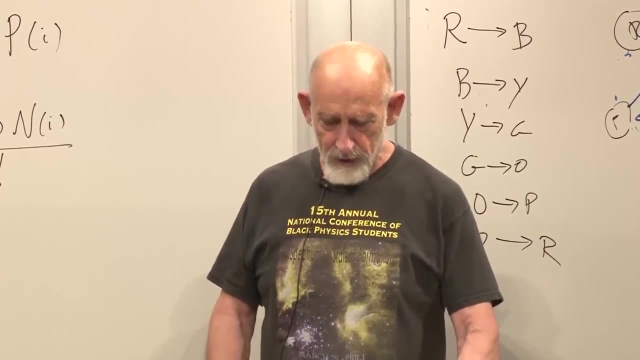 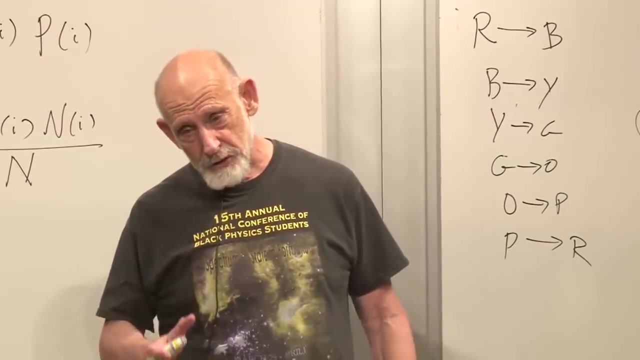 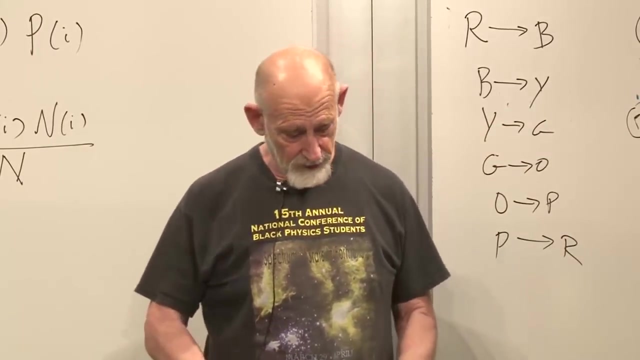 your. your timing wasn't very good. each state only lasts for a microsecond. you're a lazy guy and you only have a resolution of a millisecond, but nevertheless you're able to take a very quick flash picture and pick out one of the states. that's the circumstance that we're. 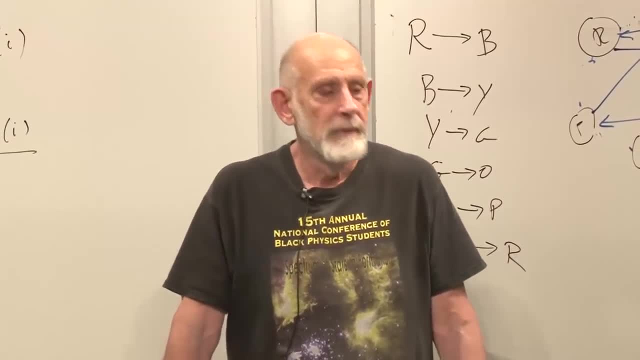 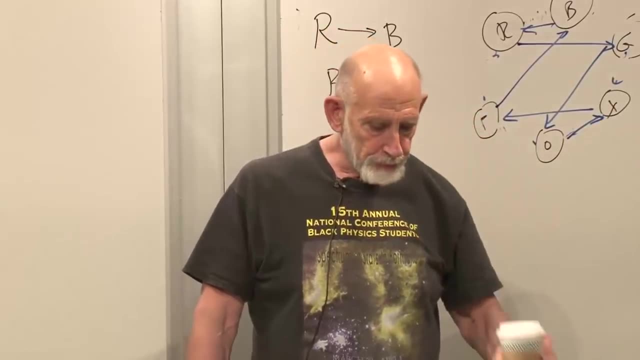 talking about? If we take two pictures, is it reasonable to then assume that if the first picture indicated that we are in one cycle, the later one should indicate the same cycle, since it couldn't get out of it? Yes, that's a good assumption. 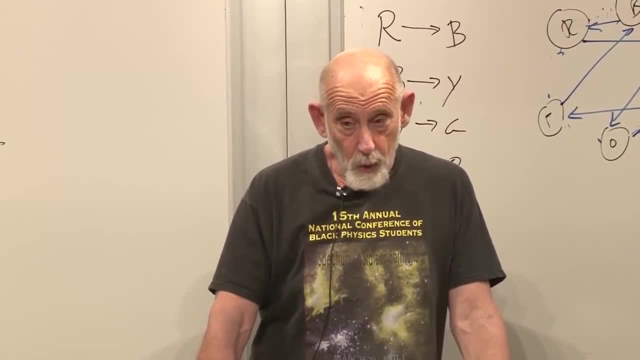 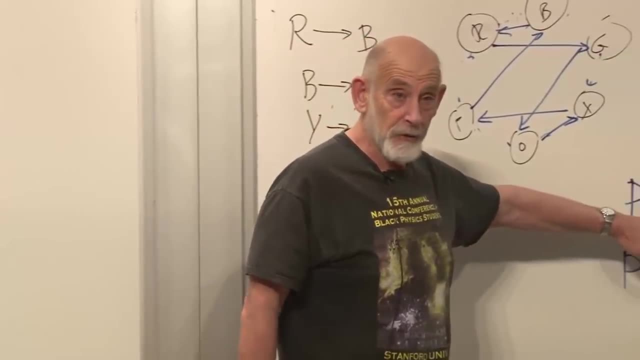 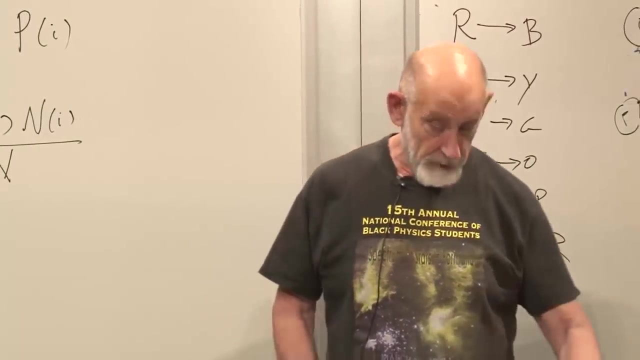 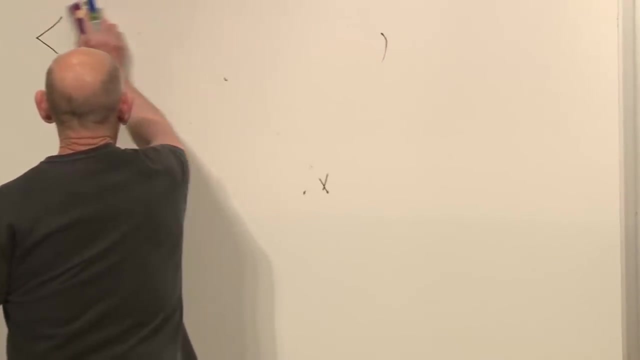 yes, right, so once you determine the value of some conserved quantities, then you know it and then you can reset the probabilities for it. okay, unless? alright. so let's talk about honest energy for a minute. yes, if we have a closed system to represent. 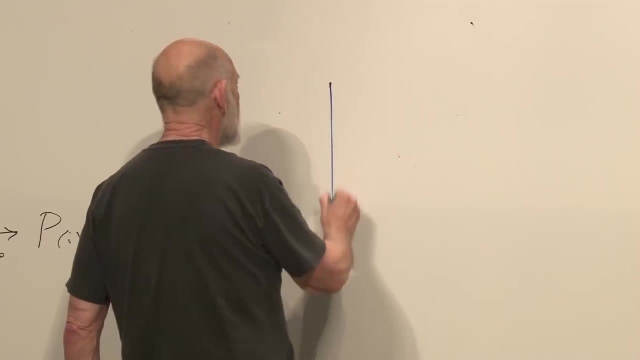 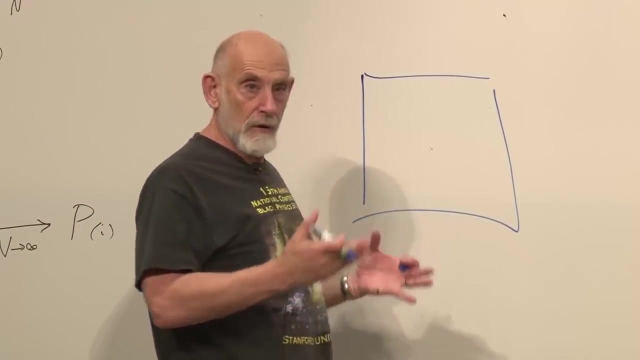 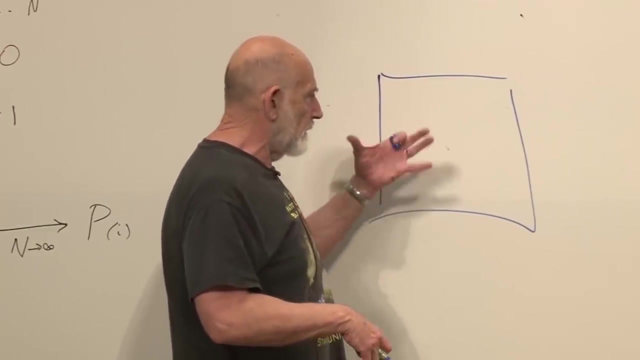 the closed system. I will just draw a box closed now. closed means that it's not in interaction with anything else and therefore can be thought of as a whole universe unto itself. okay, it has an energy. the energy is some function of the state of the system, whatever. 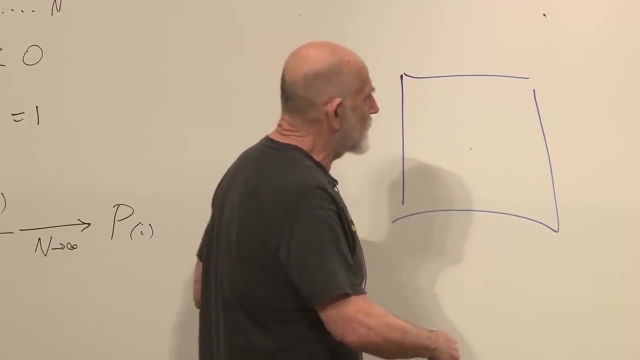 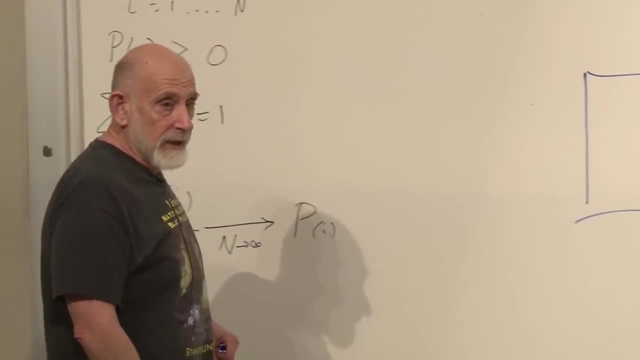 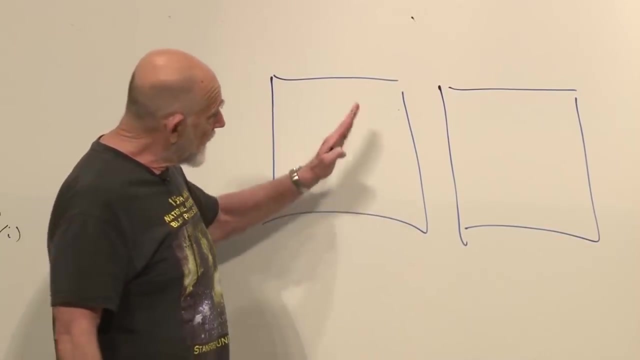 determines the state of the system. now let's suppose we have another closed system which is built out of two identical or not identical versions of the same thing. now, if they're both closed systems, there will be two conserved quantities: the energy of this system and the 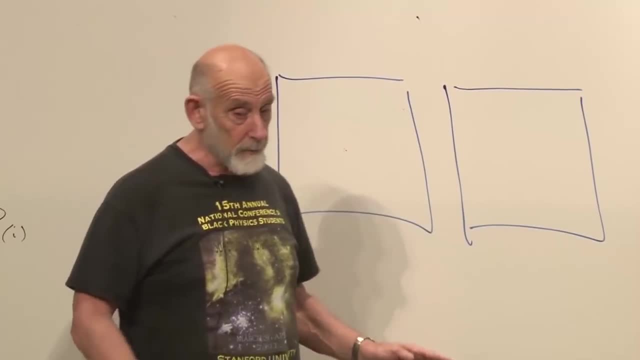 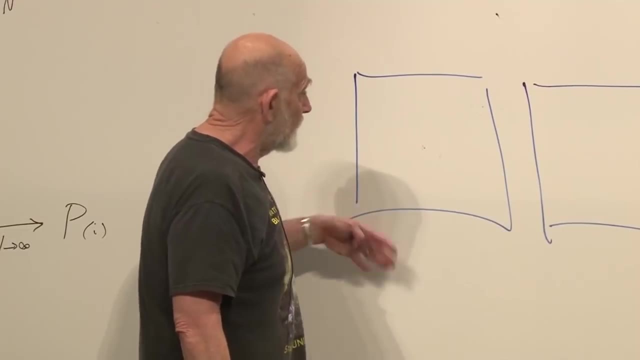 energy of this system and they'll both be separately conserved. why? because they don't talk to each other, they don't interact with each other. the two energies are conserved and you could have probabilities for each of those individuals. but now, supposing they're connected, 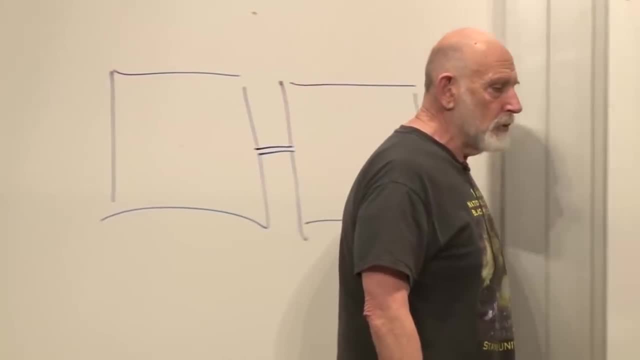 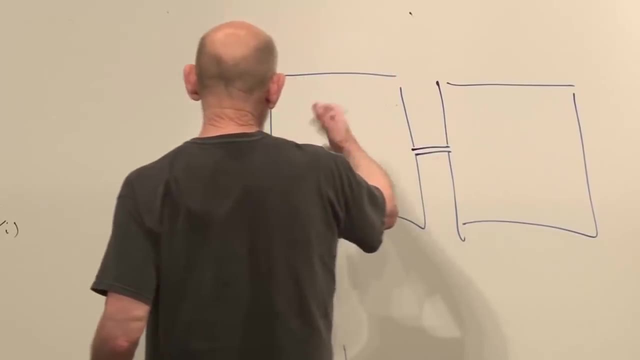 they're connected by a little tiny tube which allows energy to flow back and forth. then there's only one conserved quantity, the total energy, and it's sort of split between the two of them and you can ask what's you can then ask? 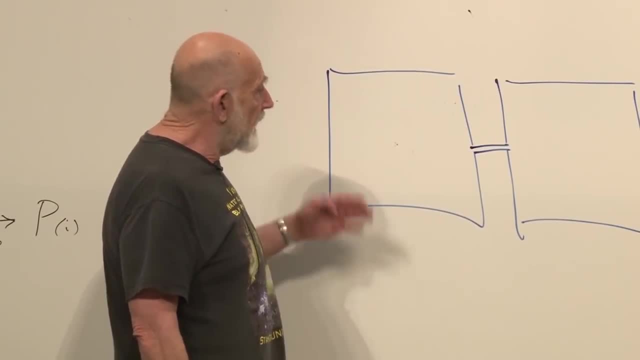 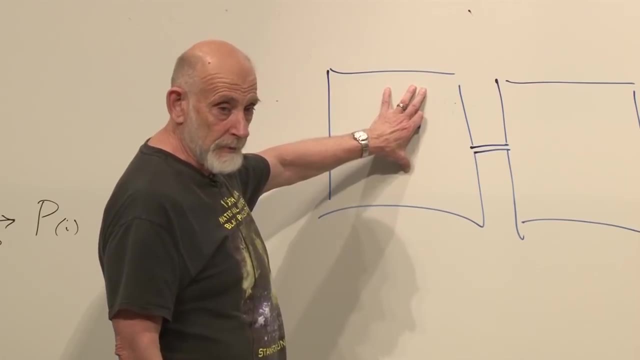 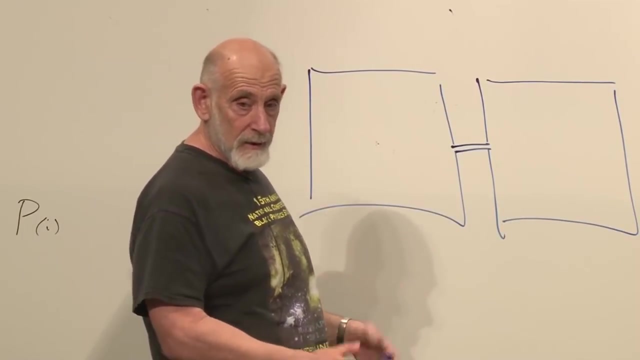 what is the probability? given a total amount of energy, you could ask what's the probability that the energy of one subsystem is one thing and the energy of the other subsystem is the other. if the two boxes are equal, you would expect on the average they have equal. 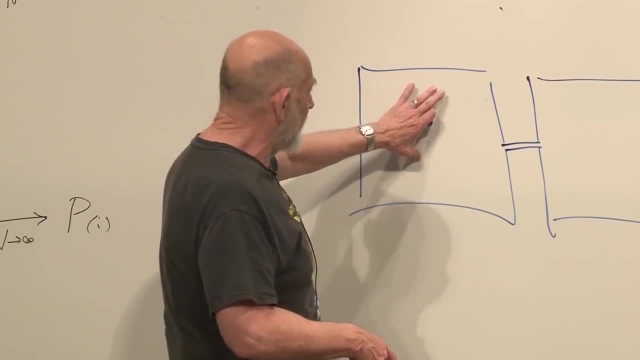 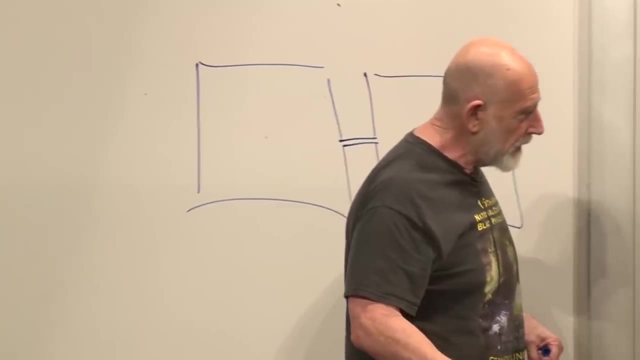 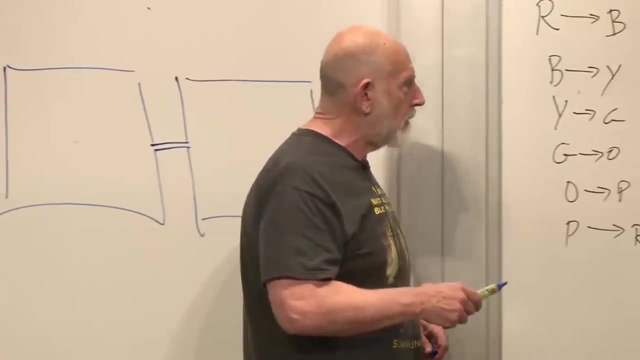 energy. but you can still ask what's the probability for a given energy in this box, given some overall piece of information. so that's a circumstance where it may be that, giving the probability for which cycle you're on now, which cycle you're on? I'm talking about the cycle. 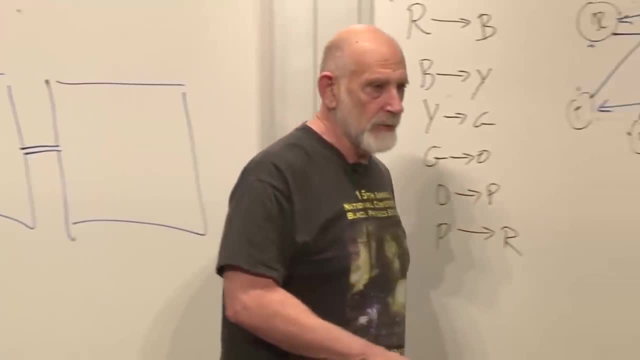 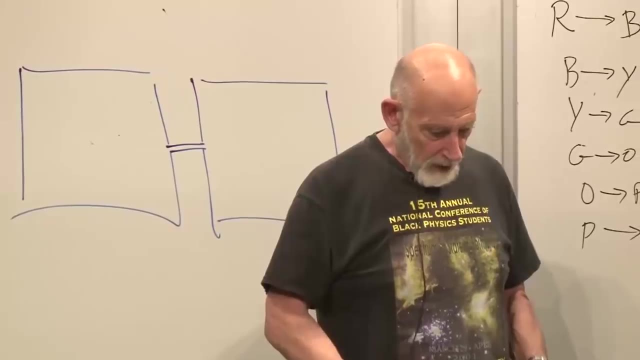 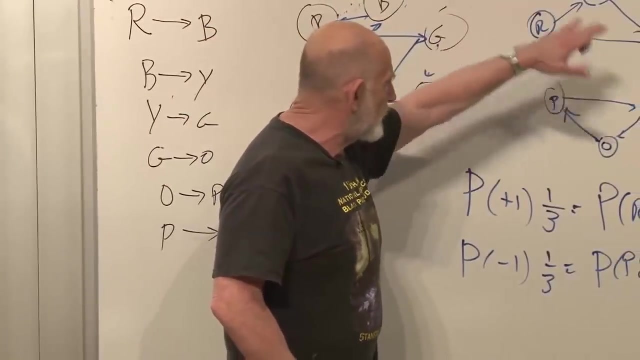 of one of these systems here may be determined by thinking about the system as part of a bigger system, and we're going to do that. that's important, but in general, you need some other ingredient besides just cycling around through the system here to tell you the relative probabilities. 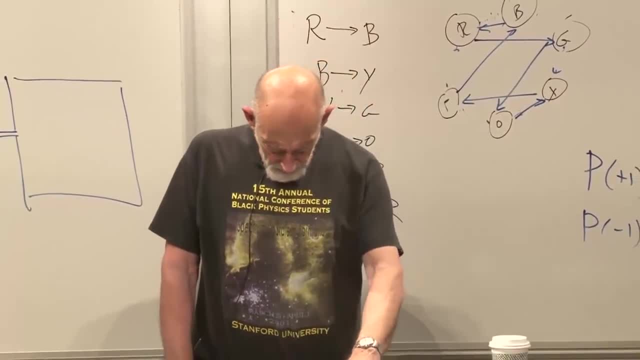 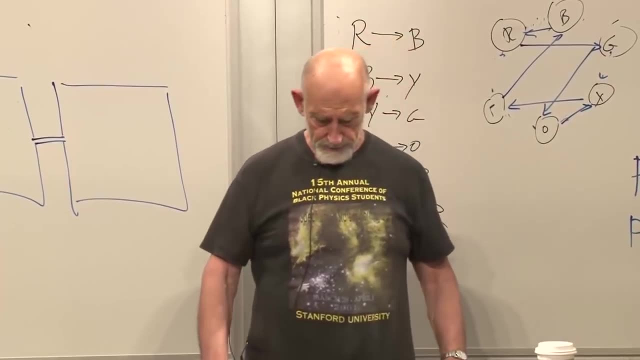 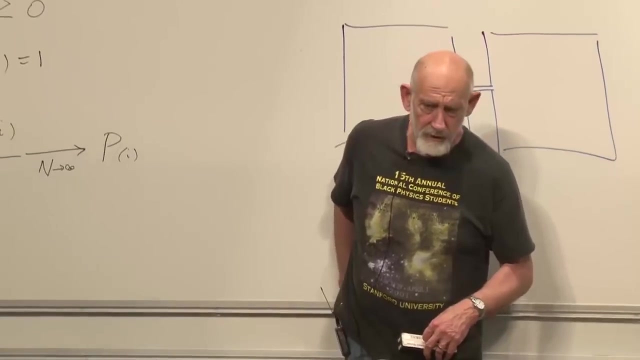 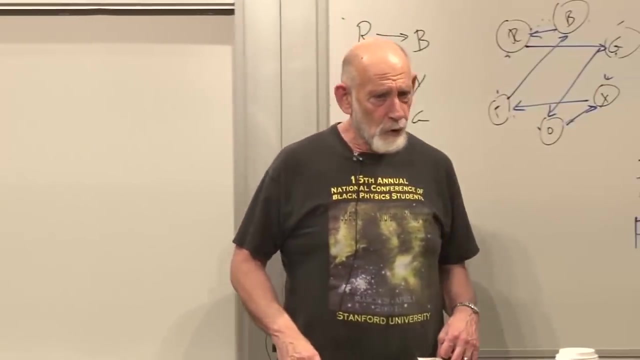 of conserved quantities. okay, so we're off and flying with statistical mechanics. there are bad laws by bad laws. I don't not in the sense of DOMA or any of those kind of laws, but but in the sense that the rules of physics don't allow them. 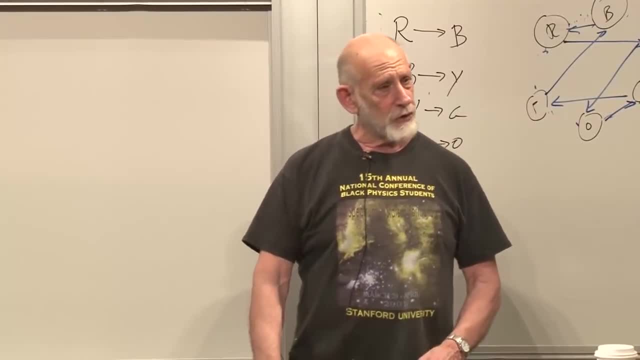 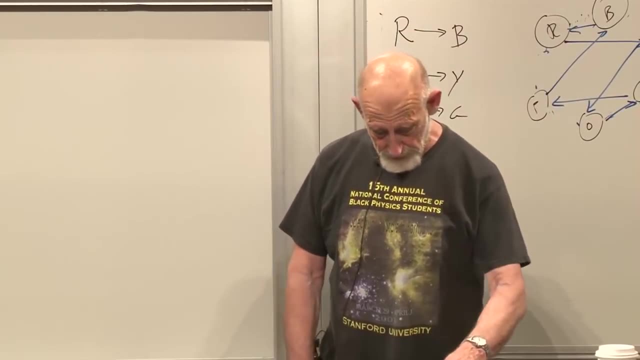 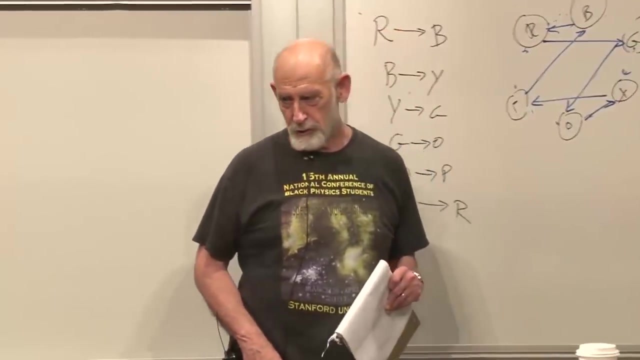 you all know what they are. they're laws that violate the conservation of information, the most primitive and basic rule of physics: the conservation of information. conservation of information is not a standard conservation law like this. it's the rule that you can keep track. you can keep track. 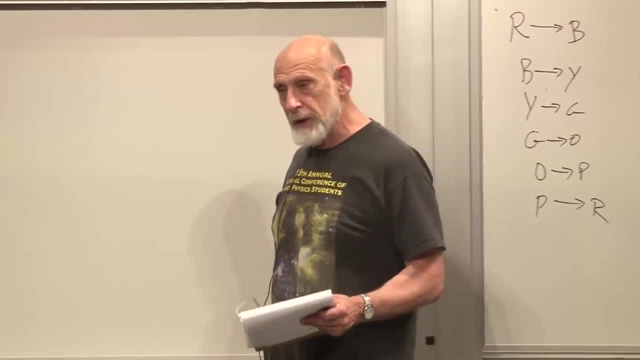 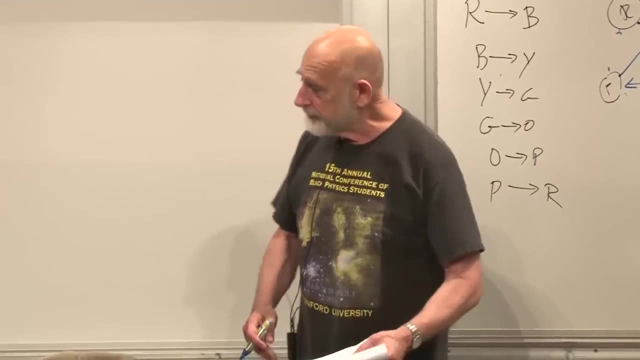 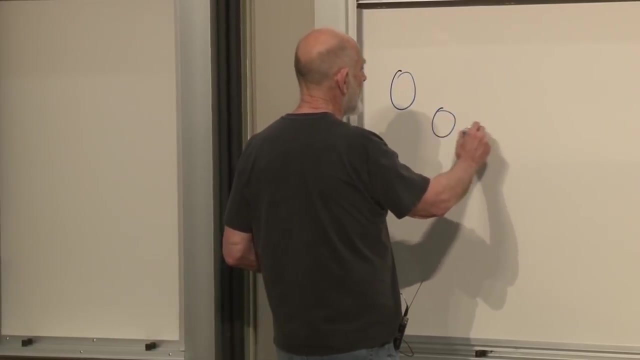 both going forward and backward. so let's just mention that again. it's all described in the classical mechanics book. I'm just reviewing it now. but let's take a bad law. it's a possible law. by bad I mean one, two, three, four. 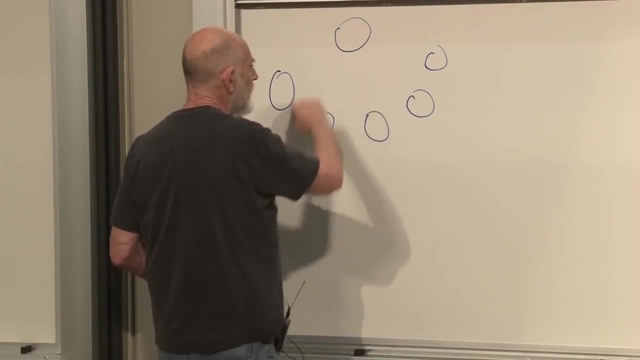 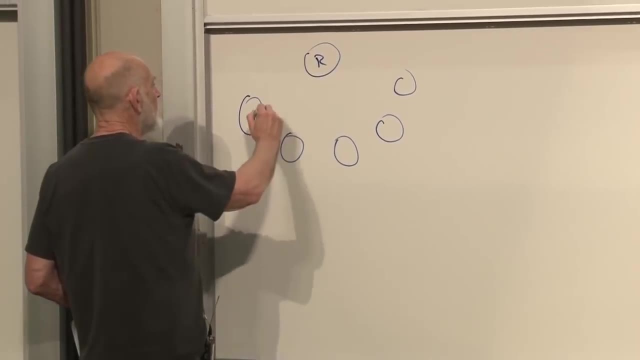 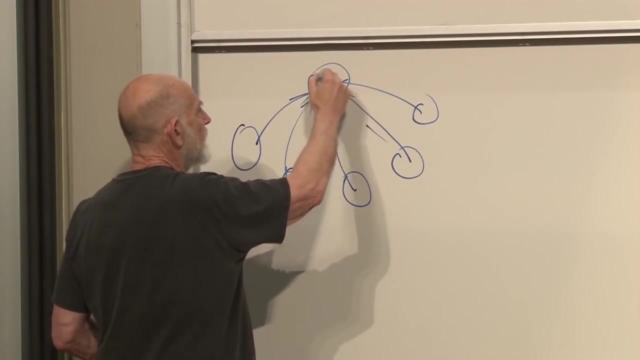 one, two, three, four, five, six. so these are the faces of a die again. but the rule is: wherever you are, this is red. wherever you are, you go to red. even if you are at red, you go to red. we'll discuss in a moment. 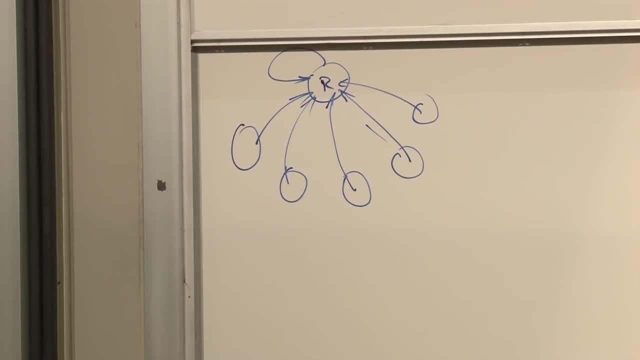 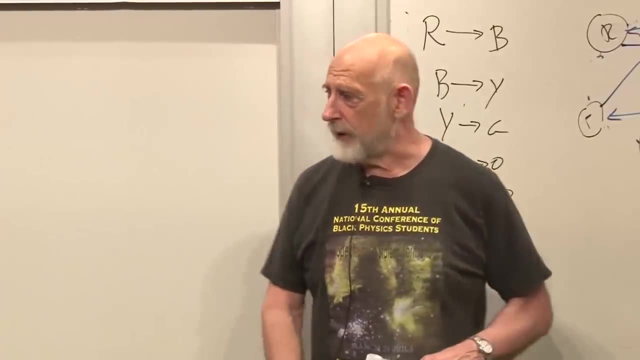 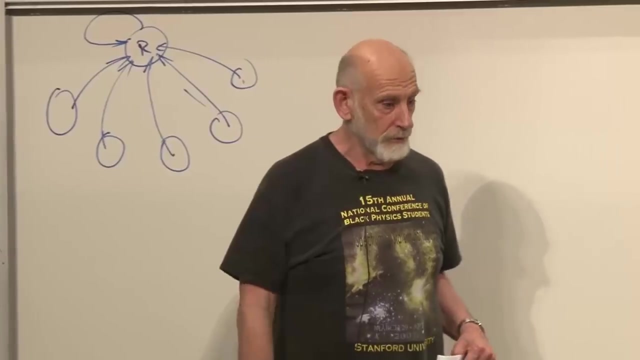 what's wrong with this law? but this law has. one of the features that it has is it's not reversible. it's not reversible in the sense that you can go from blue to red, but you cannot go from red back to blue. so in that sense it's not reversible. 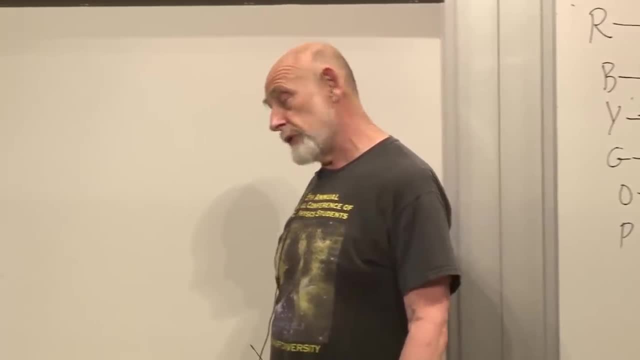 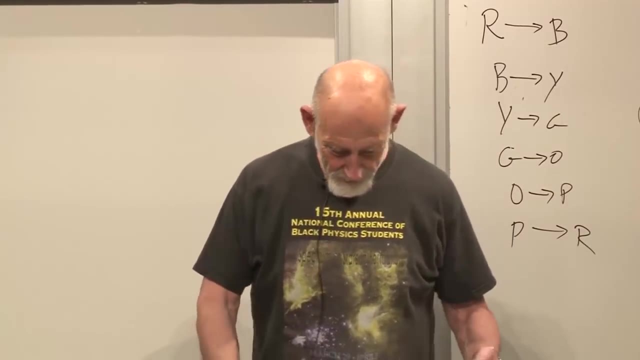 you can predict the future, wherever you are. the future is very simple for this particular law: wherever you are, you'll next be at red. you can make it more complicated. you could make a few. you can make it more complicated, but this law always winds up with red. 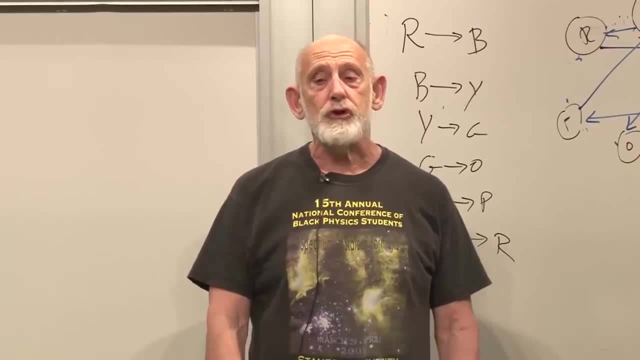 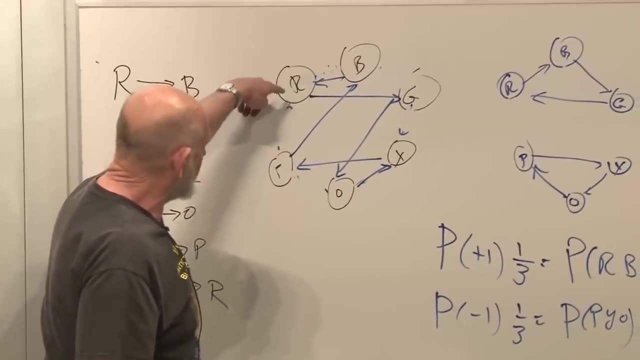 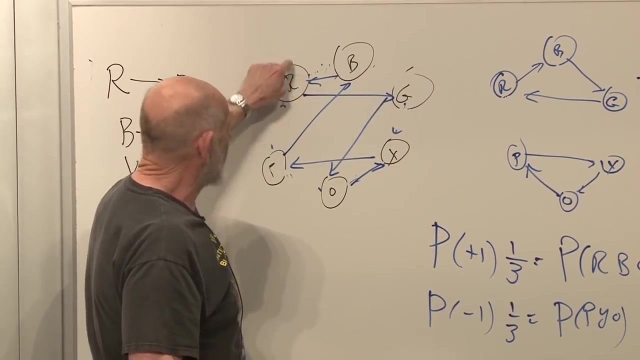 it's a bad law because it loses track of where you started, whereas these laws don't lose track. if you know that you've gone through 56, 56 and a half cycles, then you know that if you started at red, you'll come back and you can tell exactly where you'll be. 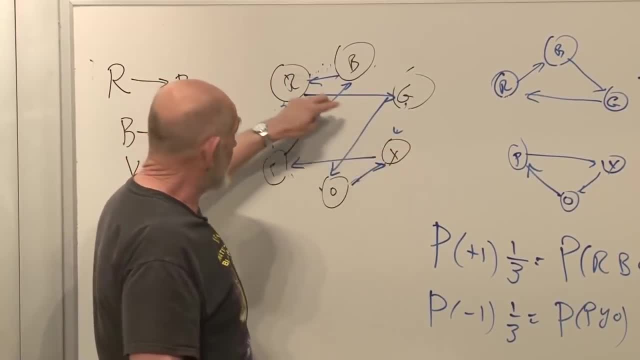 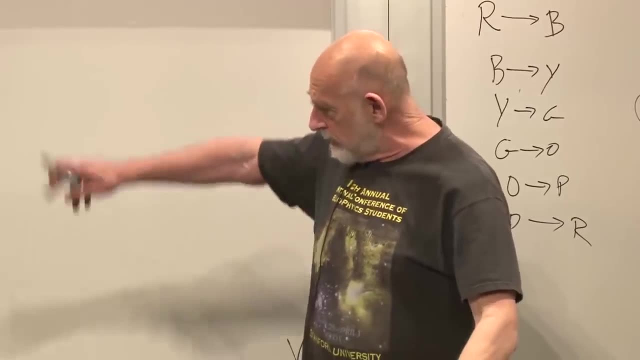 and you can also tell where you came from. you can tell not only where you'll be, but exactly where you came from. with this law, you can't say where you came from. this is a law that loses information, and it's exactly the kind of thing that classical physics does not allow. 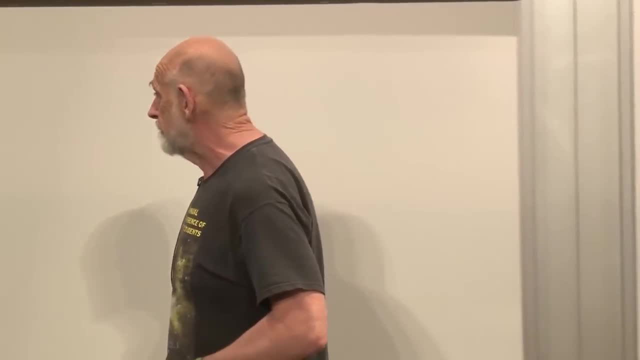 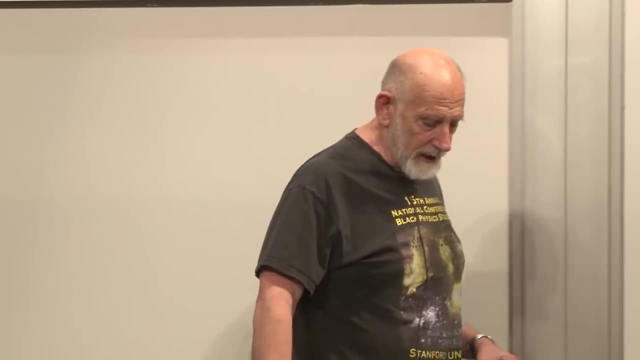 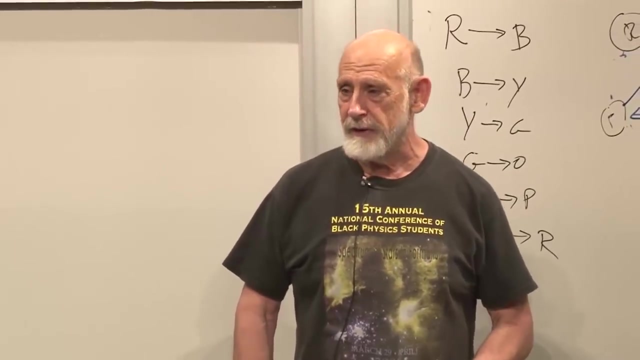 quantum physics also doesn't allow the quantum mechanical version of it, so the rule that this type of law is unallowed. I give a name to it. as I've said many times, there is no name for it. it's just so basically primitive that everybody always forgets about it. 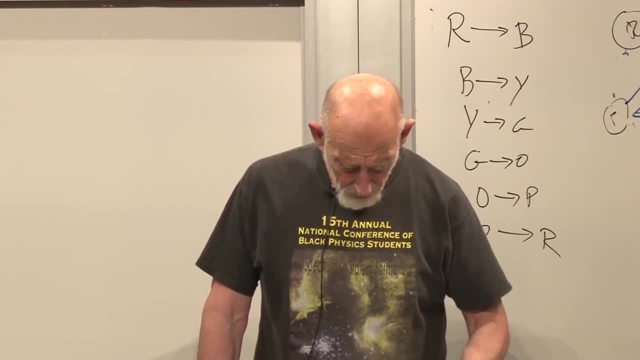 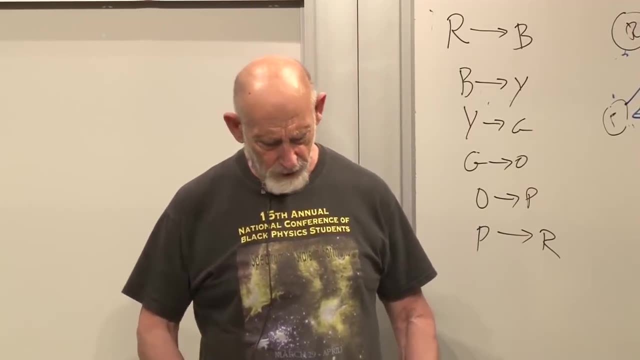 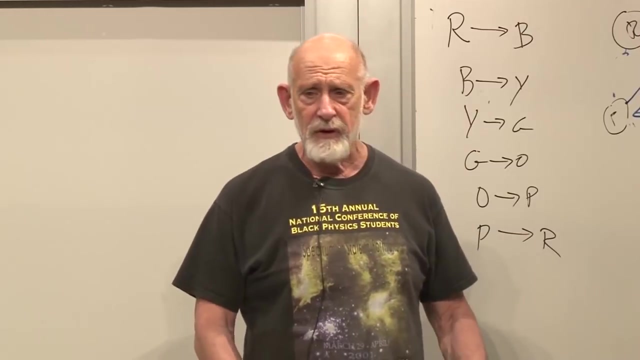 it's so basic I call it the minus first law of physics. I wish it would catch on. people should start using it. I mean, it is really the most basic law of physics that information is never lost, that distinctions or differences between states propagate with time and you never lose track. 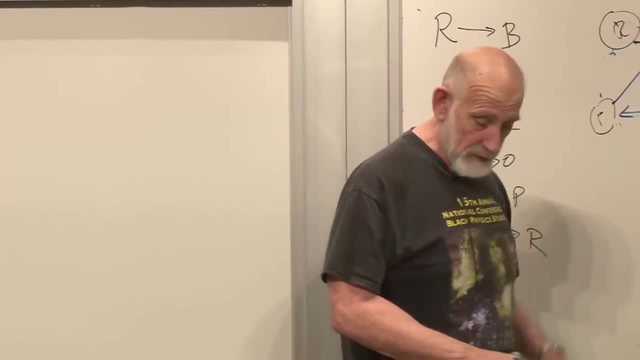 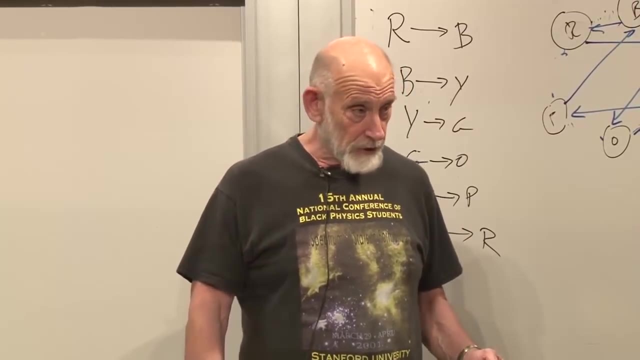 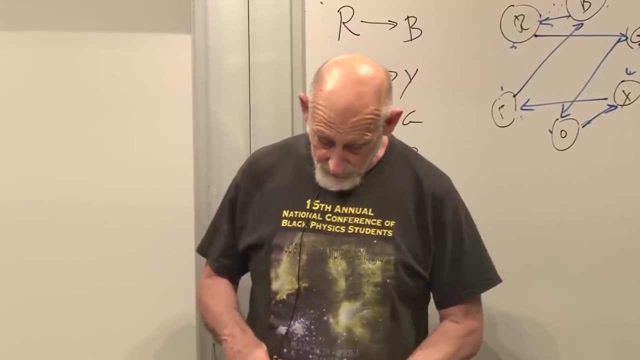 in principle, if you have the capacity to follow the system, because you may be too lazy to follow the system, that's your problem. but nature doesn't have that problem. nature allows, in principle, that you can reconstruct where you came from. alright, so that's a bad law. 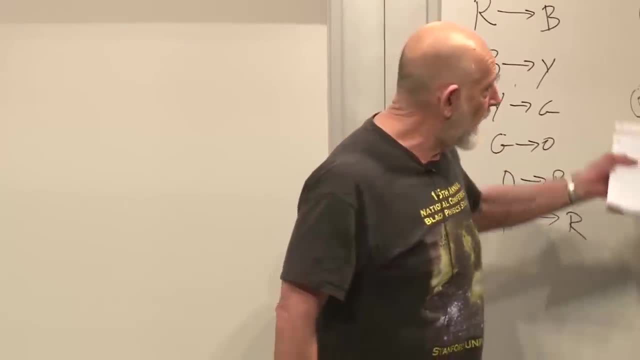 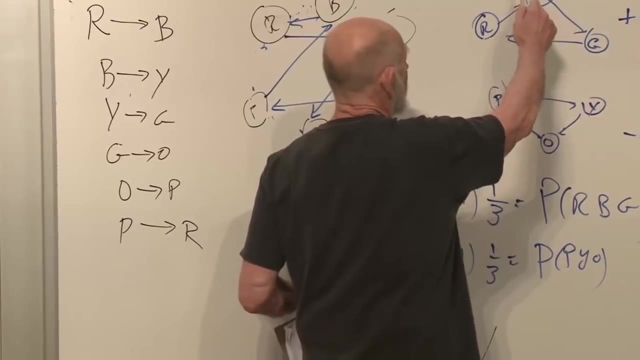 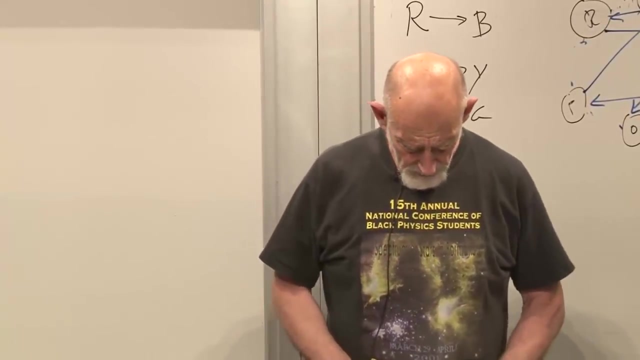 how do you tell the good laws from the bad laws? just by diagrammatics here. it's very simple. good laws: every state has one incoming arrow: an arrow to tell you where you came from and an arrow to tell you where you're going. ok, so that's. 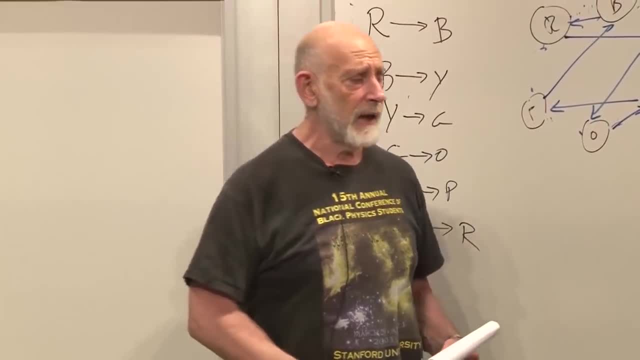 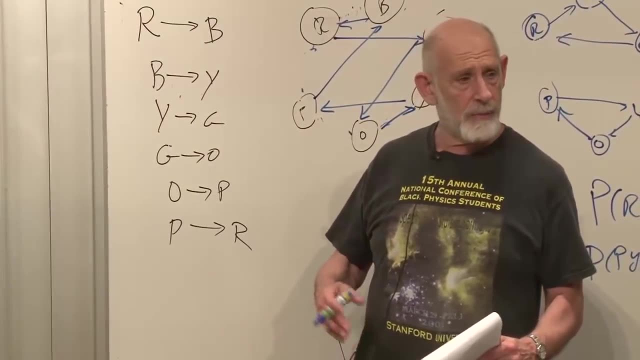 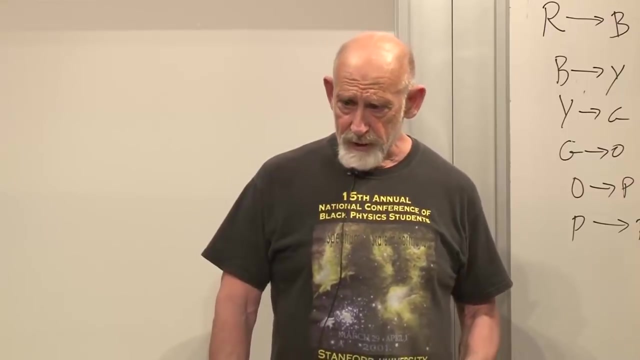 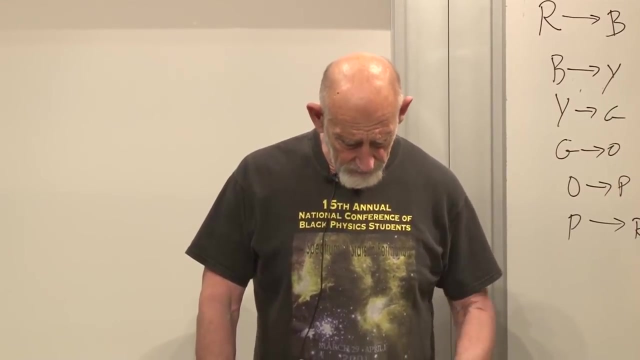 those are good laws. in classical mechanics, continuum classical mechanics, there is a version of this same law. anybody know the name of that version of the theorem that goes with the conservation of of information. it's called Leaville's theorem. we studied it in classical mechanics. but let me give you a counter example. 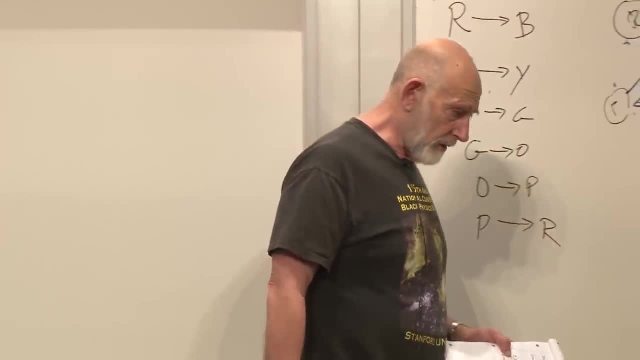 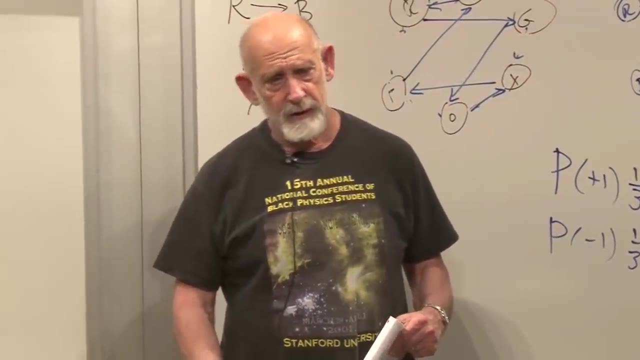 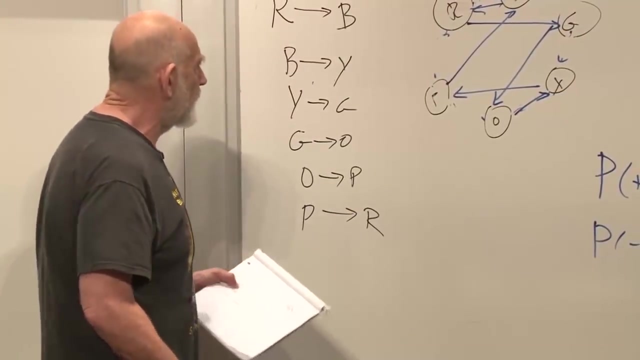 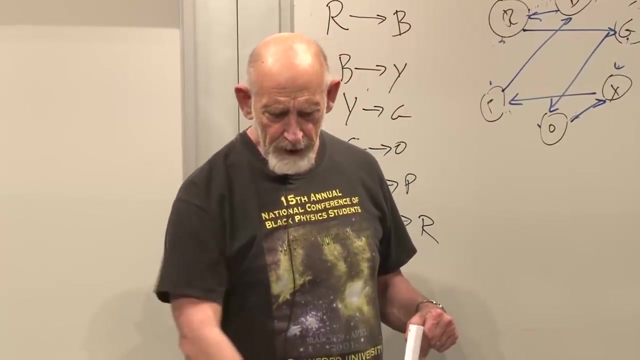 to Leaville's theorem. friction is an apparent contradiction. wherever you start, you come to rest. it's sort of like saying: wherever you start, you come to red, wherever you start, you come to rest. well, you may not know exactly where you are, but you always come to rest. 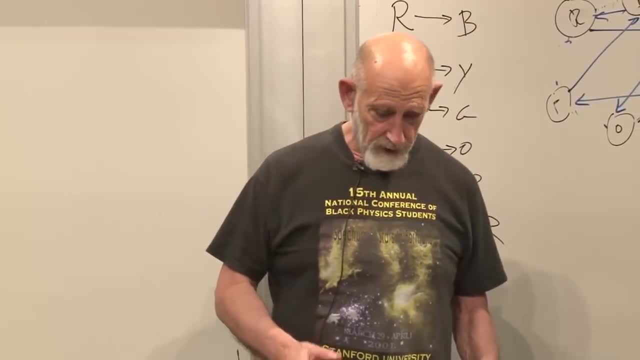 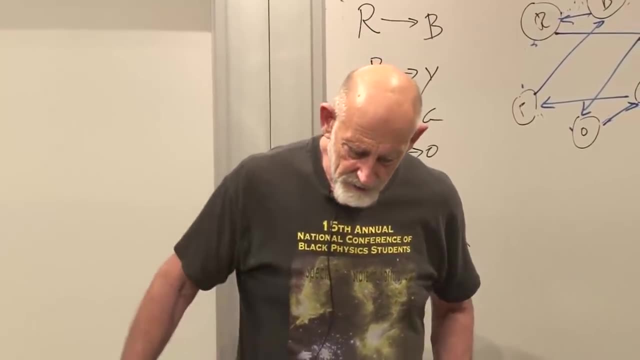 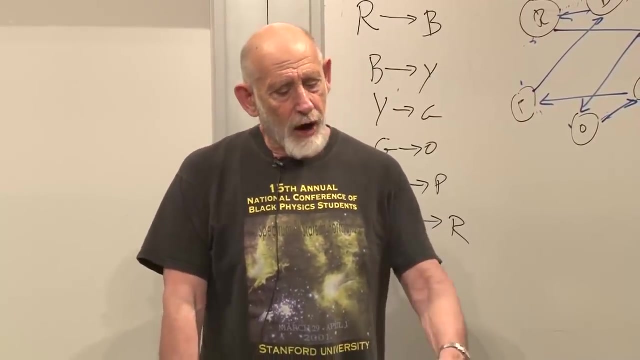 it's a violation of the laws that tell you that distinctions have to be preserved, but of course, it's not really true. what's really going on is that when you run the eraser through here, it's heating up the surface here, and if you could keep track of. 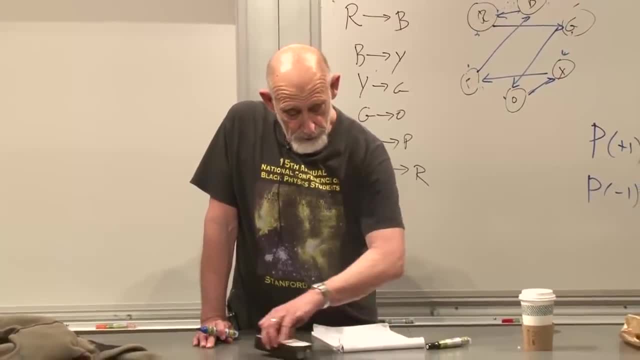 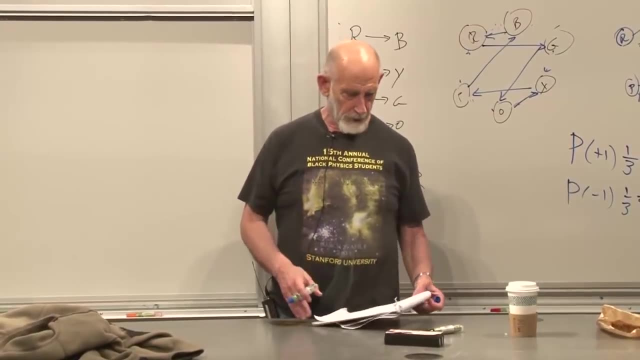 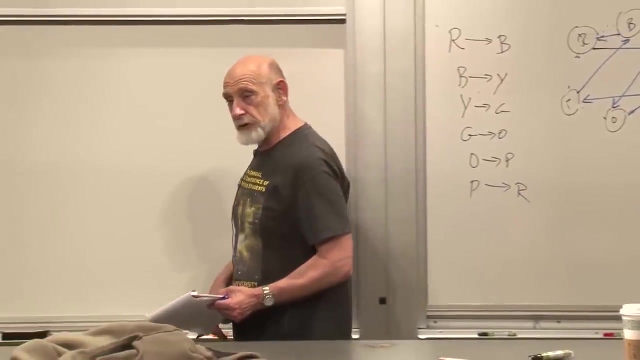 every molecule, you would find out that the distinctions between starting points is recorded. but let's imagine now that there was a fundamental law of physics. by a fundamental law I mean, you know, a rock bottom fundamental law for a series of particles, for a collection of particles and the equations of motion. 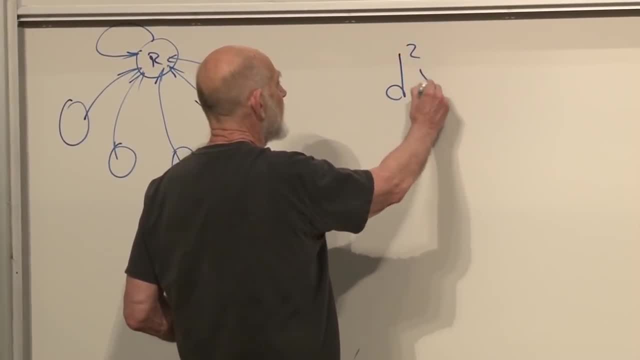 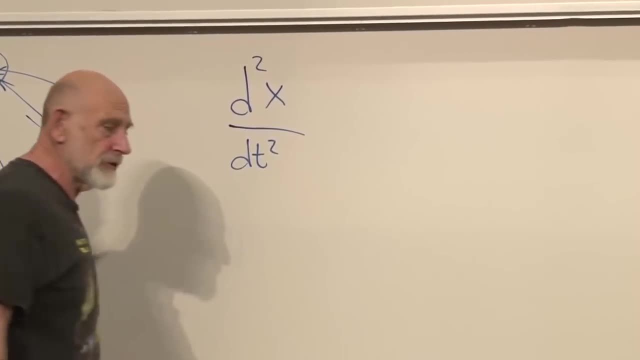 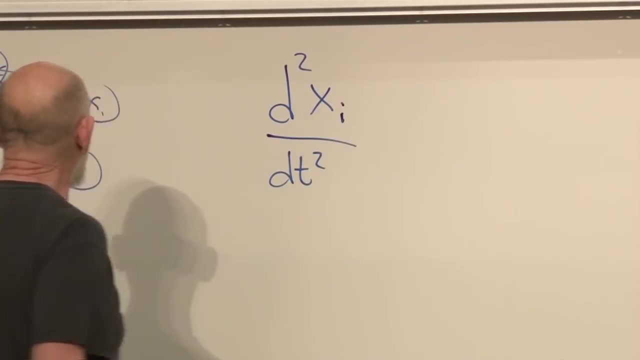 for the particles were this: d second x, that's the position of the particle, somewhere by dt, squared. that's called acceleration. we could put a mass in, but the mass is not doing anything. there's a lot of particles, so I'll label them I. we've used i to label states. 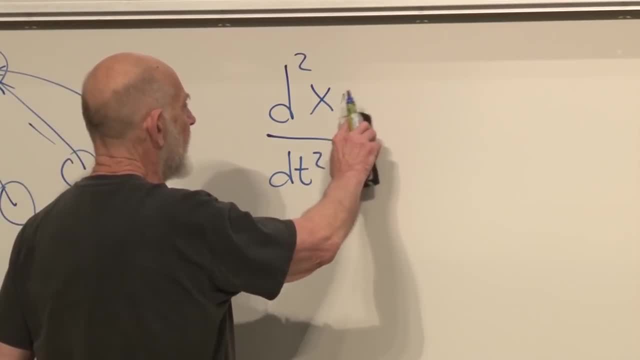 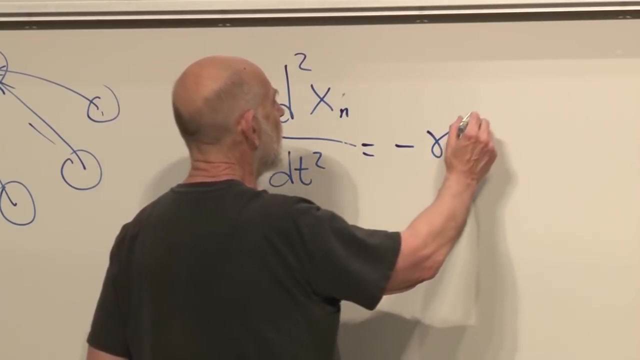 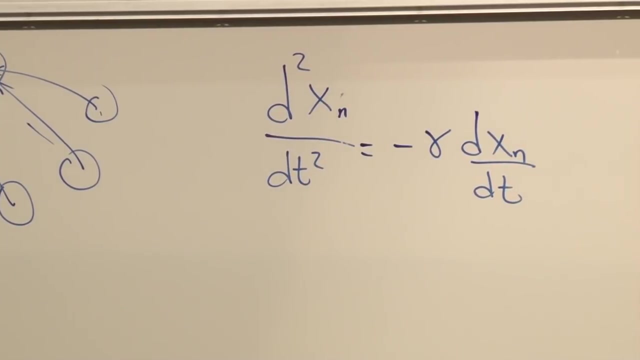 I should not do that. let's call it n little n, the nth particle. and what is that equal to? it's equal to minus some number, gamma. we've seen that number before in another context. times dxn by dt. anybody remember what this formula represents? friction, viscous drag. 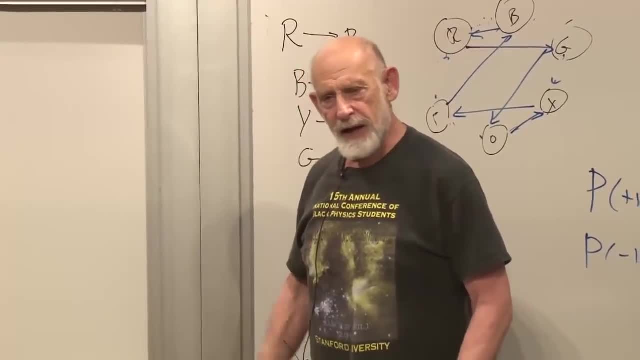 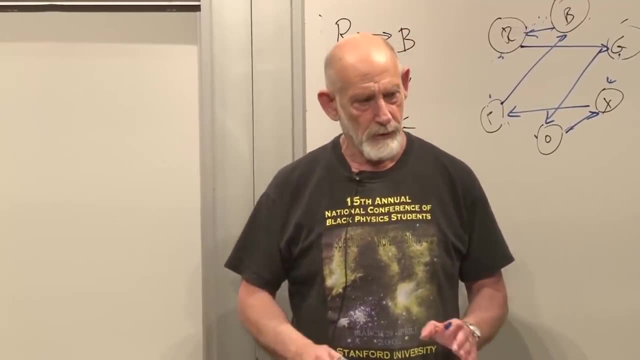 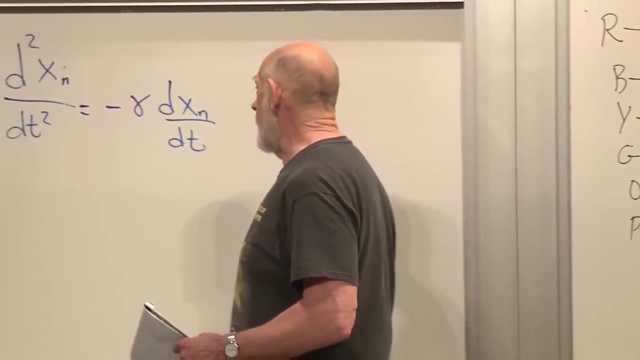 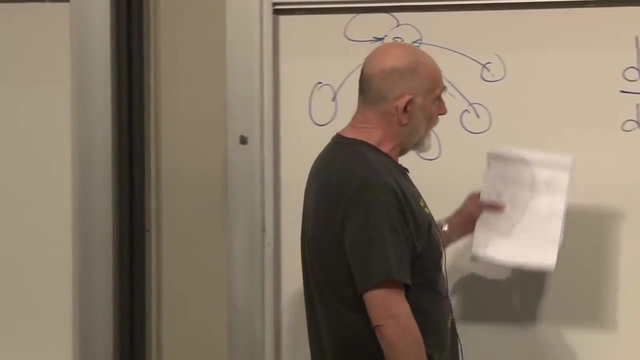 again. it has the property that if you start with a moving particle it will very quickly come almost to rest. it will exponentially come to rest pretty quickly, and so if all particles in a gas, for example, satisfied this law of physics, it's perfectly deterministic. it tells you what happens. 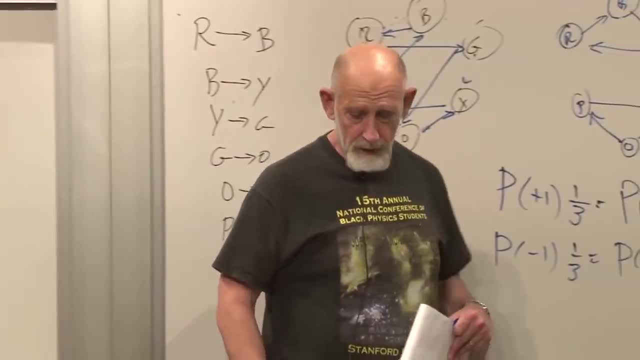 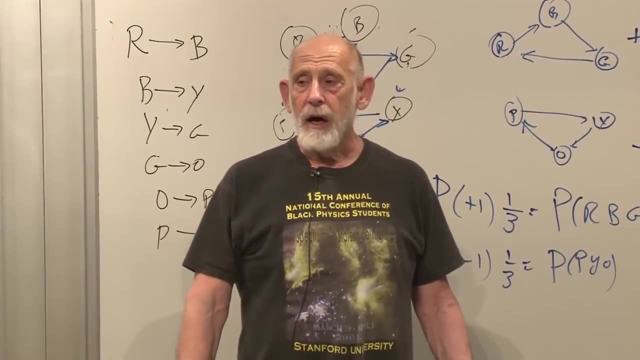 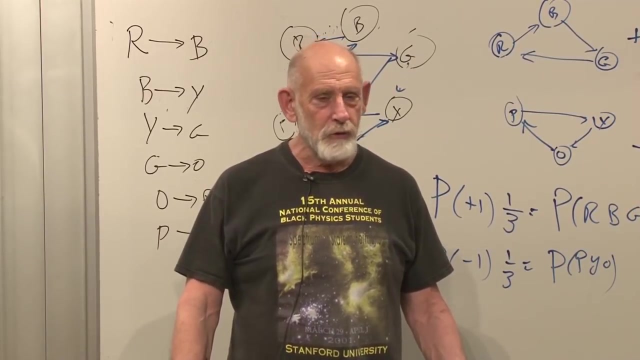 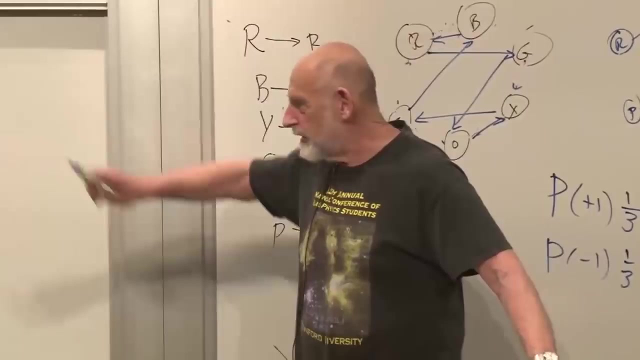 next, but it has the unfortunate consequence that every particle just comes to rest. um, that sounds odd. it sounds like no matter what temperature you start the room, it will quickly come to zero temperature. that doesn't happen. this is a perfectly good differential equation, but there's something wrong with it. 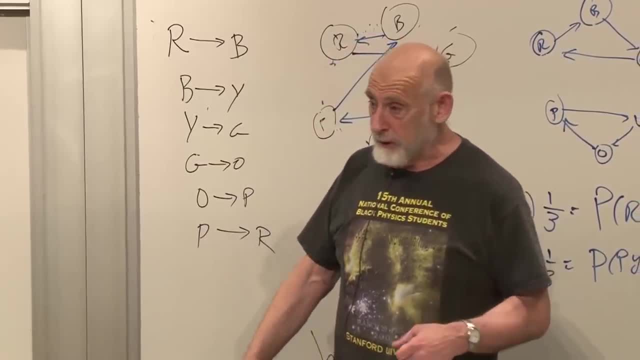 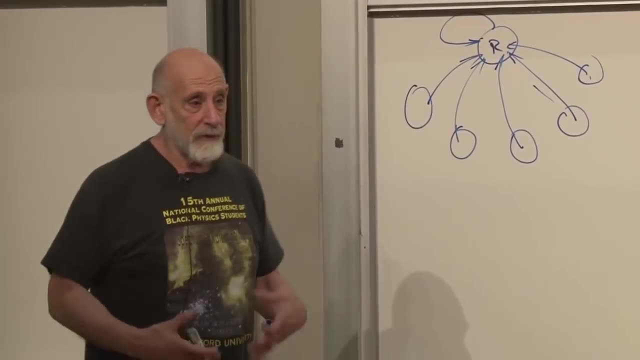 from the point of view of conservation of energy. there's something wrong with it from the point of view of thermodynamics. if you start a closed system and you start it running, you start with a lot of kinetic energy- temperature we usually call it. it doesn't run to zero temperature. 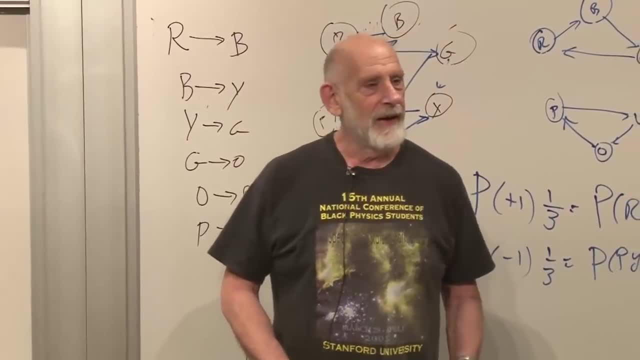 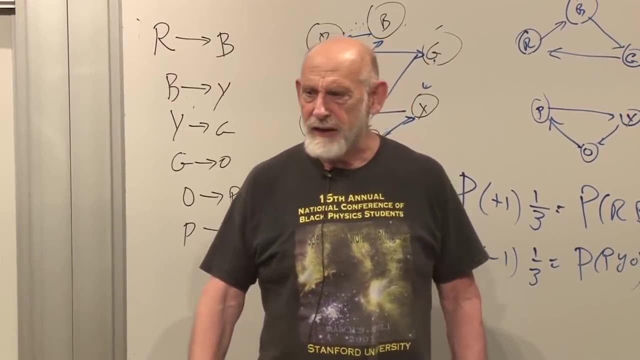 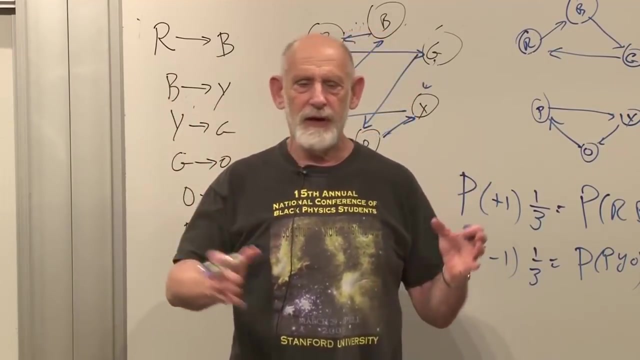 that's not what happens in fact. um, this is not only a violation of energy conservation. it looks like a violation of the second law of thermodynamics. it says things get simpler. you start with a random bunch of particles moving in random directions and you let it run. 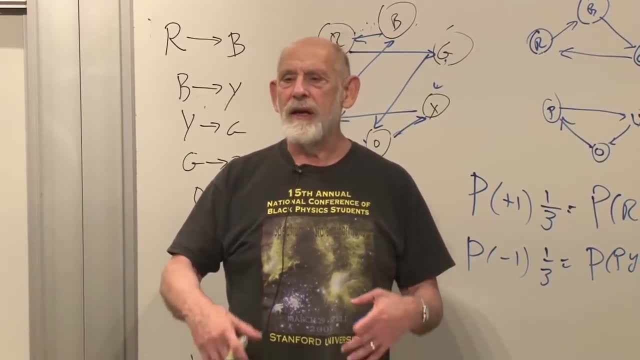 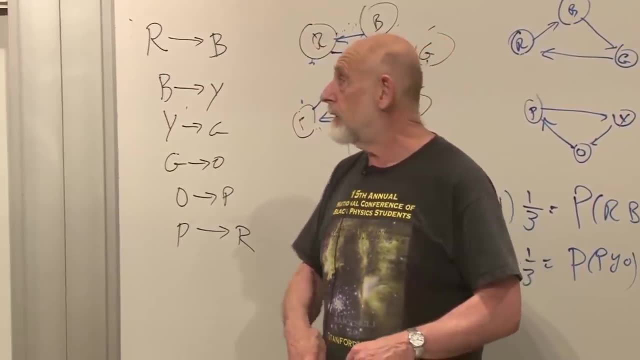 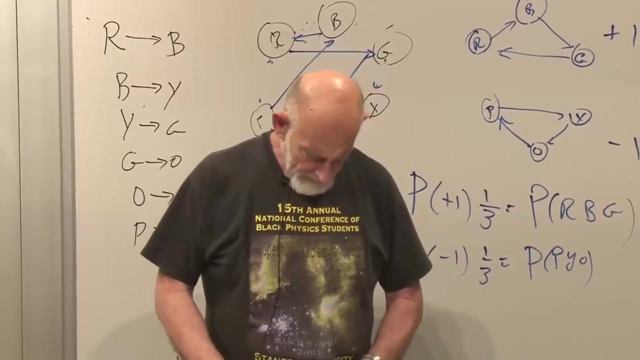 and they all come to rest. what you end up with is simpler and requires less information to describe than what you started with. that's very, very much like um, everything going to red and, among other things, it violates the second law of thermodynamics, which generally says things get worse. 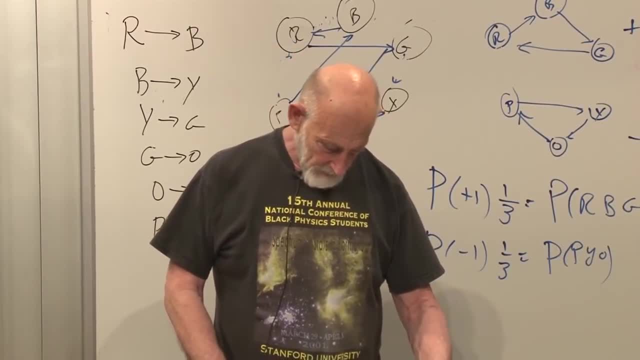 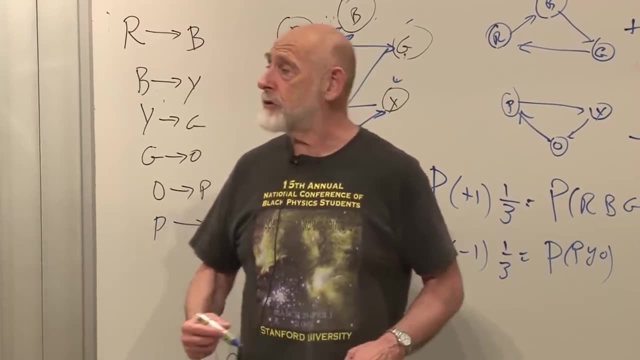 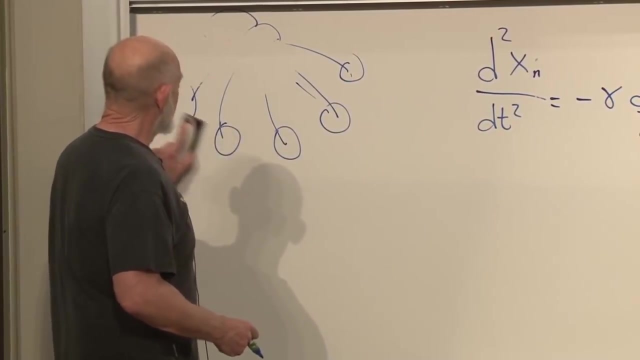 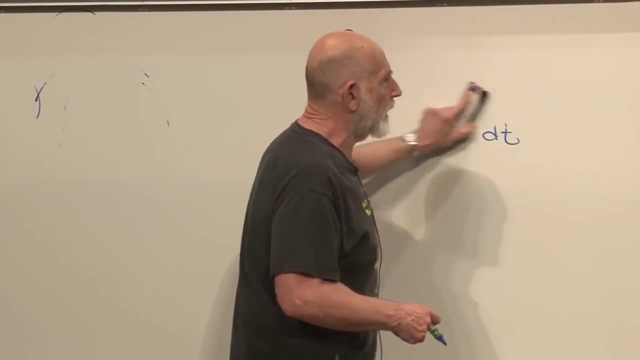 things get more complicated, not less complicated. that's um alright. now there's another way to say, another important way to say, this rule: that every state has to have one arrow in and one arrow out, the thing that I called either the minus first law or the conservation of information. 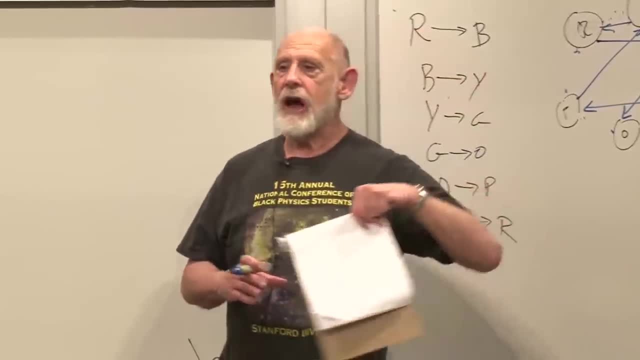 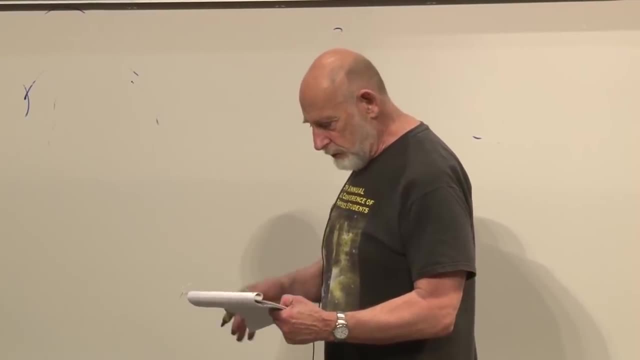 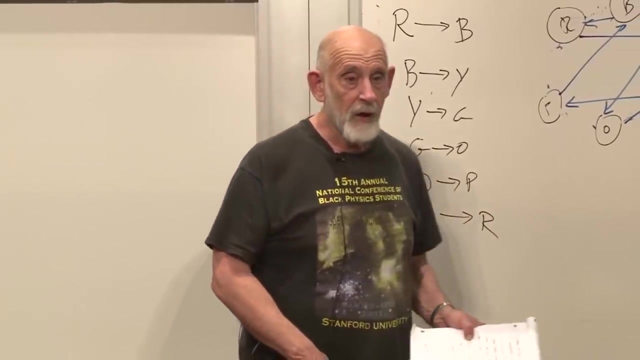 supposing we have a collection of states and we assign to them probabilities, probabilities- p of state one, p of state two, p of state three and so forth, for some subset of the states, not all of them, some subset of them. all the others we say have probability zero. 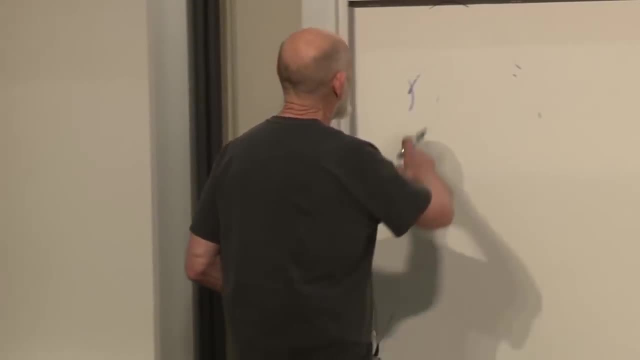 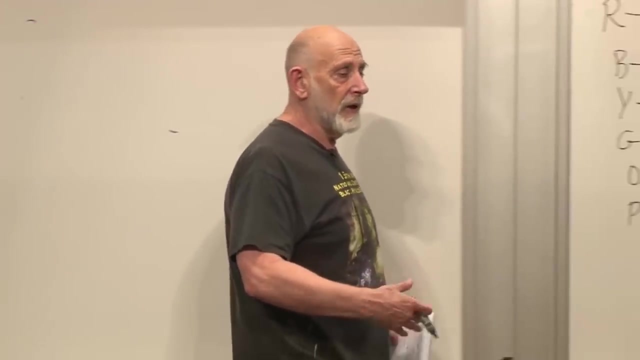 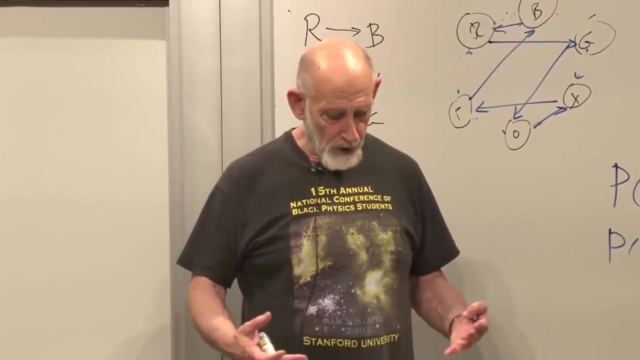 so, for example, um, we can take our die and assign red, yellow and blue probability, a third, and green, orange and pink or whatever it was. where we got that from doesn't matter, we got it from somewheres. somebody secretly told us in our ear: it's either red, yellow or blue. 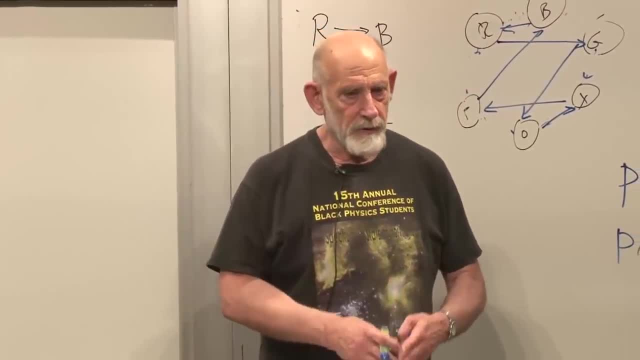 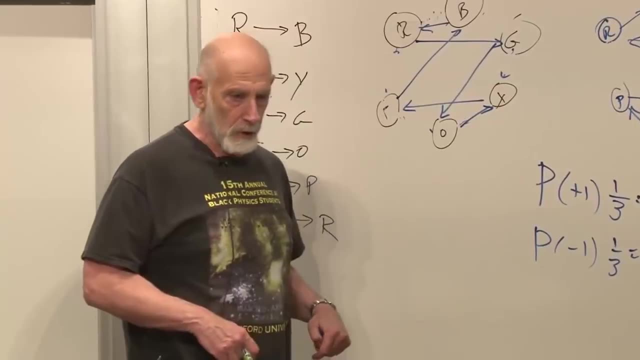 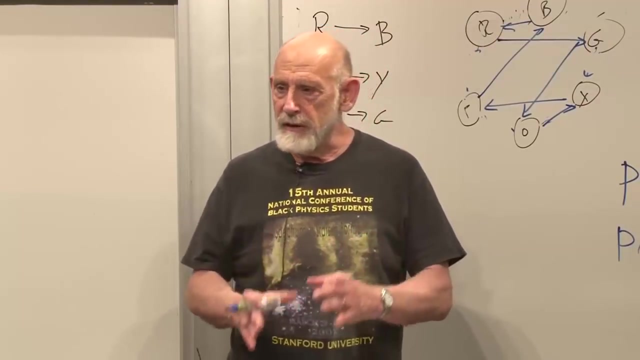 and I'm not going to tell you which. and now you follow the system. you follow it as it evolves. whatever kind of law of physics, as long as it's an allowable law of physics after a while, and you're following it in detail, you're not constrained by 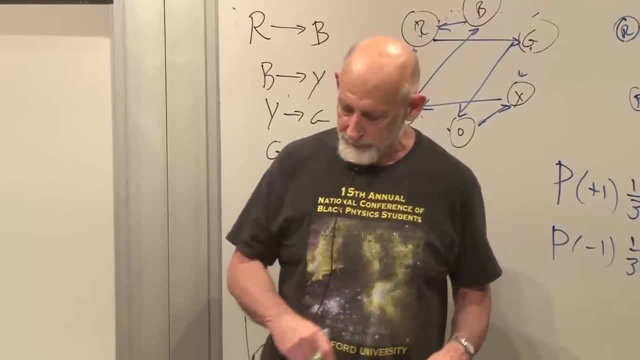 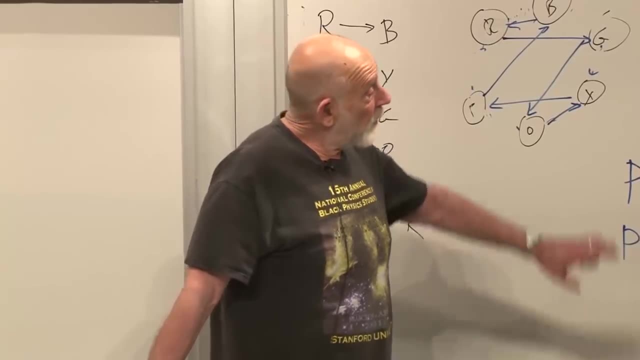 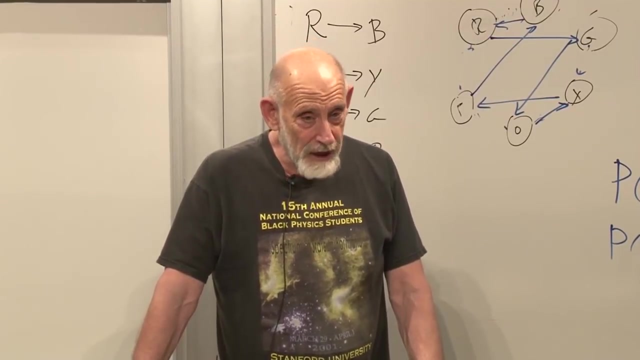 your laziness, in this case, you are capable of following in detail. then what is the probability? what are the probabilities at a later time? well, if you don't know which the laws of physics are, you can't say, of course, but you can say one thing. you can say there are three states. 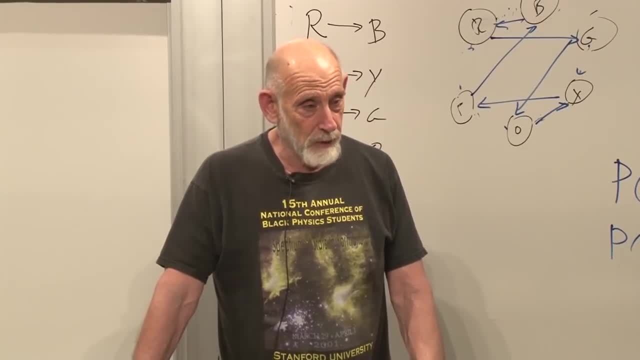 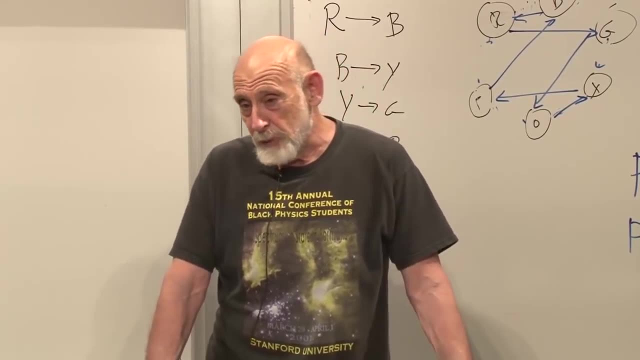 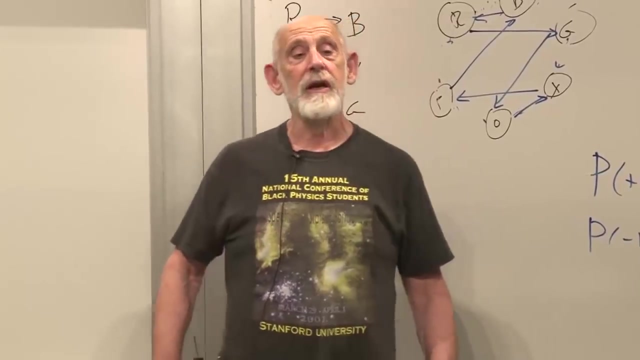 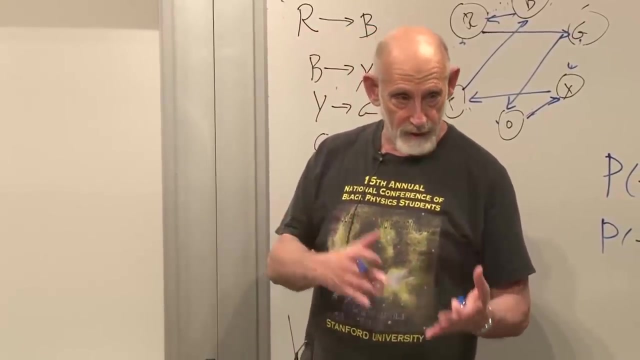 with probability one third and three states with probability zero. they may get reshuffled, which ones were probable and which ones were improbable, but after a certain time there will be those same, not the same three states, but there will continue to be three states which have probability and the rest don't. 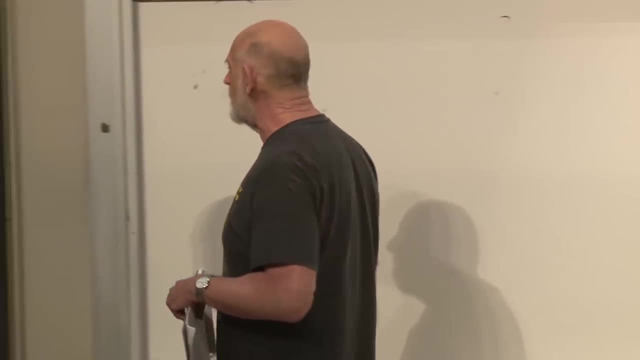 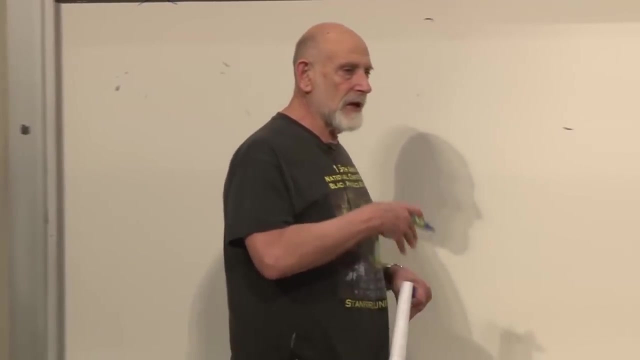 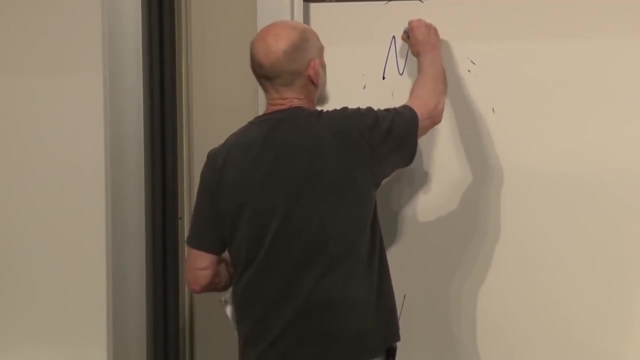 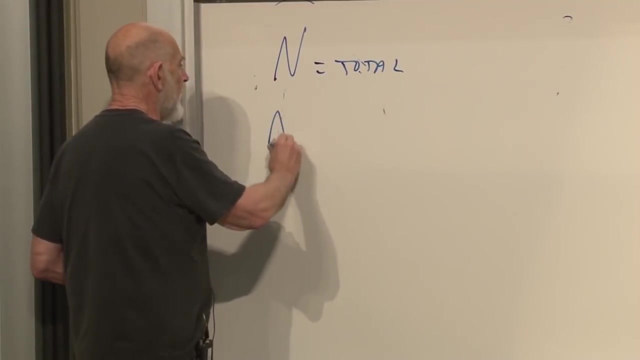 so in general, you could characterize these information conserving theories by saying: supposing you assign some subset of the states, let's say m out of n states. let's say there are n states all together, that's the total number of states. and now we look at some m. 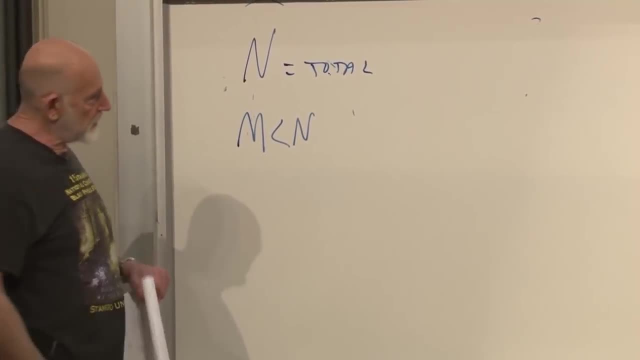 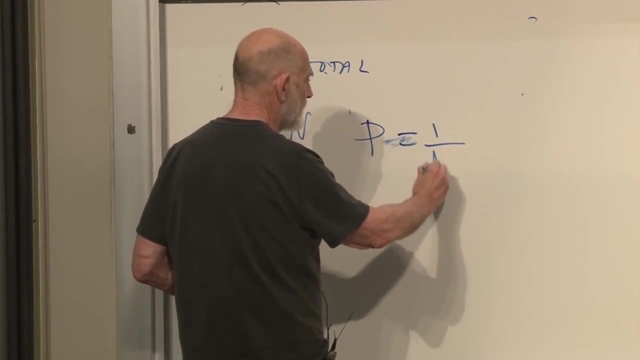 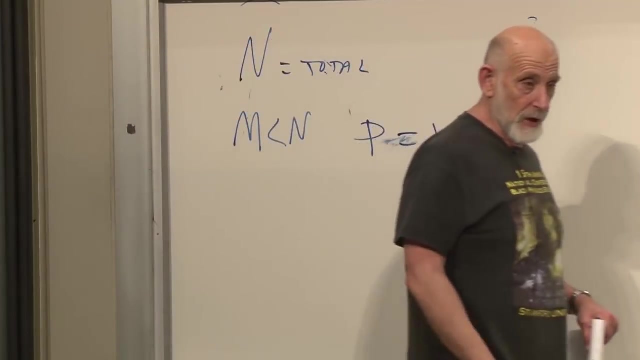 where m is less than n and we say for those m states, the probability for those m states is one over m for these states and zero for all the others. you understand why I say one over m. if there are m states equally probable, then each one has probability one over m. 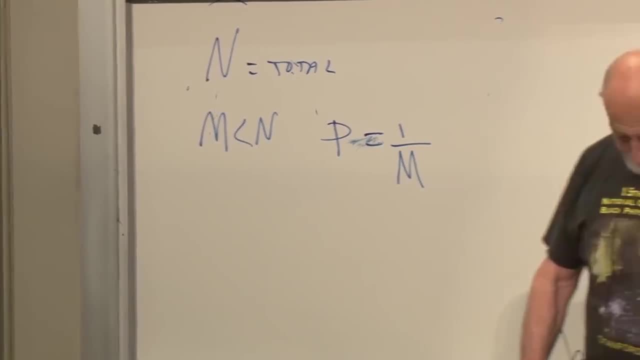 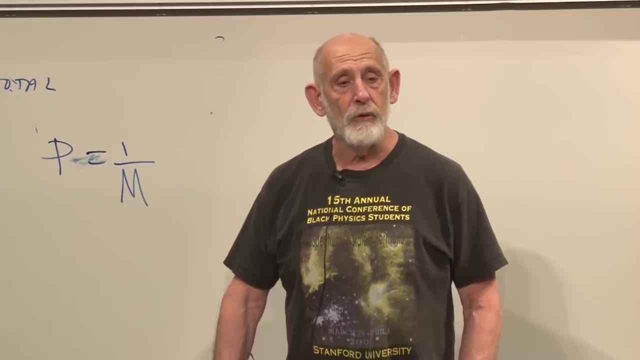 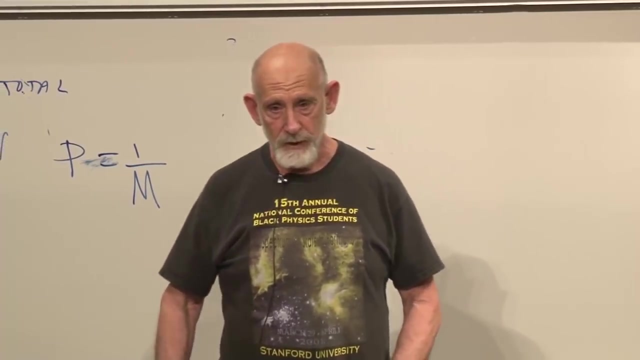 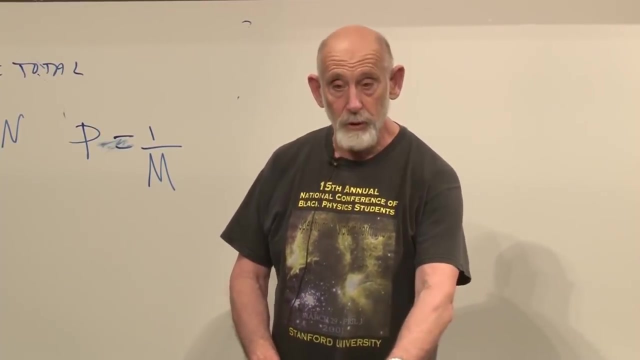 and all the remaining have probability zero, then the number of states which have non-zero probability will remain constant and the probabilities will remain equal to one over m. is that clear? is that obvious? that should be obvious. the states may reshuffle, but that the number with non-zero probability 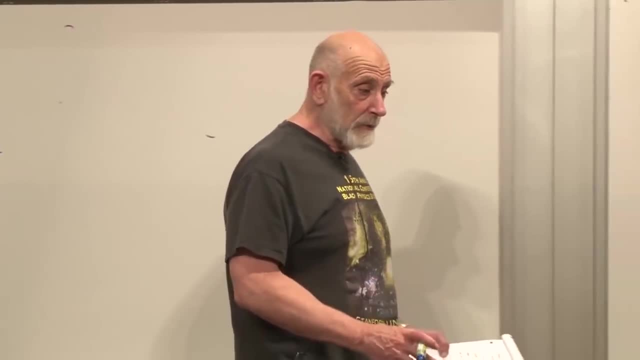 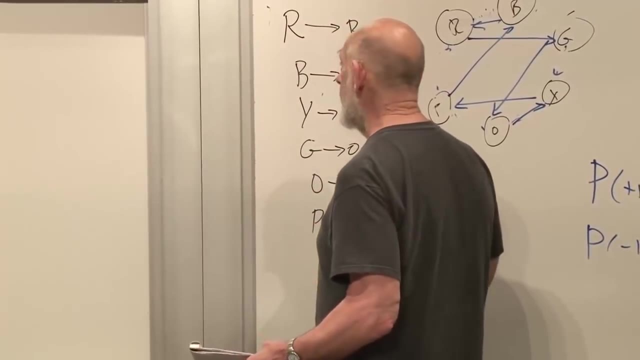 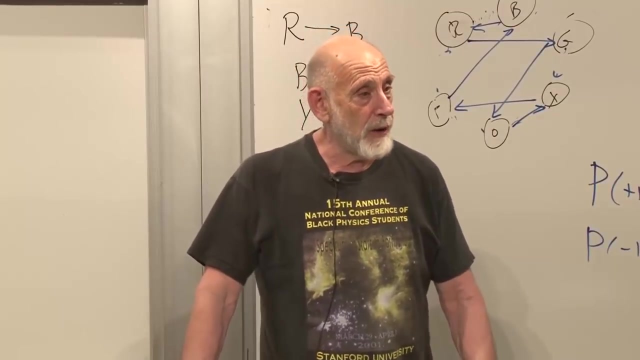 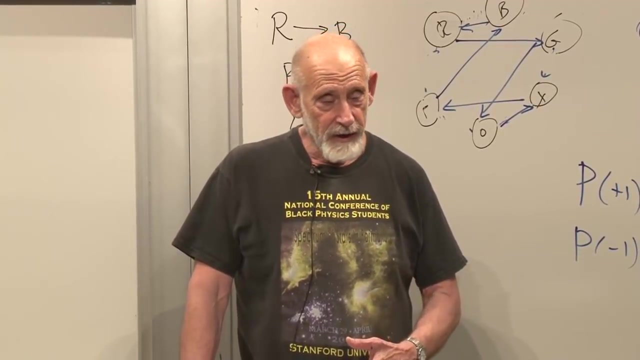 will remain fixed. that's a characterization, a different characterization of the information conserving laws for the information non-conserving laws. everybody goes to red. you may start with a probability distribution, that's one over five for red, green, purple, orange and yellow, and then a little bit. 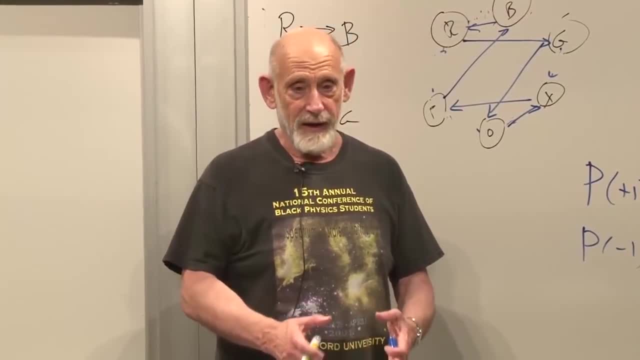 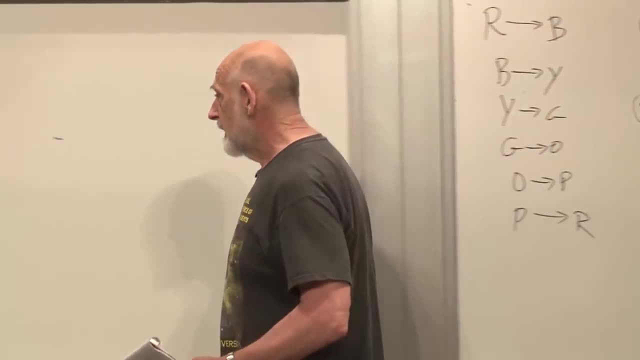 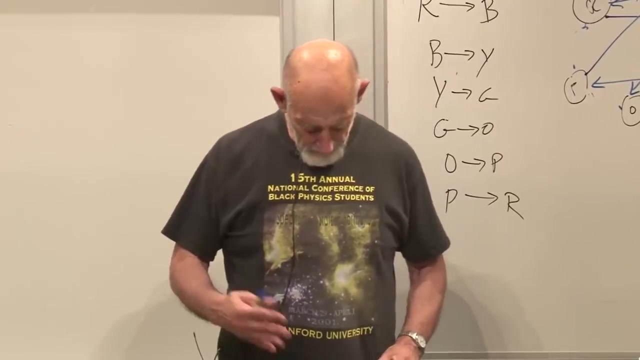 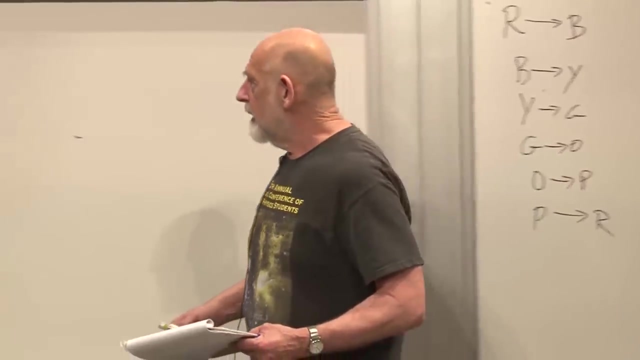 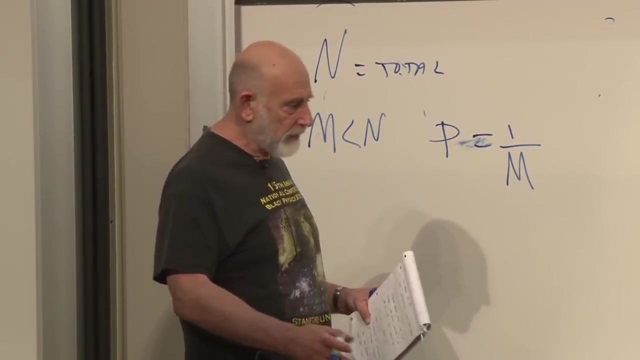 later, there's only one state that has a probability and that's red. okay, so that's- this is another way to describe information conservation- and we can quantify that. we can quantify that by saying: let m be the number of states which all have equal, under the assumption that they all have equal probability. 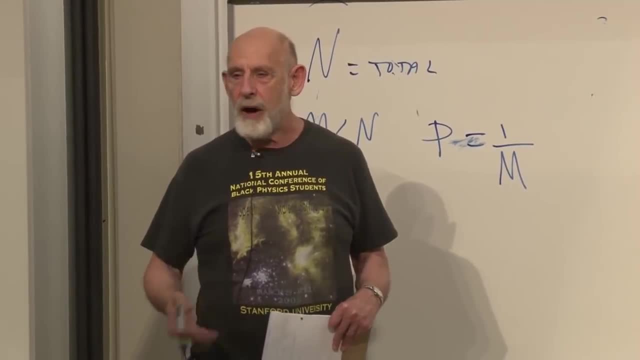 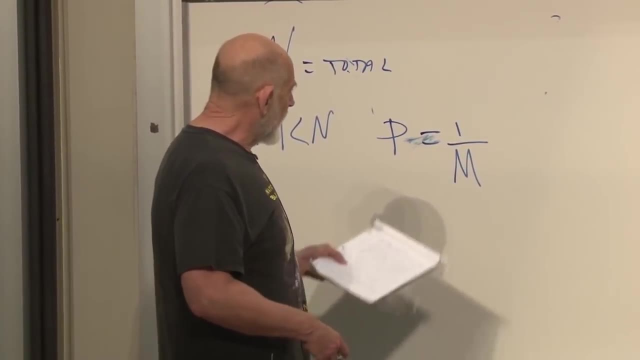 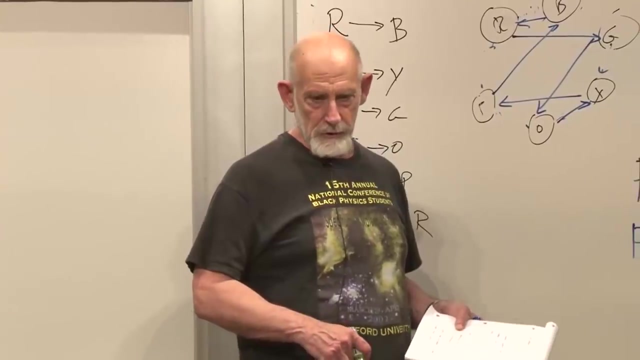 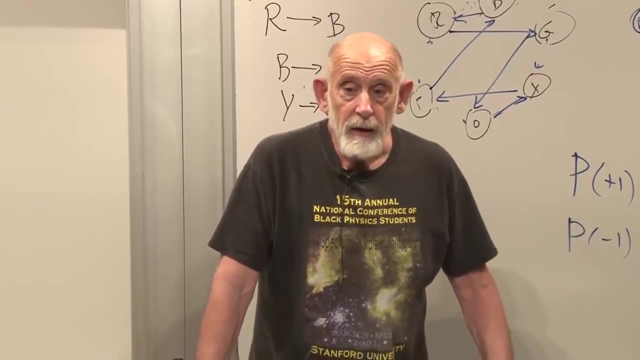 let m be the number, let's give it a name: occupied states, non-zero probability with equal probability. and then m. what is m characterizing? m is characterizing your ignorance. the bigger m is. if m is equal to n, that means equal probability for everything. maximal ignorance. 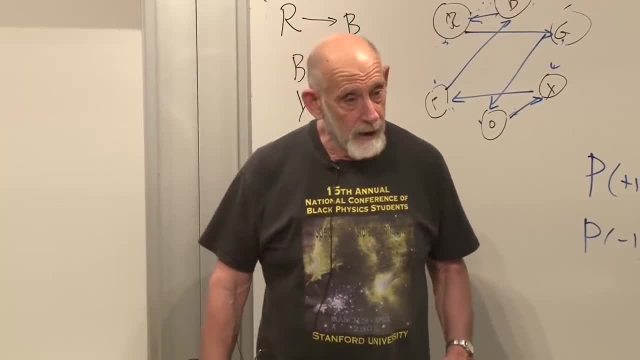 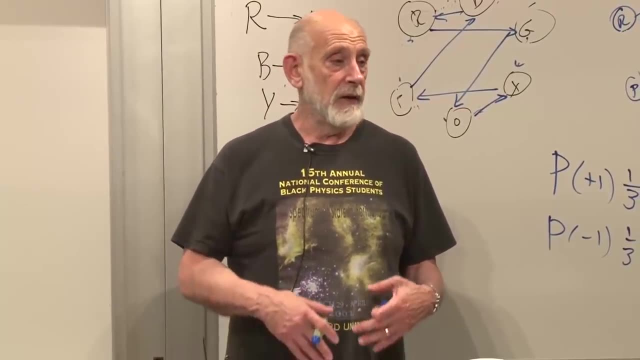 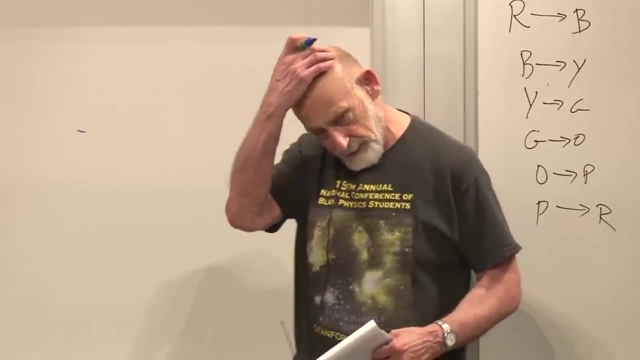 if m is equal to one half n, that means you know that the system is in one out of half the states. you're still pretty ignorant, but you're not that ignorant, you're less ignorant. what's the maximum? what's the minimum amount of ignorance you can have? 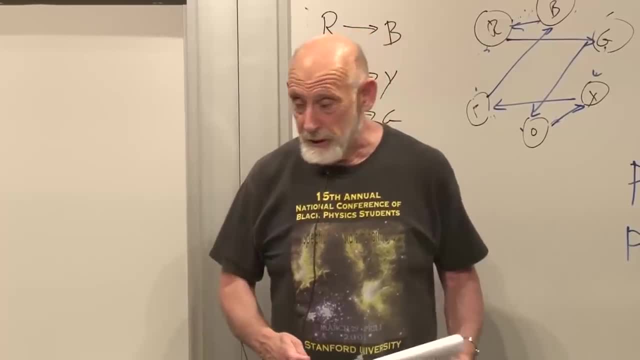 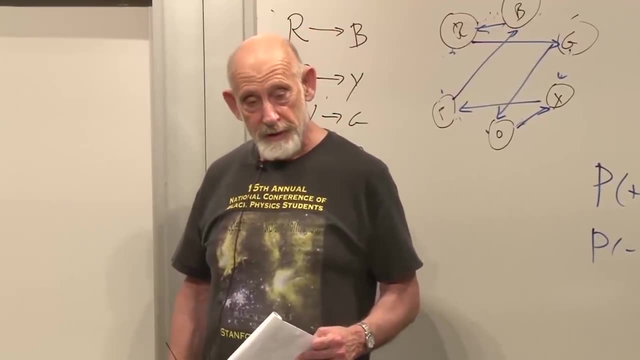 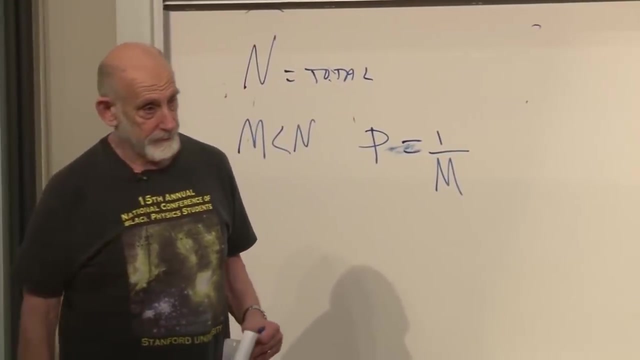 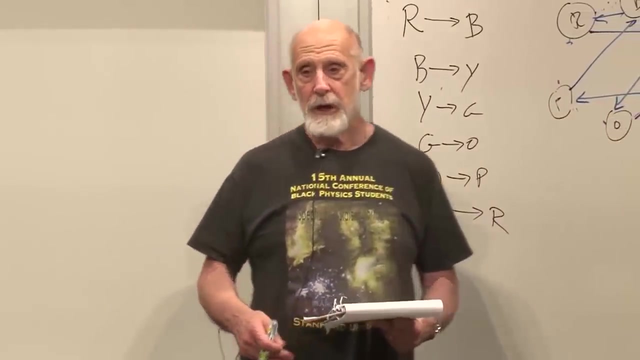 that you know precisely what state it's, in in which case m is what m is, one you know that it's in one particular state. okay, alright, so m is a measure of your ignorance. really, m in relation to n is a measure of your ignorance and associated with it. 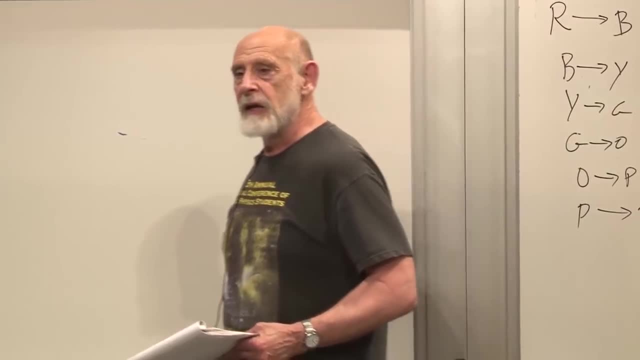 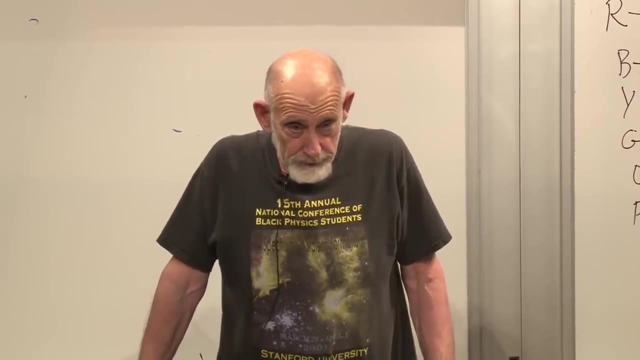 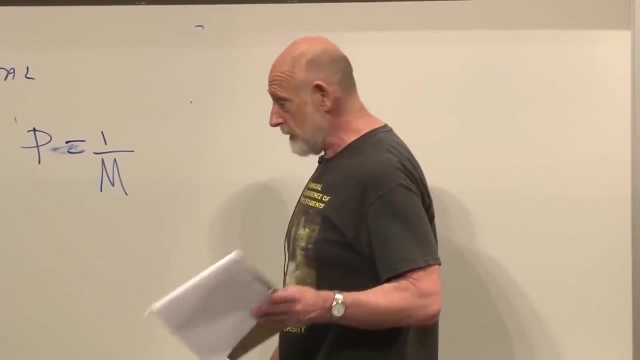 is the concept of entropy. we come to the concept of entropy. notice: entropy is coming before anything else. entropy is coming before temperature. it's even coming before energy. entropy is more fundamental, in a certain sense, than any of them, although in a certain sense, we'll discuss entropy in a minute. 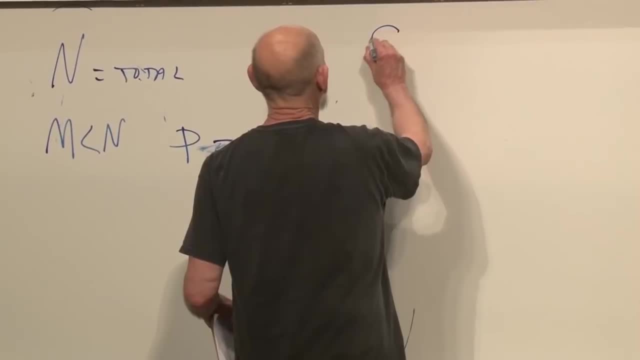 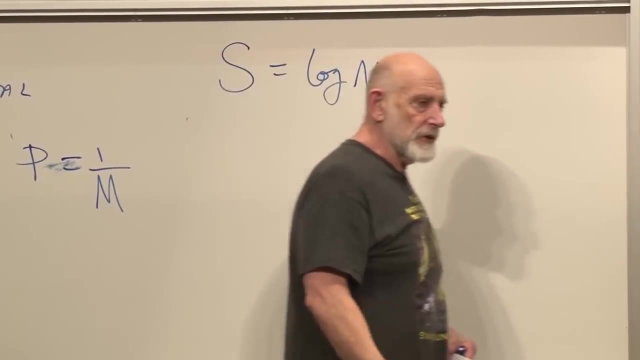 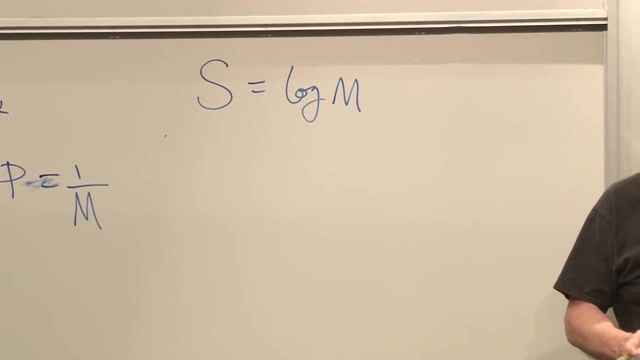 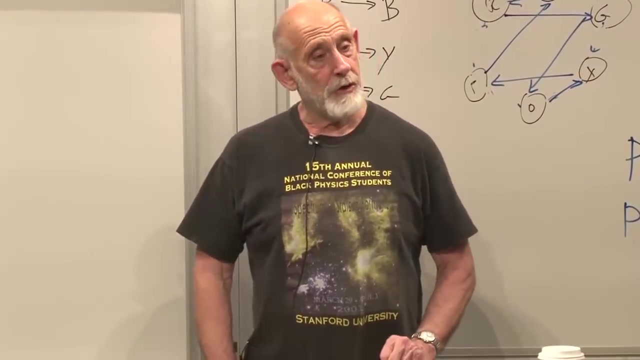 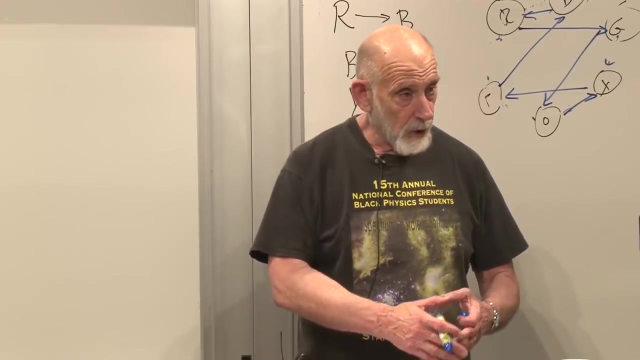 but s is a logarithm of m, logarithm of the number of states that have an appreciable probability, more or less all equal for the specific circumstance that I talked about, that entropy is conserved. all that happens is the states which are occupied reshuffle, but there will always be. 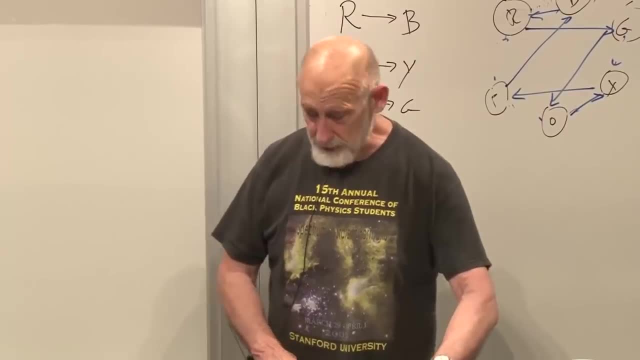 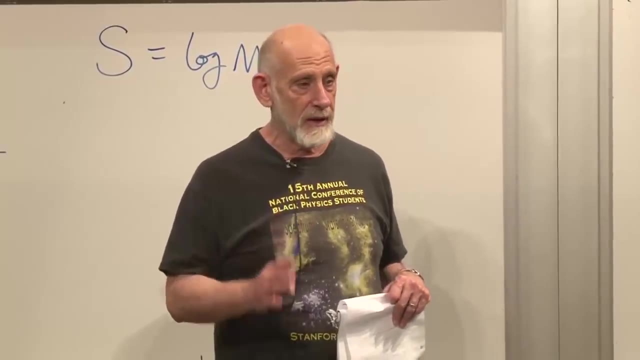 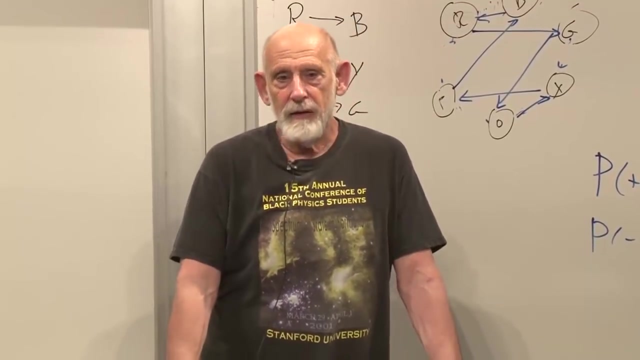 m of them, with probability one over m. okay, so that's where we are and that's the conservation of entropy, if we can follow the system in detail. now, of course, in reality we may be again lazy, lose track of the system and we might have after a point. 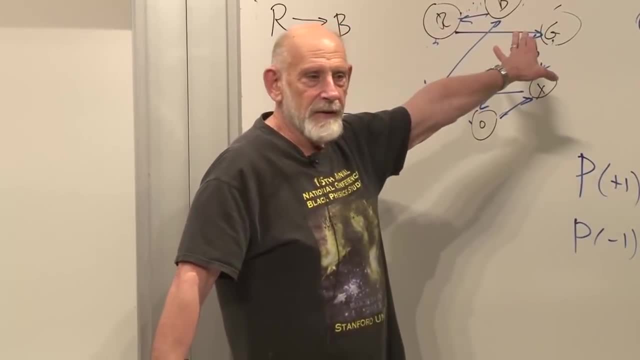 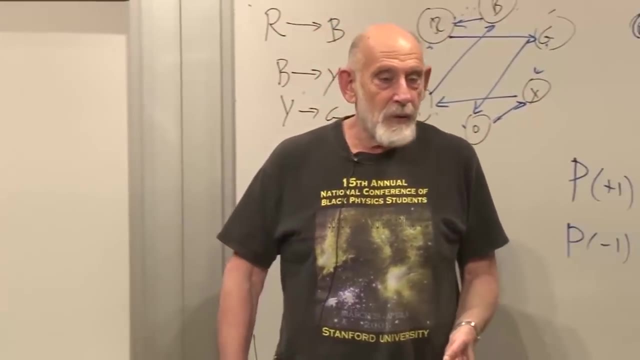 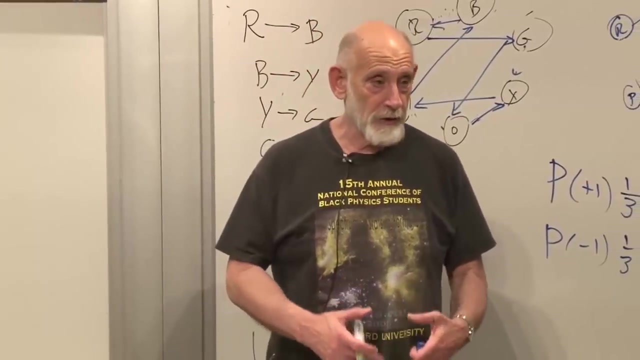 lost track of the event, of the equations, and lost track of our timing device and so forth and so on, and we may wind up. we may have started with some a lot of knowledge and wound up with very little knowledge. that's because, again, not because the equations- 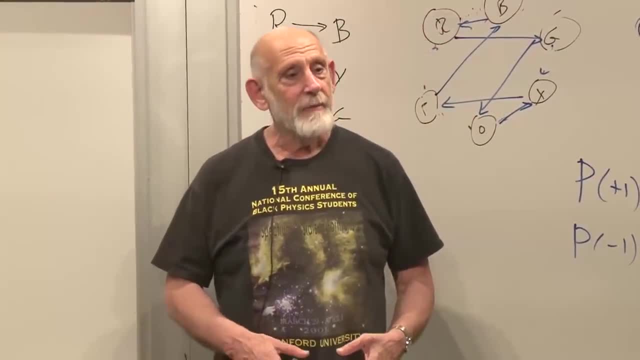 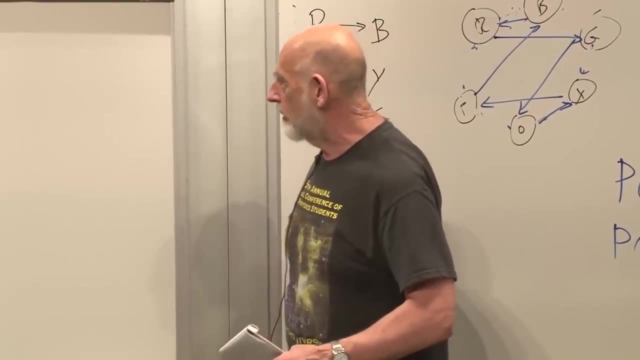 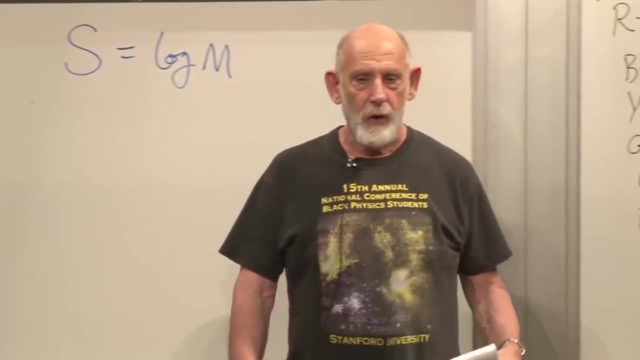 cause information to be lost, but because we just weren't careful. perhaps we can't be careful, perhaps there are too many degrees of freedom to keep track of. so when that happens, the entropy increases, but it simply increases because our ignorance has gone up, not because anything has really. 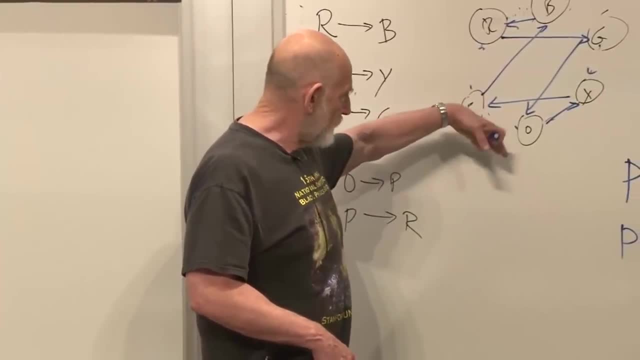 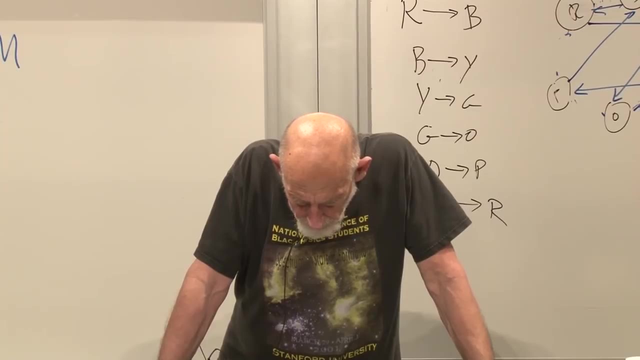 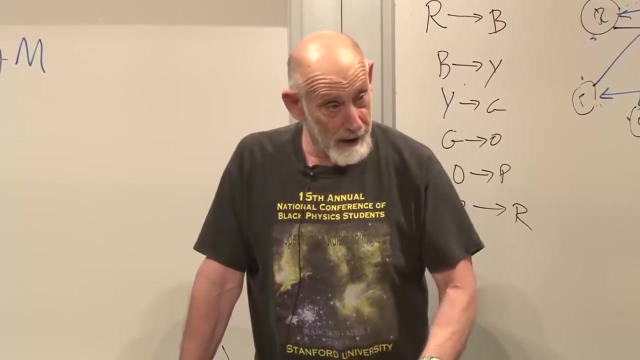 happened in the system, which has, if we could follow it, we would find that the entropy is conserved. okay, that's, that's the concept of entropy in a nutshell. we're going to expand on it a lot. we're going to redefine it with a more careful definition. 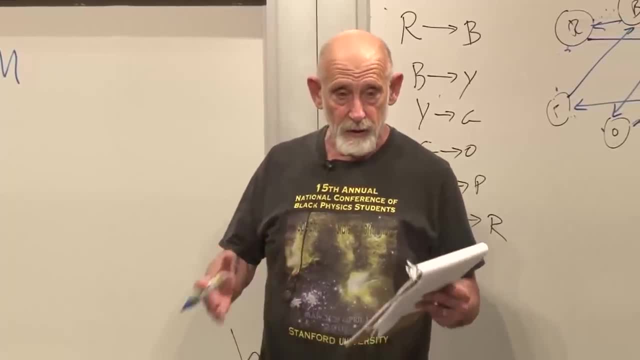 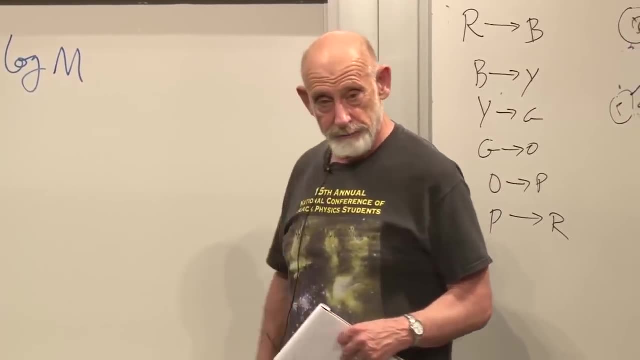 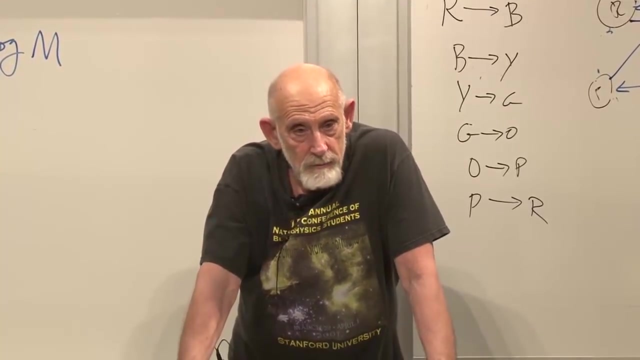 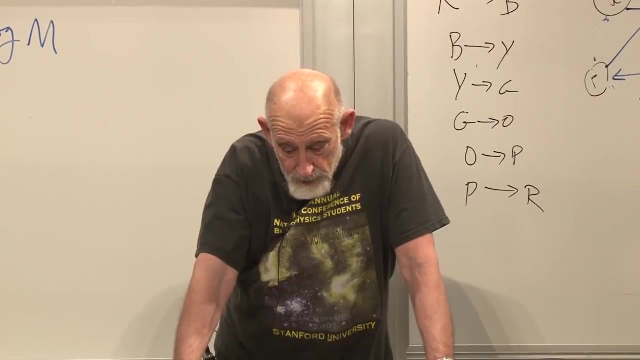 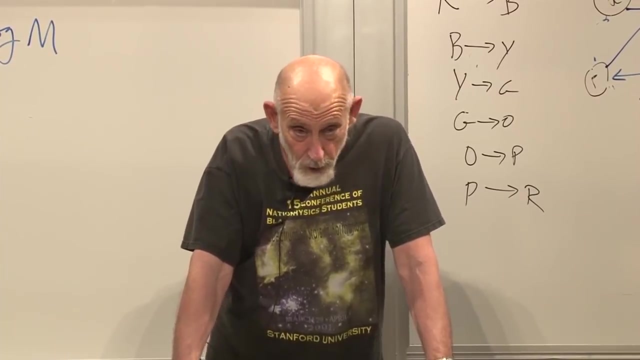 but what does it measure? it measures approximately the number of states that have a non-zero probability. okay, the bigger it is, the less. you know what's the maximum value of s login now? of course, n could be infinite. you might have an infinite number of states, and if you do, 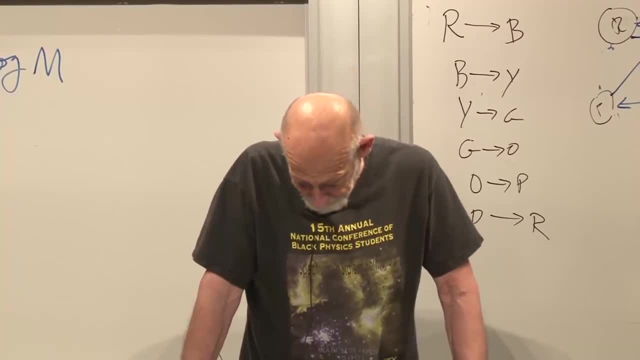 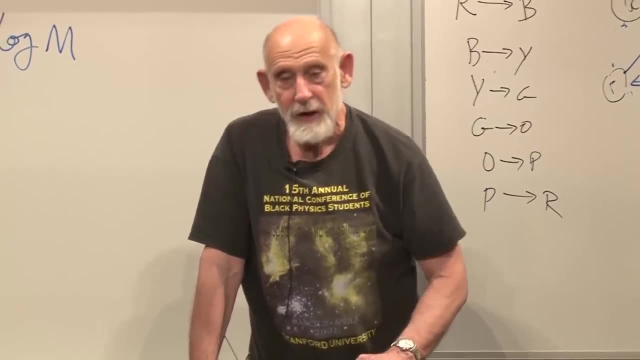 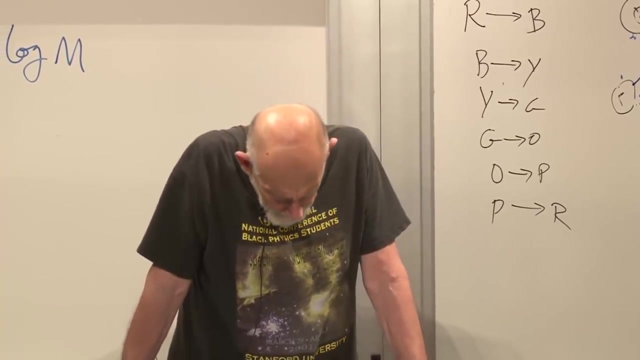 then there's no upper bound to the amount of ignorance you can have. but you know, in a world with only n states your ignorance is bounded. so the notion of maximum entropy is a measure of how many states there are altogether. now I said that entropy is deep and fundamental. 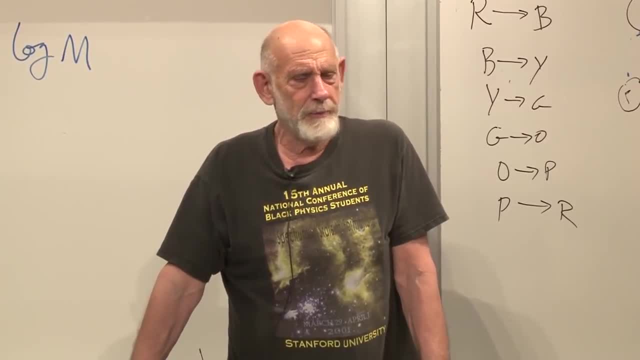 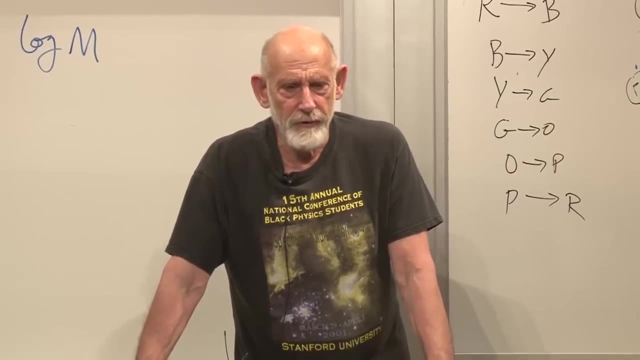 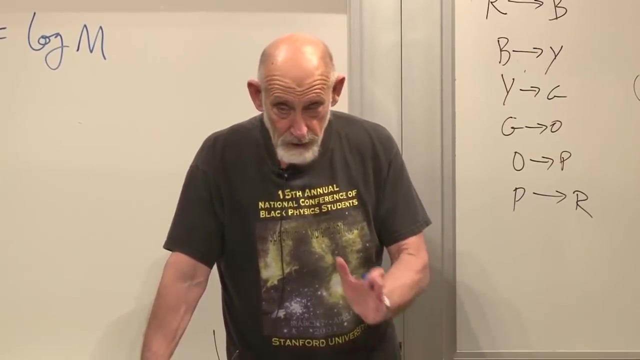 and so it is, and there's a sense to it which makes it, in a certain sense, less fundamental. it's not just a property of a system. it's a property of a system and your state of knowledge of the system. it depends on two things. it depends on characteristics. 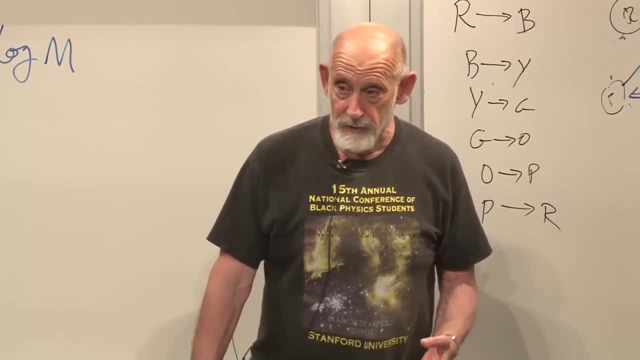 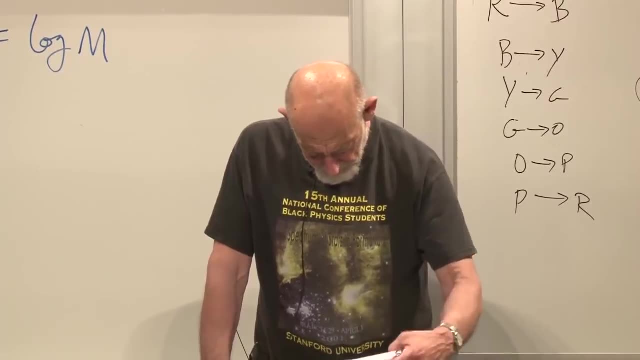 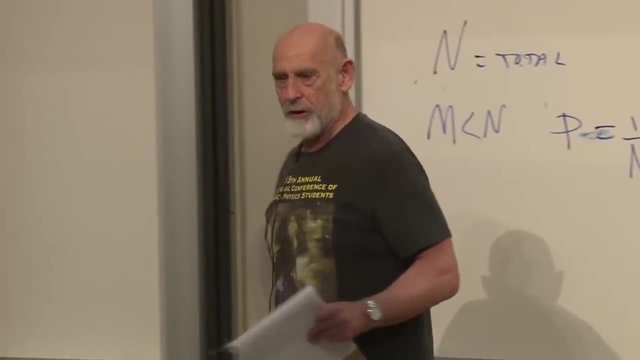 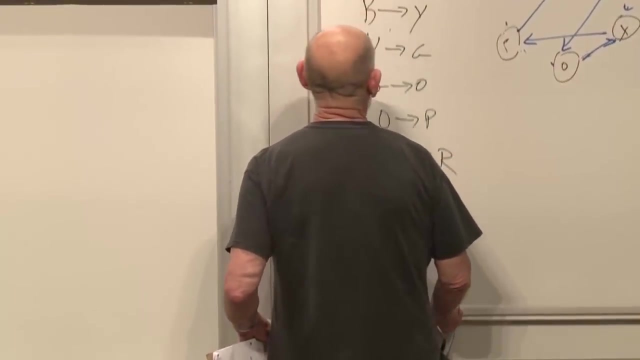 of the system, and it also depends on your state of knowledge of the system, or the state of knowledge of the system, so keep that in mind. okay, now let's talk about continuous mechanics, mechanics of particles moving around with continuous positions, continuous velocities. how do we describe that? 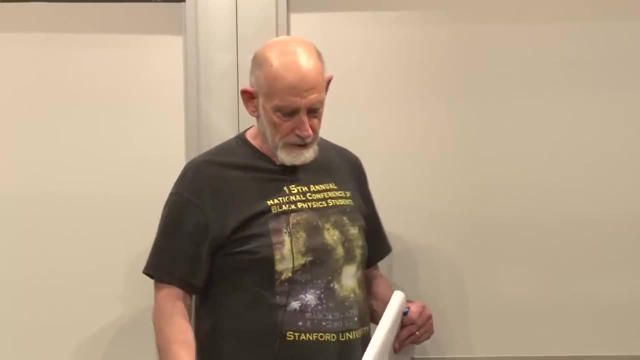 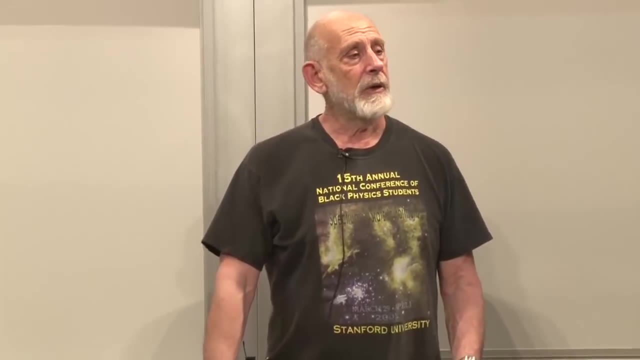 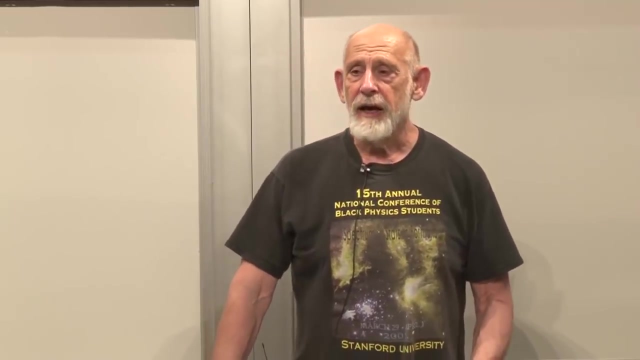 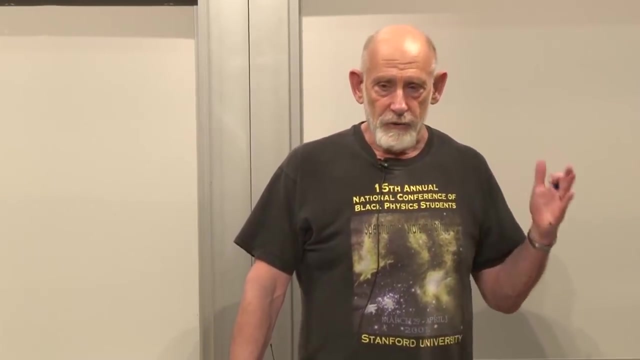 how do we describe the space of states, of a mechanical system- you know a real mechanical system- particles and so forth. we describe it as points in phase space. we learned about phase space. phase space consists of positions and momenta- momenta, in simple context, momentum is mass times, velocity. 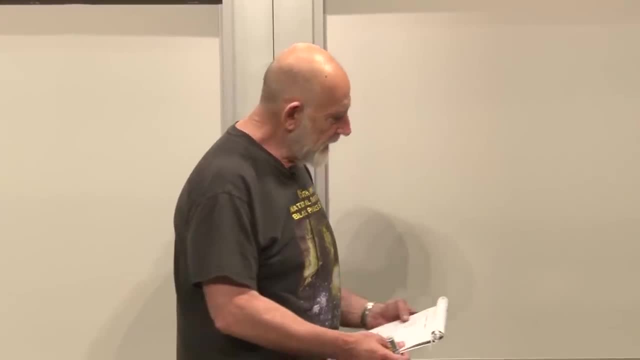 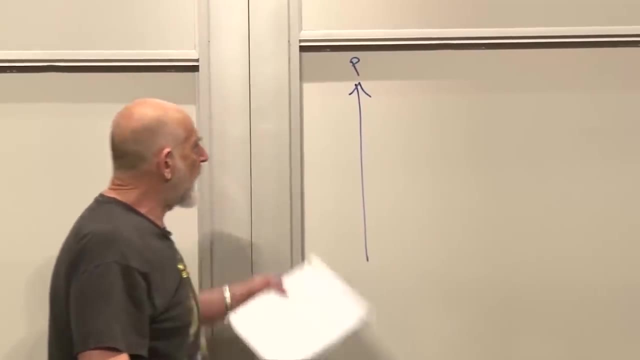 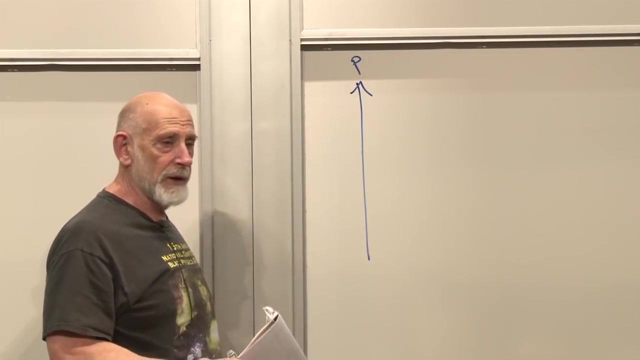 so, roughly speaking, it's the space of positions and velocities. let's draw it. p is momentum goes that way and this axis is a stand in for all of the momentum degrees of freedom. if there are 10 to the 23rd particles, there are 10 to the 23rd p's. 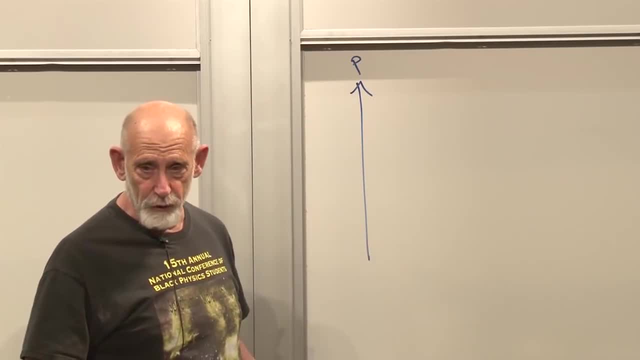 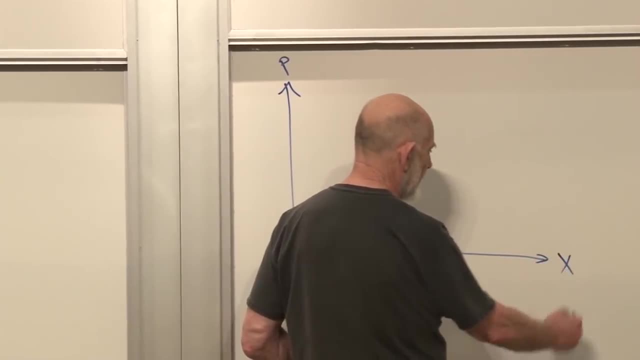 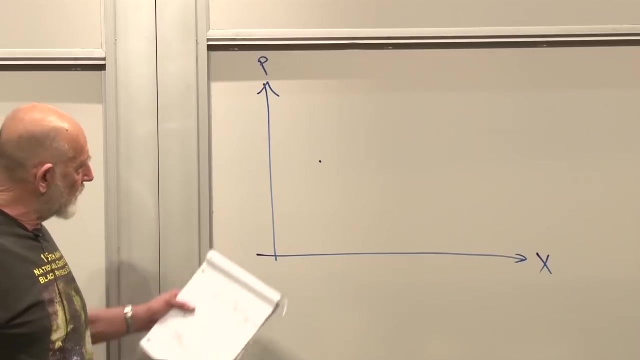 well, I could draw two of them, but then I wouldn't have any room for the q's, for the x's and, horizontally, the positions of the particles which we can call x, x or p, doesn't matter. alright, a point. here is a possible state of the system. 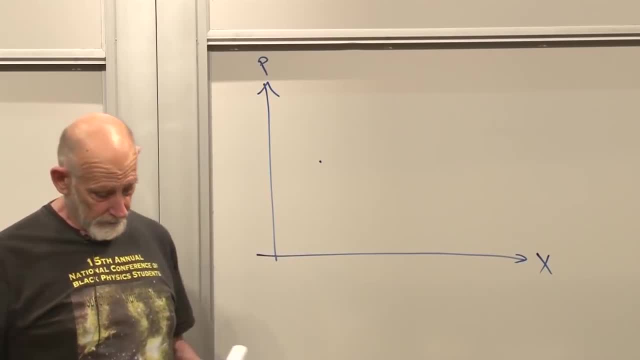 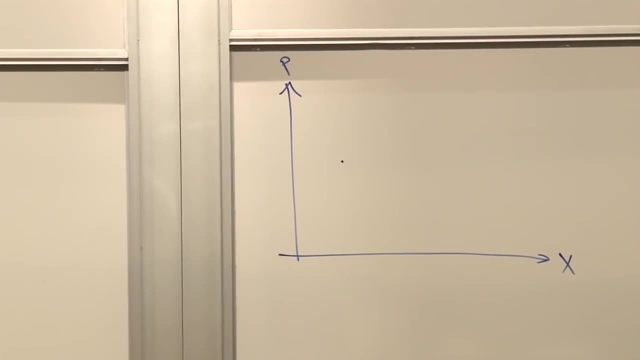 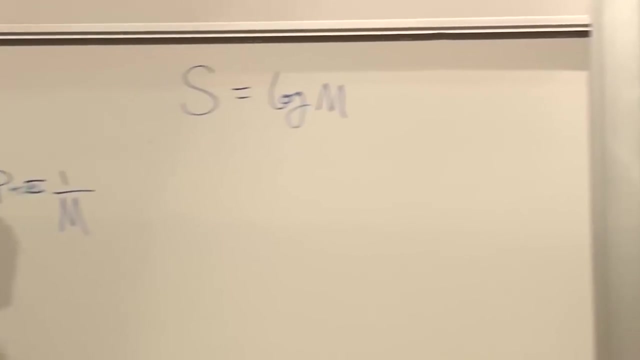 if you know a point here, you know a position and a velocity and you can predict from that. if you know the forces, okay, let's start with the analog of a probability distribution which is zero for some set of states and constant, or the same for some other set, for some smaller set. 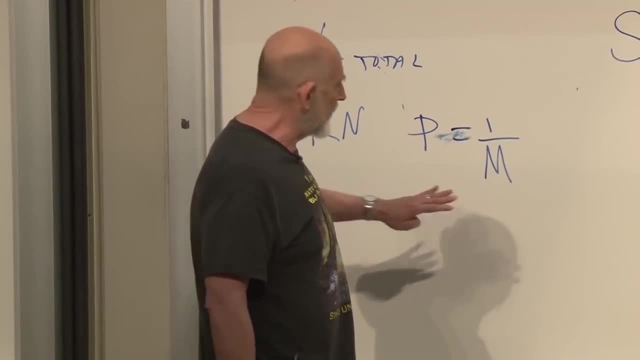 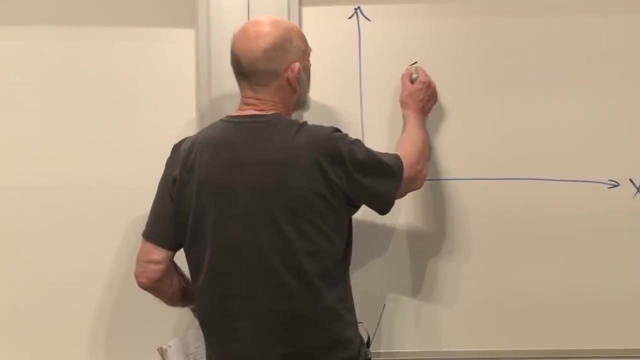 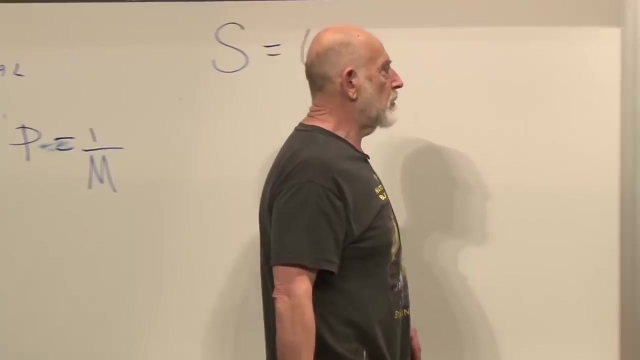 well, some fraction of the states all have the same probability and the other states have zero probability. we can represent that by drawing a, a patch in here, a subregion in the phase space, and say in that subregion there's equal probability that the system is at any point. 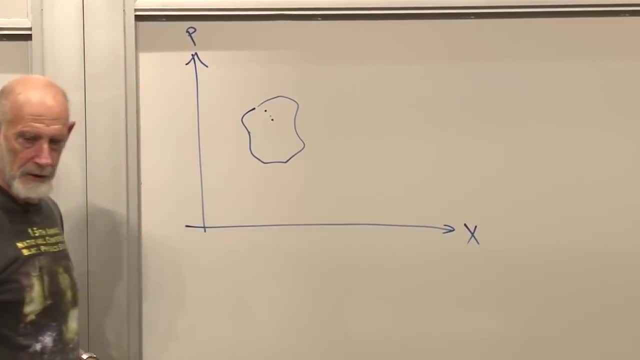 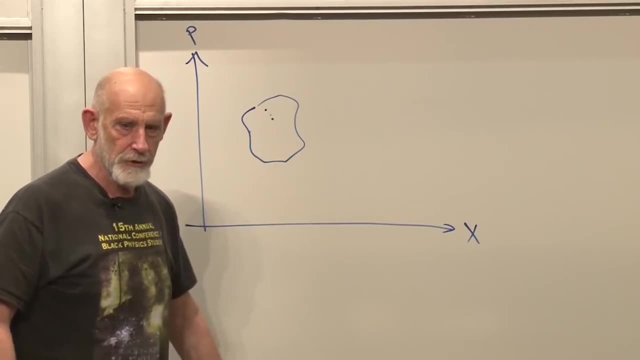 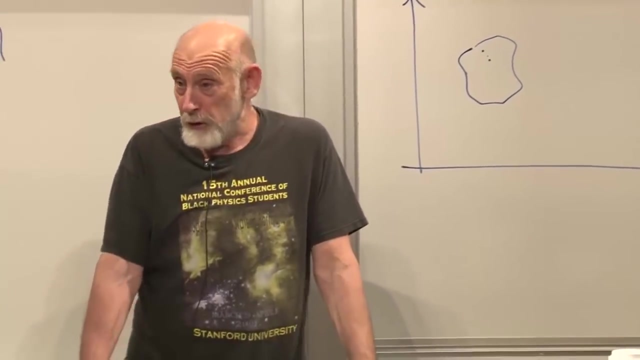 in here and zero probability outside. that's the sort of situation where you may know something, where you may know something about the particles that they're in some subregion here, for example. you know that all the particles in this room are in the room, right, so that puts some balance. 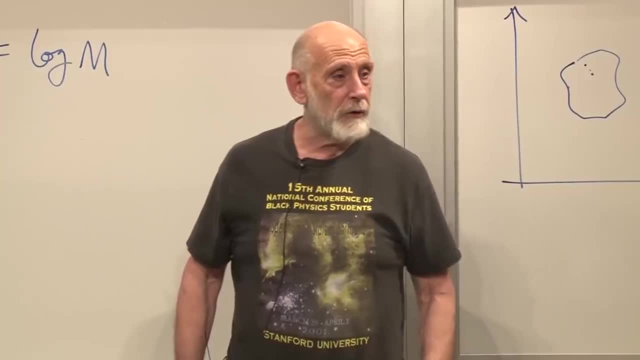 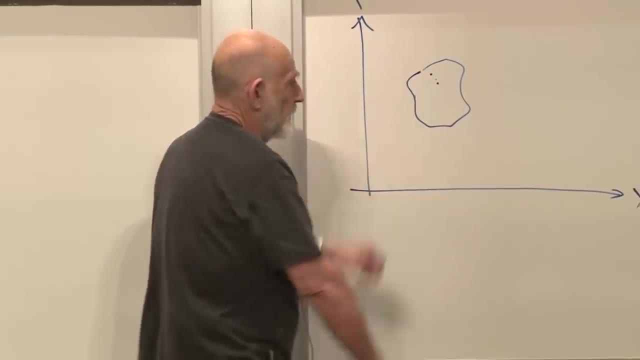 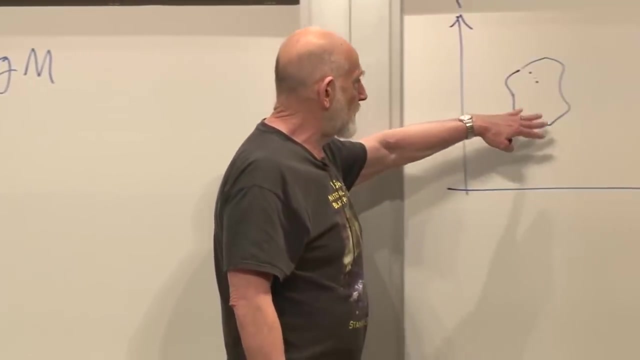 boundaries on what x are. you may know that all the particles have momentum which are within some range that confines them to this way, so a typical bit of knowledge about the room might be represented, at least approximately, by saying that the zero probability to be outside this region and a probability 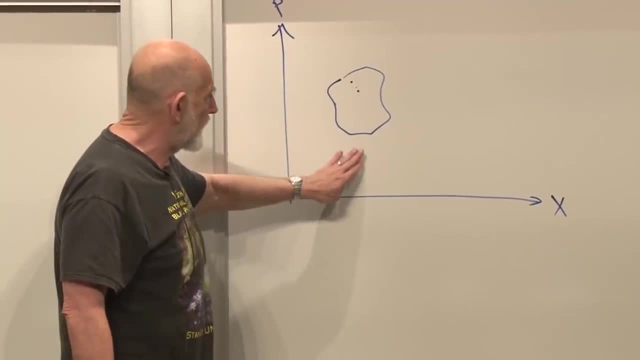 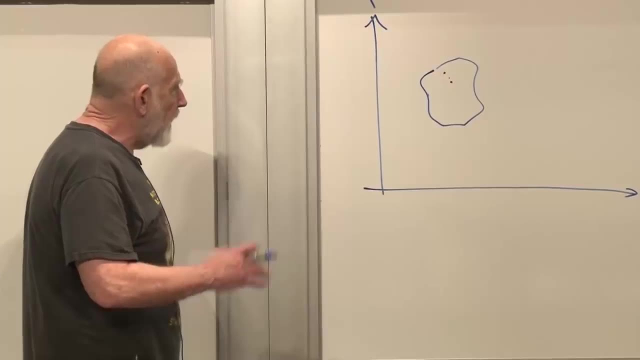 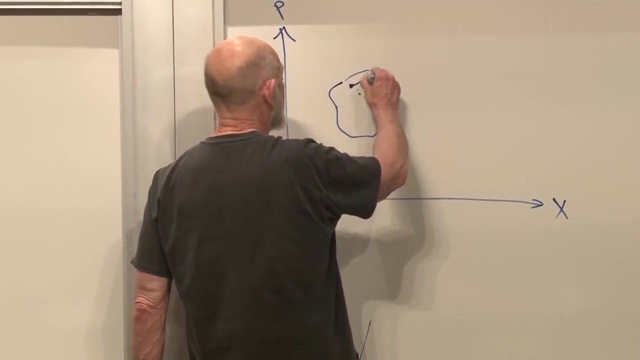 equal. I won't say one, but equal probability to be in there. okay, now what happens as the system evolves? as the system evolves, x and p change. the equations of motion say that x and p change. if you start over here, you might go to here if you start nearby. 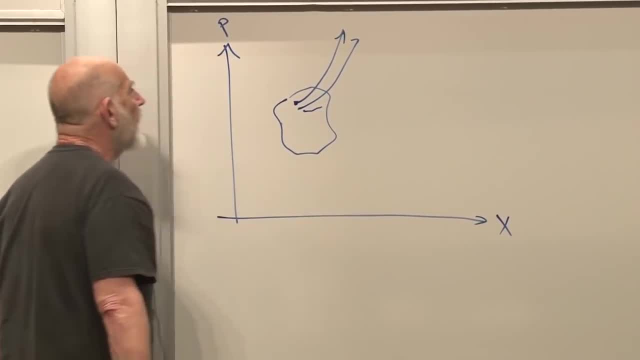 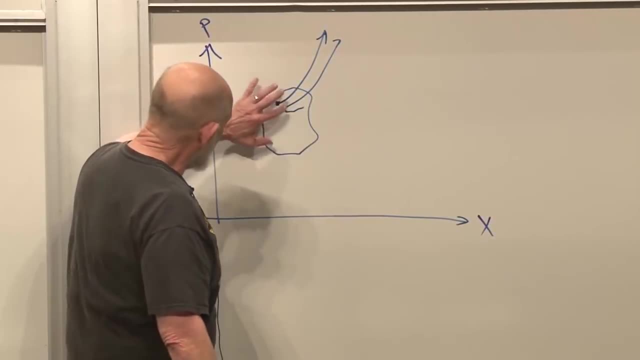 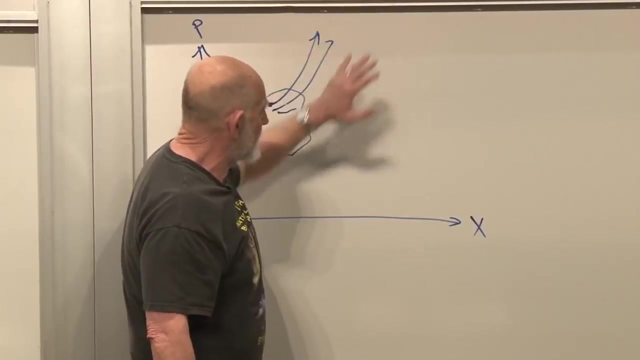 you'll go to some nearby point and so forth, and the motion of the system with time is almost like a fluid flowing in the phase space. if you think of the points of the phase space as fluid points and let time go, the phase space moves like a fluid. 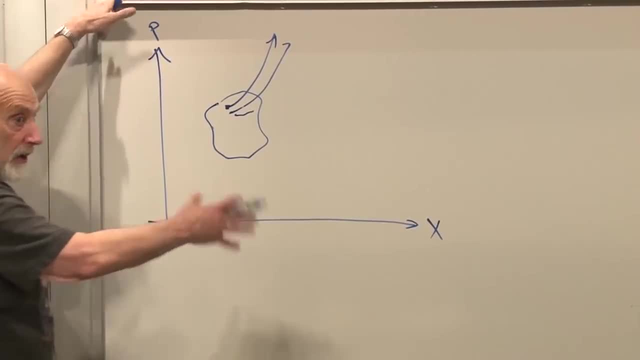 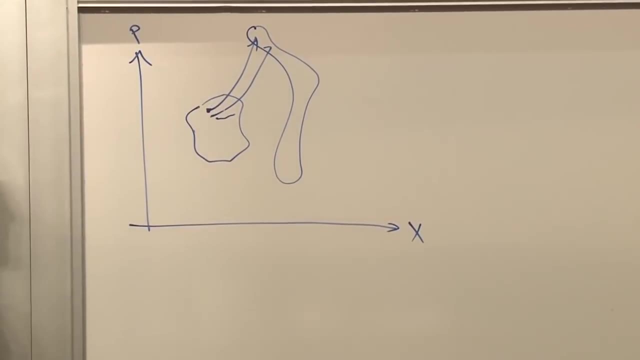 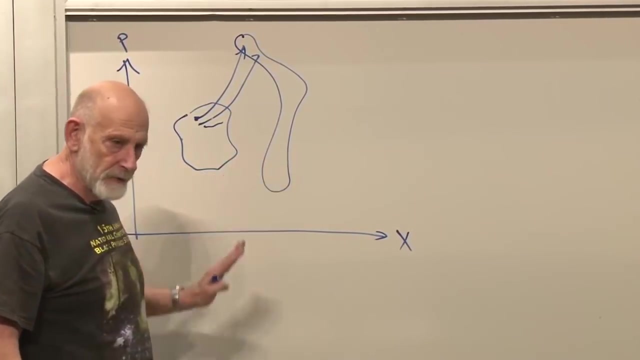 and in particular this patch over here. let's call it the occupied patch. the occupied patch becomes some other patch, that other patch, after a certain amount of time. the system now is known to be in here. after a certain amount of time we now know that the system 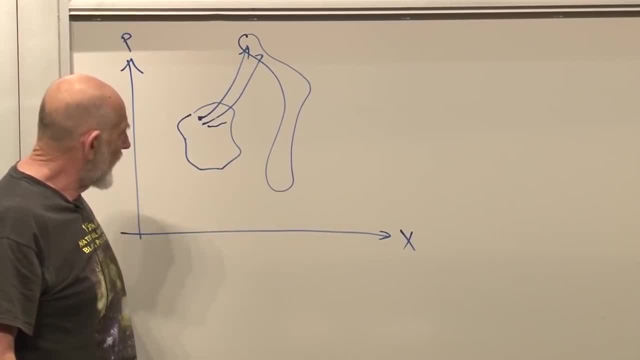 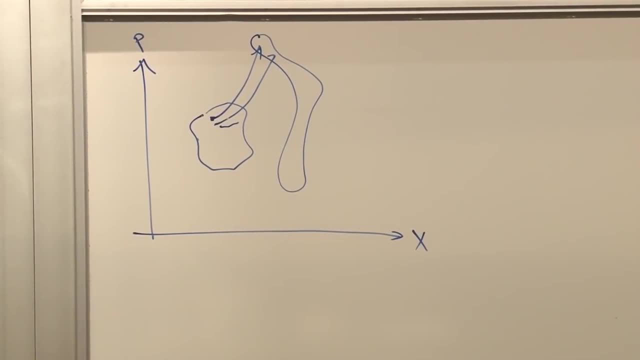 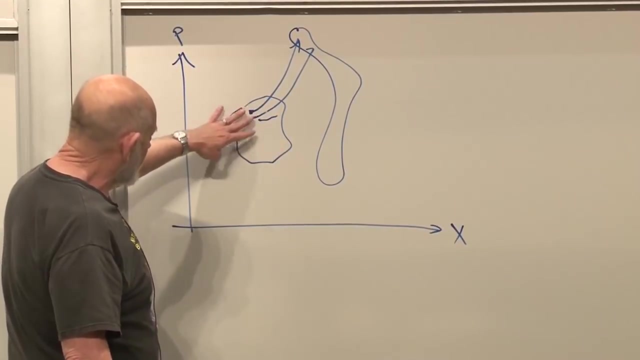 is in here, not in here anymore, and that it has equal in some sense equal- probability to be anywhere in there. okay, there's a theorem that goes with this. the theorem is called Liouville's theorem, and what it says is that the volume of phase 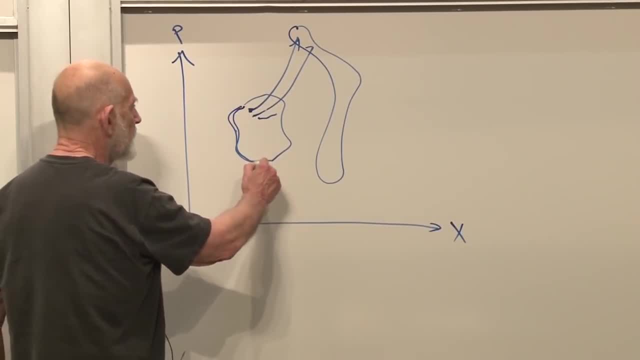 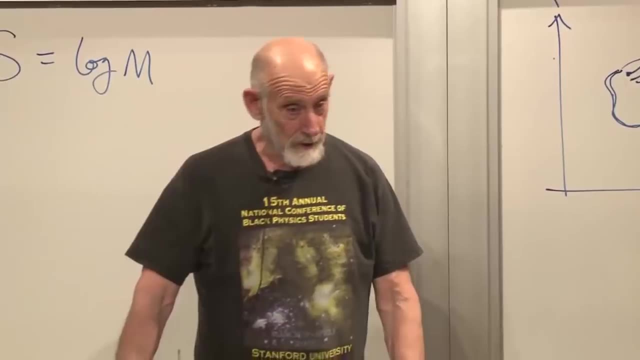 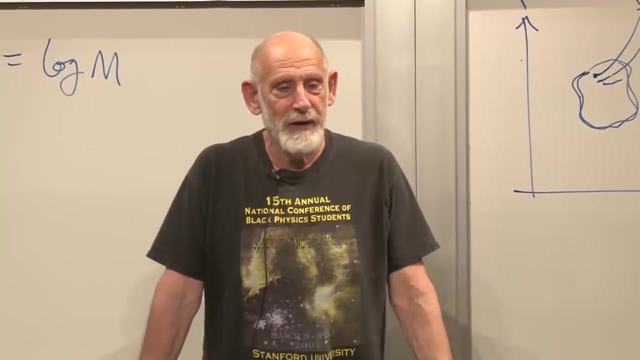 the volume in phase space, the amount of volume of this region in the xp space, and keep in mind the xp space may be high dimensional. if it were two dimensional, we would think of it as the area. phase space is never three dimensional, it's always even dimensional. 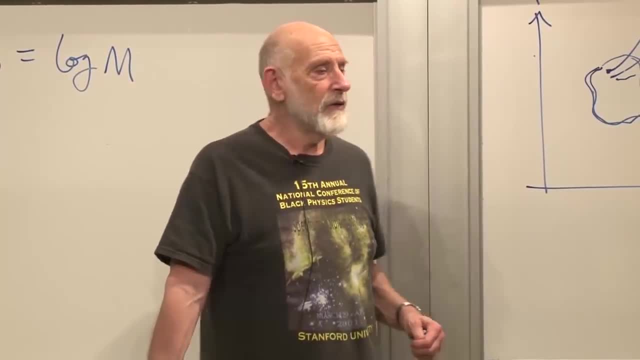 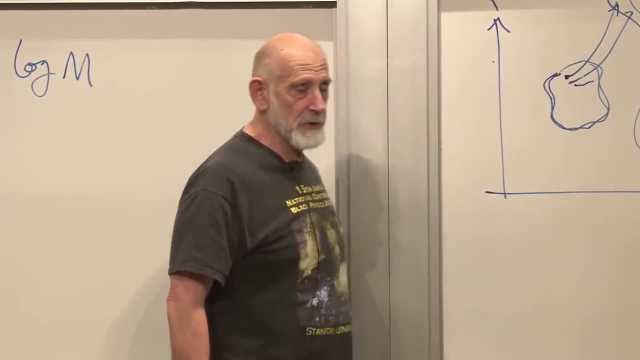 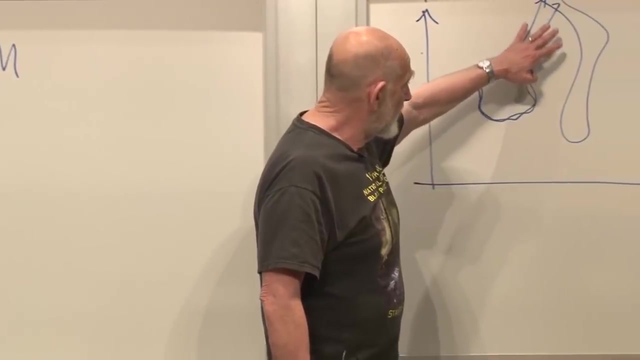 it has a p for every x. so the next more complicated system would be four dimensional. when I speak of the volume in phase space, I mean the volume in whatever dimensionality the phase space is. if you follow the phase space in this manner here, Liouville's theorem. 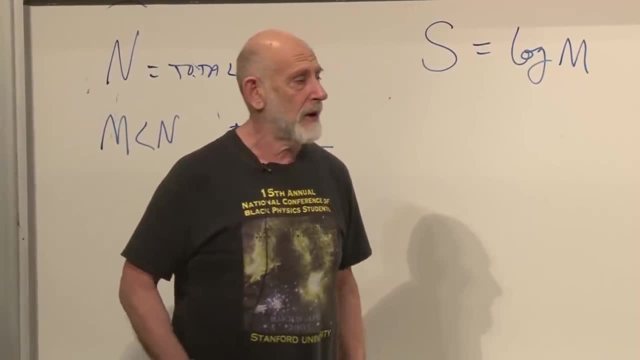 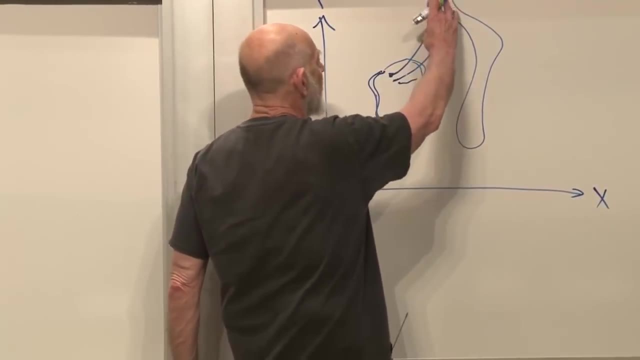 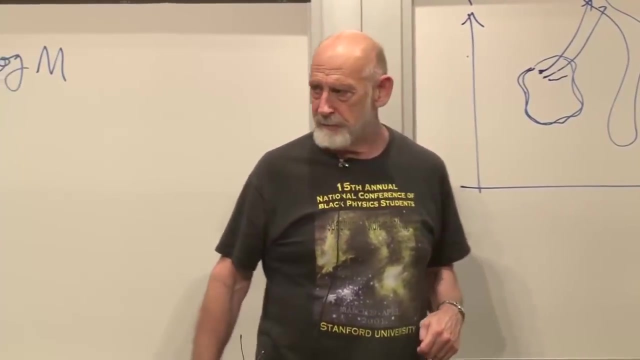 you can go back to Liouville's theorem. it's in the classical mechanics lecture notes, I think, and it tells you whatever this evolves into. it evolves into something of the same volume, in other words, roughly speaking, the same number of states. it's the immediate analog. 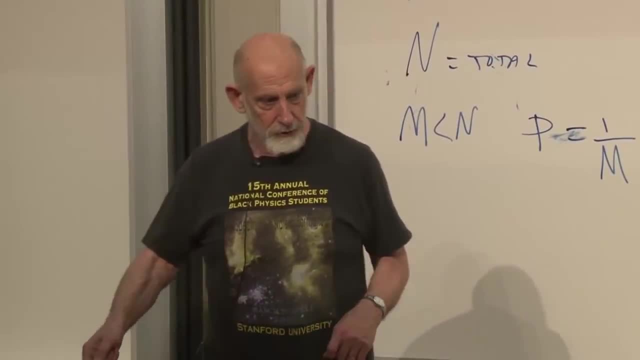 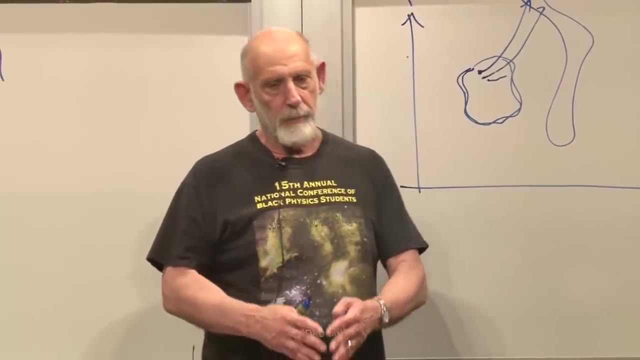 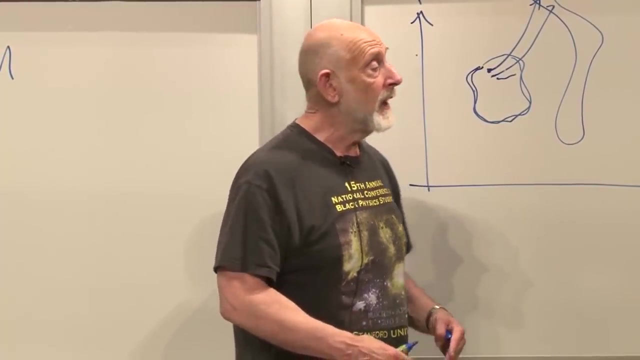 of the discrete situation where, if you start with m states and you follow the system according to the equations of motion, you will occupy the same number of states. afterwards there will be different states, but you will preserve the number of them and the probabilities will remain equal. so the rule is: 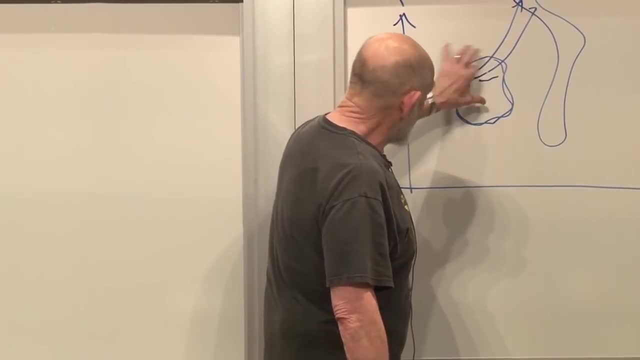 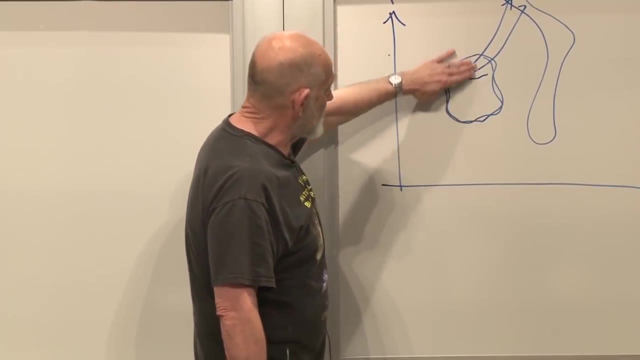 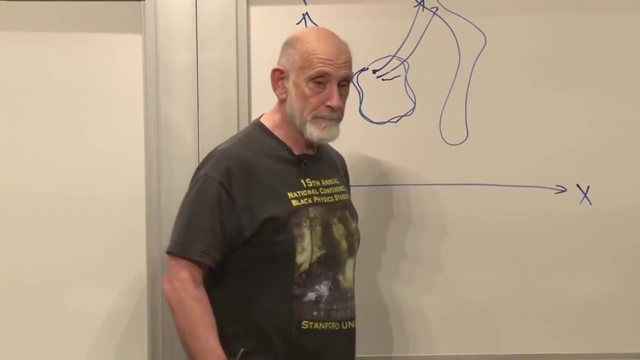 not the rule. the theorem says that the volume of this occupied region will stay the same and a little bit better. it says that if you start with a uniform probability distribution in here, it will be uniform in here. so there's a very, very close analog between. 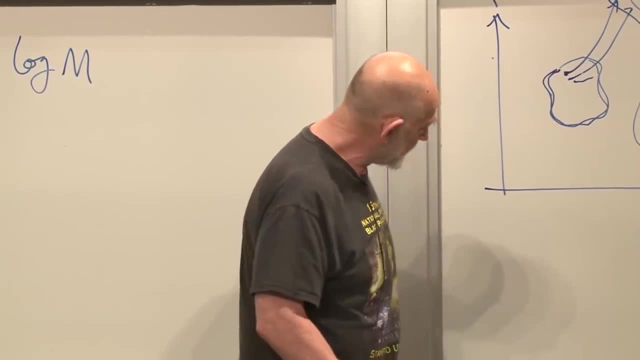 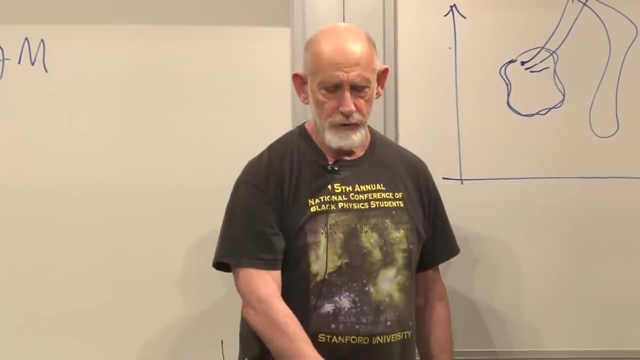 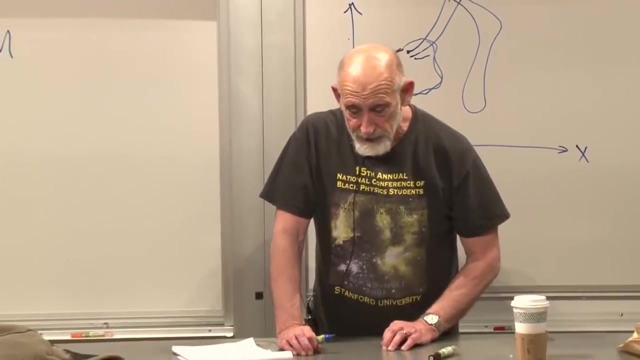 the discrete case and the continuous case, and this is what prevents this kind of fundamental equation from this kind of equation, an equation where everything comes to rest. that can't happen. ok, why not? let's see why it can't happen. let's just look on this blackboard. 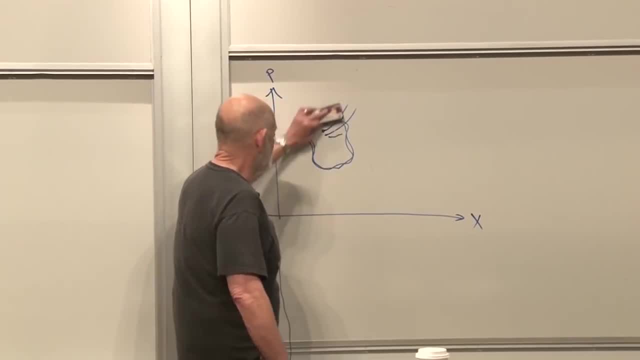 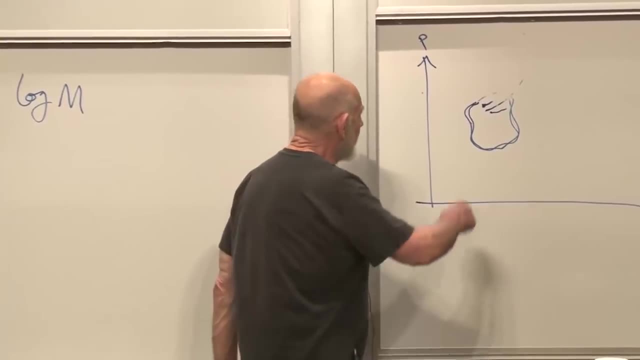 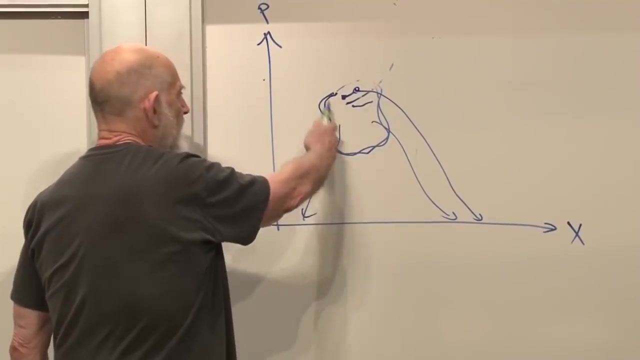 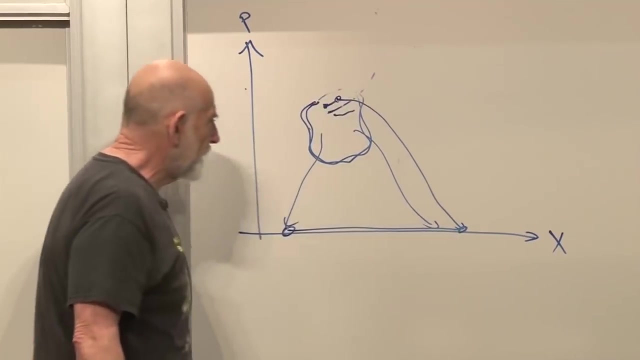 and see why. imagine that no matter where you started, you ended up with p equals zero. that would mean every point on here got mapped to the x-axis. it would mean that this entire region here would get mapped to a one-dimensional region and a one-dimensional region. 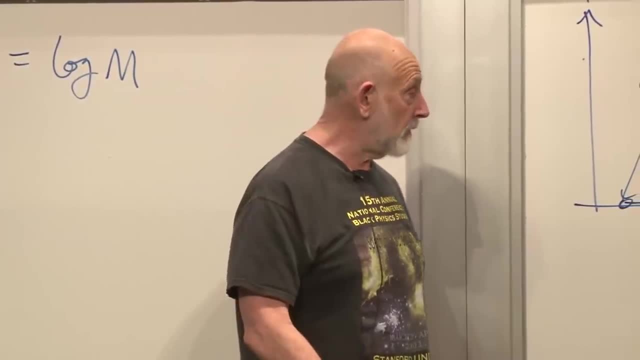 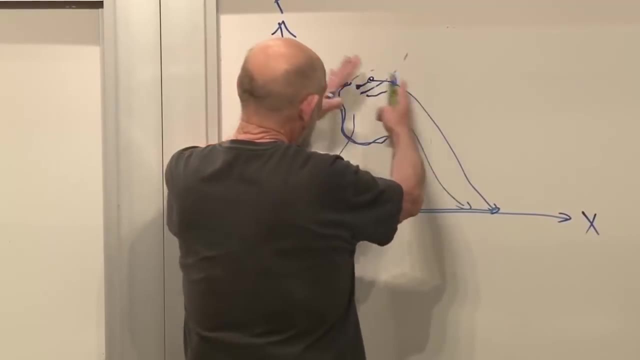 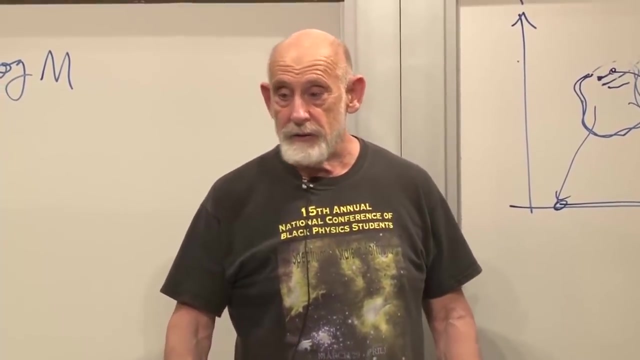 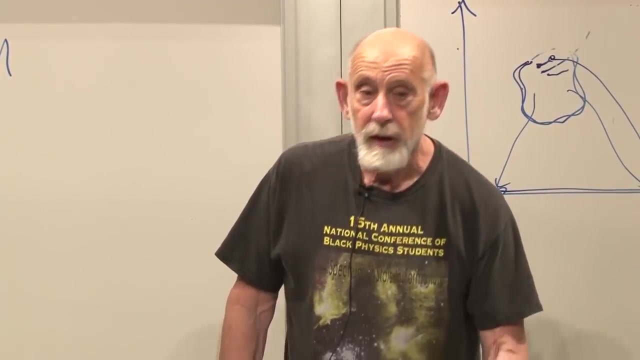 has zero area. so Leaville's theorem prevents that. what it says in fact is: if the blob squeezes in one direction, it must expand in the other direction. the situation for the moving eraser is that if the phase space of the eraser gets shrunk, 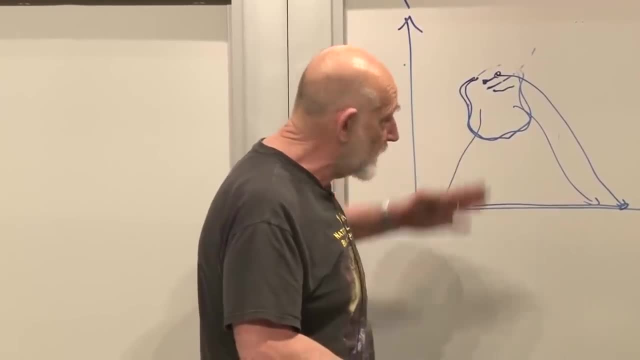 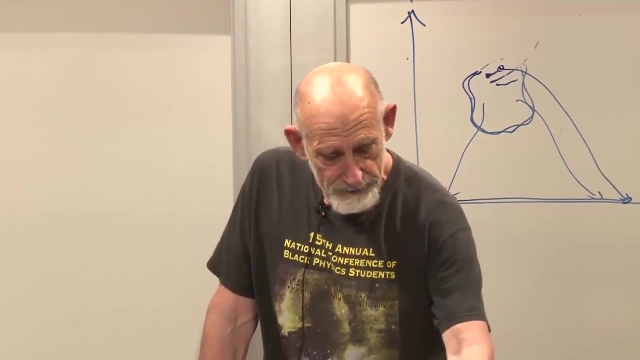 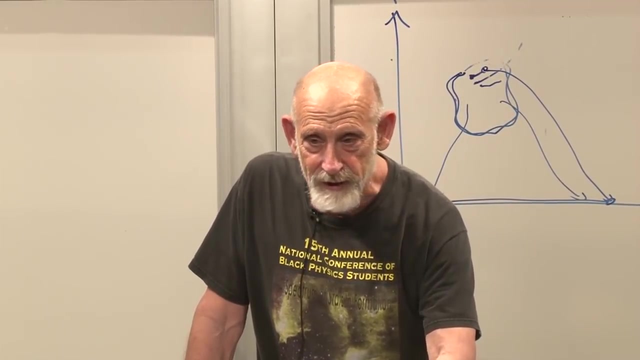 it means somebody else's some other components. in the phase space, the probability distribution is spread out. what are the other components? in this case, it's the p's and x's of all the molecules that are in the table. so for the case of the eraser, 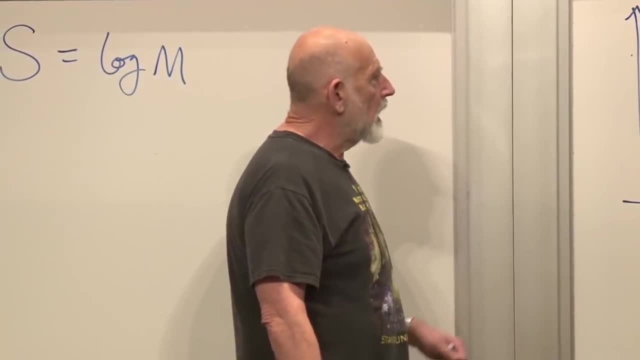 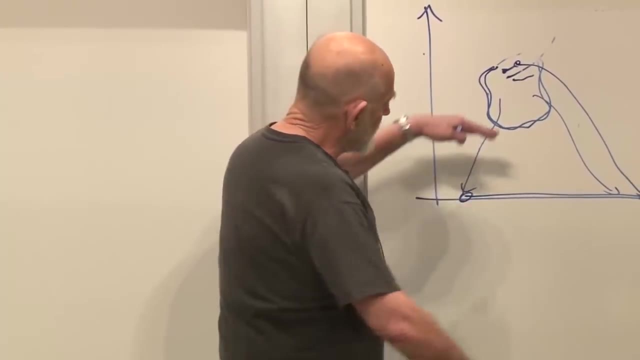 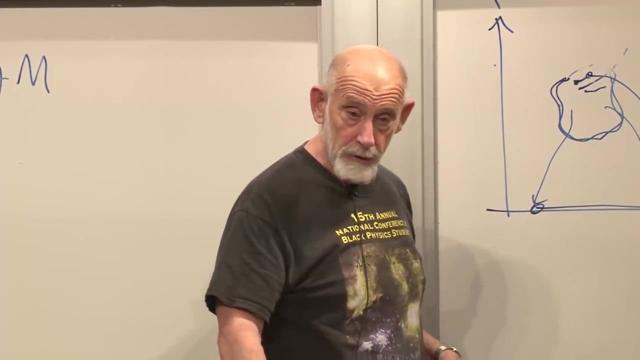 there's really a very high dimensional phase space and, as the eraser may come to rest, almost rest, so that the phase space squeezes, this way it spreads out in the other directions, the other directions having to do with the other hidden, microscopic degrees of freedom. okay, so there we are. 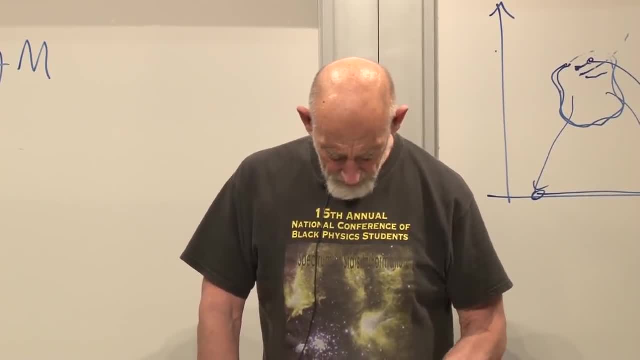 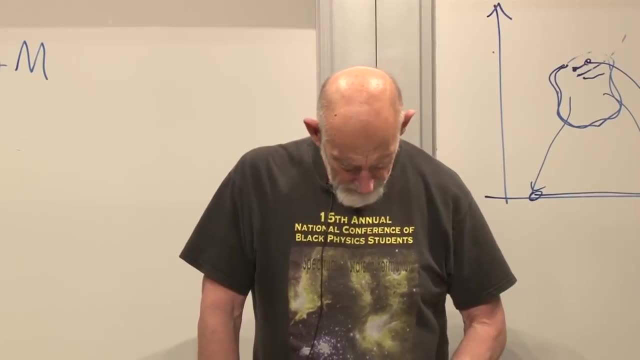 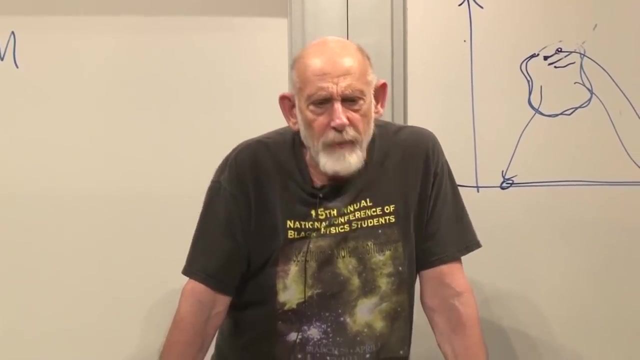 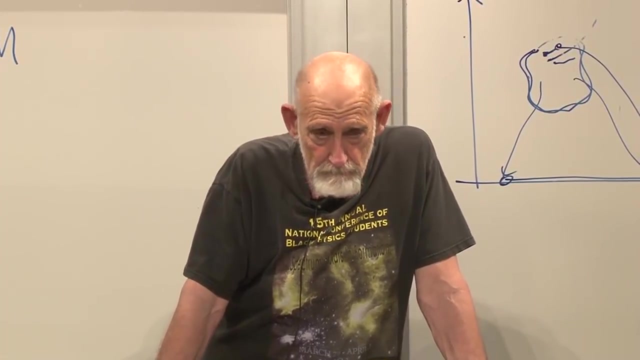 with information conservation minus first law of physics. and let's pass. let's not go to the zeroth law, let's jump the zeroth law, we'll come back to the zeroth law. anybody know what the zeroth law says? well, I'll tell you what it says. 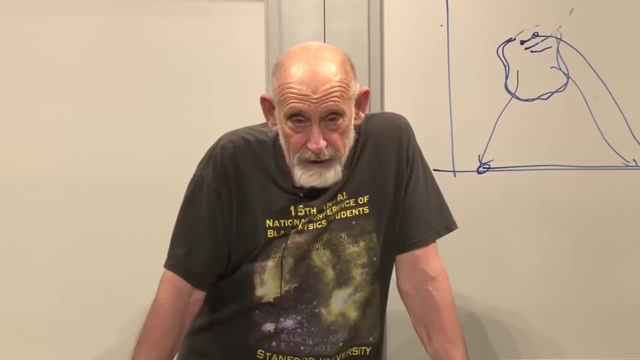 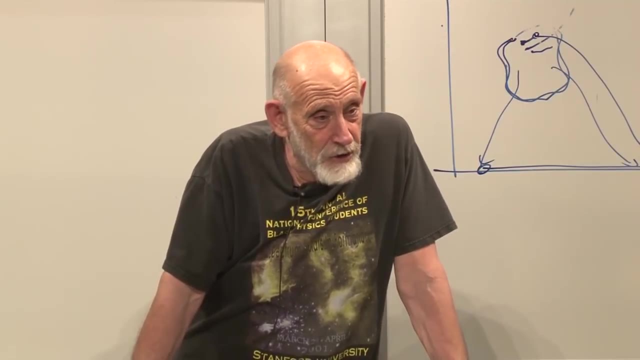 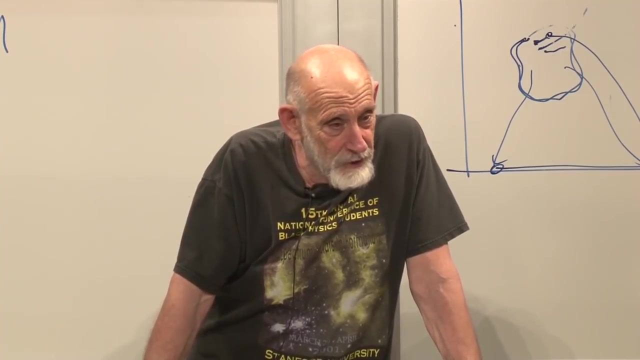 we haven't defined what thermal equilibrium is. okay, but it says whatever the hell thermal equilibrium is. if you have several systems and system A is in thermal equilibrium with B and B is in thermal equilibrium with C, then A is in thermal equilibrium with C. we will come back to that. 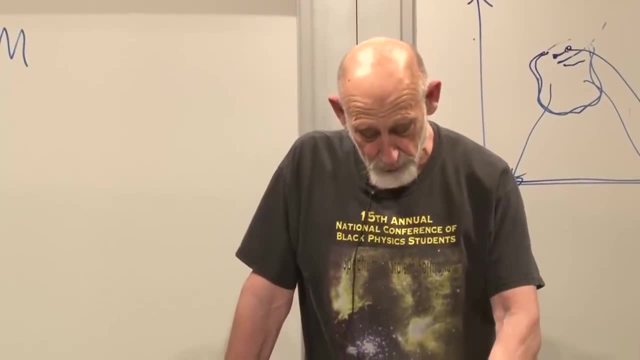 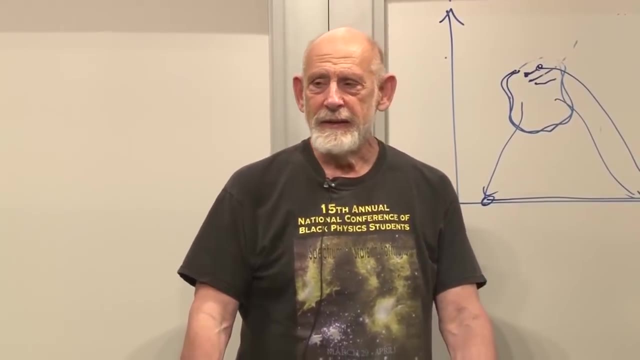 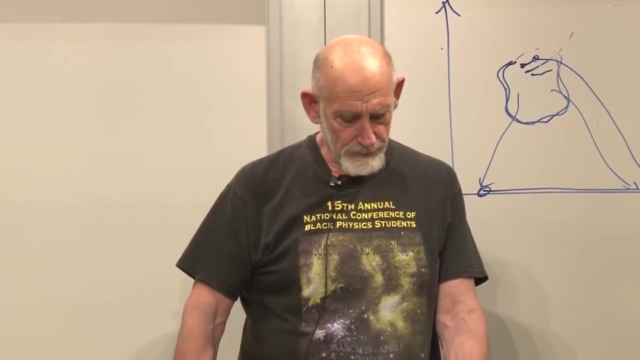 just put it out of your mind for the time being, because we haven't described what thermal equilibrium means. but we can now jump to the first law minus one zero, and first law. and the first law is simply energy conservation. it is simply energy conservation, nothing more. it's really simple to write down. 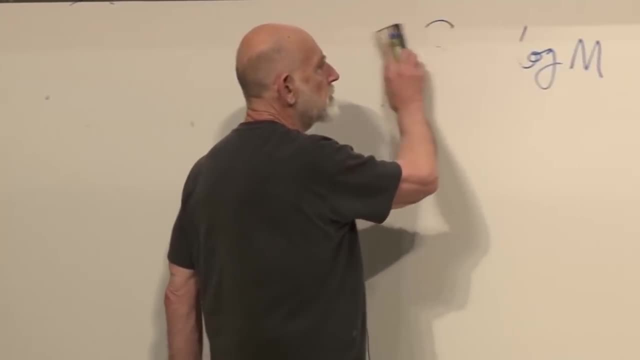 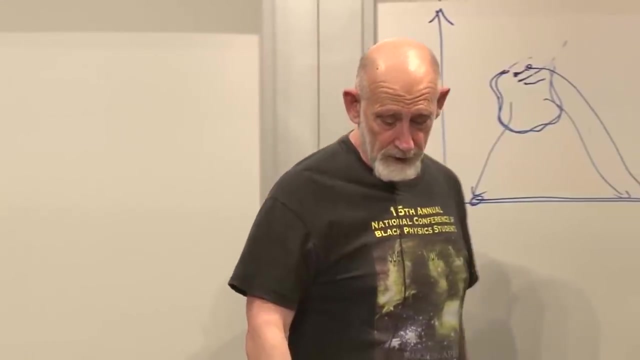 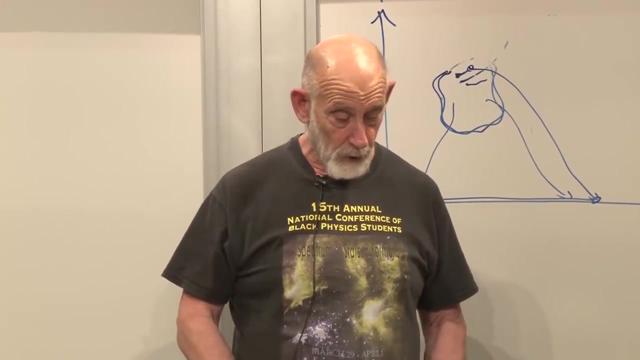 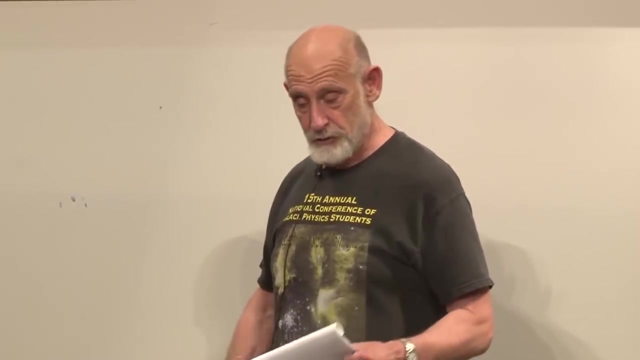 its simplicity belies its power. it is the statement that, first of all, there is a conserved quantity, and the fact that we call that conserved quantity. energy will play, for the moment, not such a big role right now, but let's just say there is energy conservation. 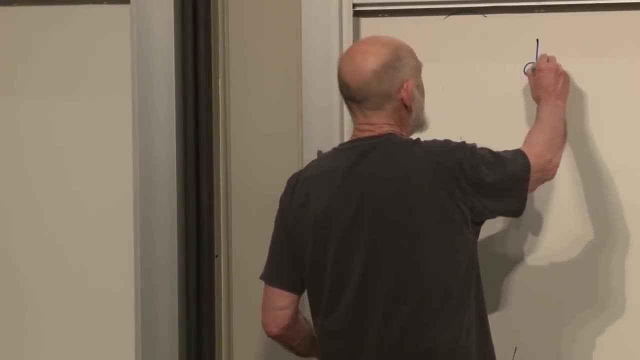 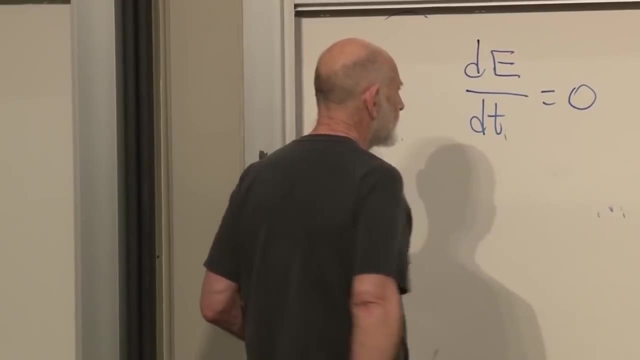 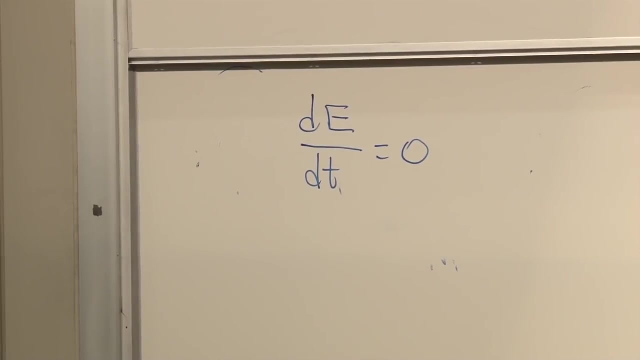 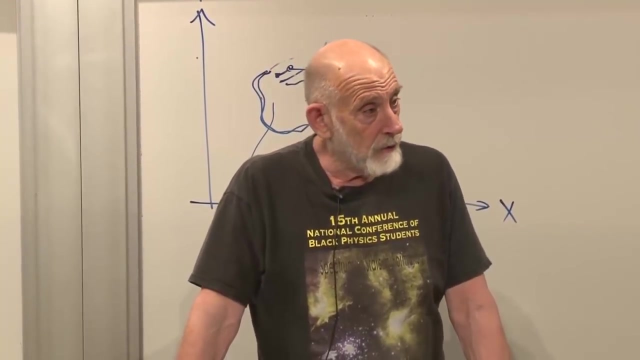 alright. what does that say? that simply says dE, whatever the energy is. dE by dt is equal to zero. this is the law of energy conservation for a closed system. if a system consists of more than one part in interaction with each other, then of course any one of the parts. 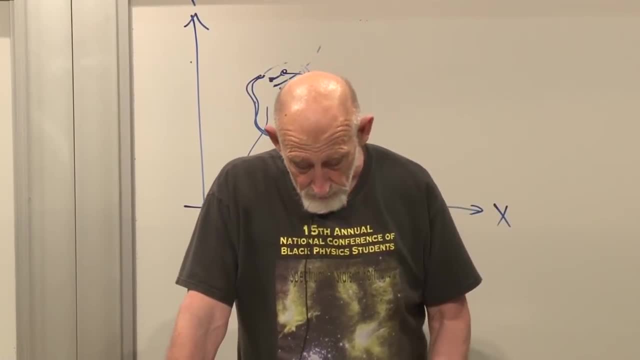 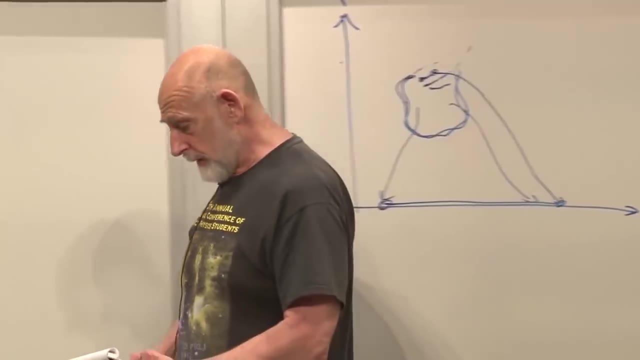 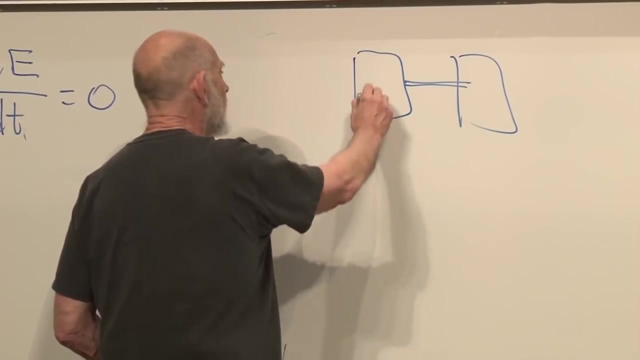 can have a changing energy, but the sum total of all of the parts will conserve energy. so if a system is composed, as I drew before, of two parts with a link between them, and this is called one and this is two, then this reads that dE1 by dt. 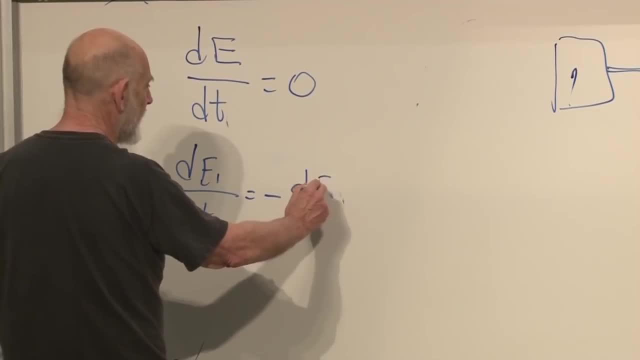 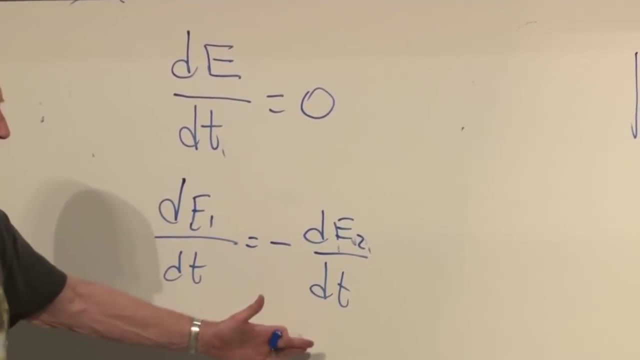 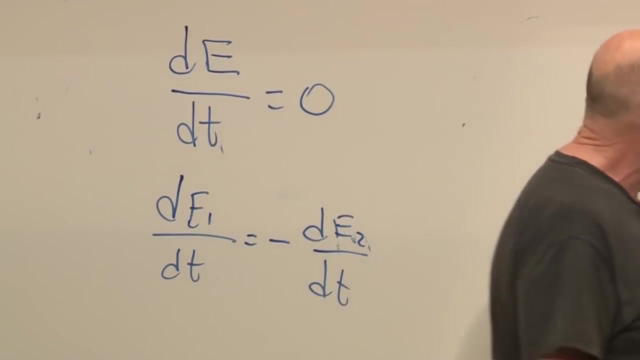 is equal to minus dE2 by dt. I've really written dE1 by dt plus dE2 by dt is equal to zero. but then I transposed one of them to the right hand side just to indicate, just to make graphic, that if you lose energy on one side, 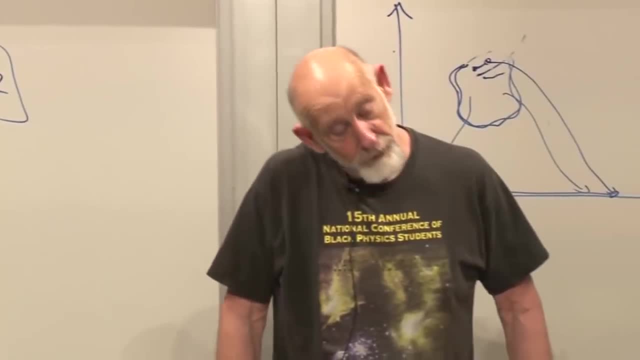 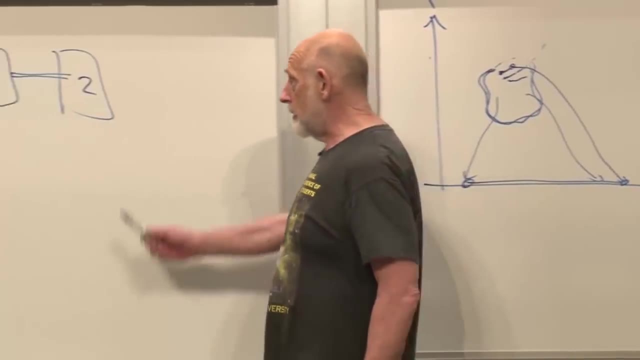 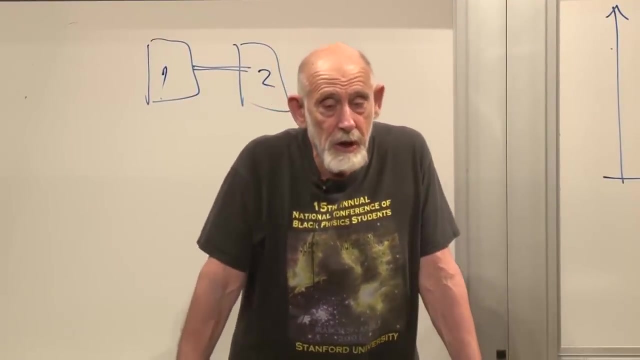 you gain it on the other. so that's the first law of thermodynamics, and that's all the first law of thermodynamics says. it says energy conservation. now, in this context, here there's a slightly hidden assumption. we've assumed that if a system is composed of two parts, 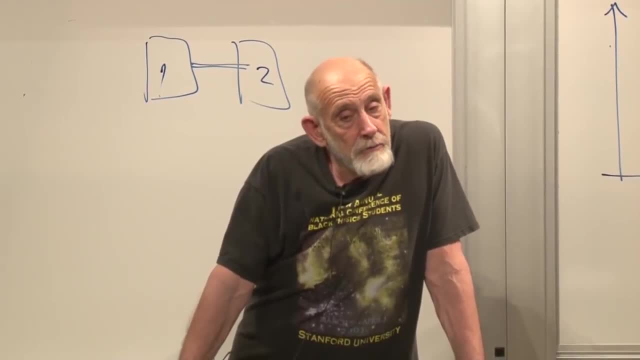 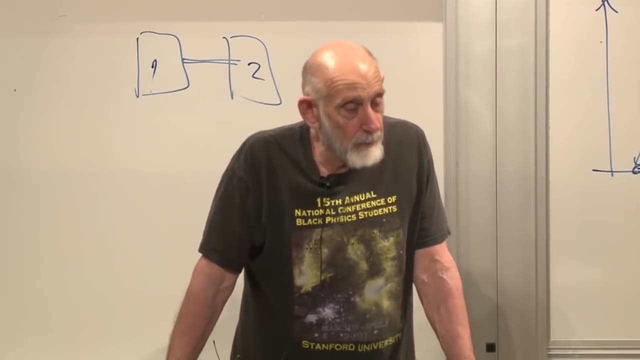 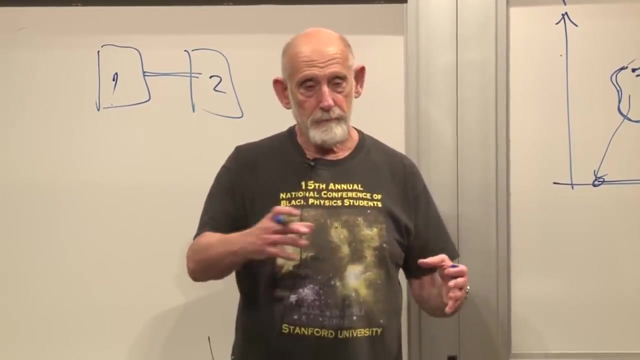 that the energy is the sum of the two parts. that's really not generally true. if you have two systems and they interact with each other, there may be, for example, forces between the two parts, so there might be a potential energy. that's a function of both of the coordinates. 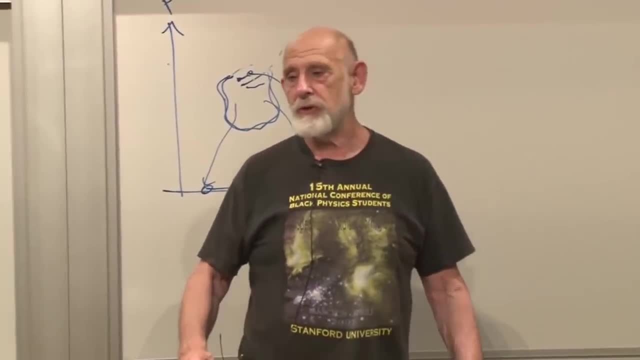 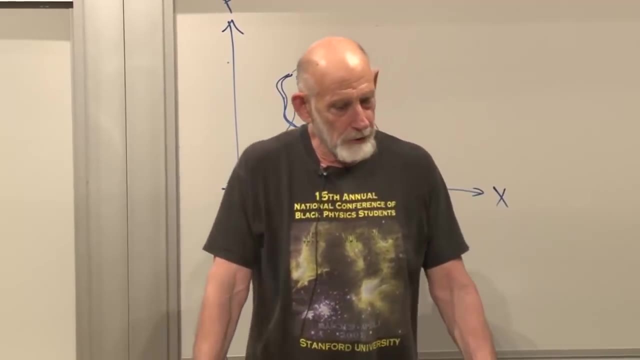 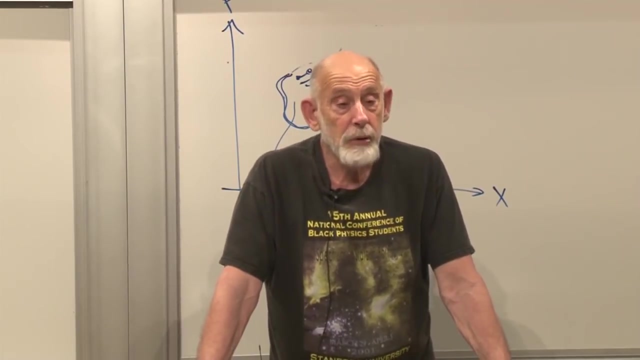 for example, the energy of the solar system. I'm being very naive. I'm thinking of the solar system as two orbiting Newtonian particles. the energy consists of the kinetic energy of one particle plus the kinetic energy of the other particle, plus a term which doesn't belong to either particle. 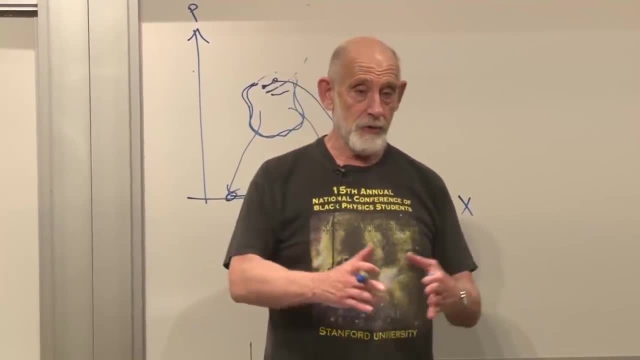 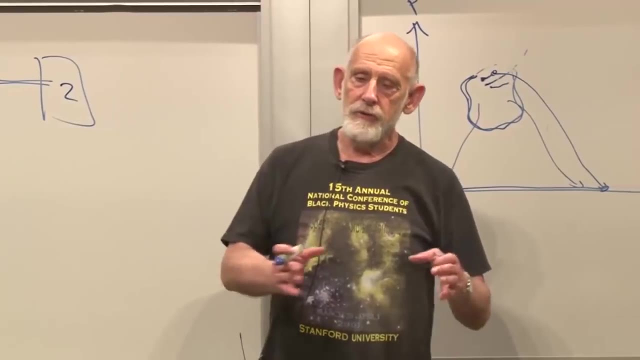 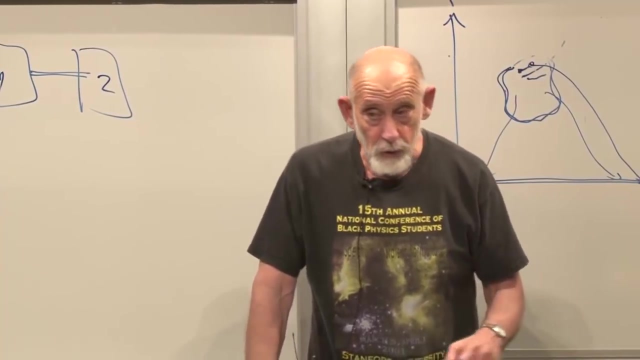 it belongs to both of them in a sense, and it's the potential energy interaction between them. in that context, you really can't say that the energy is the sum of the energy of one thing plus the energy of the other thing. energy conservation is still true, but you can't divide. 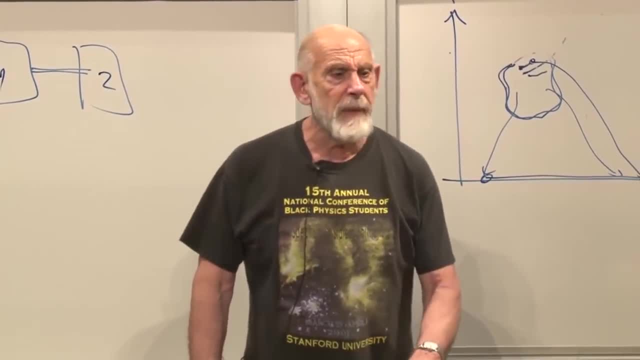 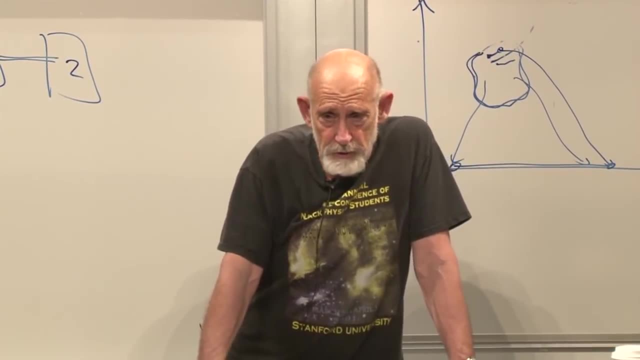 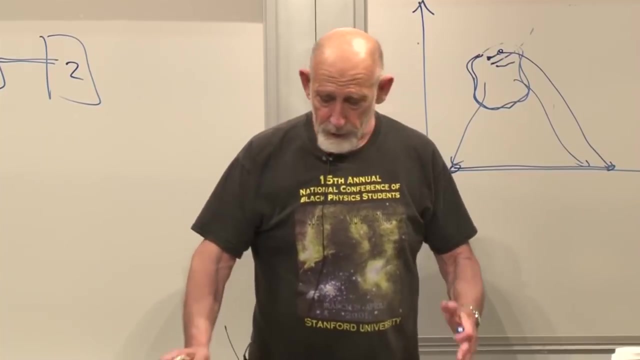 the system into two parts this way. on the other hand, there are many, many contexts where the interaction energies between systems is negligible compared to the energy that the system themselves have. if we were to divide this table top up into blocks, let's think about it. divide the table top up into blocks. 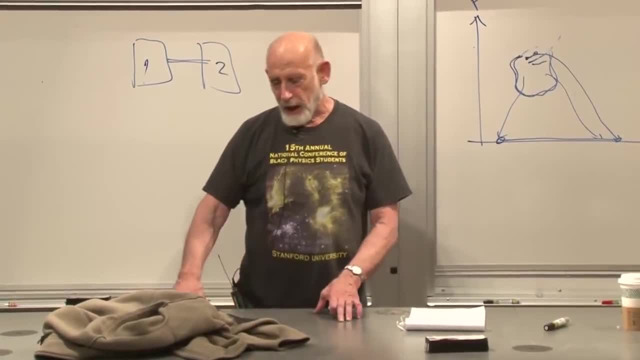 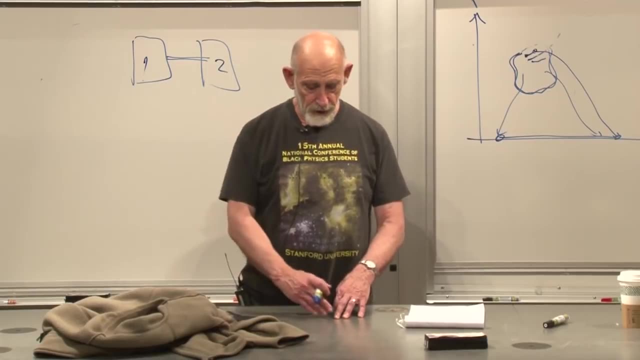 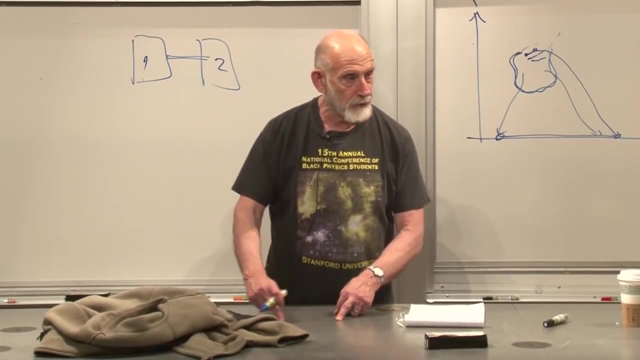 how much energy is in each block? well, the amount of energy that's in each block is more or less proportional to the volume of each block. how much energy of interaction is there between the blocks? the energy of interaction is a surface effect. they interact with each other. 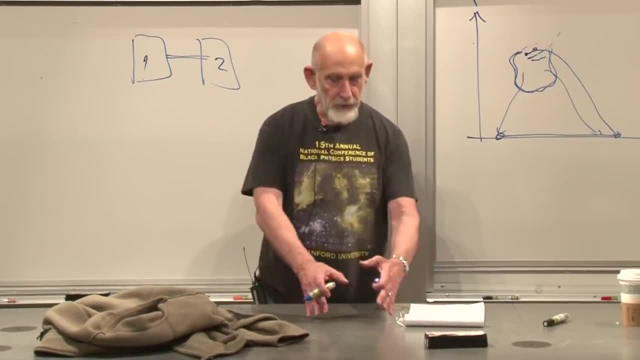 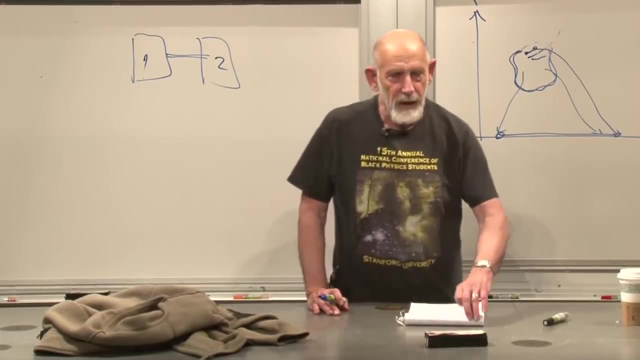 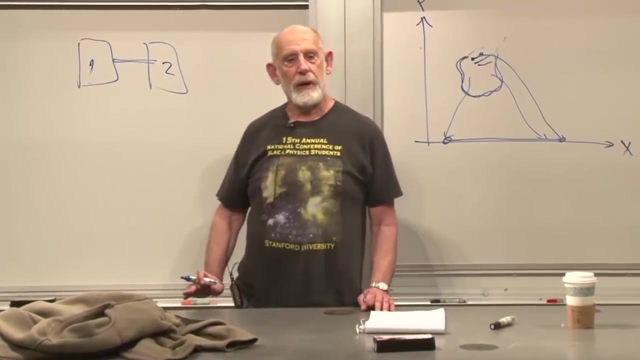 because their surfaces touch. typically surface area is small by comparison with volume. we'll come back to that. but in many, many contexts the energy of interaction between two systems is negligible compared to the energy of either of them. when that happens, you can say: to a good approximation. 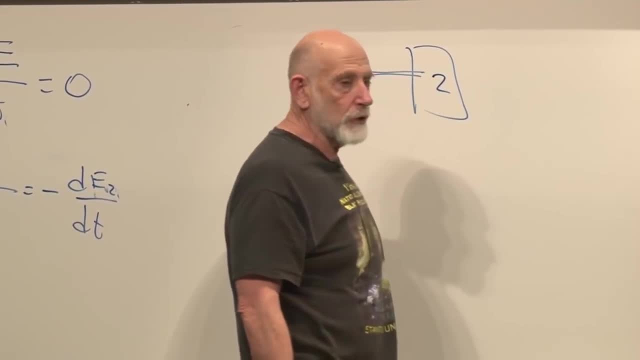 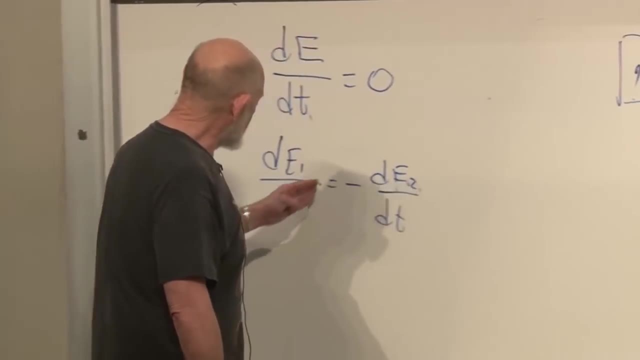 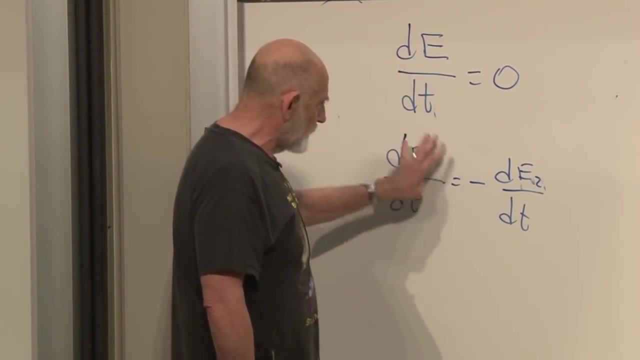 the energy can just be represented as the sum of two energies, of the two parts of the system, plus a teeny little thing that has to do with their interactions. and under those circumstances, the first law of thermodynamics- this is the top- is always true. the second: 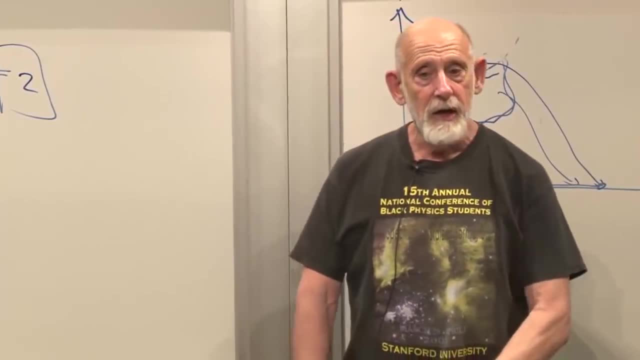 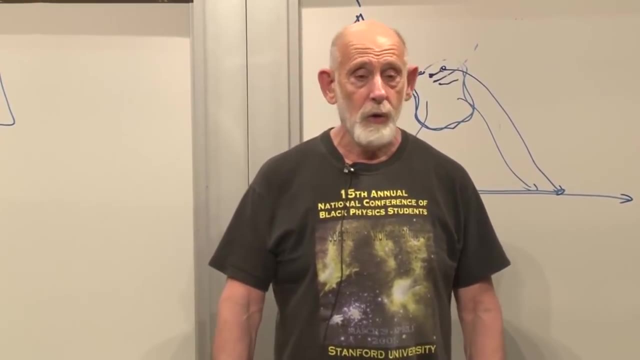 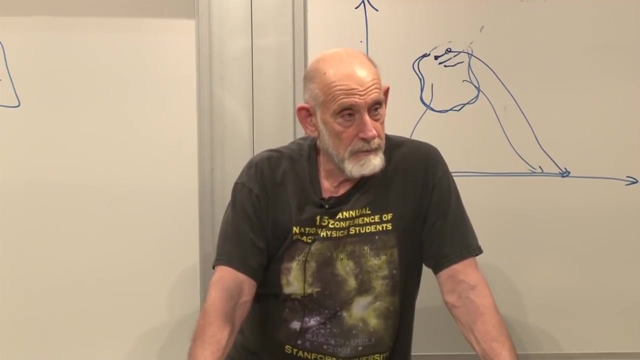 has that little caveat that we're talking about systems where energy is strictly additive, where you add energies. does everybody understand why I say you don't always add energies, that sometimes energies are not additive? we assume that we have the same possible problem with the probabilities. we assume that the outcomes were 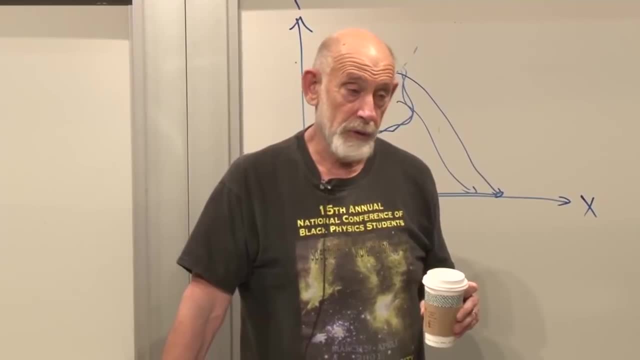 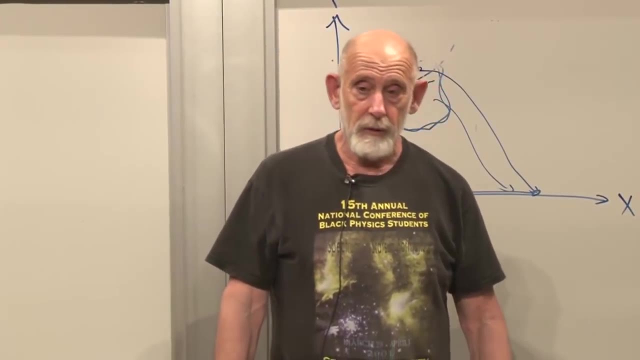 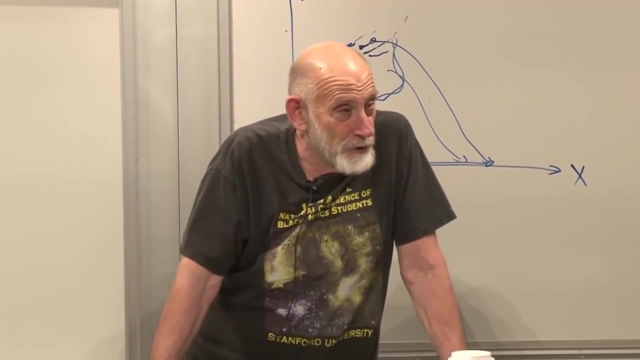 mutually exclusive. otherwise the sum law- well we do, otherwise the sum law doesn't work. yeah, okay. so in all the contexts which we've talked about, the dye: if it's yellow, it can't be red. you say orange, orange is both yellow and red. well, we don't count that way. 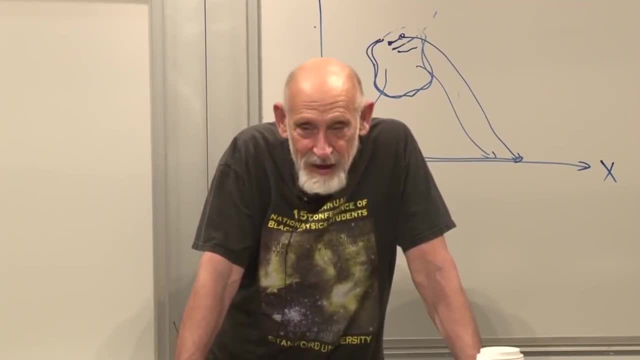 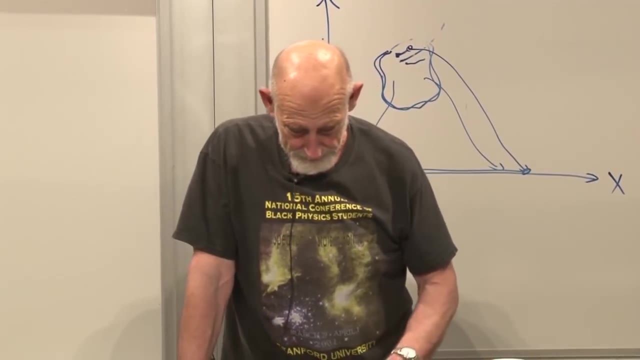 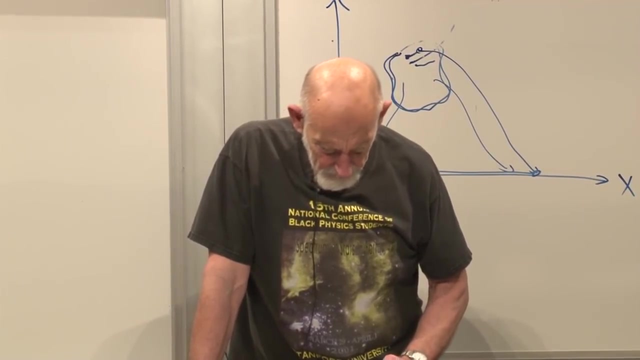 yeah, so that's correct. that's absolutely correct. we made the assumption that what I call states, what I call states, are mutually exclusive. absolutely okay, let's come back to entropy. we're not finished with entropy. we've done entropy. we've done energy. we haven't gotten to temperature yet. 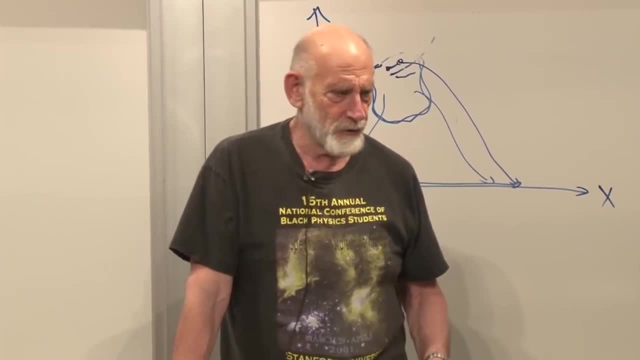 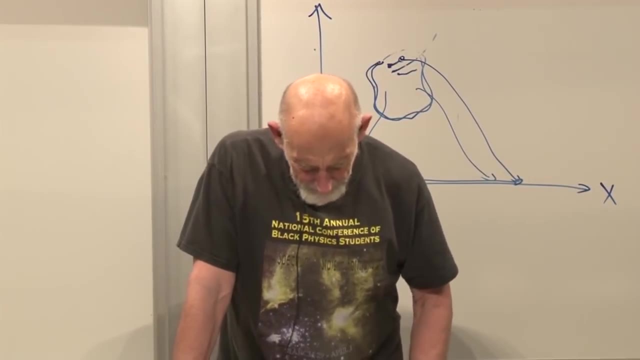 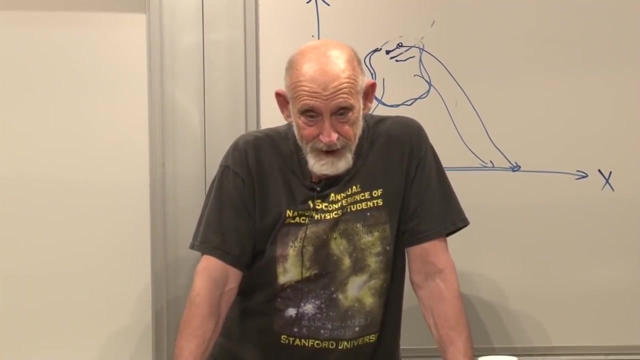 notice that temperature comes in behind entropy and even energy comes in behind entropy. but temperature is a highly derived quantity. by highly derived I mean it's a despite the fact that it's the thing you feel with your body, so it makes it really feel like it's something intuitive. 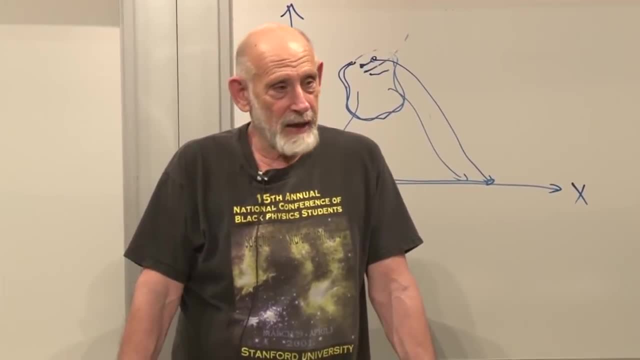 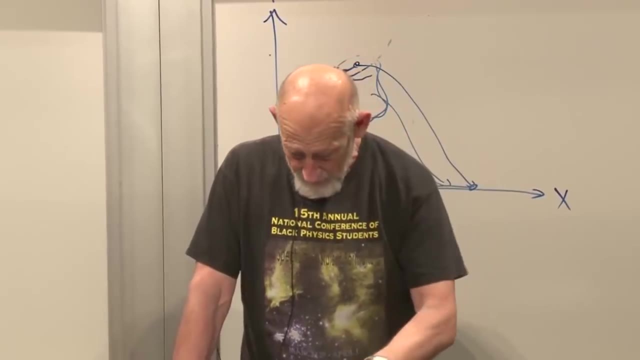 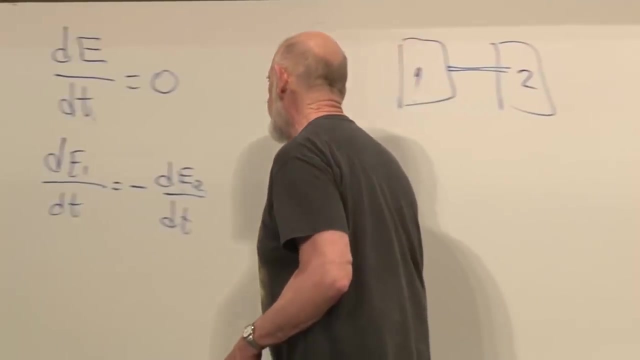 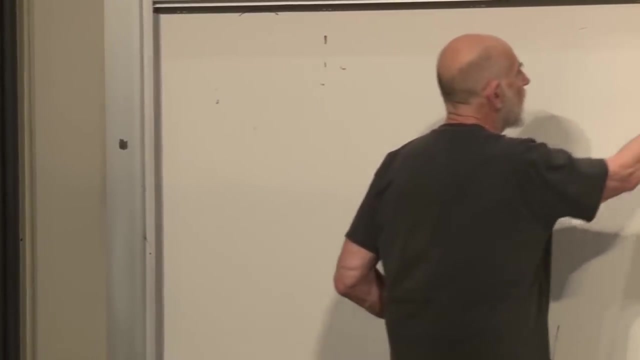 it is a mathematically derived concept, less primitive and less fundamental than either energy or entropy, but we'll come to it. let's come back to entropy. we defined entropy, but only for certain special probability distributions. let's lay out on the horizontal axis, just to be schematic. 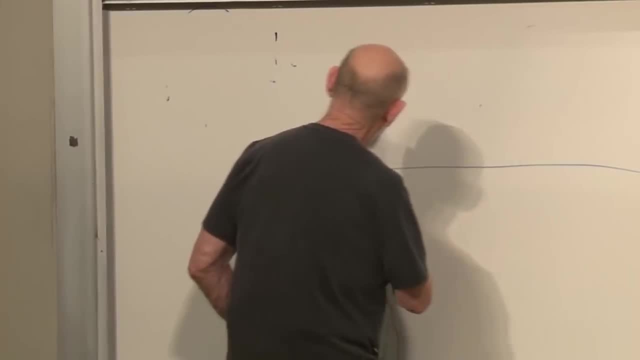 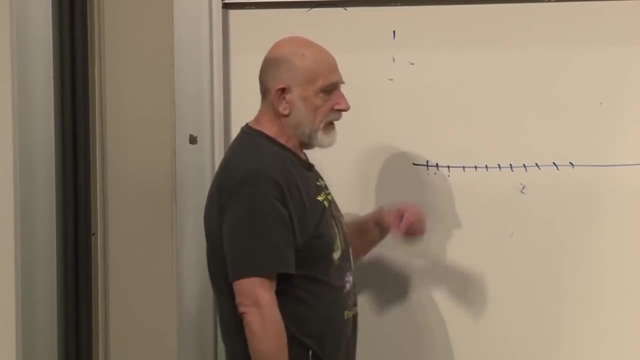 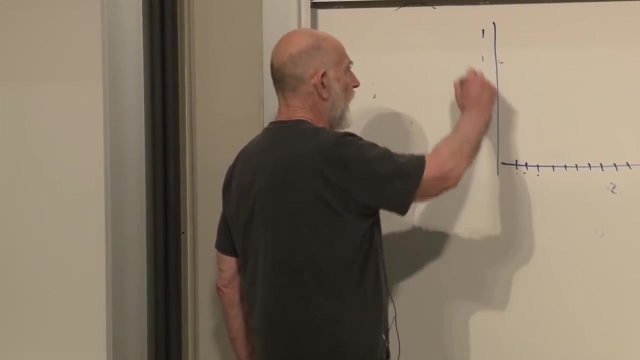 on the horizontal axis, we will put down all the different states: here's i equals one, here's i equals two, here's i equals three. this axis just labels the various states. and, of course, vertically, let me plot probability. okay, well, the probability, of course, is: 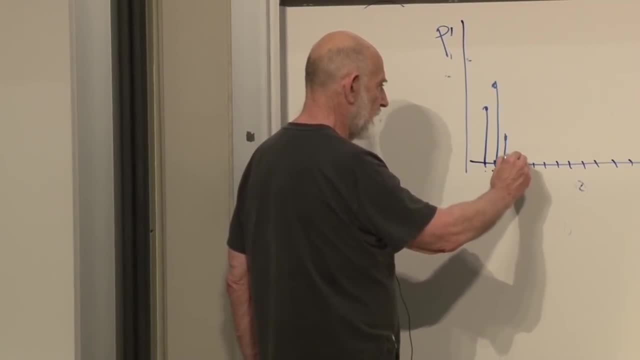 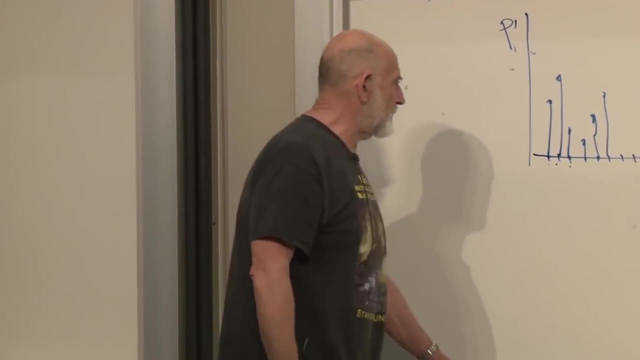 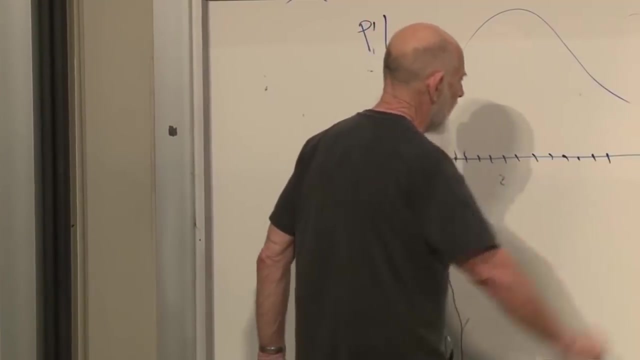 only defined on the, on the integers here. that's not very good. it's some probability, but let's, I don't want to have to draw such a complicated thing. every time I want to draw a probability distribution. let's just draw a graph. some probability distribution. 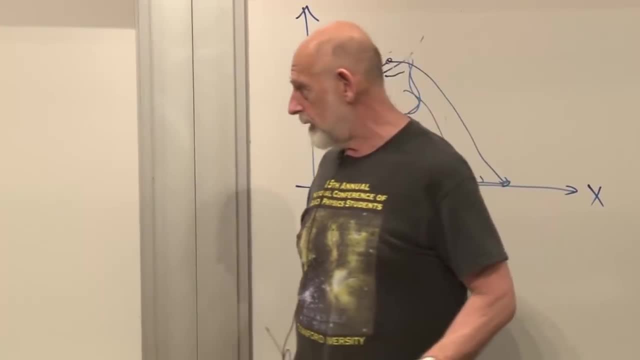 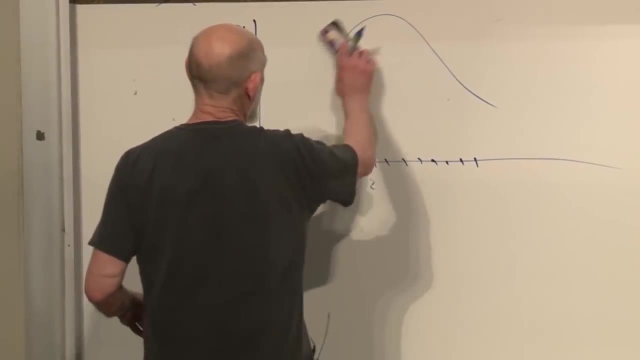 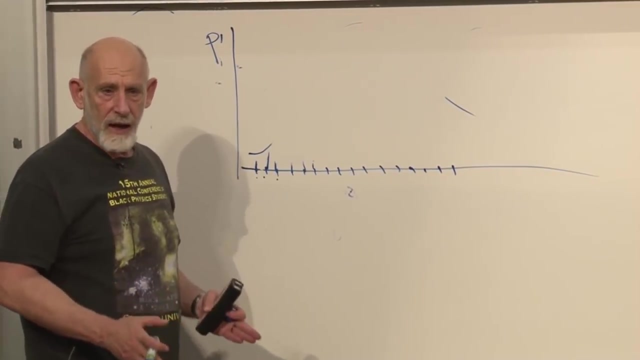 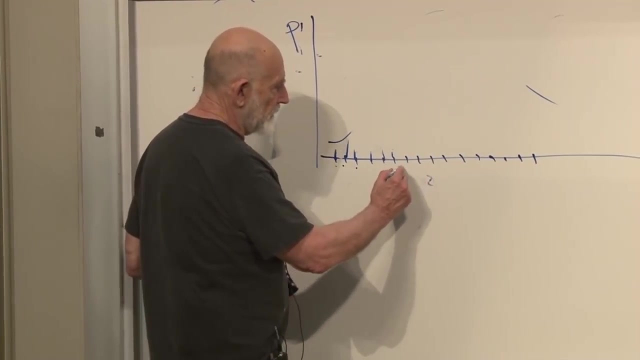 or some probability for each distribution. now, what we did was we defined entropy for a very special case, the special case being where some subset have equal probabilities and the rest have zero probability. for example, if our subset consists of this group over here of m, the whole group being n. 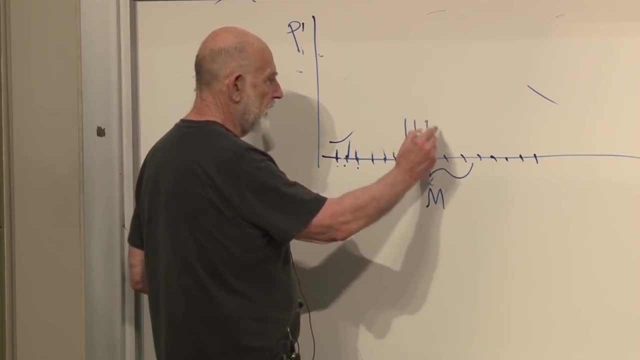 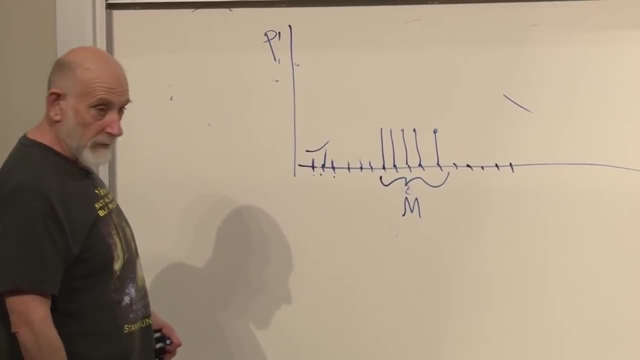 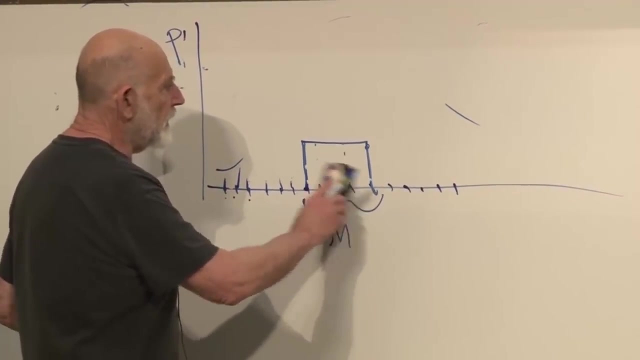 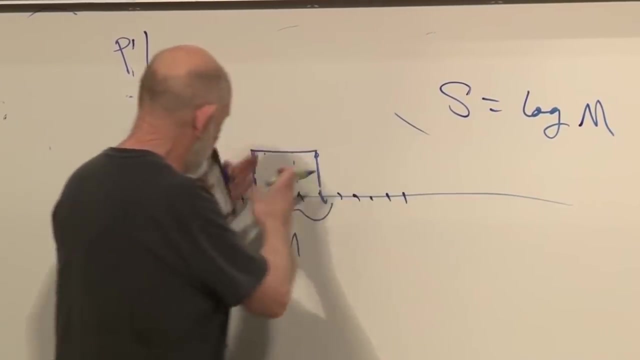 then all of these have the same probability and their probabilities have to add up to one, so the probability is one over n. we'll just draw that. by drawing a box like that, then we define the entropy to be the logarithm of the number of states in here. 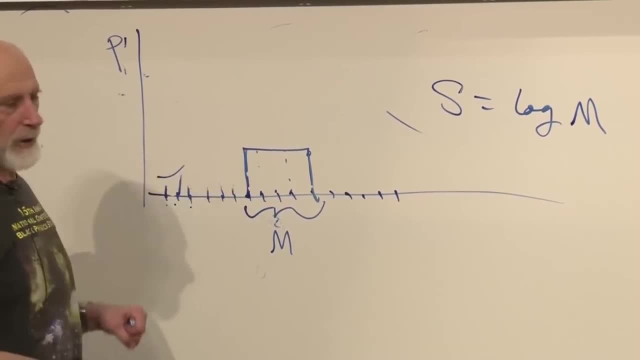 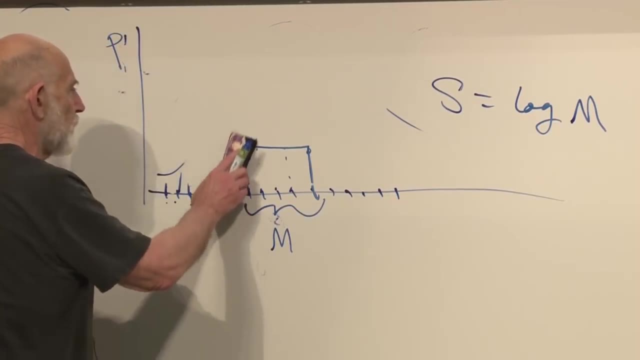 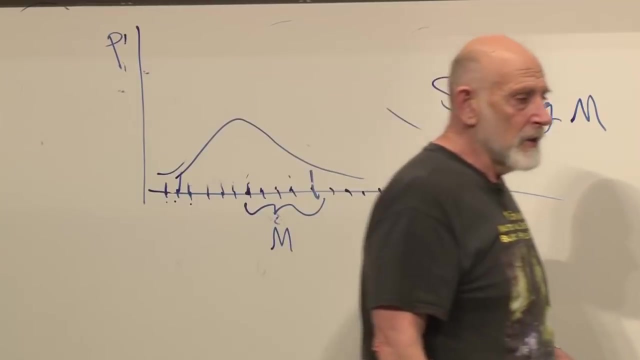 generally speaking, we don't have probability distributions like this. generally speaking, we have probability distributions which are more complicated. in fact, they can be anything as long as they're positive and all add up to one. so the question is: how do we define entropy in a more general context? 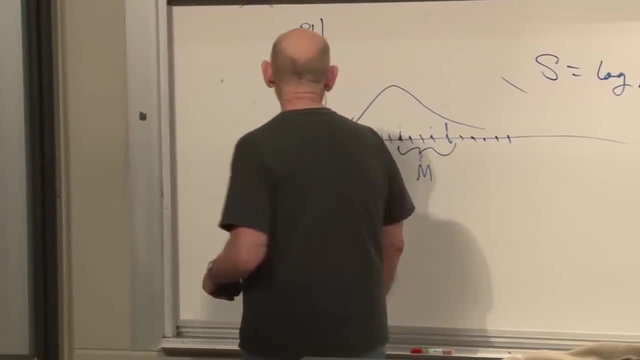 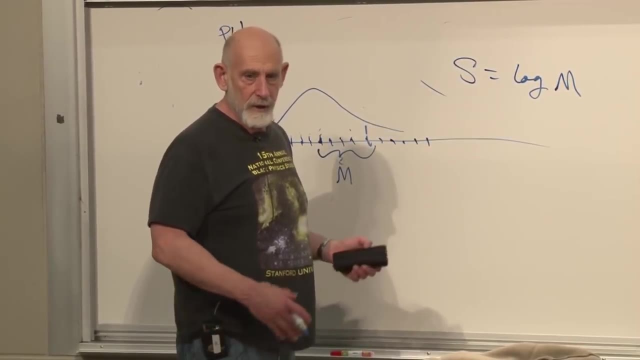 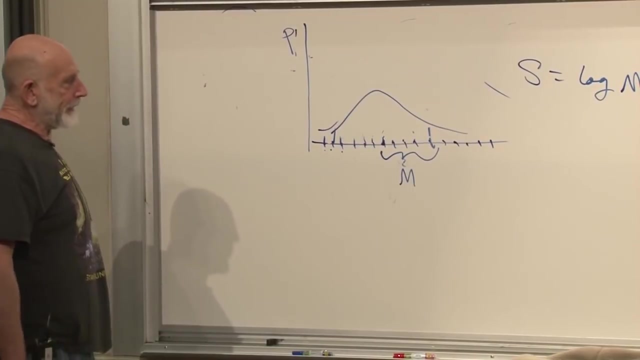 where the probability distribution looks like this. I'm going to write down the formula and then we're going to check that it really gives this answer when it should give this answer. and for today, I'm just going to write it down and tell you this is the definition. 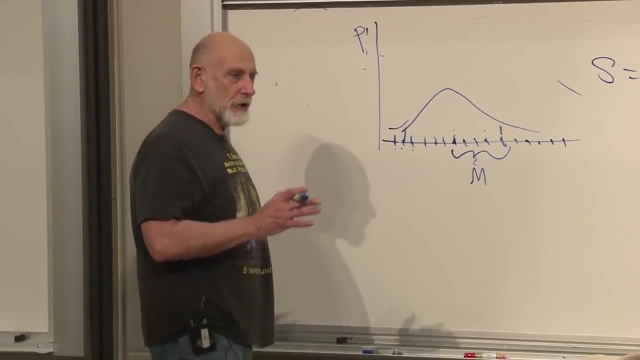 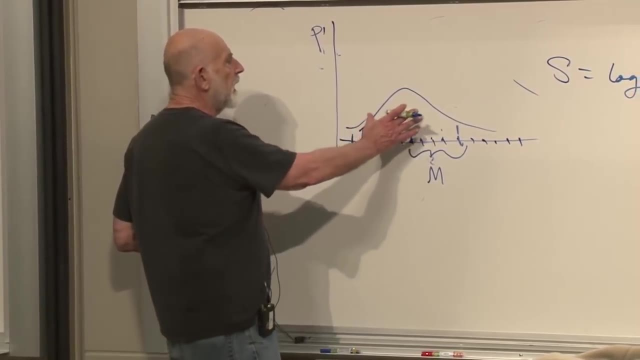 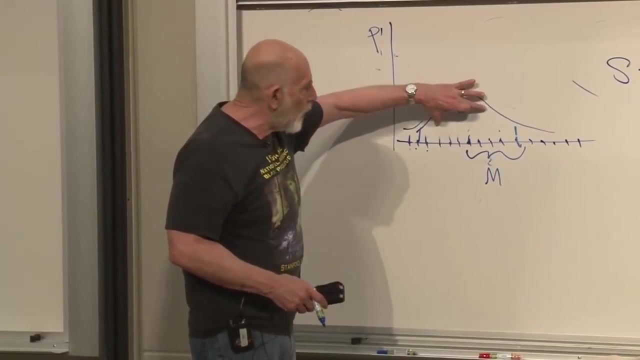 you'll get familiar with it and you'll start to see why it's a good definition. it's representing something about the probability distribution, and what it's representing is, in some average sense, the average number of states which are importantly contained inside the probability distribution. the narrower the probability distribution. 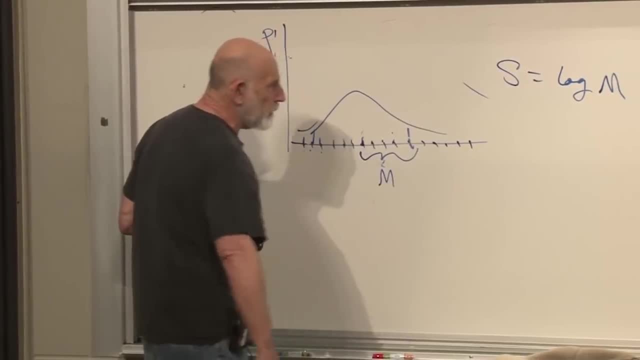 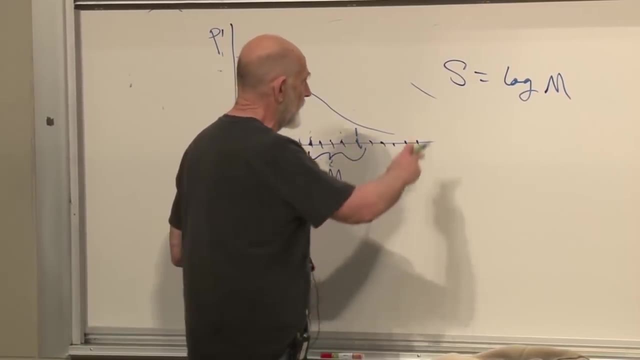 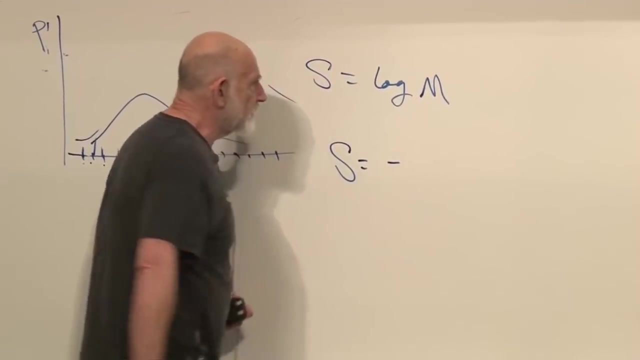 the smaller the entropy will be. the broader the probability distribution, the bigger the entropy will be. I'll write it down for you now. we'll write it down and then explore it just a little bit. tonight S for a general probability distribution is first of all minus. that's funny, because this is positive. 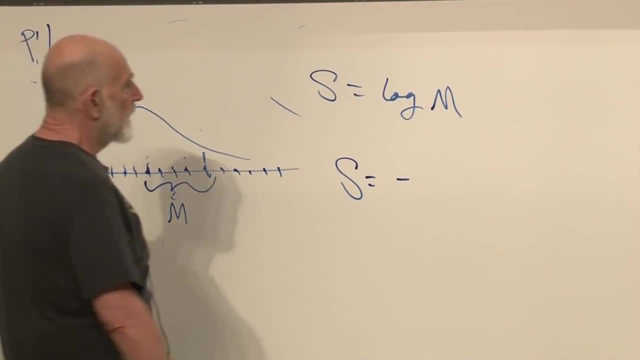 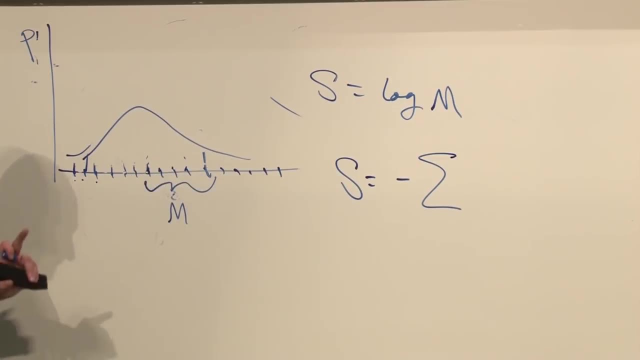 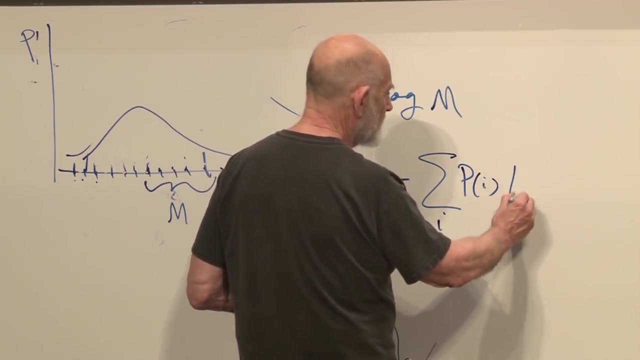 but nevertheless the formula begins with minus a sum and it's a sum over all of the states, all of the possibilities, so it's a sum over i. there's a contribution for each place. here, the probability of i times the logarithm of the probability of i. 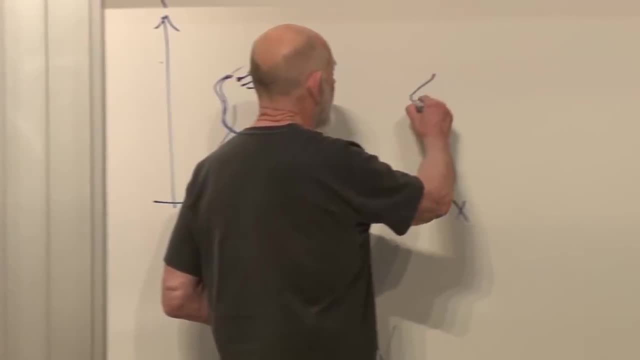 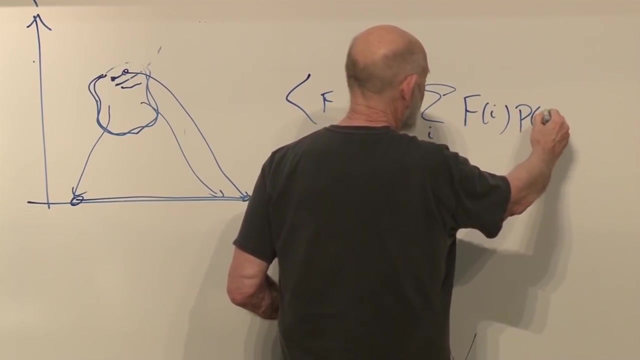 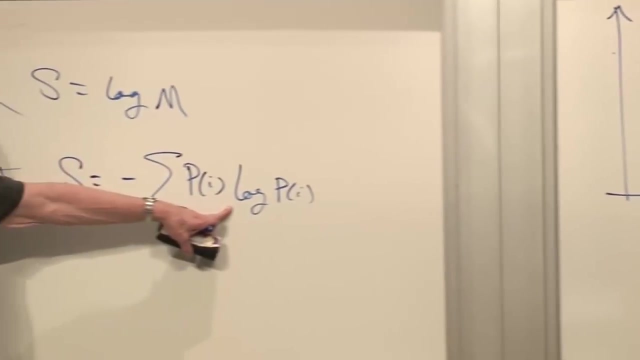 do you remember- let's write something else down- do you remember that the average of f is equal to the summation over i? f of i times p of i? this is actually the average of log p sub i. it's the average of log p sub i. 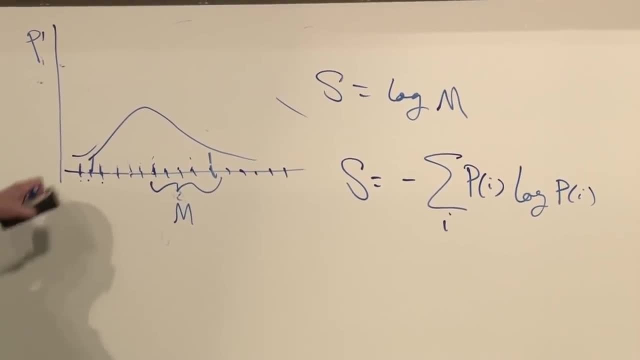 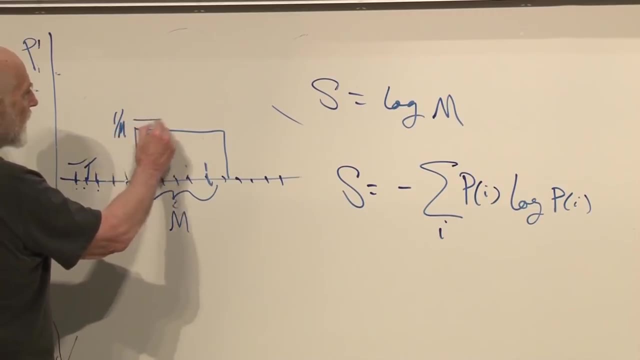 alright, let's work this out, let's see what this gives. in the special case where the probability distribution is one over m for m squared, it has two states all together. it has with m and because it has with m, it must have height one over m, because all the probabilities have to add up to one. 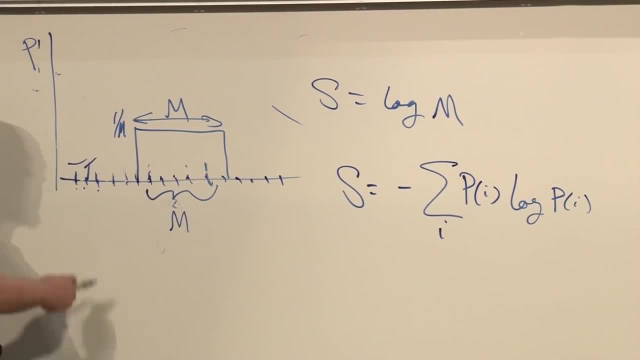 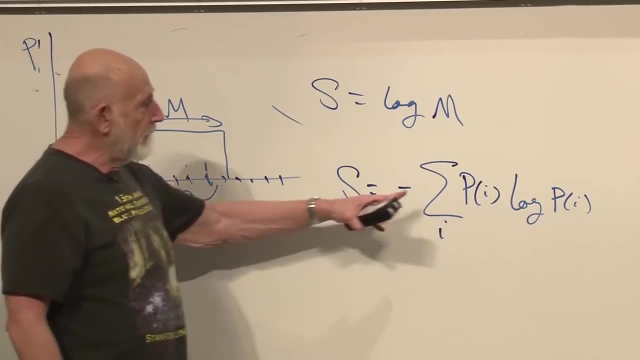 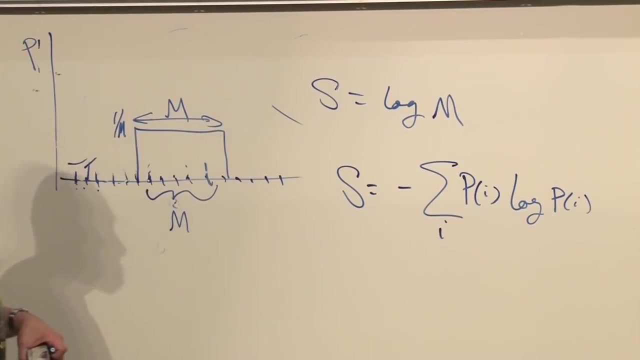 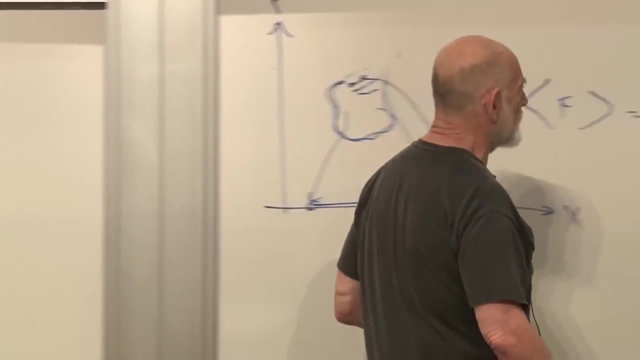 alright, so let's work this out. let's take the contribution for all the unoccupied states. from all the unoccupied states, p sub i is zero, so you get nothing. yeah, that's right. so now what's the alright good? so let's consider the limit of p. 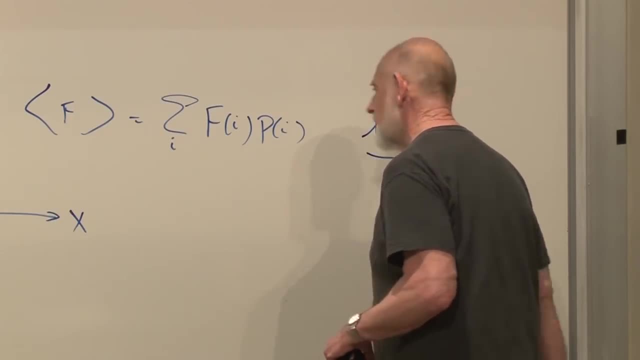 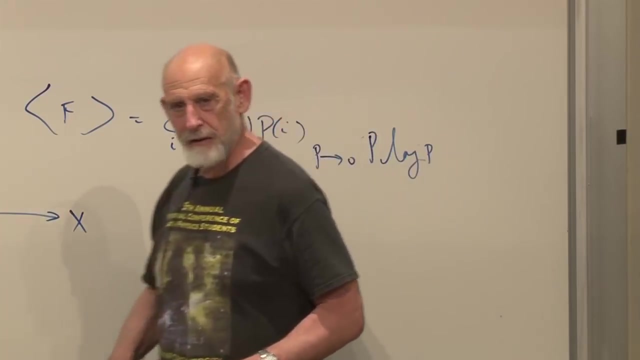 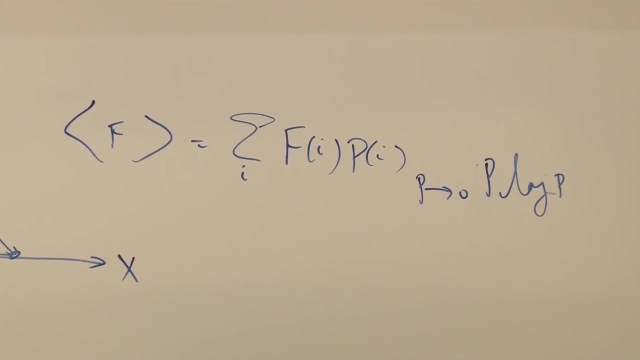 sorry- of log p over p, or let's just say the limit of- no, that's not right. the limit of p log p, as p goes to zero. you know how to calculate that. ok, I'm going to leave it to you. it's a little calculus exercise. 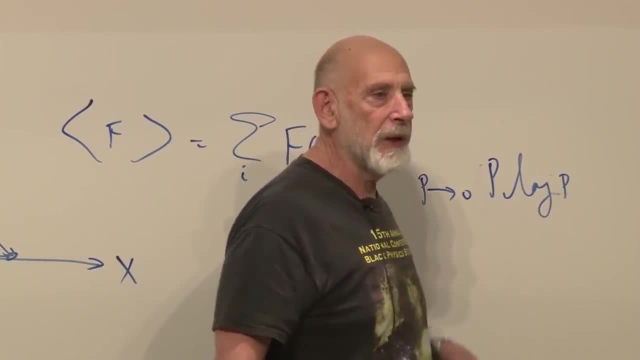 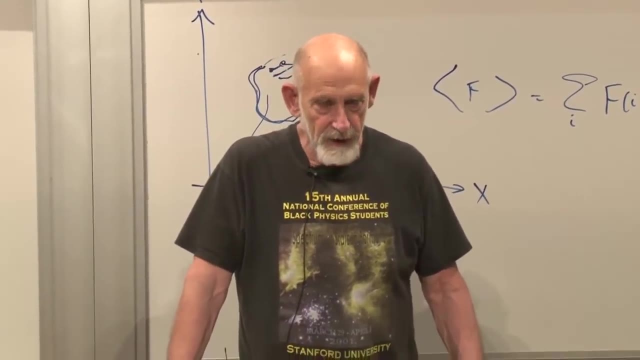 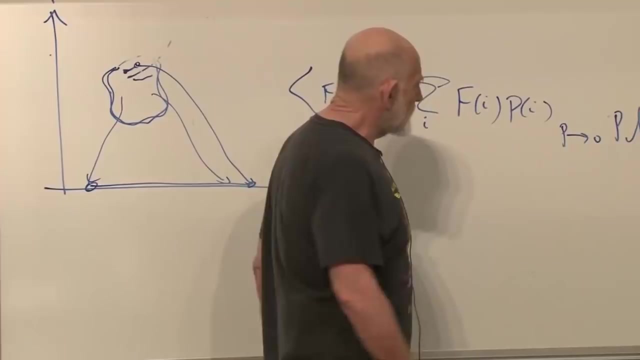 to calculate the limit as p goes to zero of p. log p at zero. the point is that p goes to zero a lot faster than log p goes to infinity. log p as p goes to zero is very slow. p goes to zero fast, so this goes to zero. 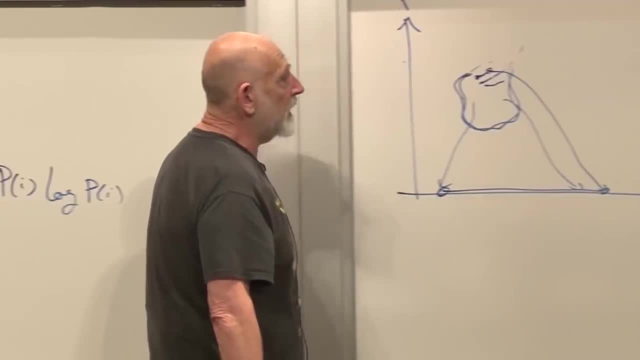 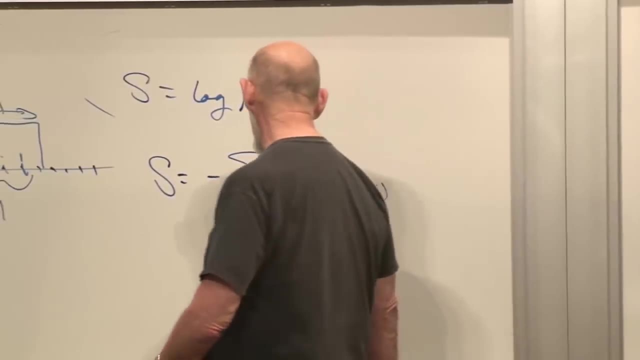 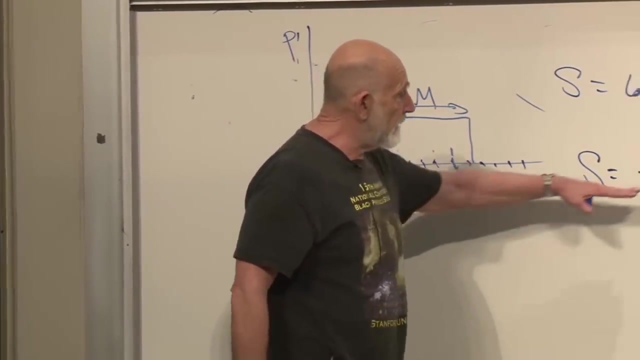 you're absolutely right, though that has to be shown. log p in the limit that p goes to zero is zero. so with that piece of knowledge, the contribution from states with very, very small probability will be very, very small. and as the probability for those states goes to zero, 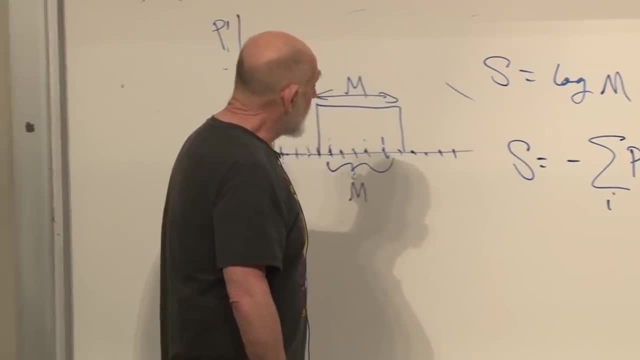 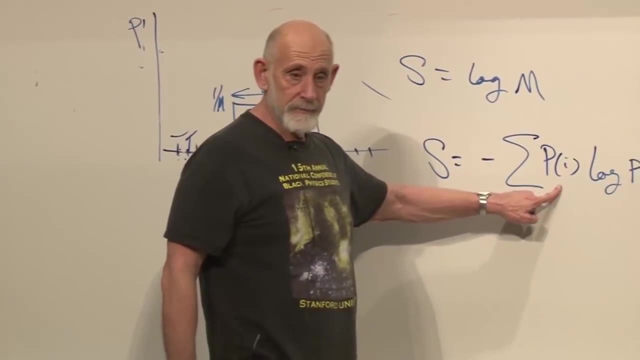 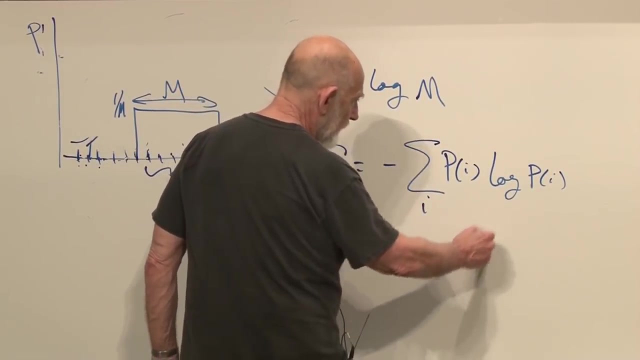 this quantity, the contribution will go to zero. but what about the ones here which have significant probability? they all have the same p sub i and they all have the same log p, log p sub i, log p sub i. the log p sub i is logarithm of one over m. 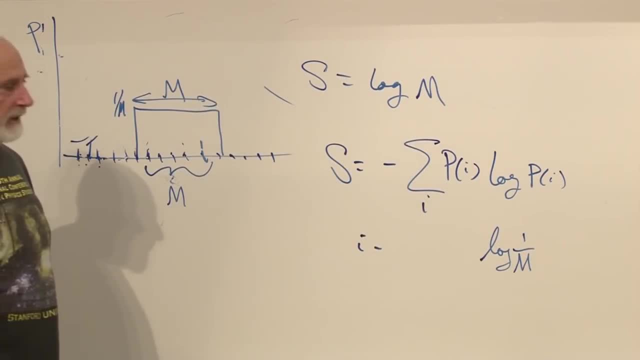 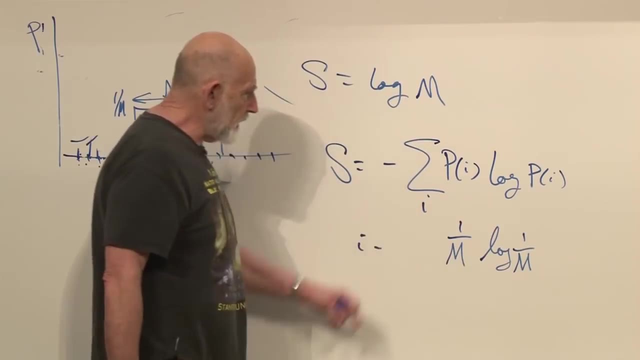 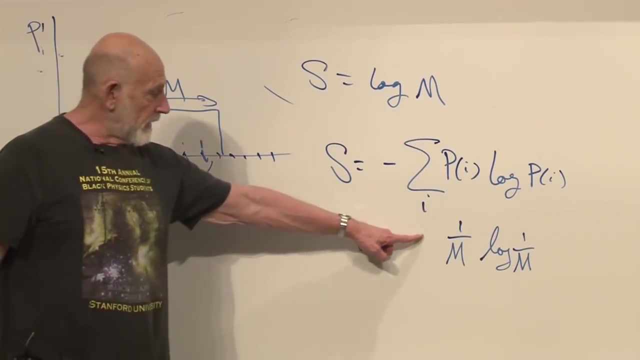 for all of them. the p sub i is also one over m, not log one over m, but one over m. so each contribution is one over m times log one over m. how many contributions are there like that? alright, so we multiply by m and get rid of. 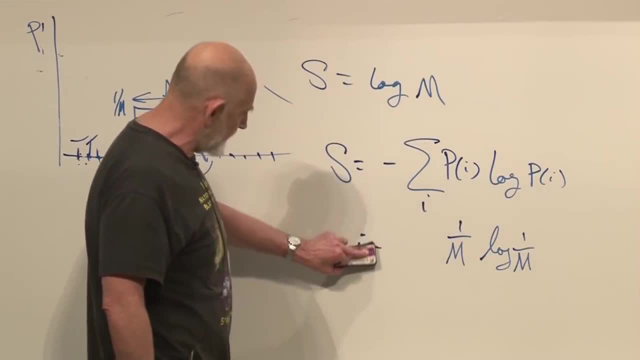 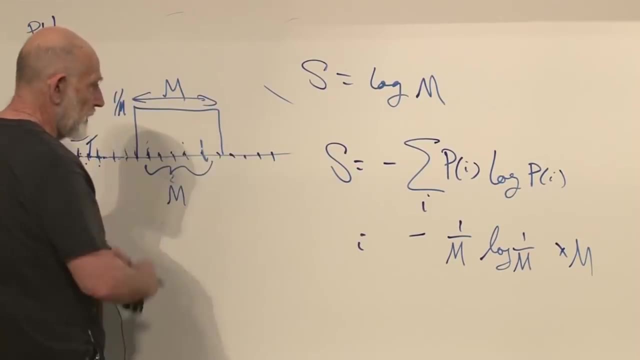 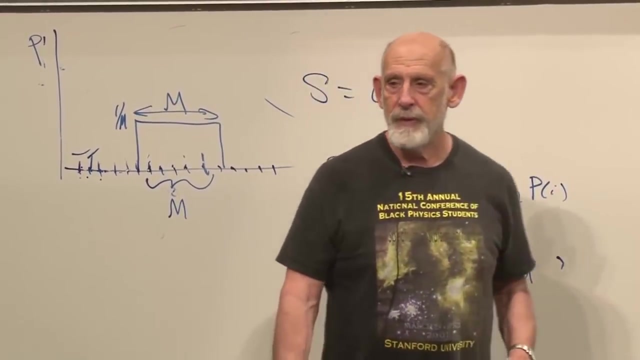 the one over m there. there's a minus sign here. carry it along all times m because there are m such terms. so the one over m cancels and we're just left with log one over m. what's log one over m? minus log m, right? so that's why the minus sign was put there. 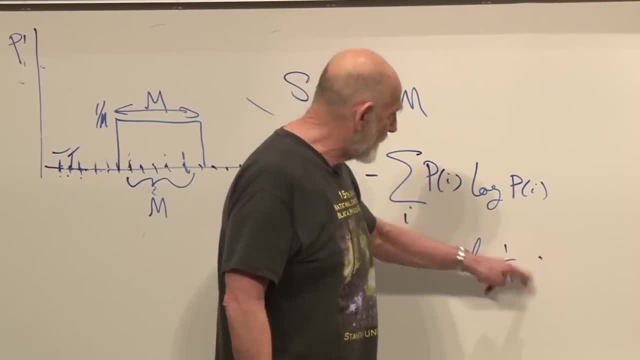 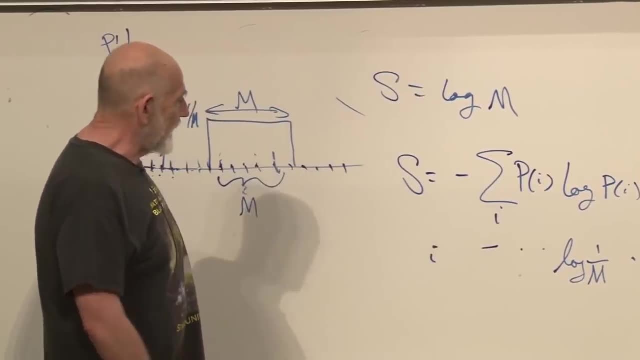 in the first place. there's no miracle the minus sign was put there. there's a less than one, and so the logarithms of them are always negative. so you soak up that negative with an overall negative sign and entropy is positive. but this is exactly the same. 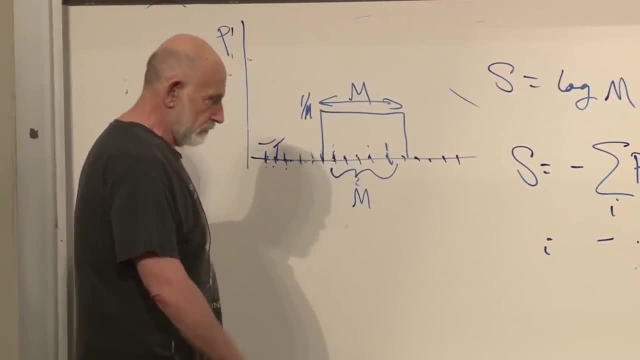 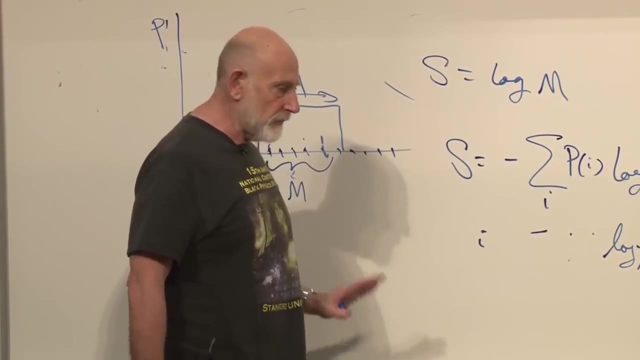 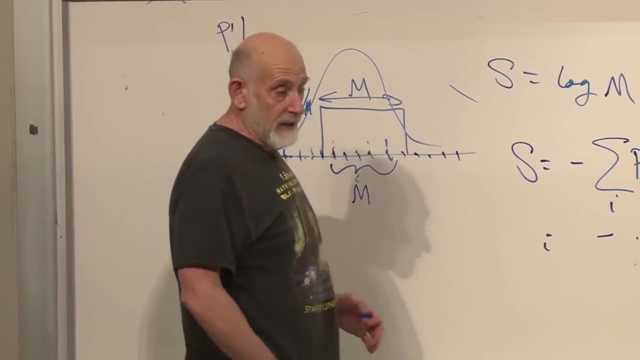 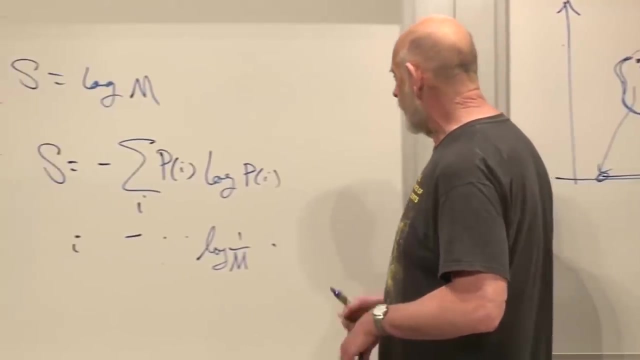 answer that we, or by the original definition, just s equals log m, logarithm of the number of states. but this is a definition now that makes sense even when you have a more complicated probability distribution, and it is a good and effective. it's the average of log p. 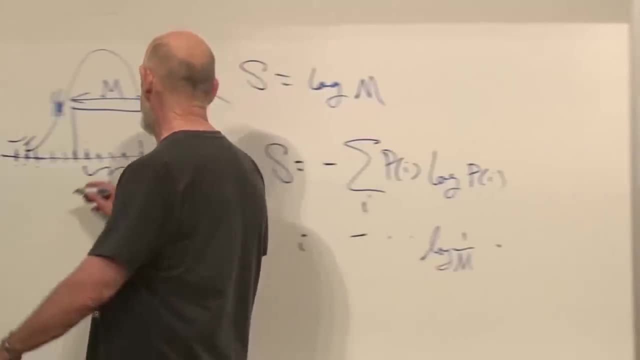 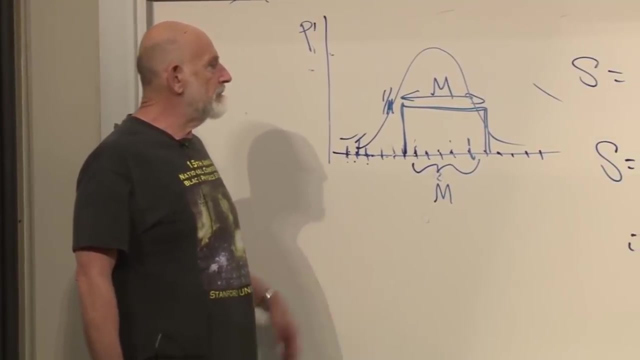 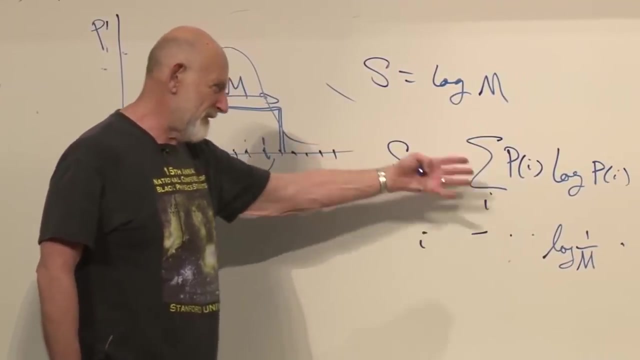 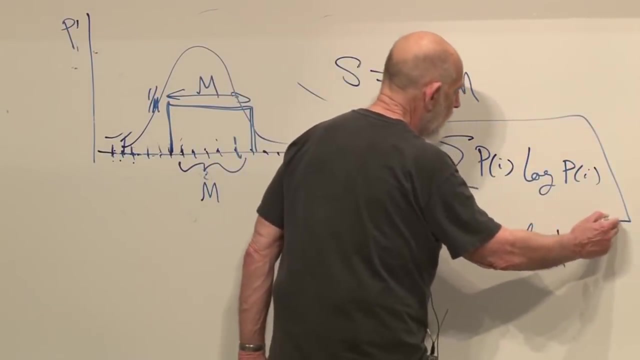 for the special case where the probability distribution is constant, like this, then all of the probabilities in here are one over m, and calculating the average of one over m, well, it's just log. one over m just gives you this. so this is the general definition of the entropy. 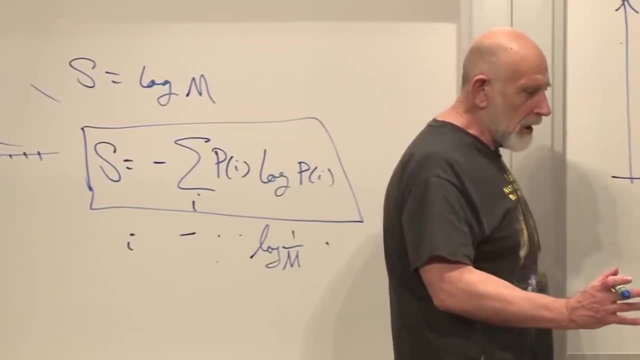 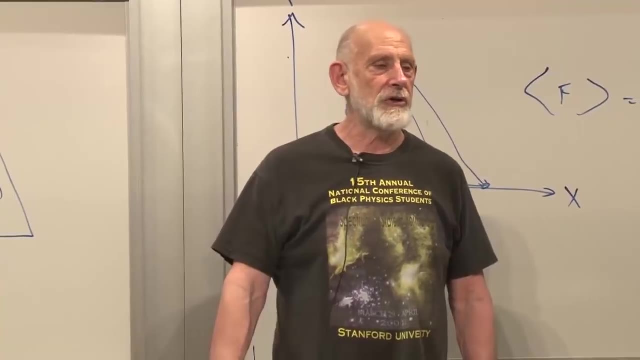 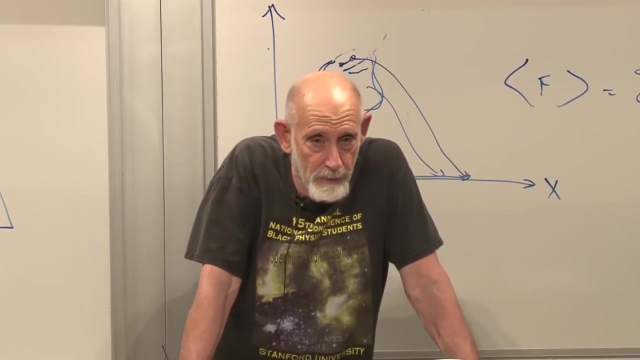 that's associated with a probability distribution. and notice, entropy is associated with a probability distribution. it's not a thing like energy, which is a property of a system. it's not a thing like momentum, it's a thing which has to do with a specific probability distribution. probability distribution on. 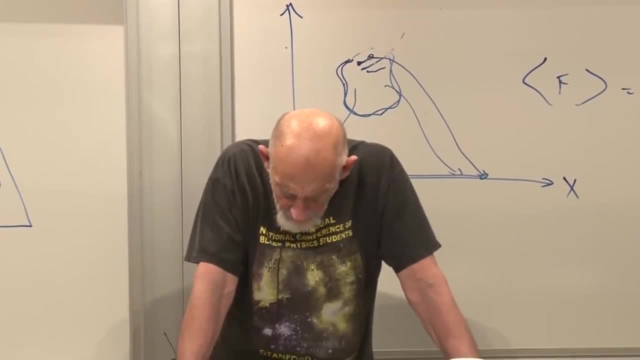 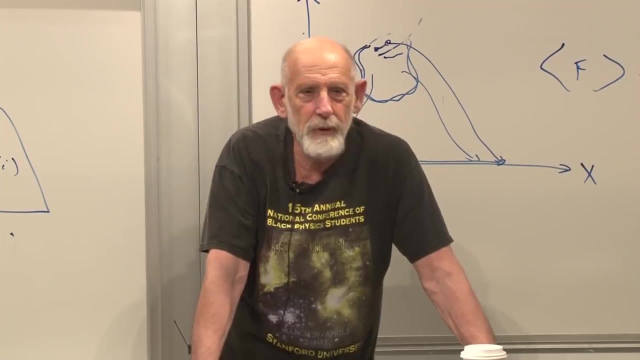 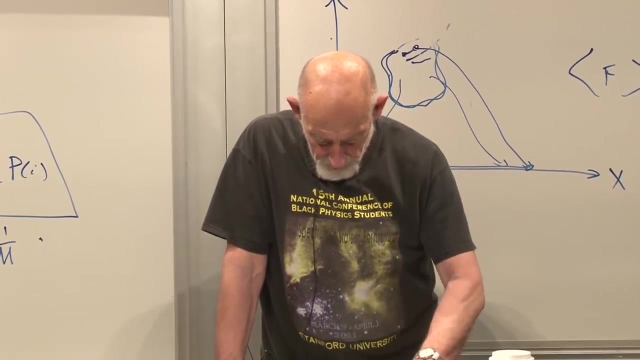 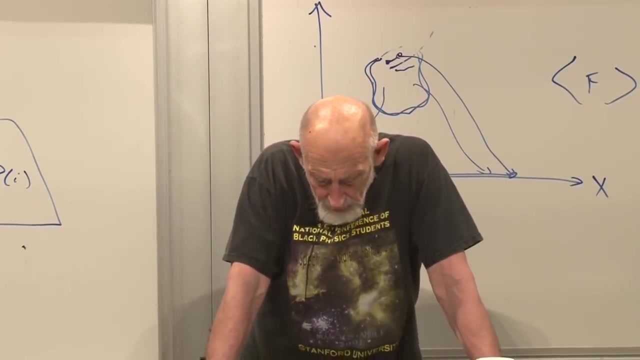 the space of possible states. so that's why it's a little bit of a more obscure quantity from the point of view of intuitive definition. as I said, it's definition has to do with both the system and your state of knowledge of the system. let's do. 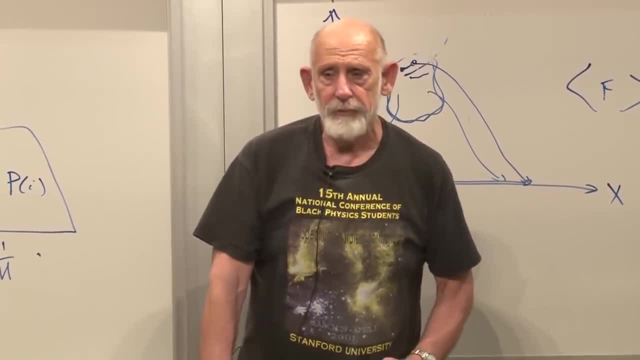 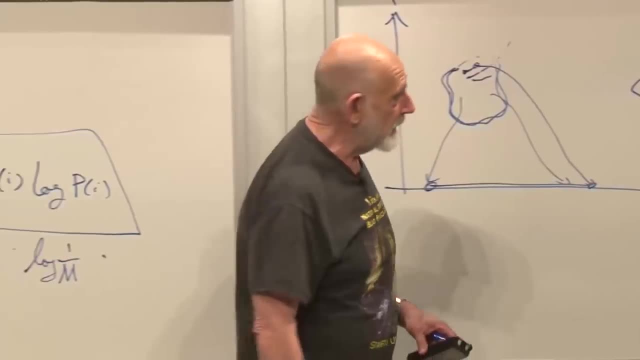 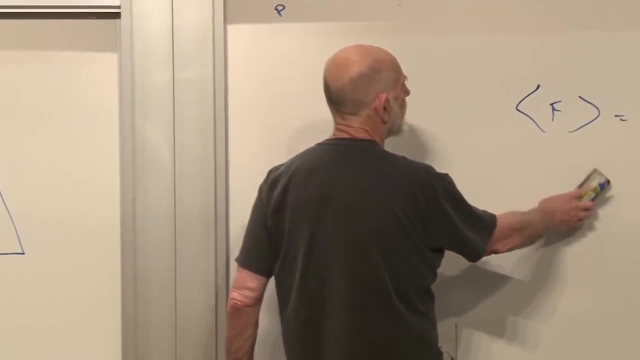 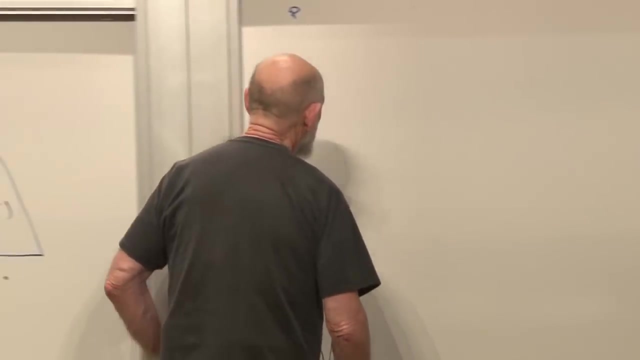 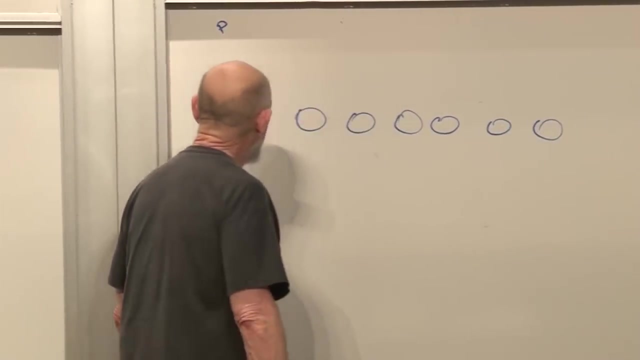 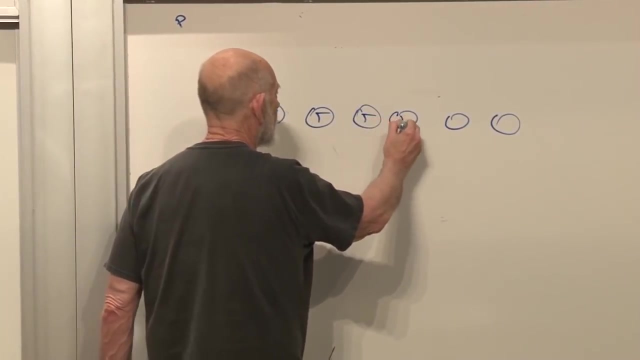 some examples. let's calculate some entropy for a couple of simple systems. our first system is just going to be not a single coin but a lot of coins, so we have capital N coins, n of them, and each one can be heads or tails, et cetera. 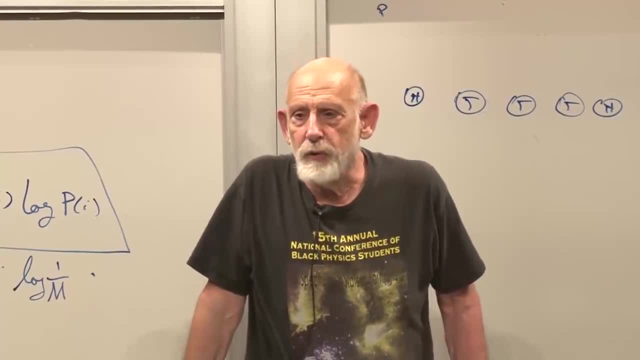 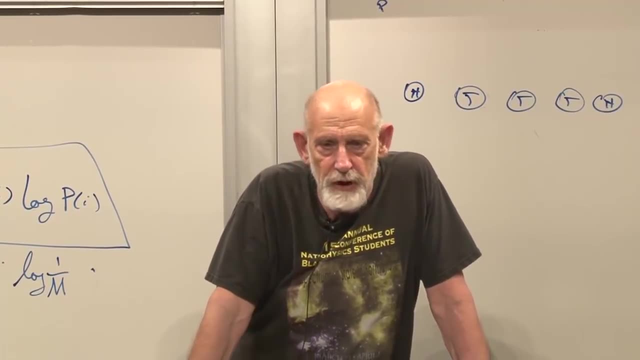 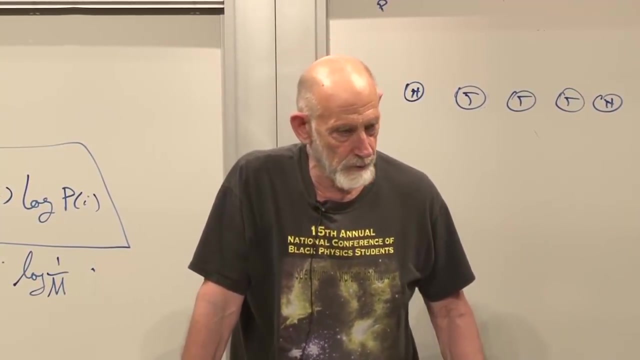 and so on. as a matter of fact, we have no idea what the state of the system is. we know nothing. the probability distribution, in other words, is the same for all states. complete ignorance, absolute ignorance. what is the entropy associated with such a configuration? there are N of these. 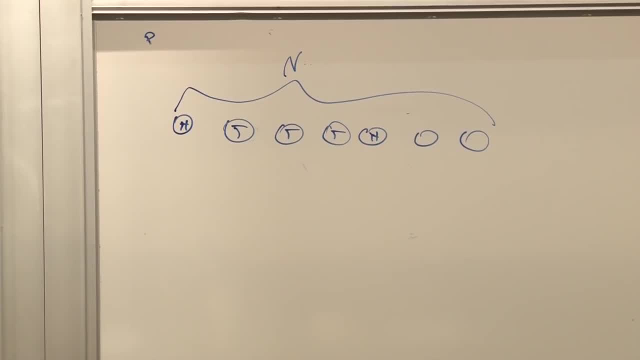 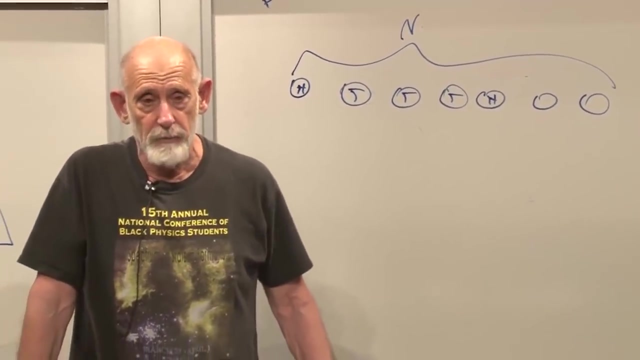 all the probabilities are equal. under the circumstance where all of the probabilities are equal, we just get to use logarithm of the number of possible states. the answer here is the logarithm of the number of total states. how many states are there all together? two to the N. 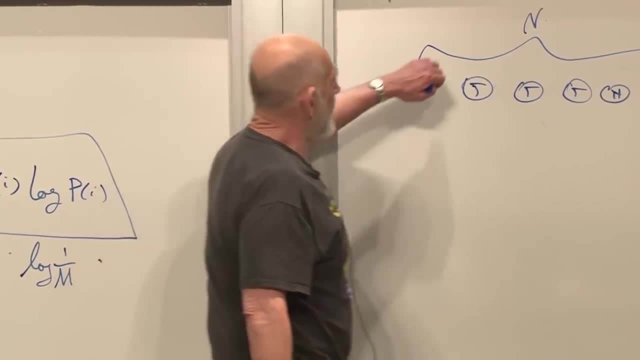 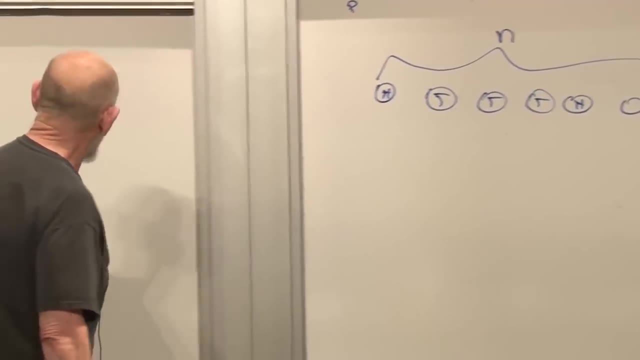 right two to the N. oh, let's. I'm sorry, I'm going to change definitions for a minute. you'll see in a minute I'm going to call this little n. number of coins is little n over here. big N stood for the total. 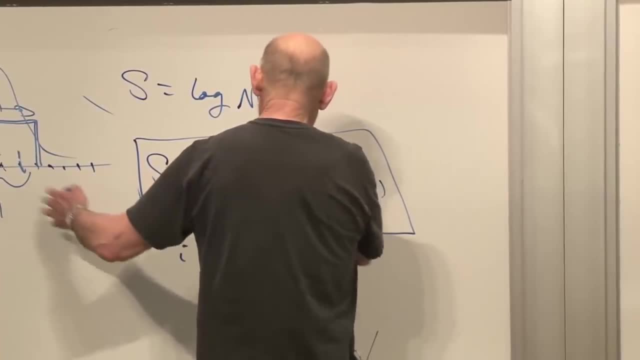 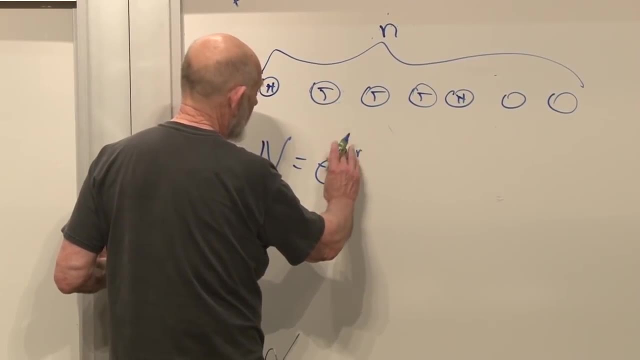 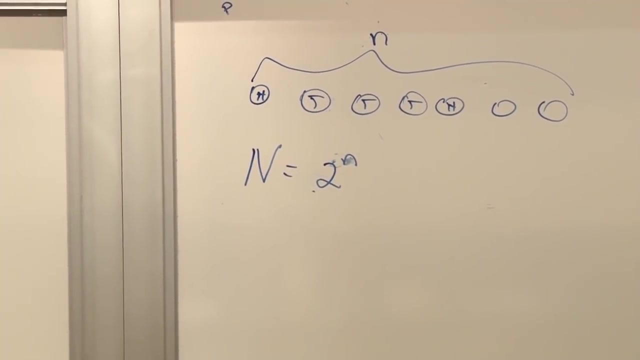 number of states. so if I match terminologies- big N- the total number of states is E to the two N, no, two to the N. sorry, I'm getting tired. two to the N, two to the N states. all together two states for the first coin. 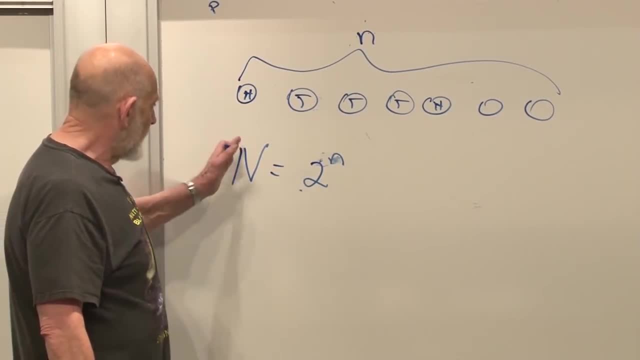 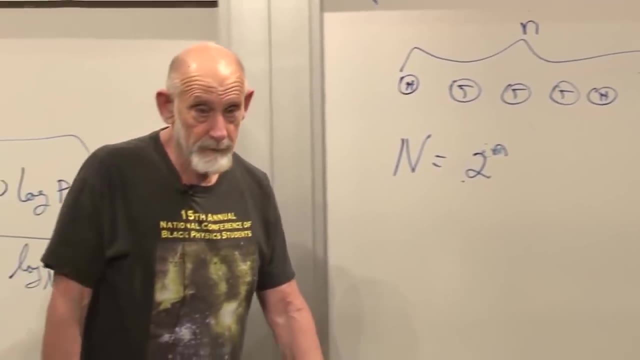 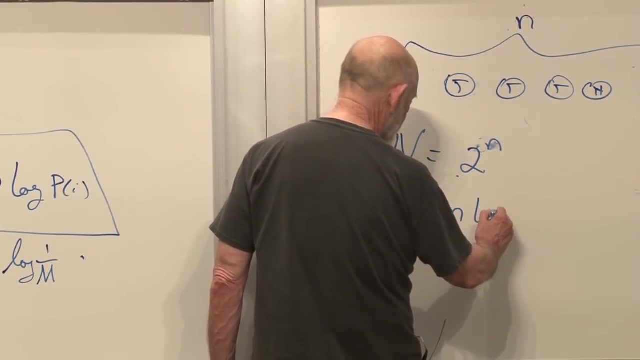 two states for the second coin, and so forth. two to the N all together, and the total number of states is capital N. what's the entropy, given that we know nothing? two log N, N log two S is equal to N log two. that's the logarithm of 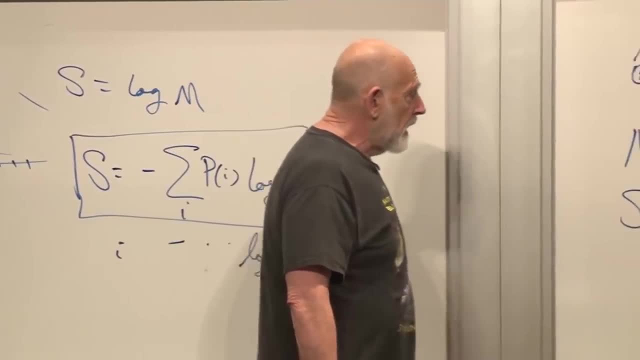 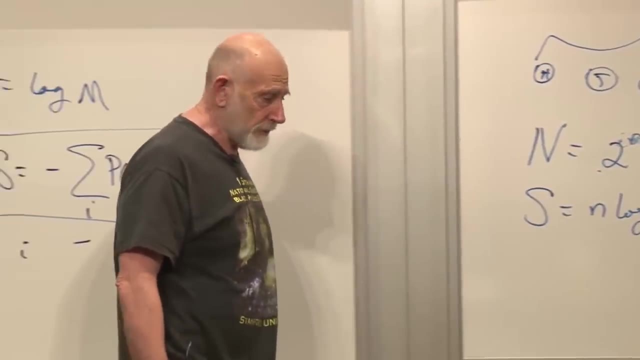 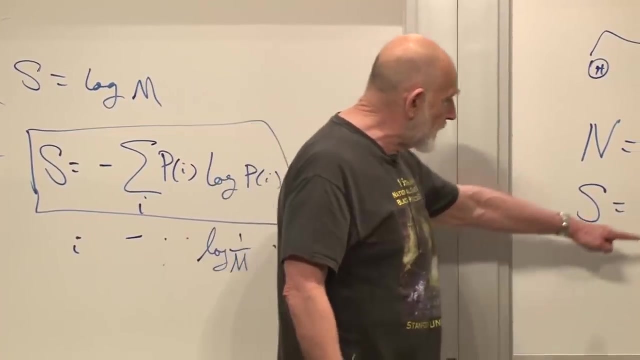 two to the N. so here we see an example of the fact that entropy is kind of additive over the system. it's proportional to the number of degrees of freedom, in this case N times log two, and we also discover a unit of entropy, the unit of entropy. 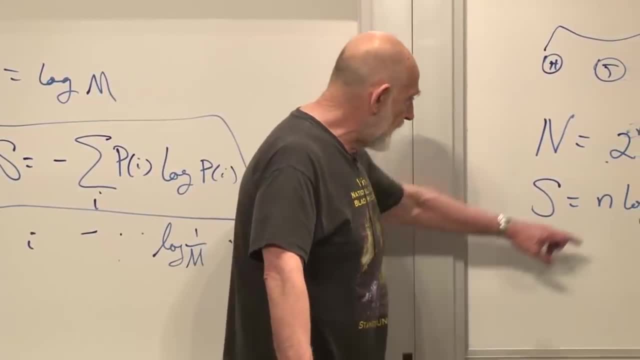 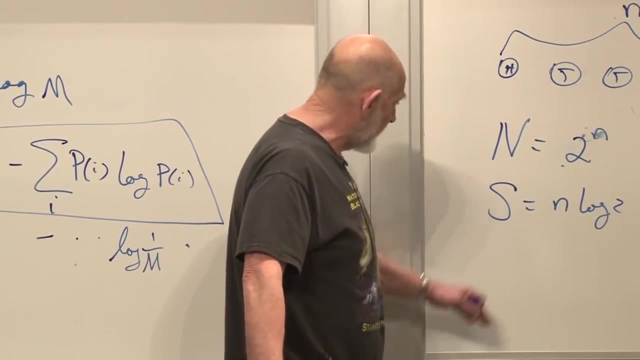 is called a bit. that's what a bit is in information theory. it's the basic unit of entropy for a system which has only two states, up or down, heads or tails or whatever. the entropy is proportional to the number of bits, or, in this case, 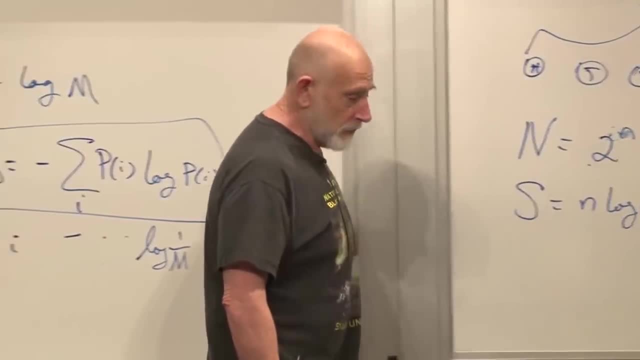 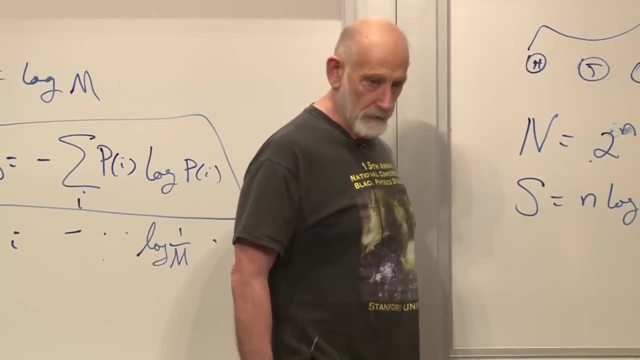 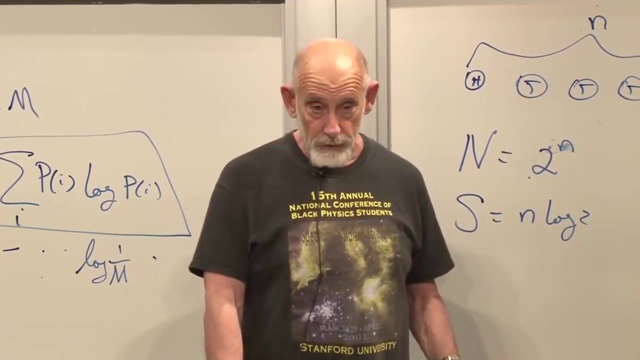 the number of coins times the logarithm of two. so log two plays a fundamental role in information theory as the unit of entropy. it does not mean that in general that entropy is an integer multiple of log two. we'll see in a second. it doesn't mean that 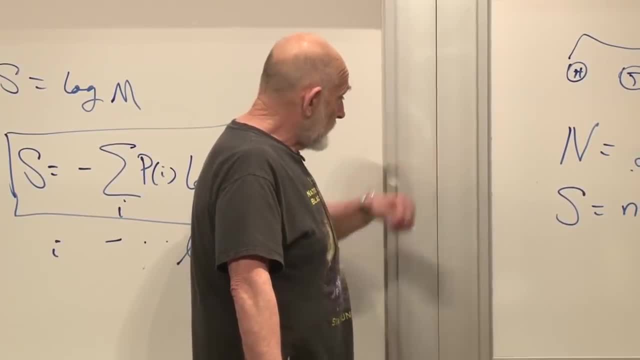 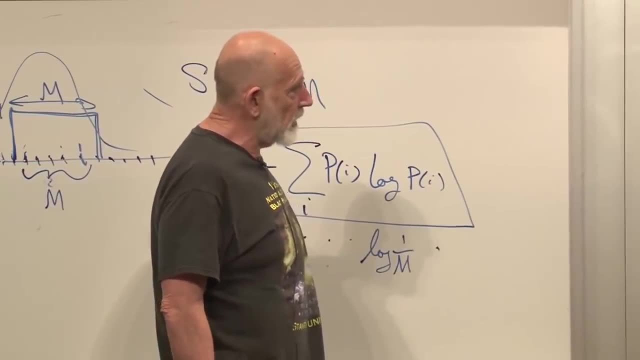 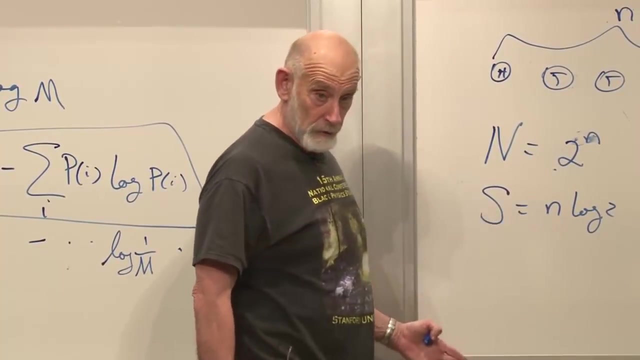 um, okay, so that's, that's this case over here. let's try another case. let's try another state of knowledge here. our state of knowledge was zilch. we knew nothing. this is the maximum entropy. maximum entropy, logarithm of capital N, or logarithm of two to the little n. 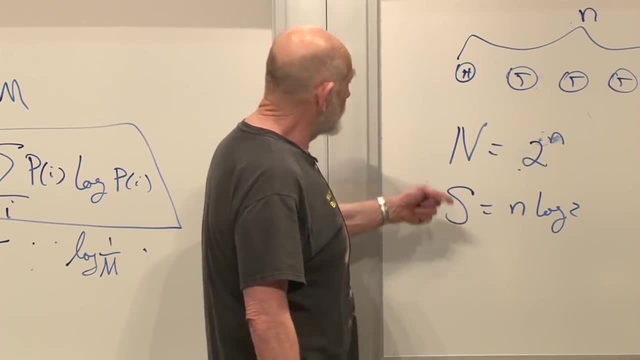 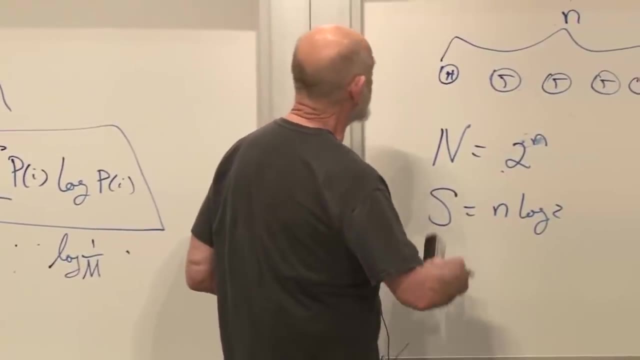 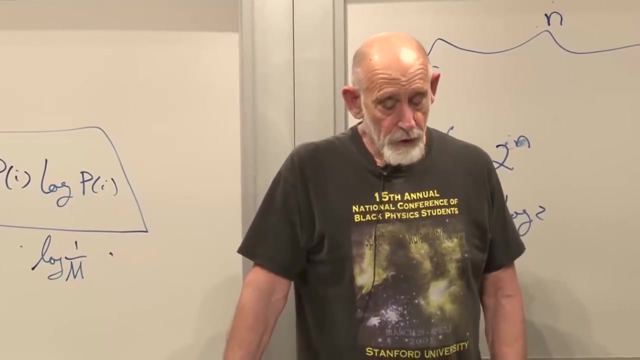 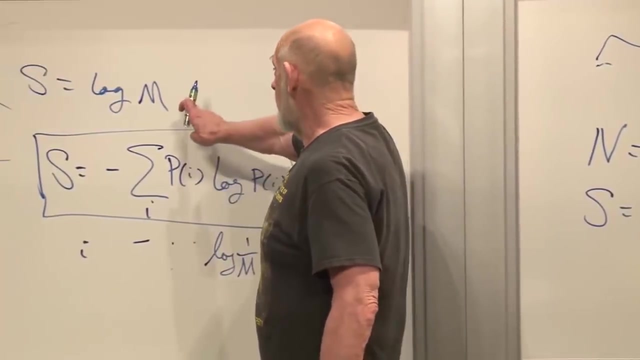 which is N log two. one bit of entropy for each coin, if you like. okay, let's try something else. let's try a state in which what we know is, oh, something else, supposing we know the state completely. another word. that's the case where M is equal to one. 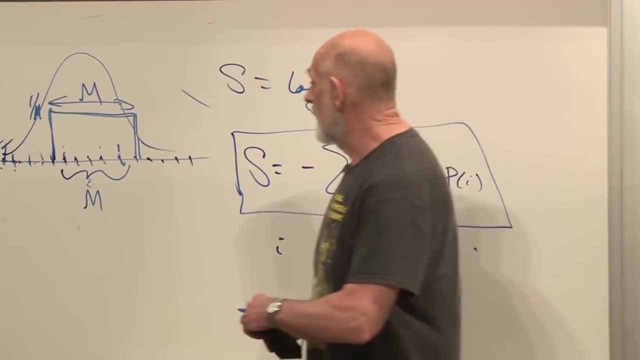 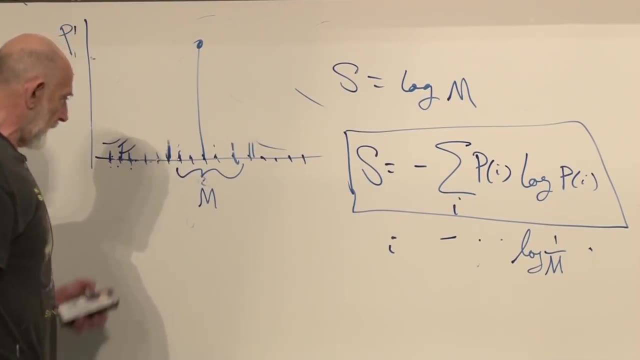 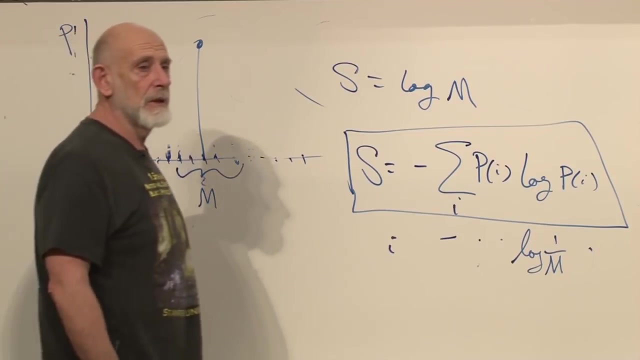 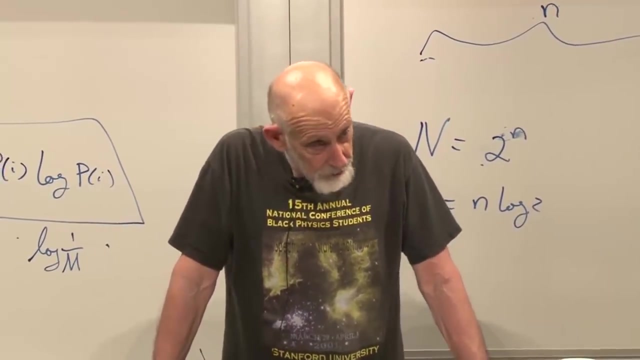 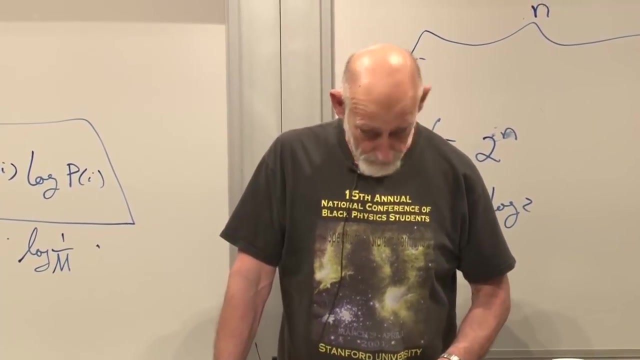 that would be the case where we know that the probability is only non-zero for one state, then M is one and S is zero. logarithm of zero. so absolute knowledge, perfect knowledge, complete knowledge, corresponds to zero entropy. the more you know, the smaller the entropy. 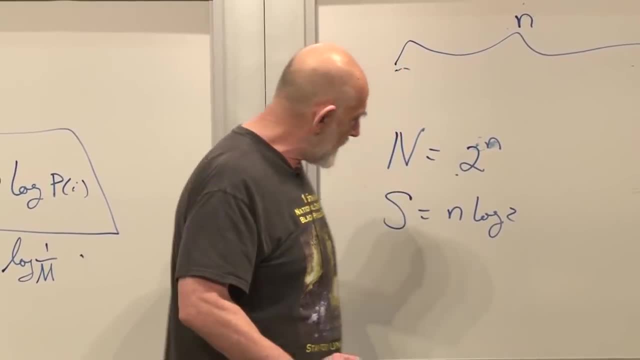 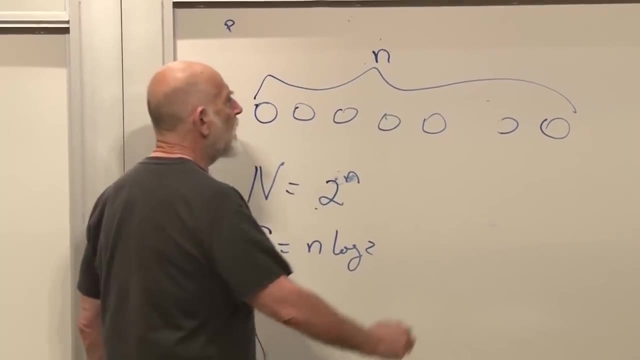 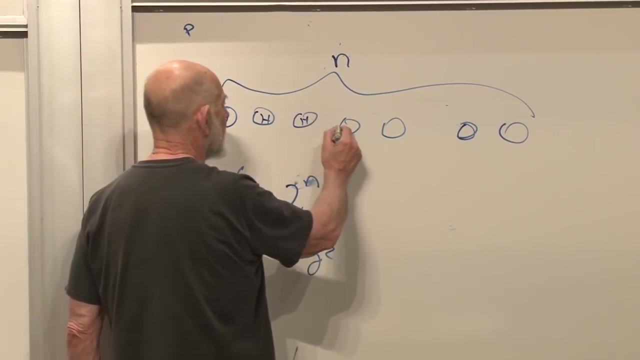 excuse me. okay, let's take a case, an interesting case. let's take our heads and tails again, and here's what we know. we know that all of them are heads. let's begin with that. all of them are heads. what's the entropy then? zero except. 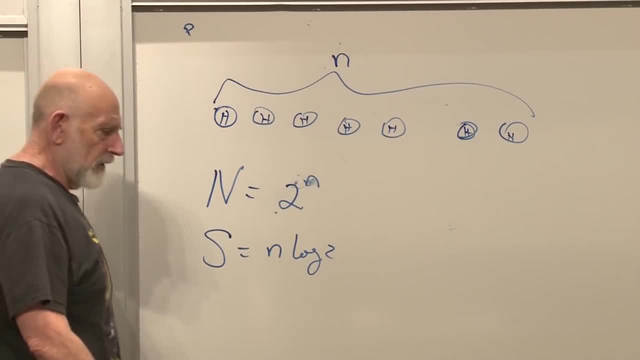 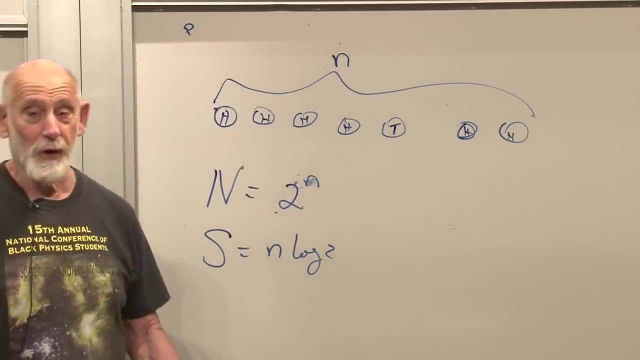 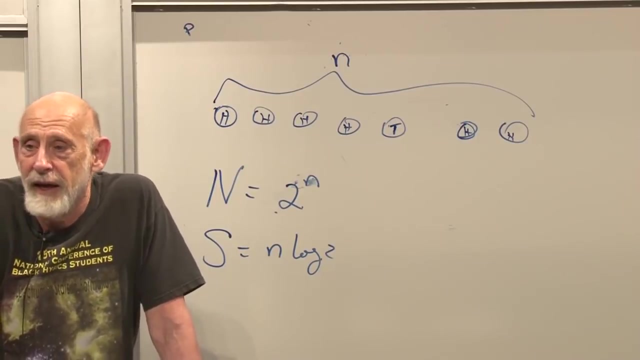 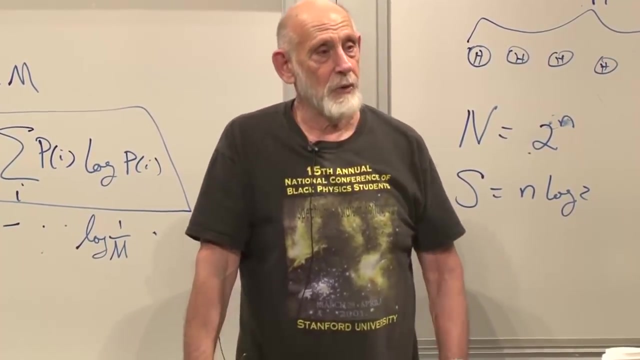 for one of them, which is tails. now, supposing we know which one is tails, what's the entropy? zero, but suppose we don't know which one is tails. equal probability for all states which contain one tail and n minus one heads. what's the entropy? indeed okay, so why is it log n? 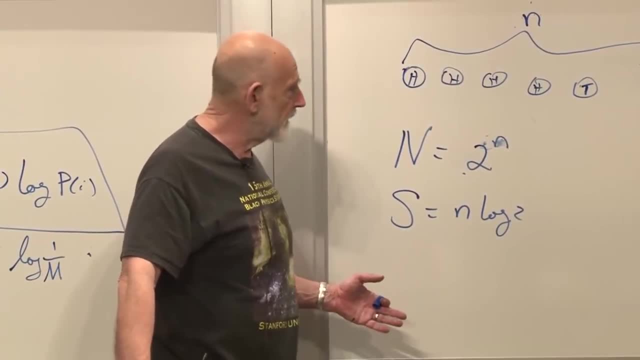 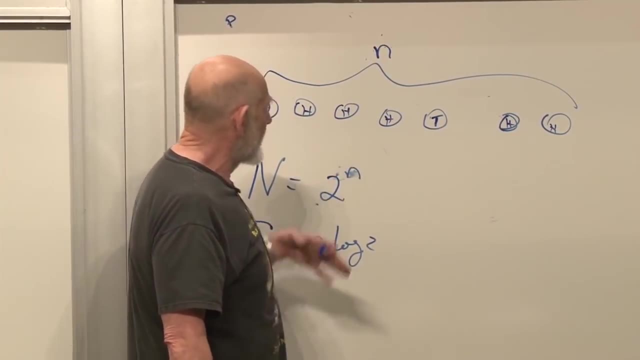 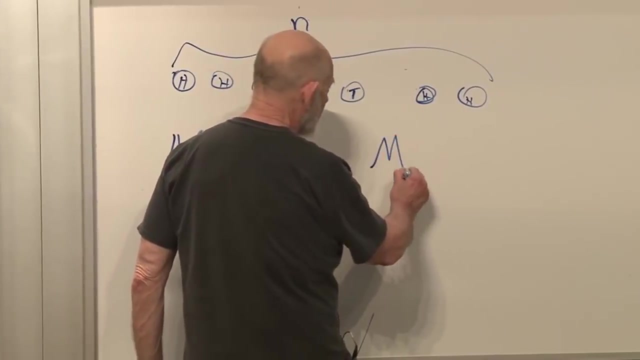 how many states are there with non-zero probability? the answer is little n. it could be this one, it could be this one, it could be this one. in other words, for this particular situation, capital M- the number of states that have non-zero probability- is just little n. 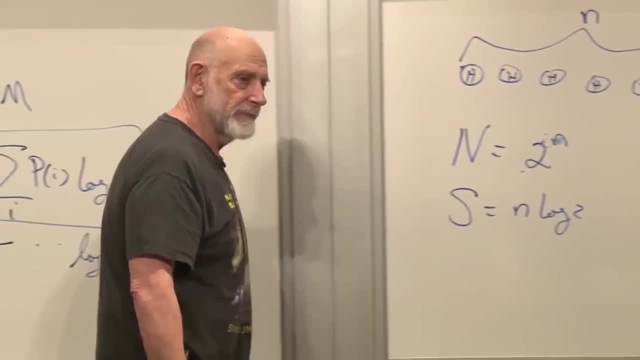 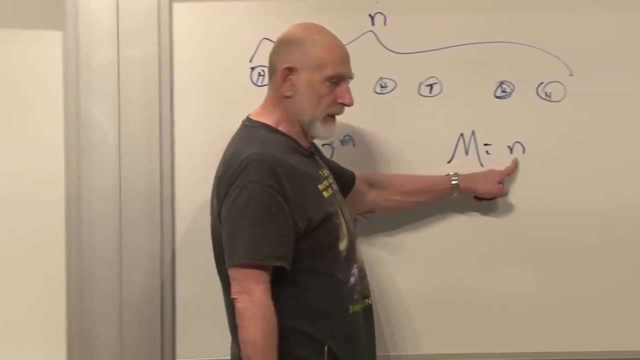 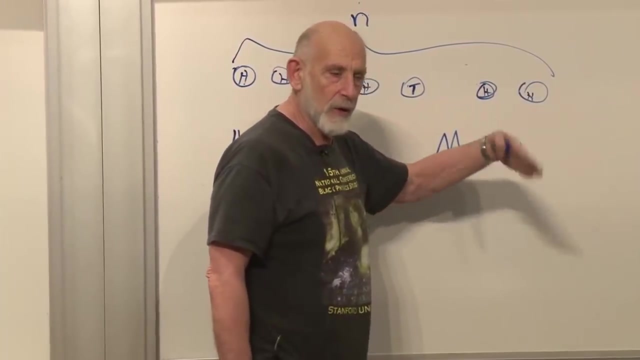 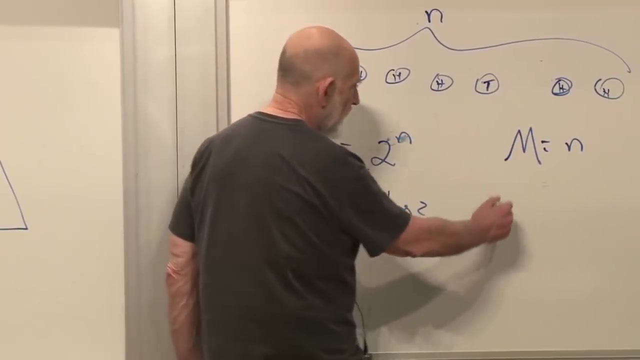 all the states have the same probability. so we're in exactly this situation, except that M is equal to little n n possible states. this one could be tails, this one could be tails, this one could be tails. they all have equal probability. so capital M is n and the entropy now is: 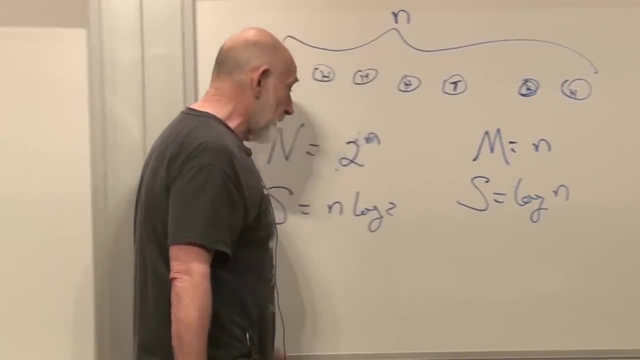 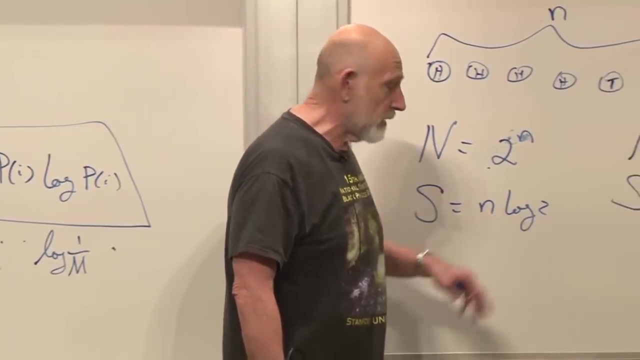 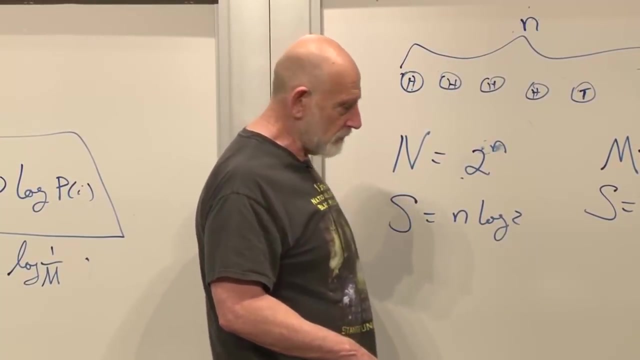 for this situation the entropy is equal to logarithm of little n. notice that that's not an integer multiple of log 2 in general. so in general entropy is not an integer multiple of log 2. it's a basic unit of entropy. it's called a bit. 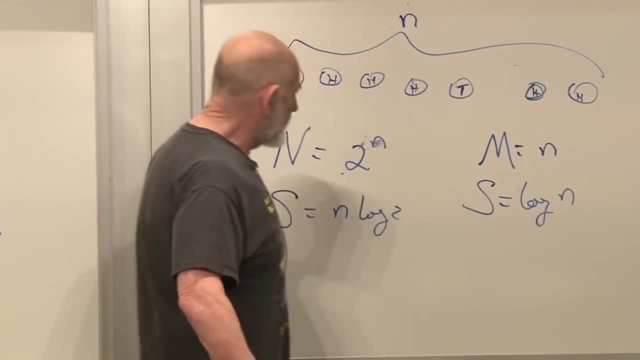 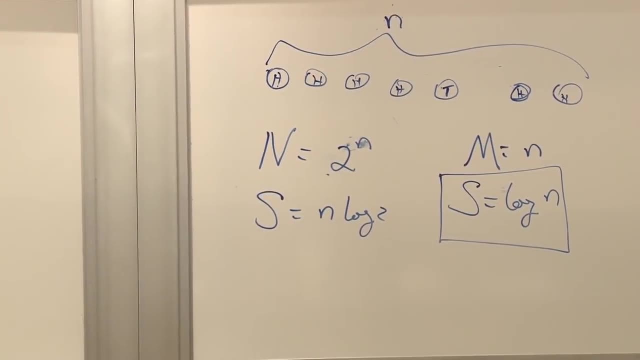 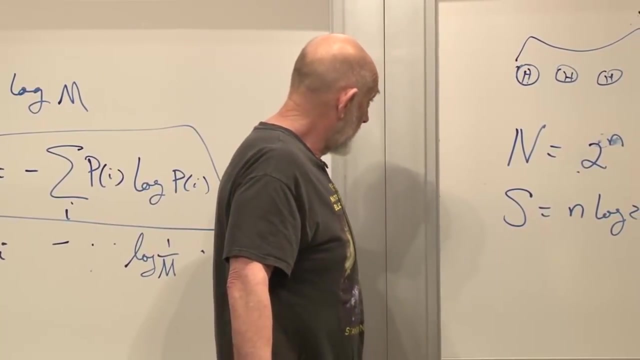 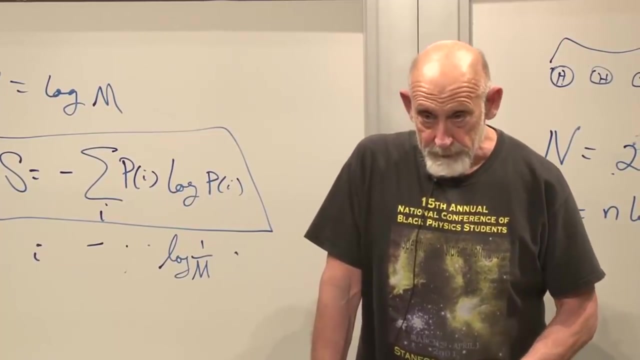 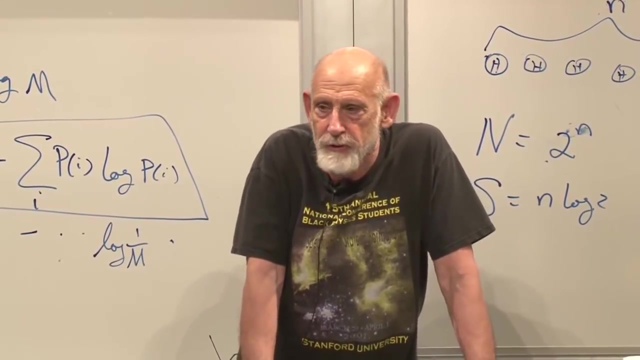 s in this case is equal to log n. yes, the 2 in the log 2 comes from the fact that you only have probability of heads or tails, right? yeah? so if you had 3, it would be log 3, absolutely right. Now, computer scientists, of course, like to think in terms of two for a variety of 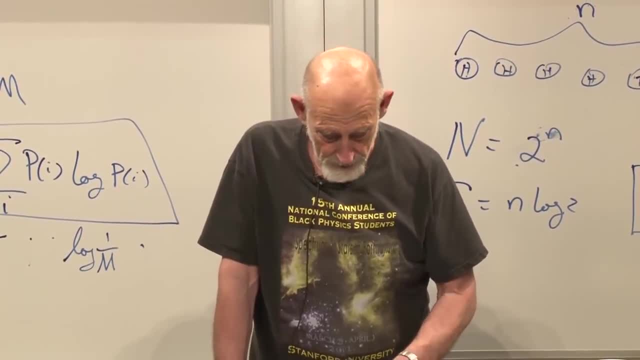 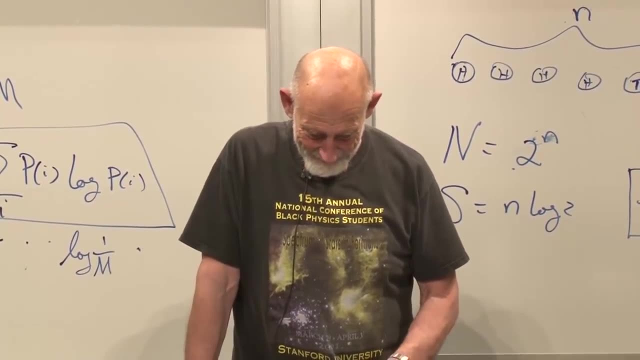 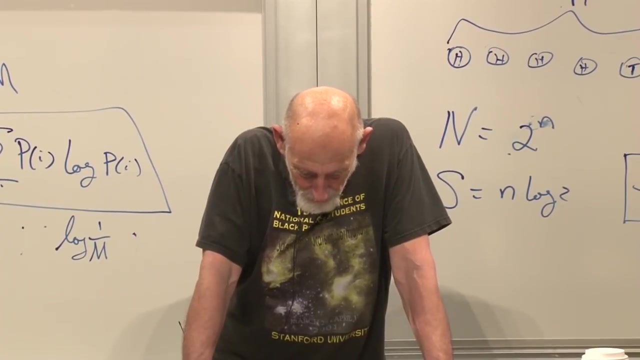 reasons. First of all, the mathematics of it is nice, but two is the smallest number, which is not one. Yeah, it's the smallest integer that's not equal to one. But it's also true that the physics that goes on inside your computer is connected with. 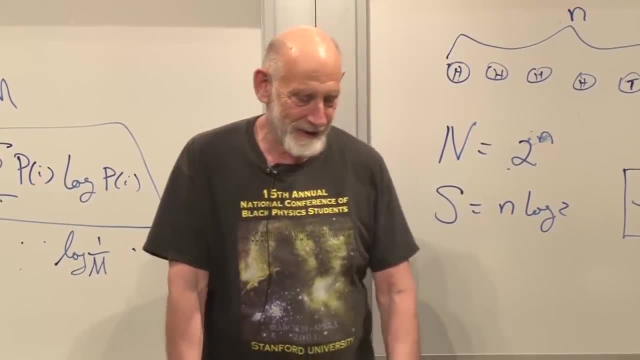 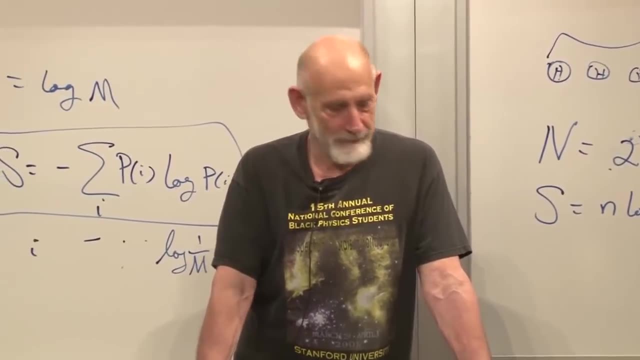 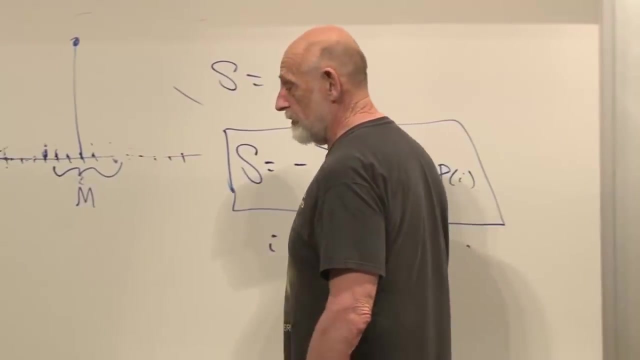 switches which are either on or off. so counting in units of log two is very useful. Excuse me, Yeah, It's probably not important, but what is the base of the logarithm? Yeah, the standard. this is a definition. of course, this is a definition. 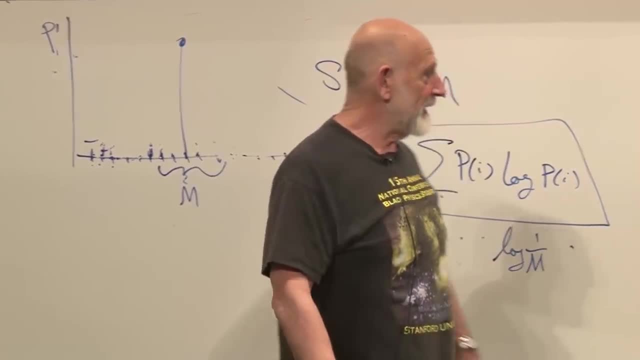 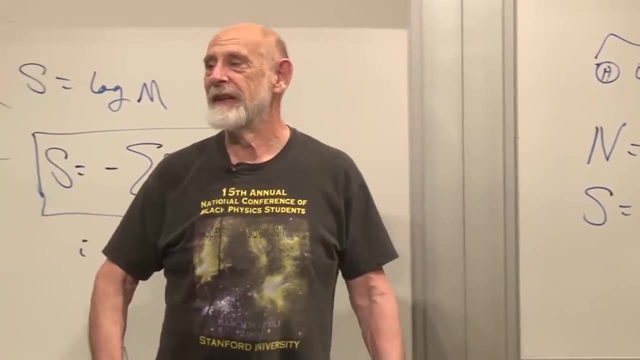 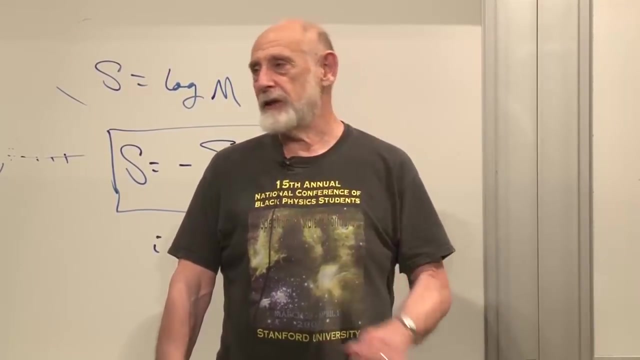 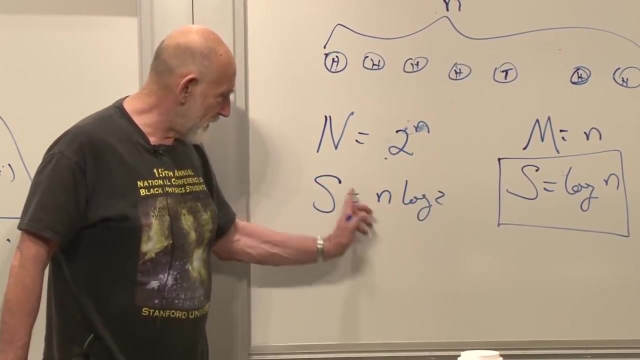 The definition. okay, good, It depends on who you are. If you're an information theorist, a computer scientist often, or a disciple of Shannon, then you like log to the base two, In which case this is just one n and the entropy here is just n, measured in units. 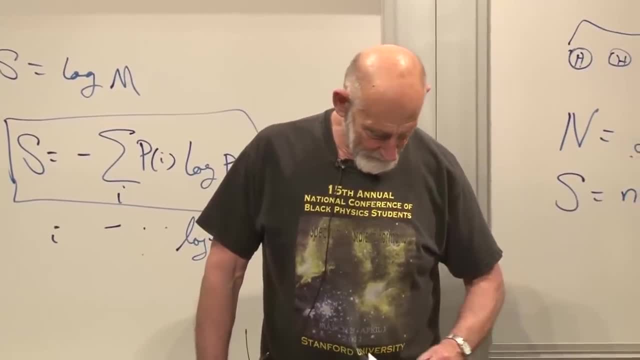 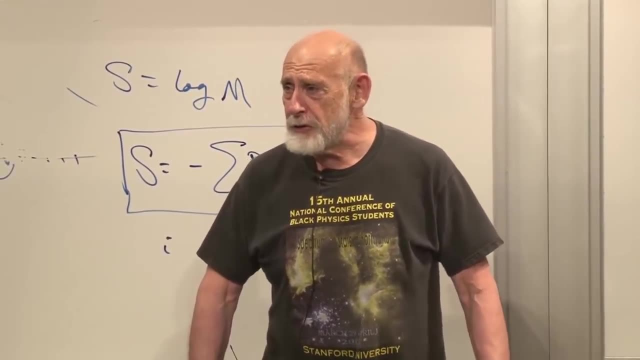 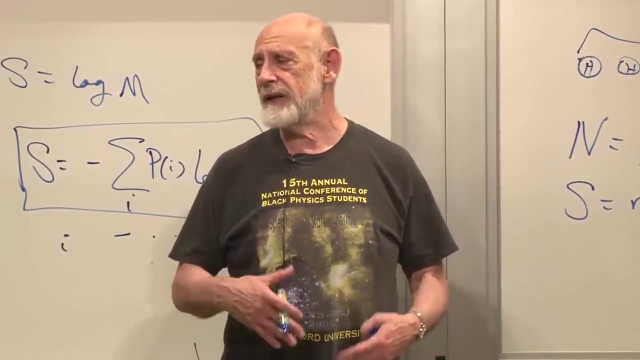 of bits. If you're a physicist, Yeah, Then you usually work in base e, okay, But the relationship is just a multiplicative. you know, log to the base e and log to the base two are just related by a numerical factor. that's always the same. 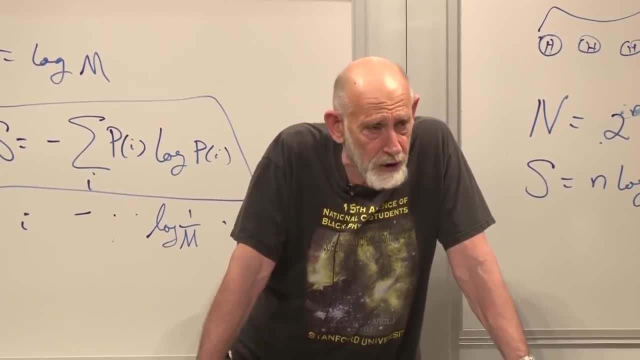 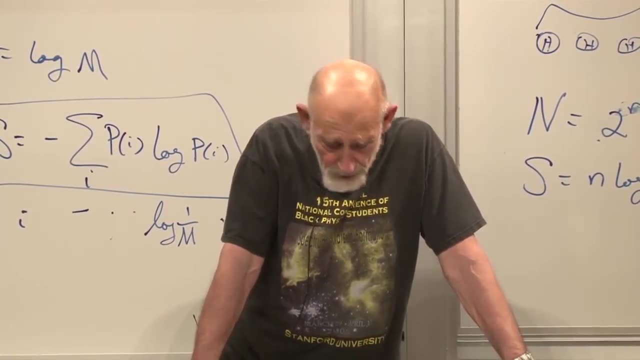 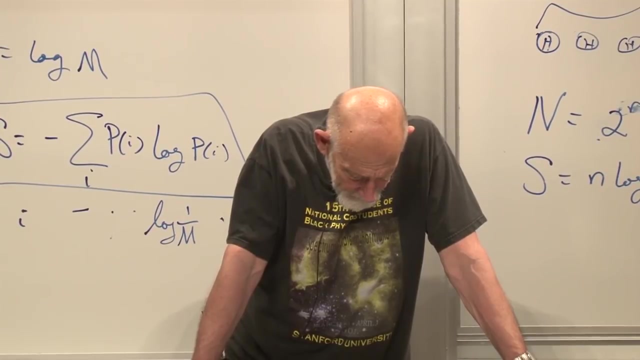 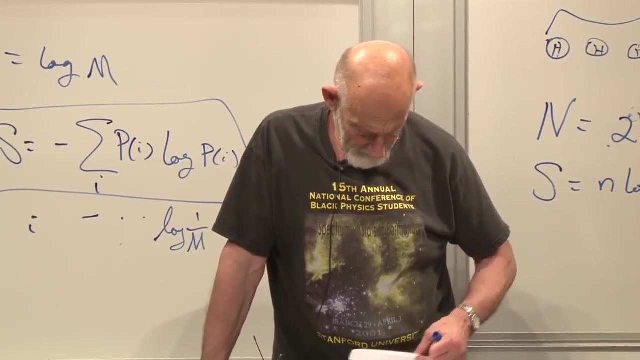 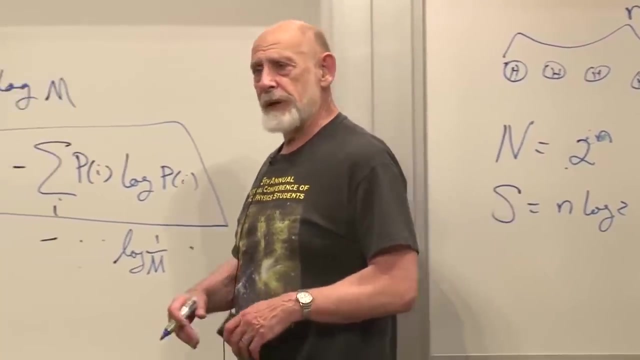 Okay, so when I write log l-o-g, I mean log to the base e, but very little would change if we use some other base four. But if we write log to the base two, we use that base four and we use that base four. 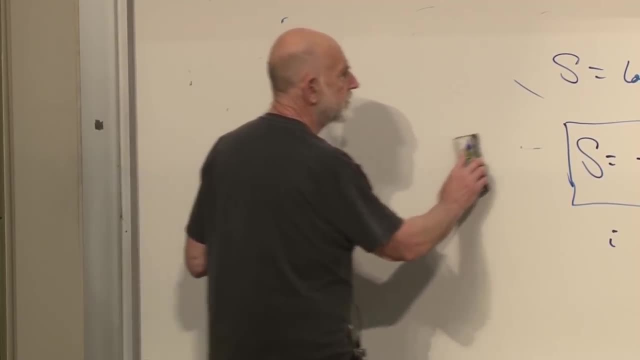 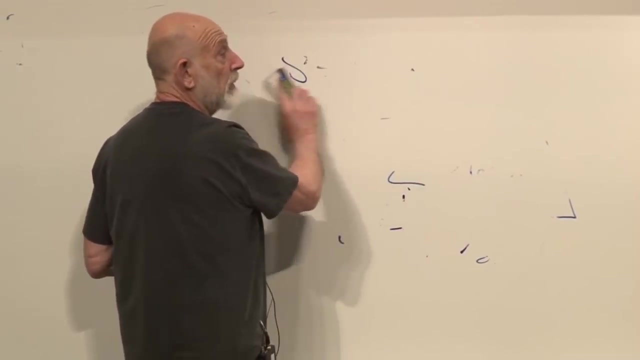 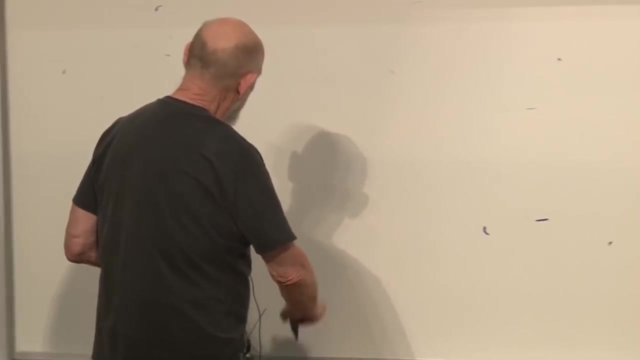 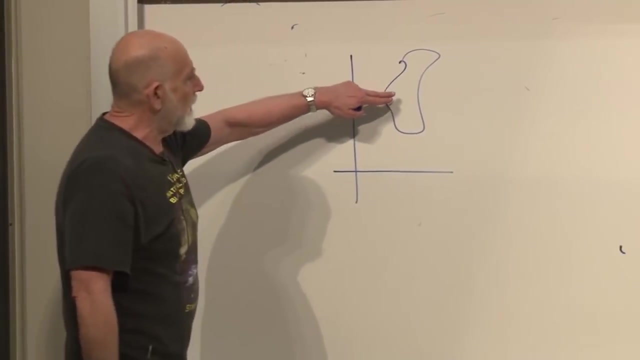 as an expression, Okay, talking about? if we're not talking about these finite, discrete systems like this, we're talking about continuously infinite systems, phase, space. and let's begin, supposing the probability distribution is just some blob, where the probabilities are equal inside the blob and 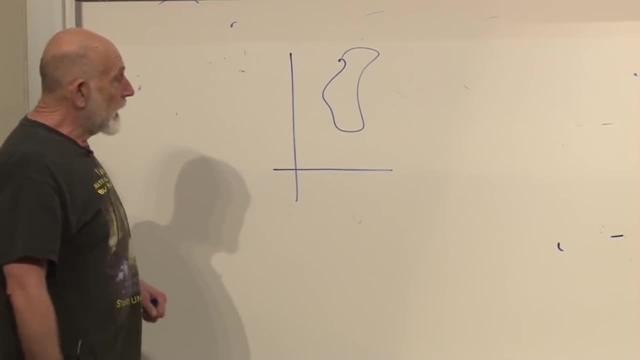 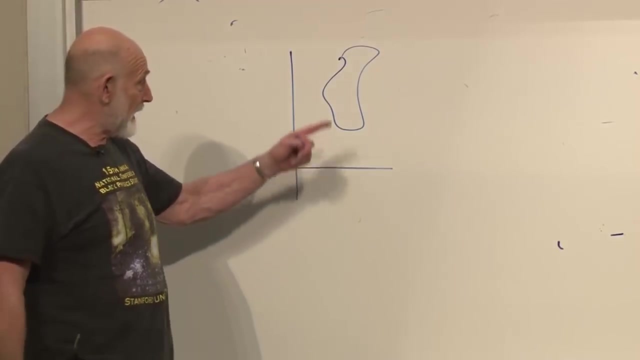 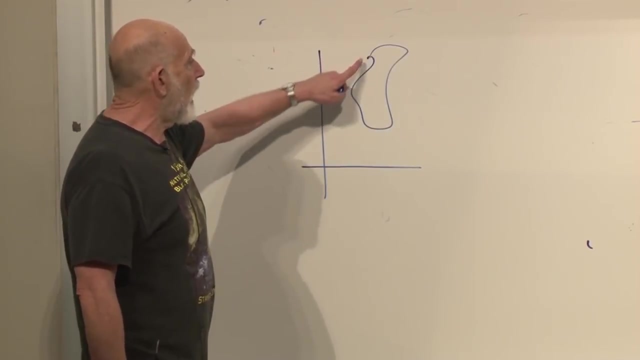 zero outside the blob. In other words, the simple situation. Then the definition of the entropy is simply, well, you could say the logarithm of the number of states. but how many states are there in here? Clearly a continuous infinity of them. So instead you just say it's the log of the 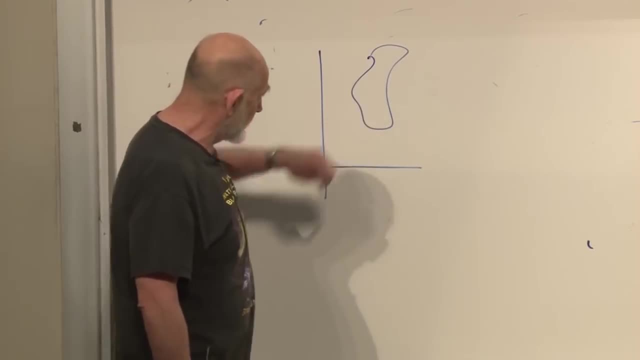 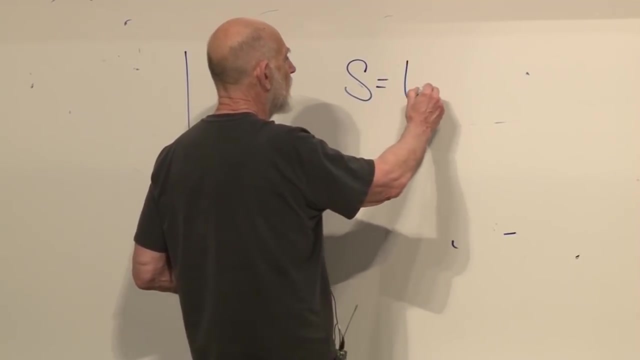 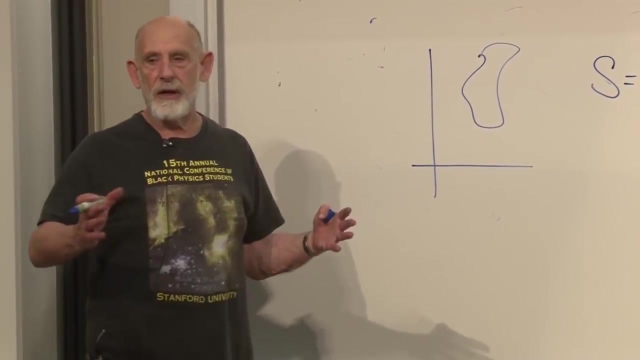 volume of the probability distribution in phase space. S for a continuous system is just defined to be the logarithm of the probability distribution in phase space, The volume in phase space. Now, if I wrote V, you might get the sense that I'm talking about. 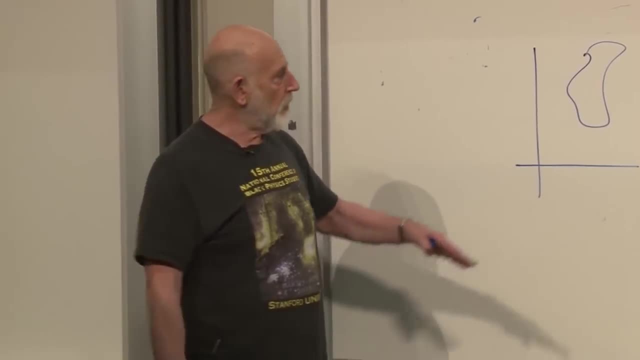 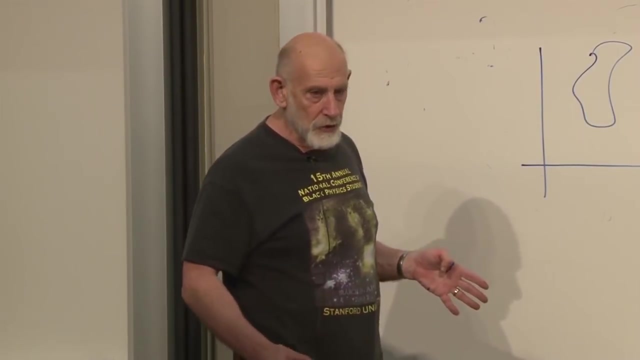 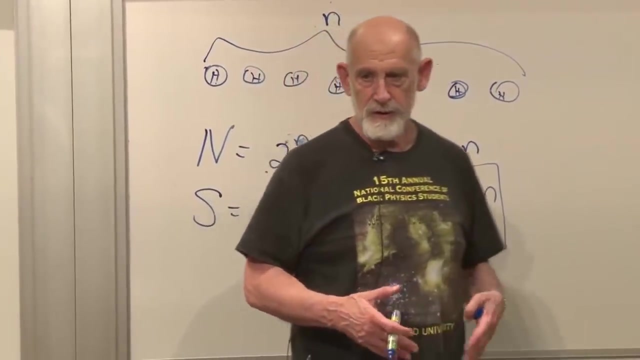 volume in space. No, I'm talking about the logarithm in phase space, the volume in the phase space. The phase space is high dimensional. Whatever the dimensionality of the phase space is, the volume is measured in those kind of units of momentum, times, velocity to the power of the. 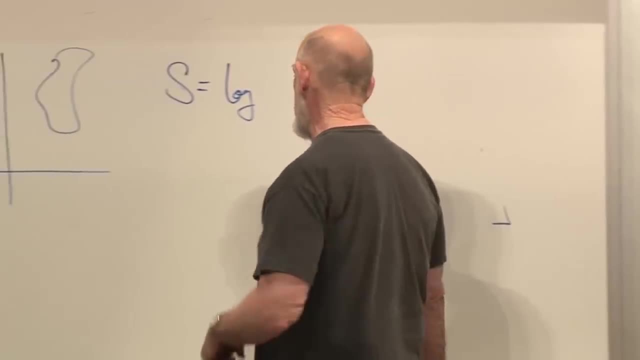 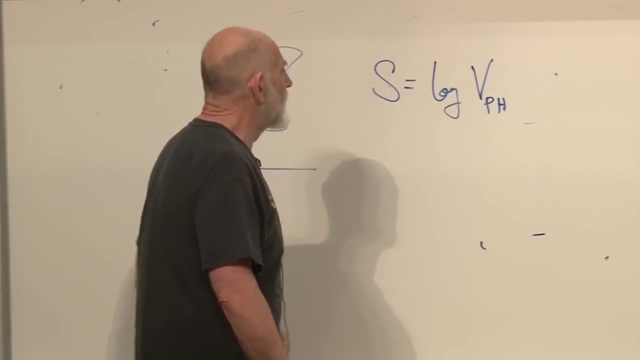 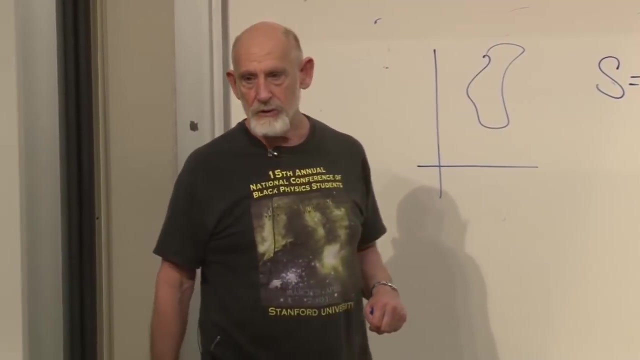 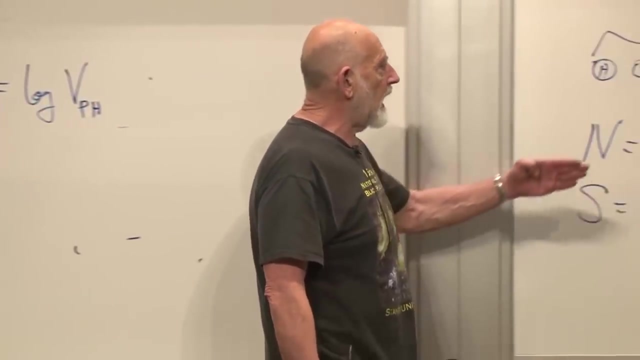 number of quads. There's no coordinates in the system, All right, But S is equal to the logarithm of the phase space volume. Let's call it V phase space, That's under the volume of the region which is occupied and has a non-zero probability distribution. This is the closest analog that we can think of to log M. 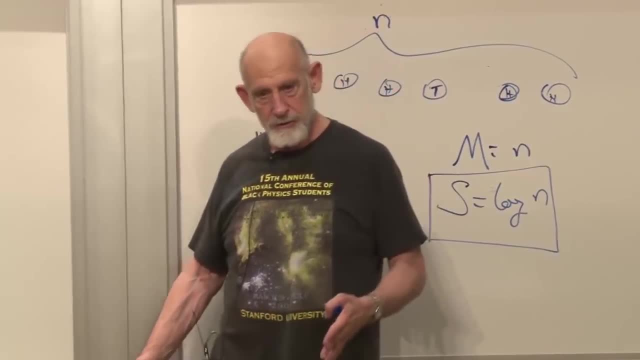 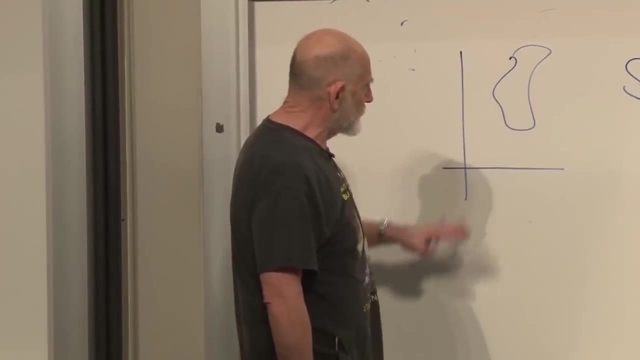 where M represents the number of equally probable states. Now I now don't have to know the partitions per second right more, But I know the ratio of odd to within. So if I multiply the дос in order to2020, I can see Qt of review. 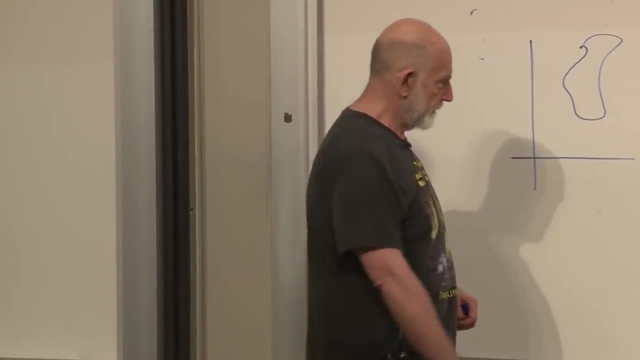 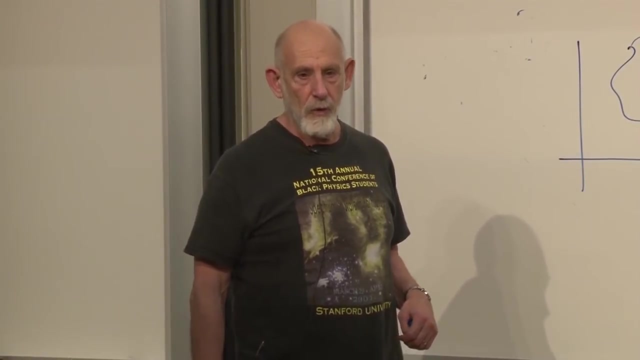 That makes sm right. the motive is: 10% of N times the time spent on the relative…. theอง and I dial bringing vectors. Equivalence is that whule. it's going to be on an igual and I'm kind of adding on there a half of two. 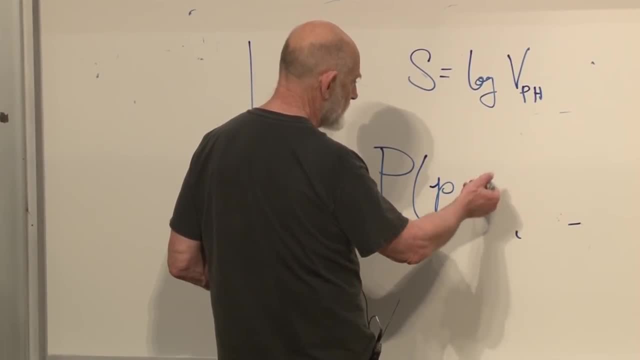 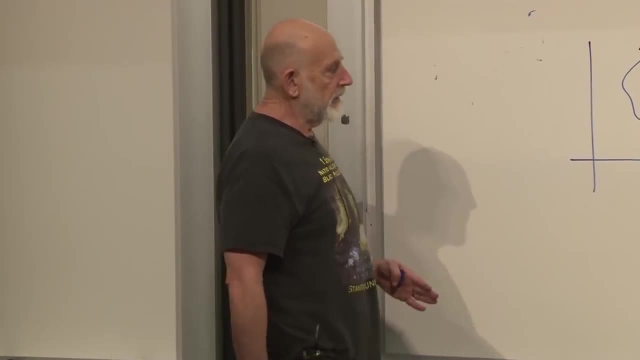 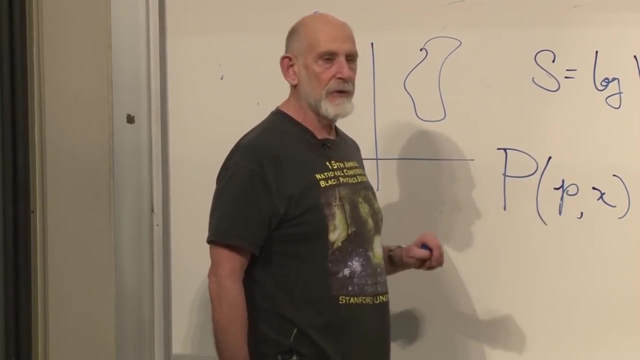 So it's 10 entire π's on x. this takes the same thing: 0,, 0,, 2, dow 2, Xs, whichever you like, all of them. Probability for the system to be located at point of phase space P and X. 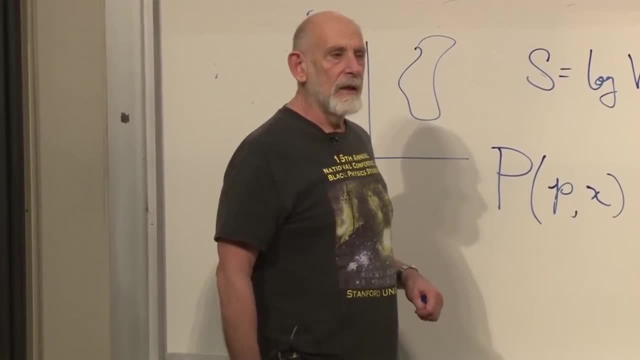 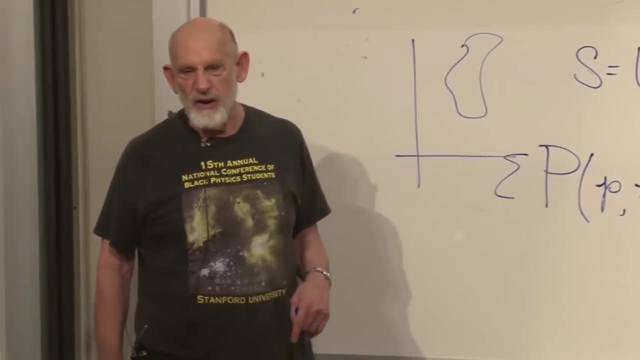 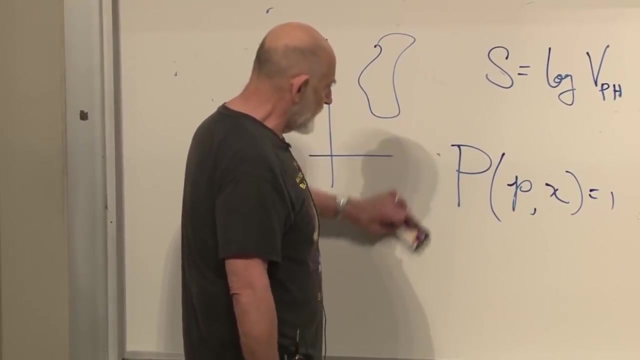 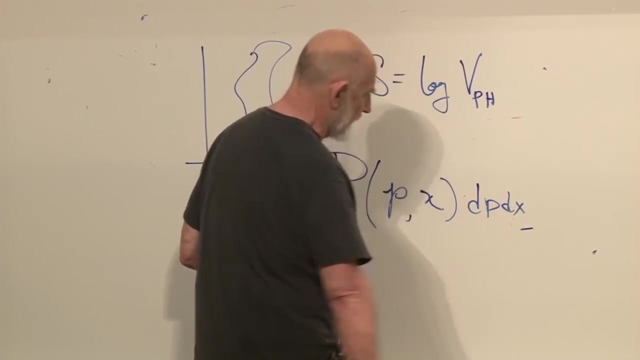 Incidentally, when you have continuous variables like that, do you write that the sum is all equal to 1?? That wouldn't make sense. You can't sum over a continuously infinite set of variables. It becomes integral. We'll come back to this, but let's just spell it out right now. 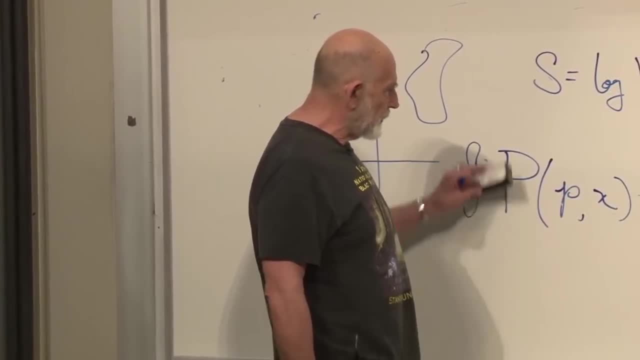 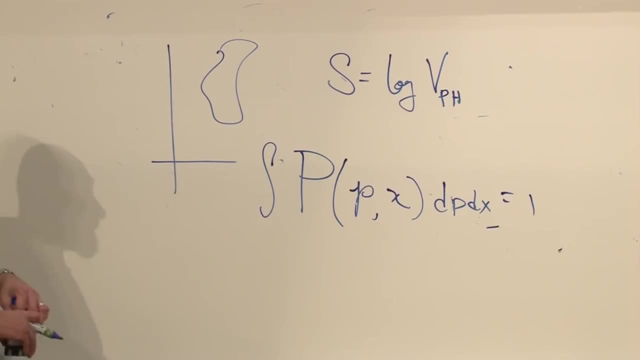 that if you have a probability distribution on a phase space, the rule is that the integral of it is to be equal 1.. P is really a probability density on phase space. It's a probability per unit cell in phase space And what would you expect the entropy to be? 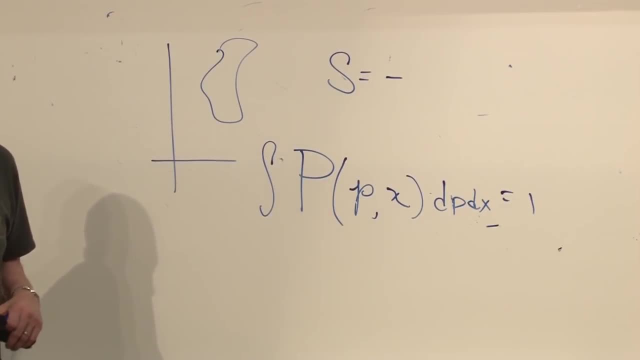 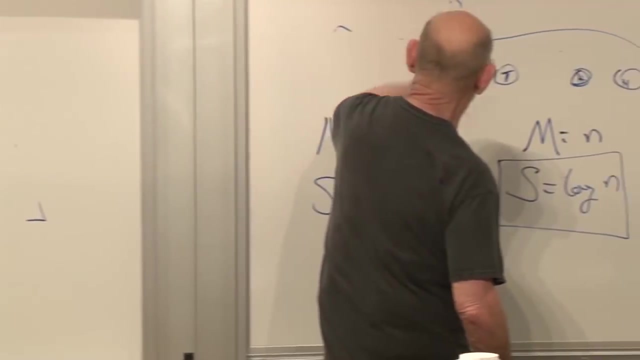 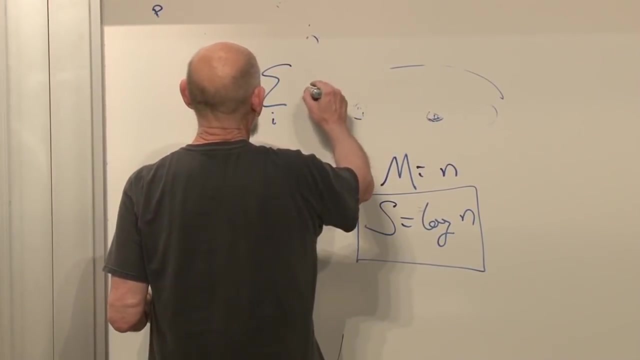 I'll give you a hint. It starts out with minus. Where's the formula that we had here before? Let's rewrite the formula that we had before. S is equal to minus. summation over I of P sub I. log of P sub I. 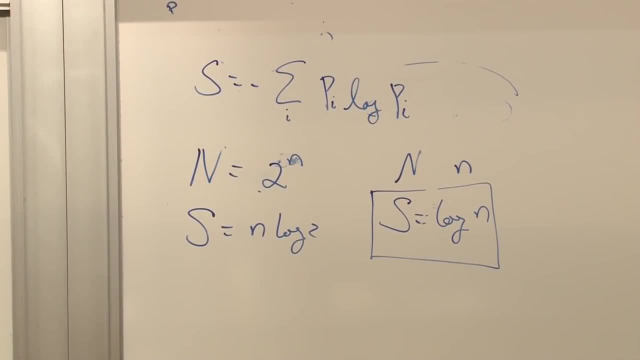 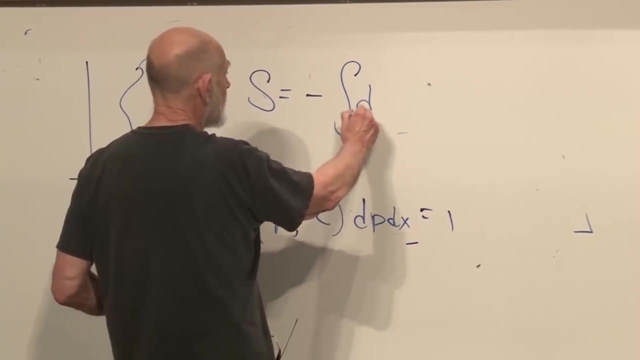 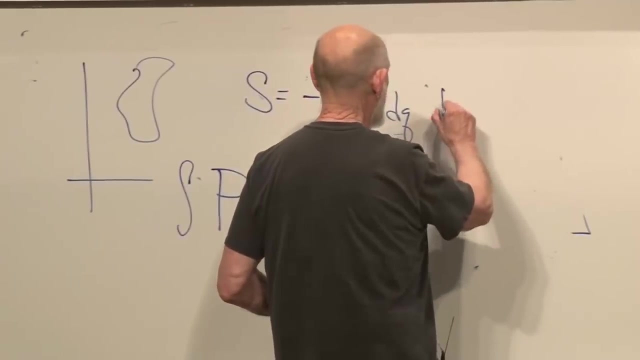 To go to the continuum, you simply replace sum by integral. So there's an integral over the phase space, That's like the sum over I, And then probability of P and Q times the logarithm of the probability. That's the probability. 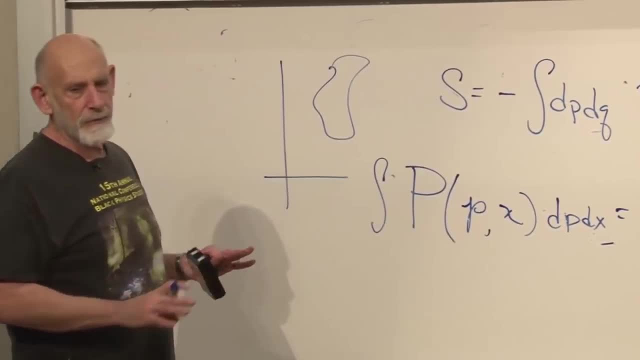 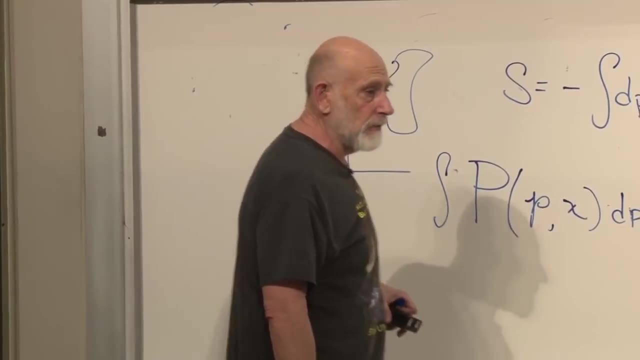 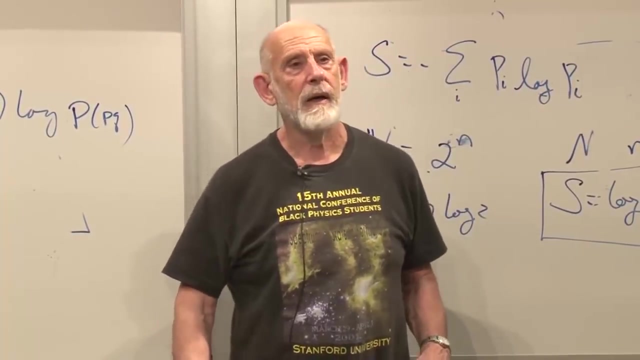 But in first Approximation I don't mean first approximation numerically, I mean first conceptual approximation. It's measuring the logarithm of the volume of the blob, the probability blob in phase space. Okay, Why did you move from X to Q? 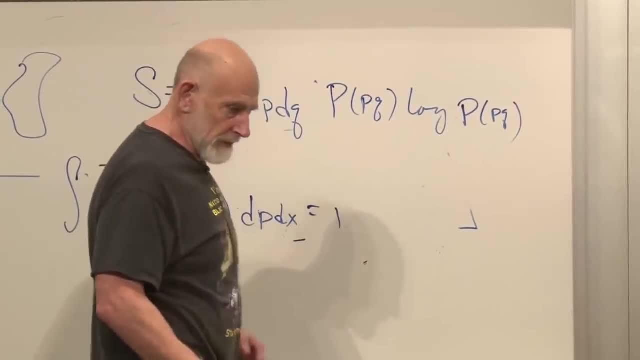 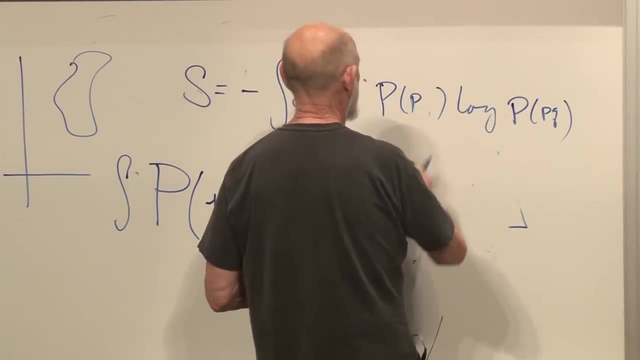 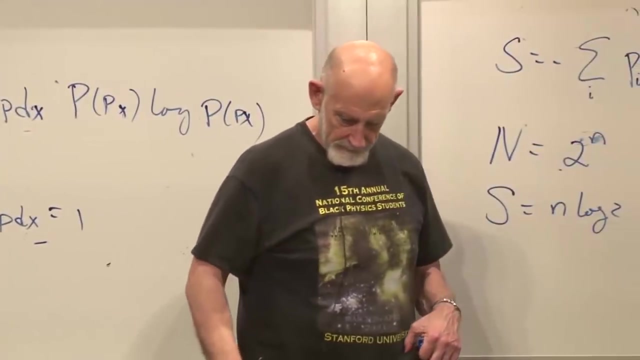 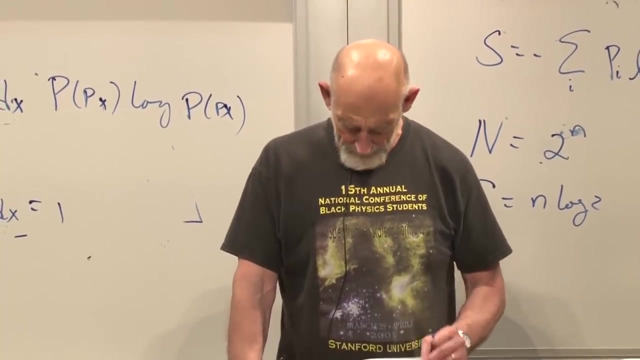 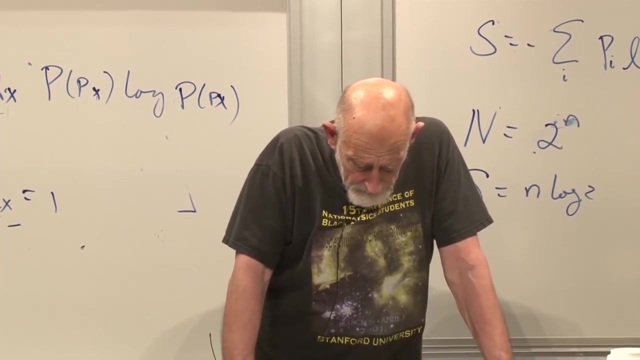 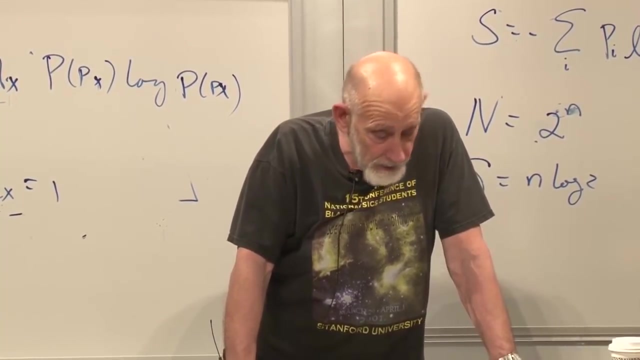 Oh, I could No Mistake. Mistake: In classical mechanics X's and Q's are coordinates and P's are momenta. But you know that. Okay, So we've now defined entropy which, as we've seen, depends on a probability distribution. 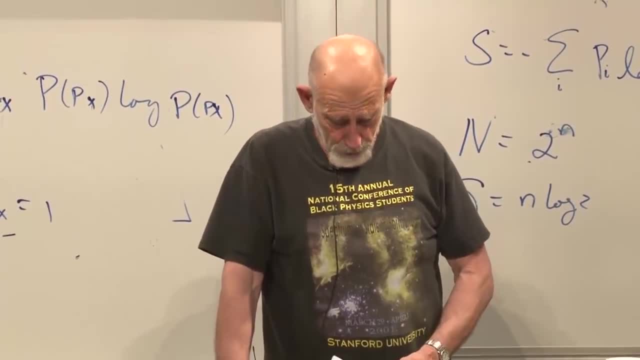 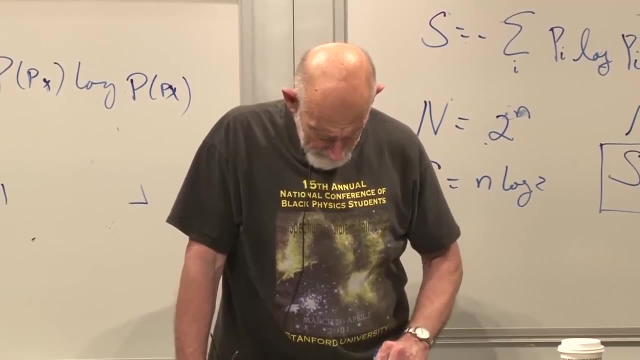 I'm going to go one more step tonight and define. I'm going to go one more step tonight and define. I'm going to go one more step tonight and define Temperature. Well, we could stop here. I think that's probably enough for one night. 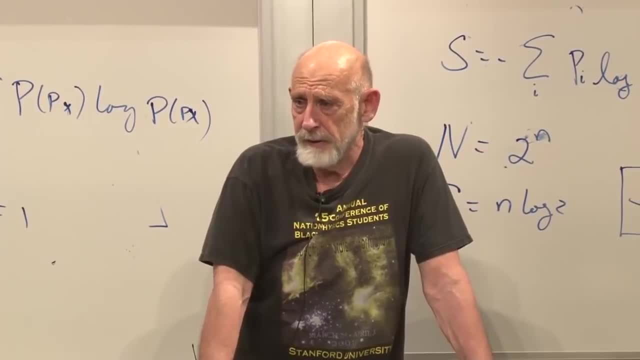 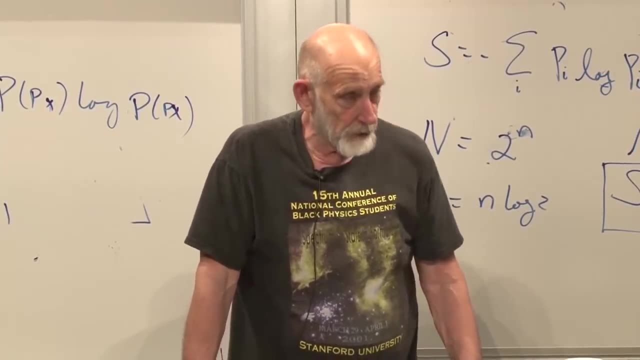 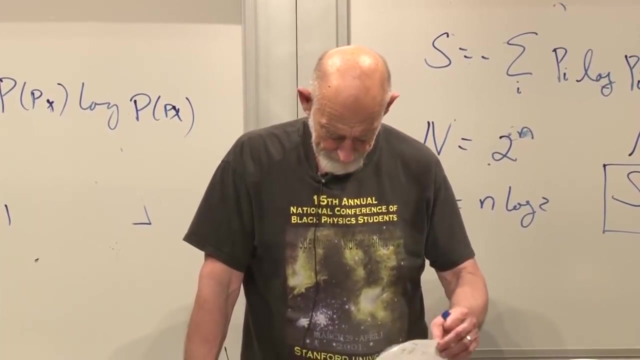 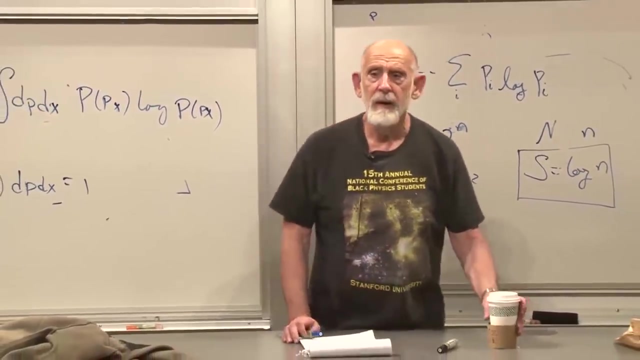 Next time we'll do temperature and then discuss the Boltzmann distribution, which is the probability distribution for thermal equilibrium. We haven't quite defined thermal equilibrium yet, but we will. You can ask some questions. I don't mind some questions now. 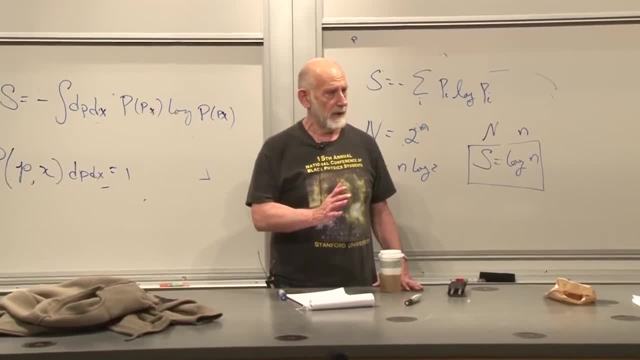 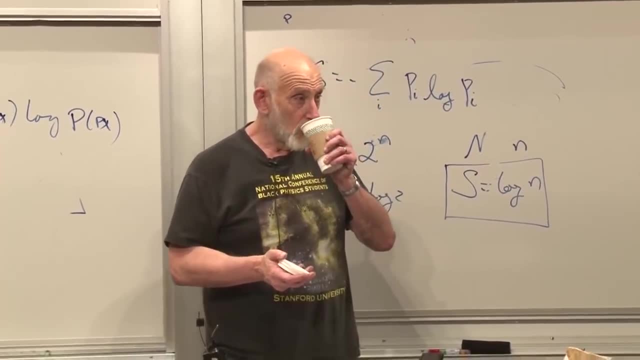 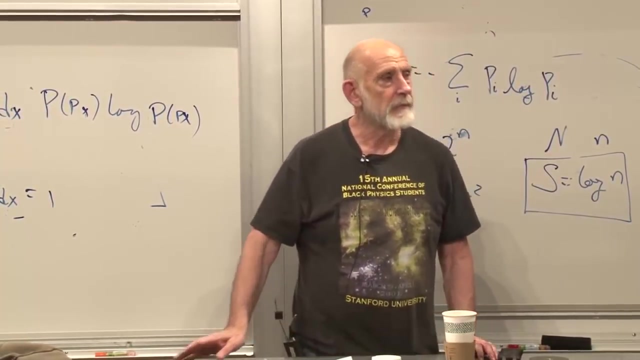 I just have the feeling that I've probably done enough for one night. There seems to be an assumption that the point that I don't know if it's independent of the other clips, Oh That if, If you get a heads, if the probability of the next one is a heads, that this 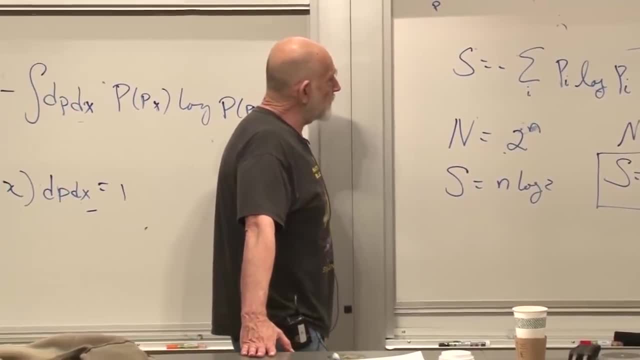 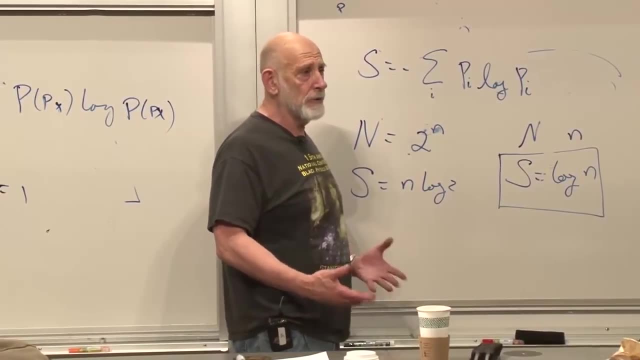 Well, I haven't made any such assumption. I haven't made any such assumption. My only assumption in calculating the various entropies was either that you know nothing or I told you what you know, How you got to know that and what the reasoning was, and whether it had to do with knowing. 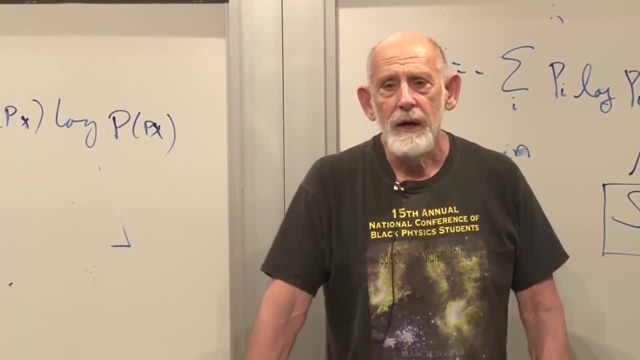 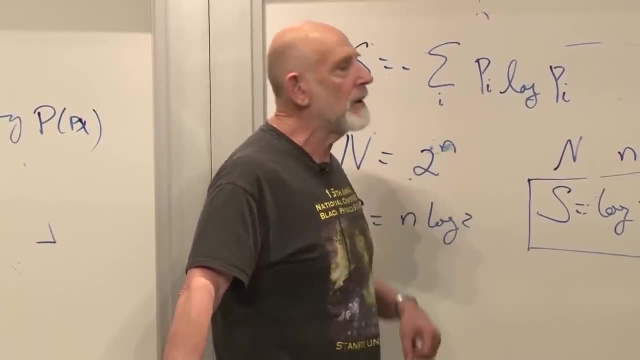 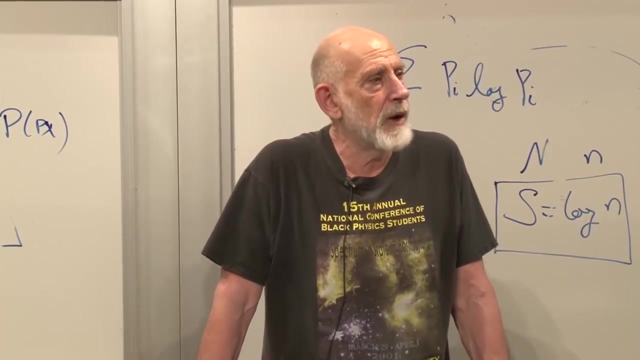 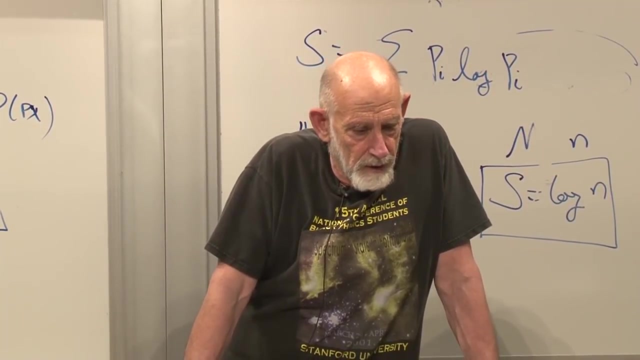 something about the dynamics and the independence and so forth. Uh, May come into your, into your calculation of what p is, but in saying you know nothing, the implication was that all states are equally probable. And without asking how you knew that, to say that all states are equally probable is closely. 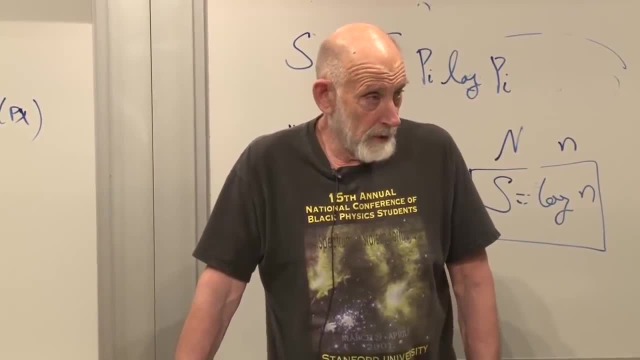 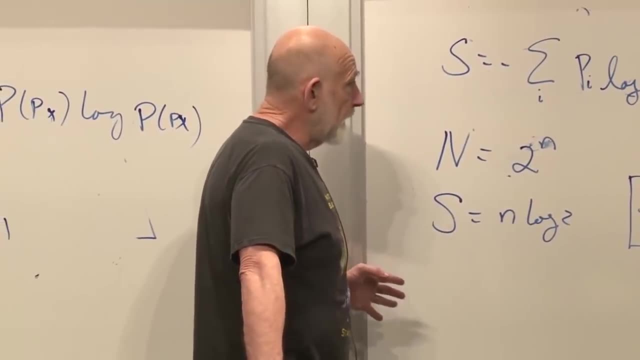 related to saying that there are no correlations. It does say that, if you All right, Well, let's Good, Let's talk about correlations for a moment. To say that you know nothing means you know nothing. So, in particular, if you. 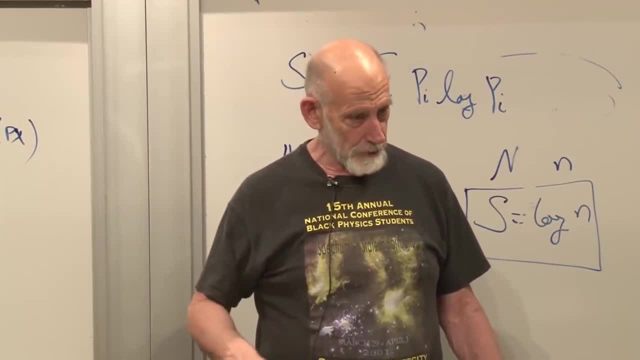 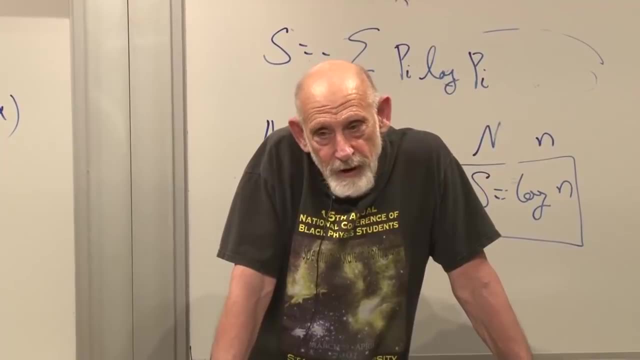 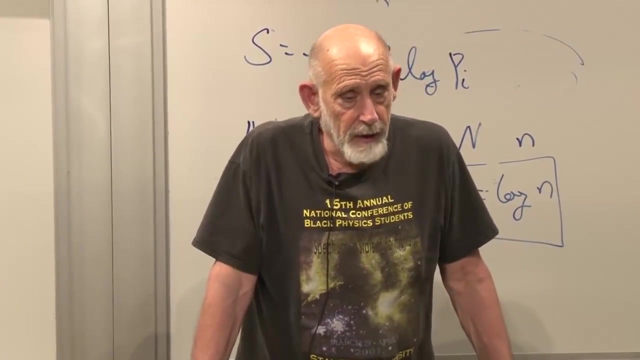 You begin knowing nothing and you measure one of the coins. what do you know about the other ones? Nothing, Nothing. You started knowing nothing about them. you measured one of them. you still know nothing about the other ones. Of course, you know about the one that you've measured. 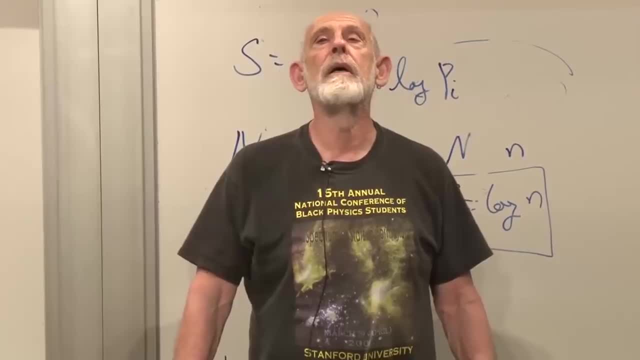 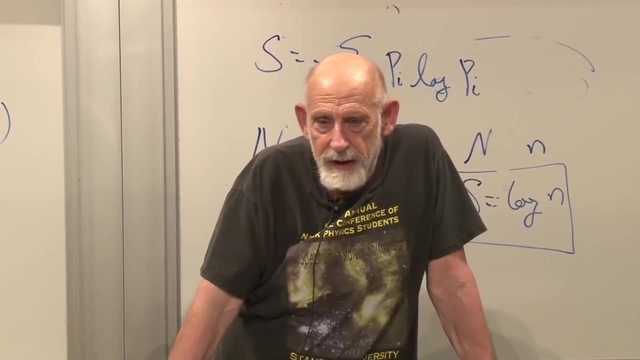 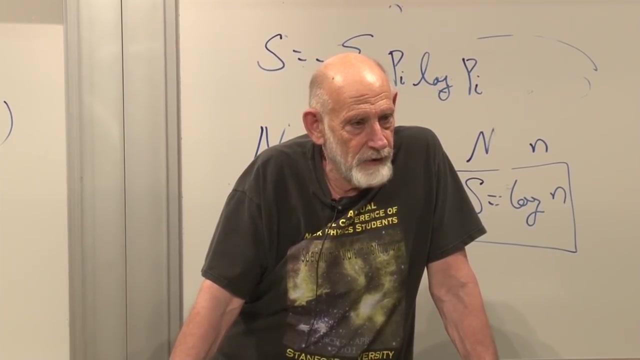 Now let's take the other, The other case that we studied. Supposing we know that all coins are heads except for one, which is tails, and we now measure one of them and we find that it's tails, What can we say about some other one? 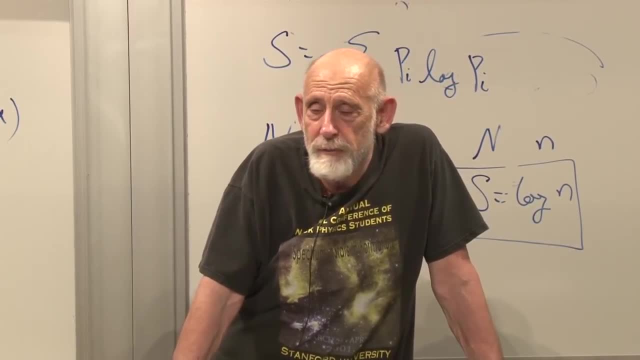 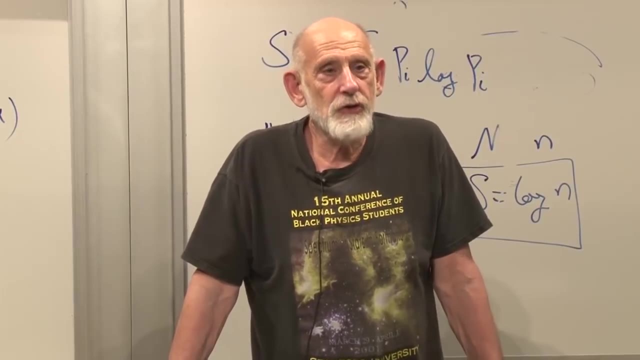 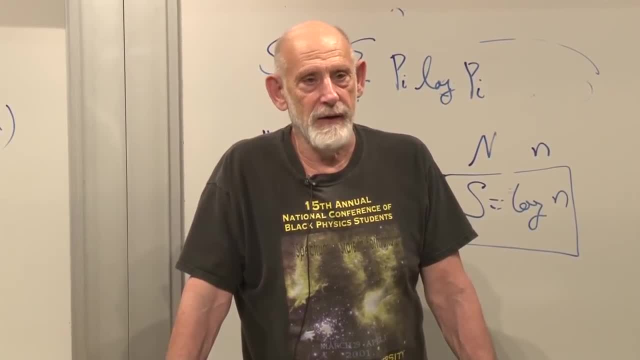 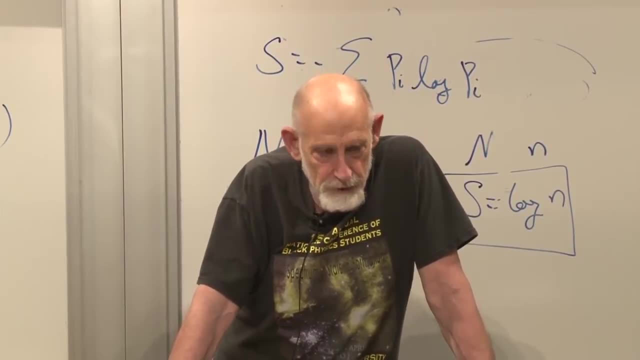 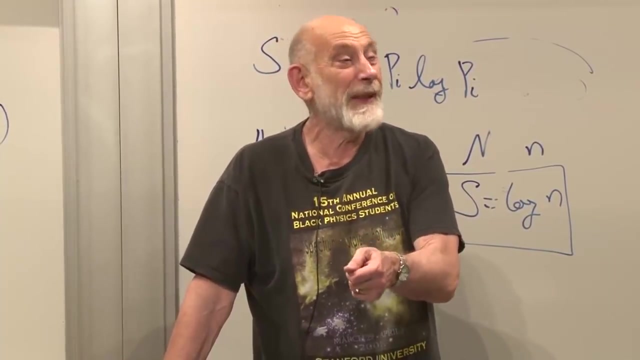 Right, It's one over n minus one instead of one over n minus one, So that's correlation. That's correlation where when you measure something, you learn something new, or the probability distribution for the other things is modified by measuring something. That's called correlation. 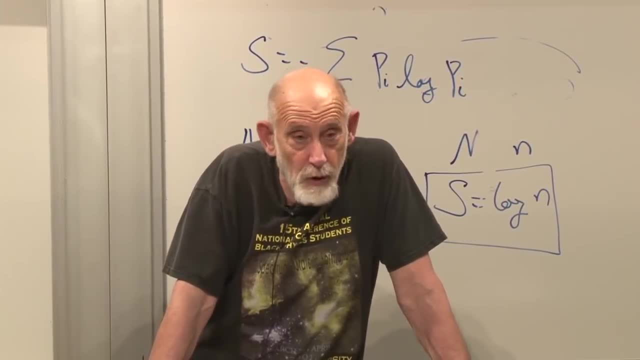 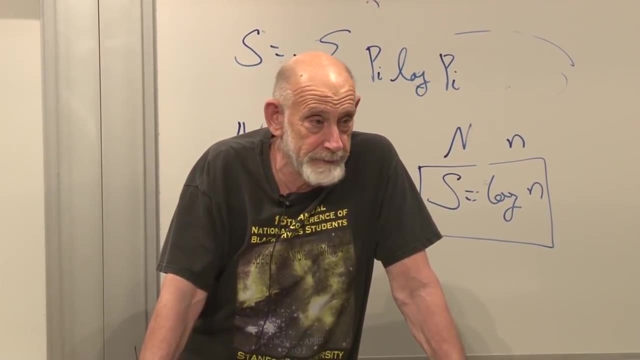 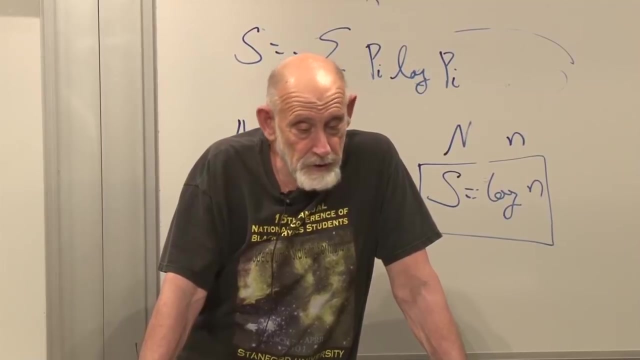 For the complete ignorance. there is no correlation For any other kind of configuration in general. there's very likely to be some, not necessarily, but there's very likely to be some correlation. Correlation, as I said, means you learn something about the probability distribution of other. 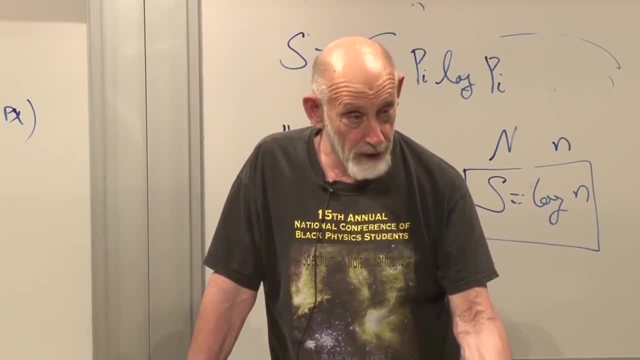 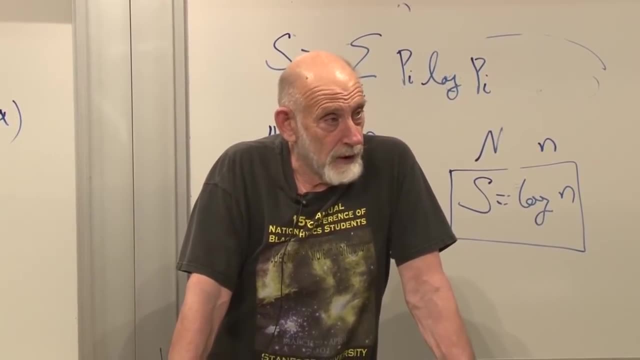 things by measuring the first one, or you modify the probability distribution. Good, Okay, Thank you. I don't know if that's what you asked about or not, but yeah, Okay, All right, That original system there where we had two parts. 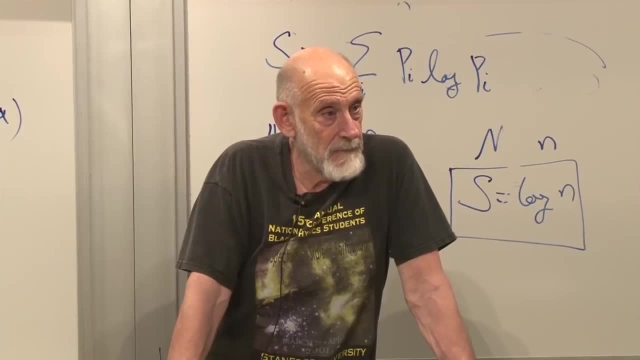 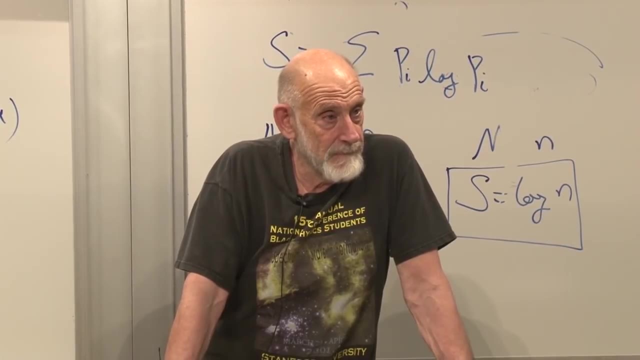 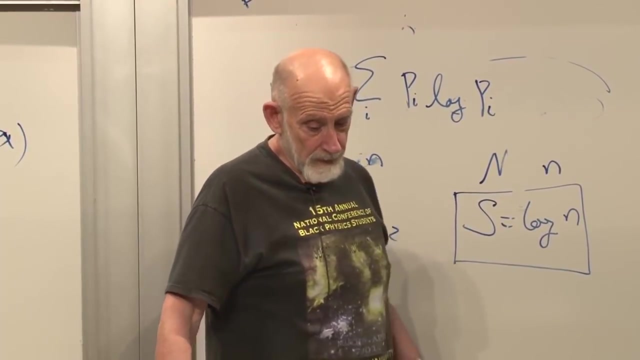 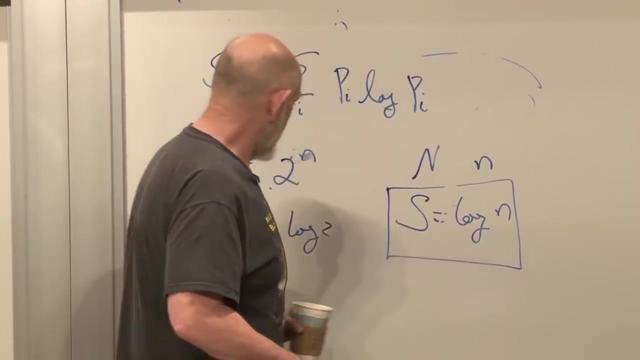 Once we measured one thing, we had to conserve quantity. What's that? again, We had to conserve quantity. there, that once we did one measurement, we knew which side we were on. Yeah, Yeah, Incidentally, entropy is additive, It's additive. 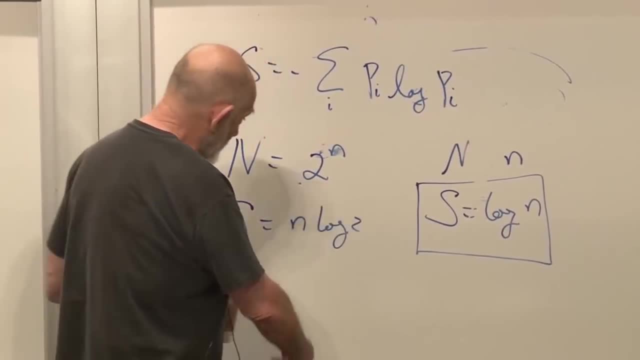 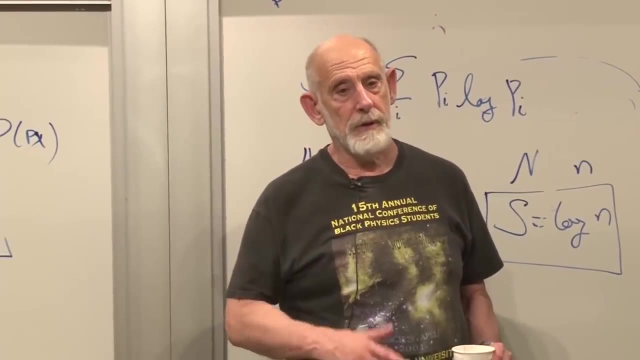 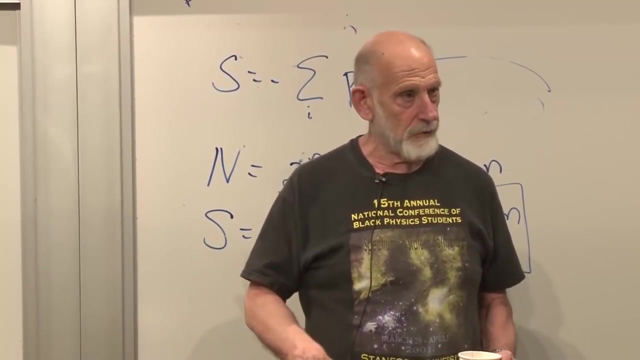 It's the sum of the entropies of all the individuals. It's proportional to the number of things. It's additive whenever there is no correlation. When there's no correlation, it's additive. Now, uncorrelated systems have additive entropies. 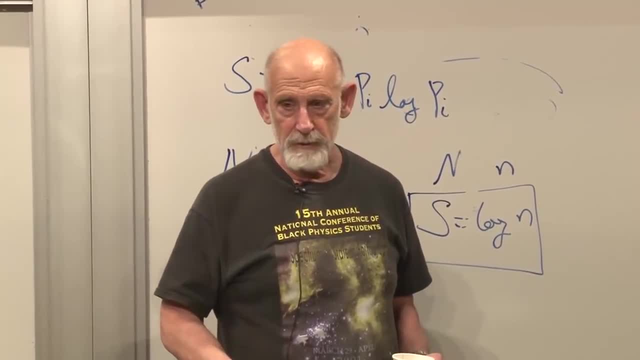 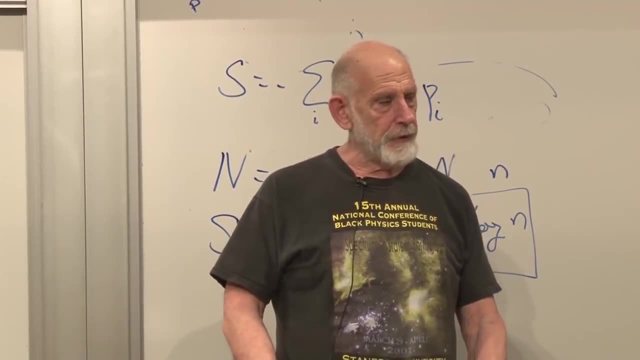 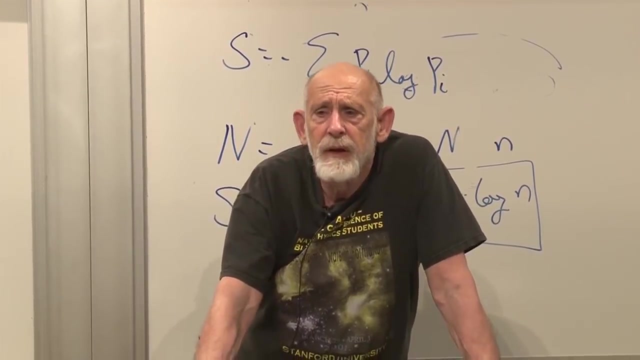 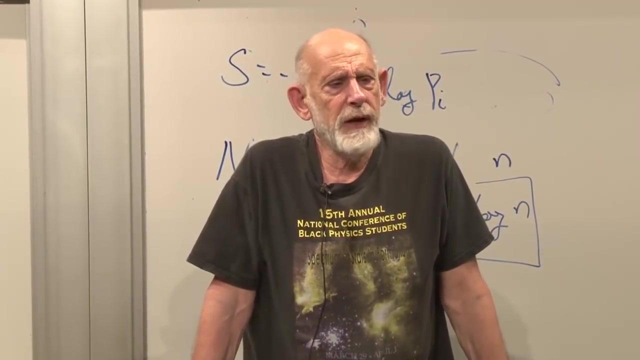 We'll come back. That's a theme that we'll come back to in a minute. Here's an interesting question, Supposing here's what you know. You know that if you measure a coin up, then with three-quarter probability they're laid. 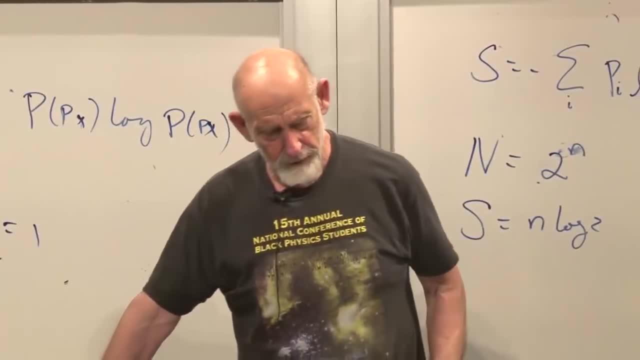 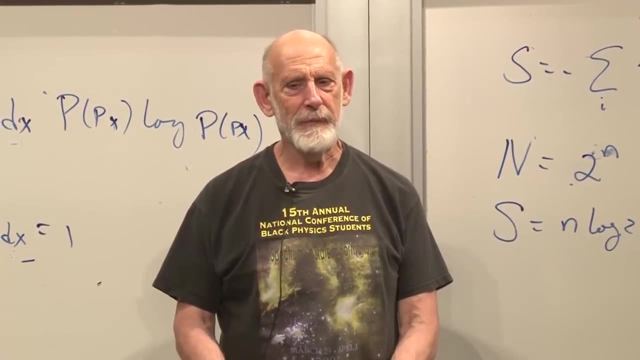 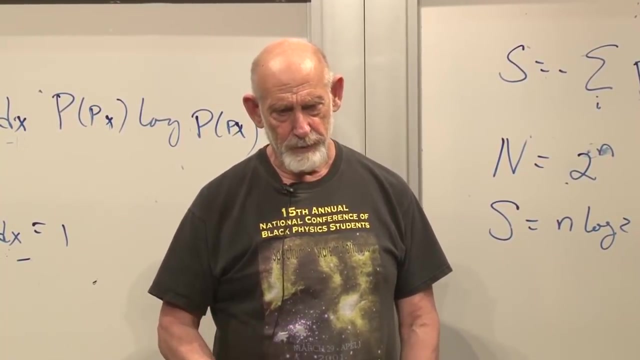 out in a row. If you measure one of them and it's up, then the probability for its neighbors is three-quarters to be down. That's what you're given. That's all you know. That's all you know is that if one of them is up, if any one of them is up, its neighbors. 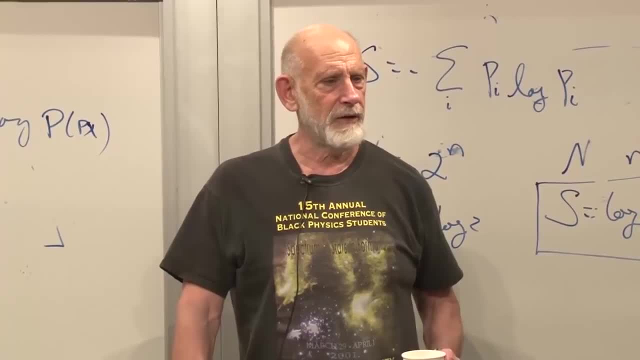 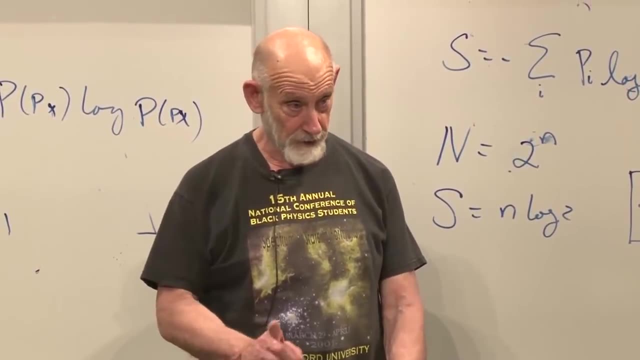 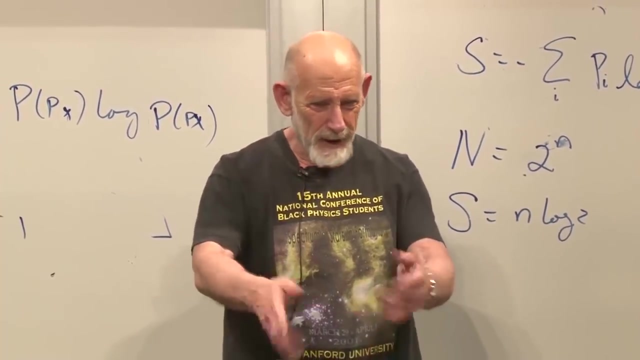 are three-quarters likely to be down. It's an interesting thing to try to calculate the entropy of such a distribution. That is correlated, of course. That is correlated because when you measure one, you immediately know something about its neighbor. Well, make up your own example like that. 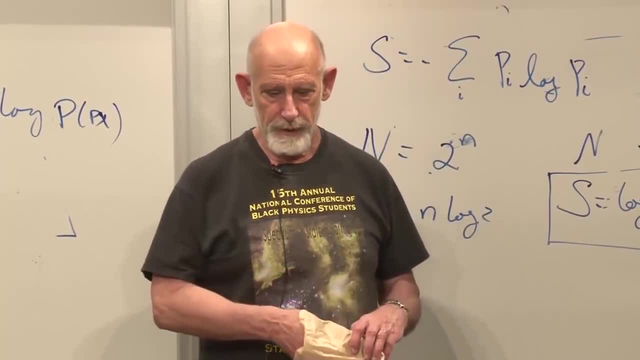 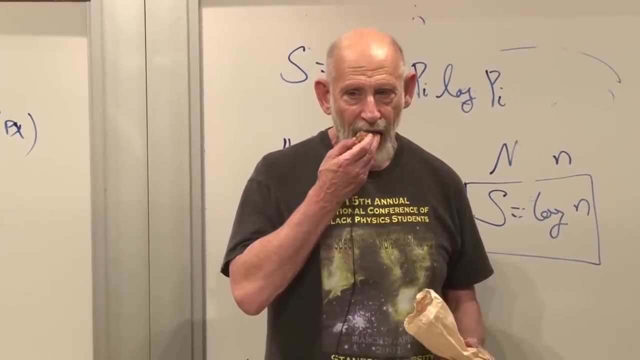 Make up your own example like that and compute the entropy. You'll learn something from it. Okay, Any other questions before we go home? Yeah, One quick one. Haddon had information theory in 1949.. Physicists had entropy a long time before that. 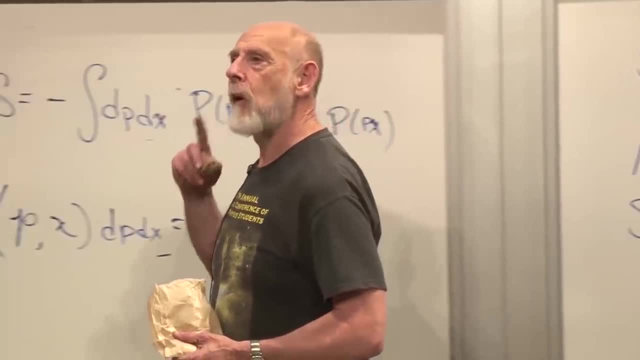 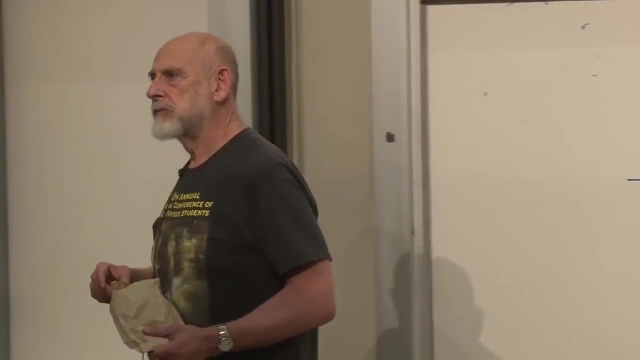 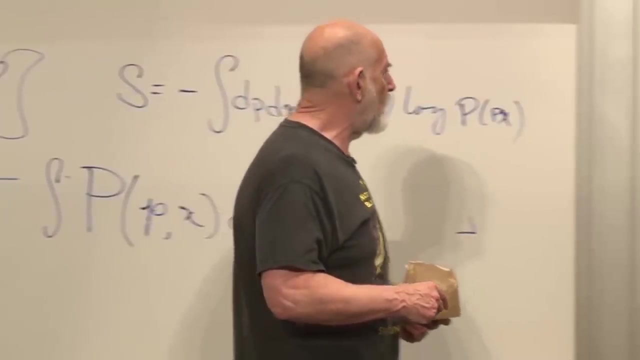 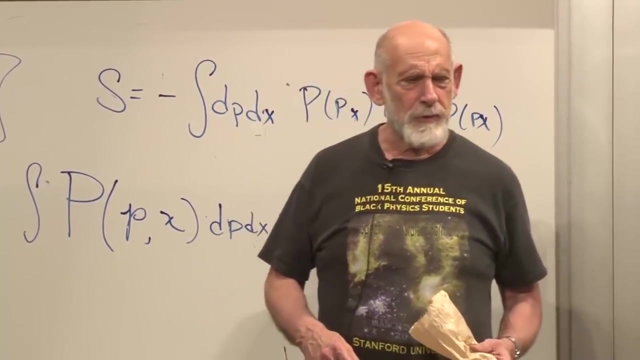 Are you still discussing the relationship between the old entropy and the new? Not particularly, Not particularly. The formula here is due to Boltzmann, I think. is this the one that's on Boltzmann's tomb? I'm not sure. 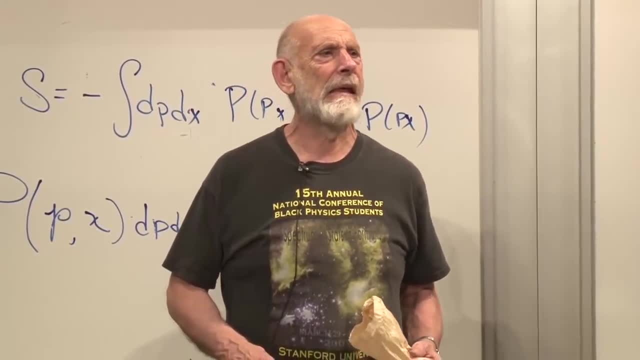 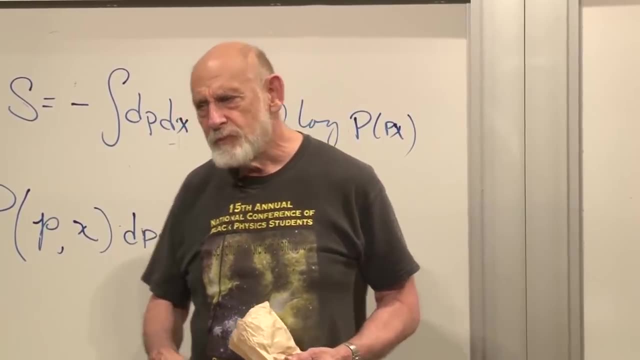 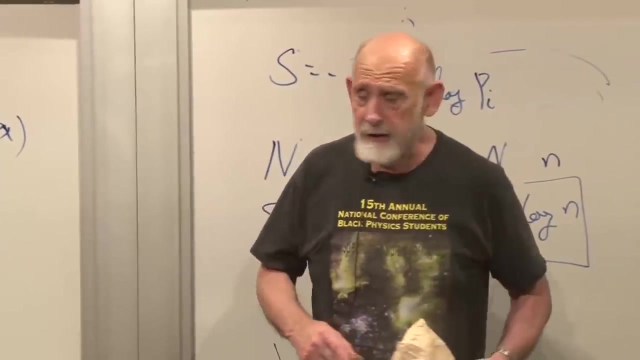 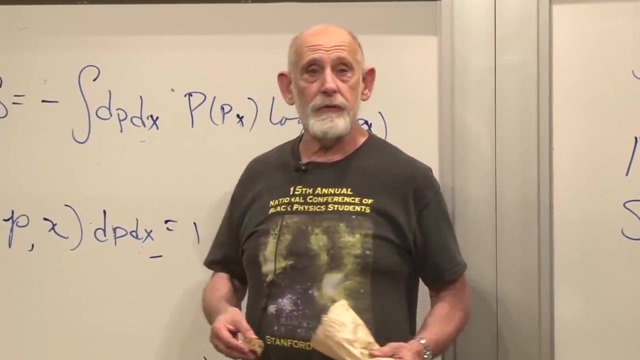 What's on Boltzmann's tomb s equals entropy minus y of w? He meant this. Well, he did write this. This is Boltzmann's formula, final formula for entropy, And the only difference between the Shannon entropy and the Boltzmann entropy is that Shannon used log two. 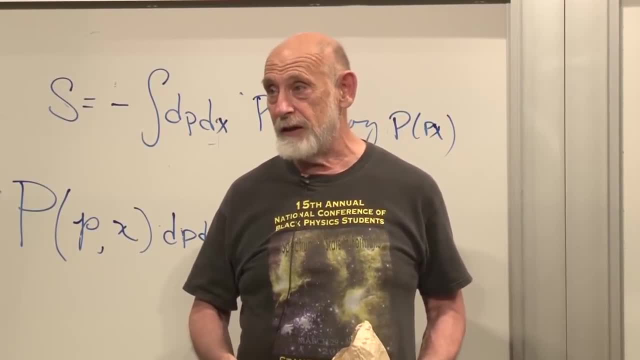 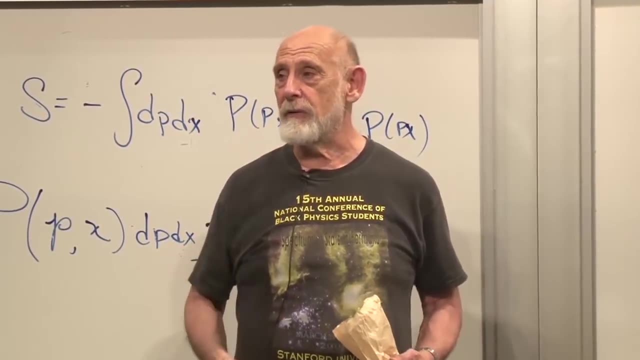 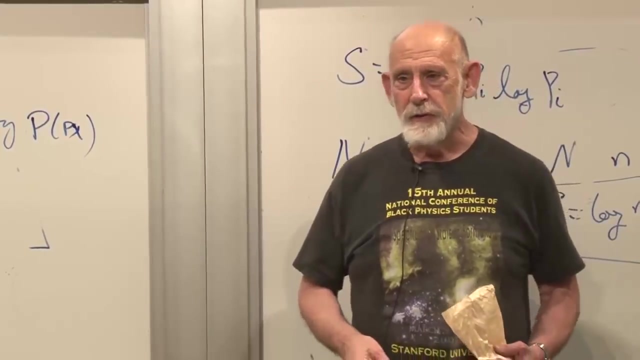 Now, of course, Shannon discovered this entirely by himself- He didn't know Boltzmann's work- And from an entirely different direction from information theory rather than from thermodynamics. but none of it would have surprised Boltzmann. Nor do I think Boltzmann's definition would have surprised Shannon. 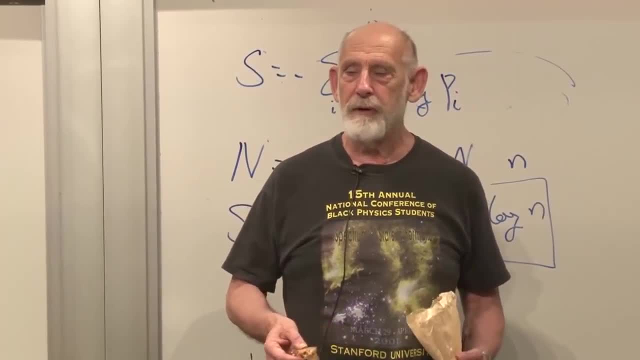 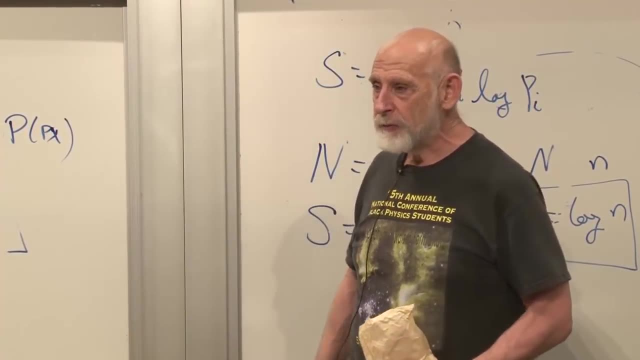 So they're really the same thing. There's no real point in comparing them because comparing them they are the same. There's no real difference. Shannon may have- I don't know whether he did or not put the minus sign in here- 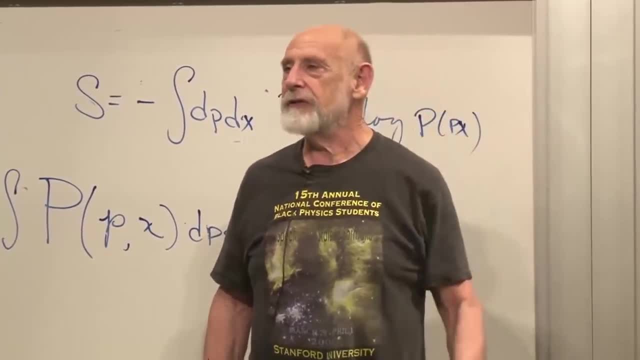 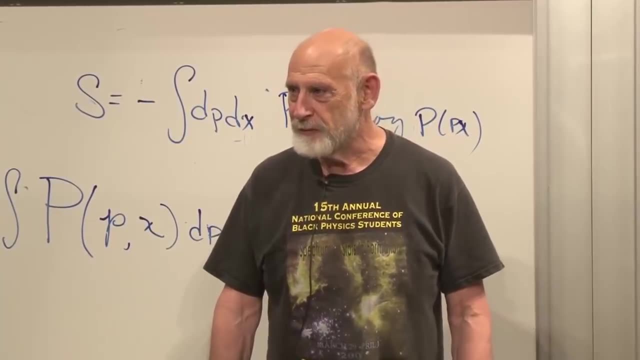 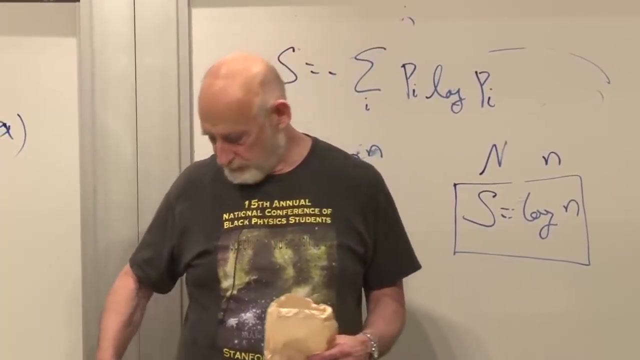 If you don't put the minus sign in there, it's called information. If you put the minus sign, it's called lack of information or entropy. So I don't know which Shannon wrote down, but anyway, Shannon wrote down entropy. 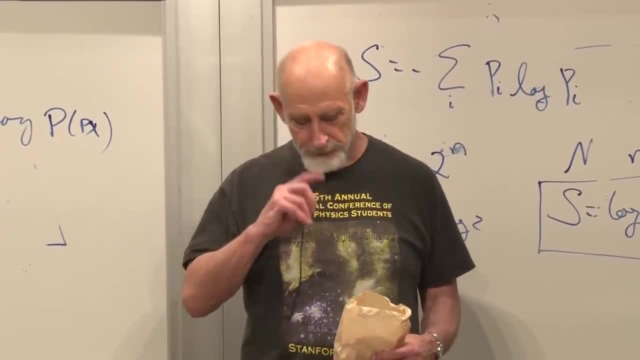